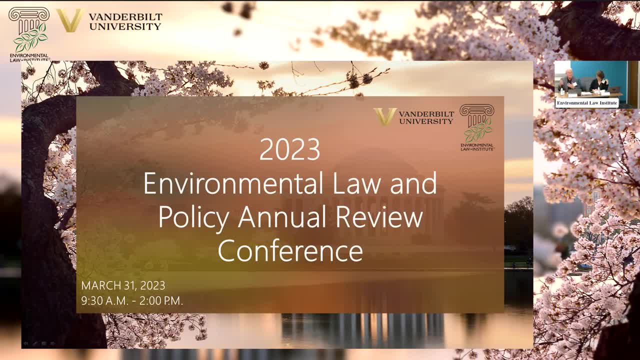 academic pieces that have feasible implications, And then we try to test those ideas out with the kind of panels you're going to be seeing today. So that's one of the functions of what we're trying to do here. A second function is that we wanted to create an opportunity to create. 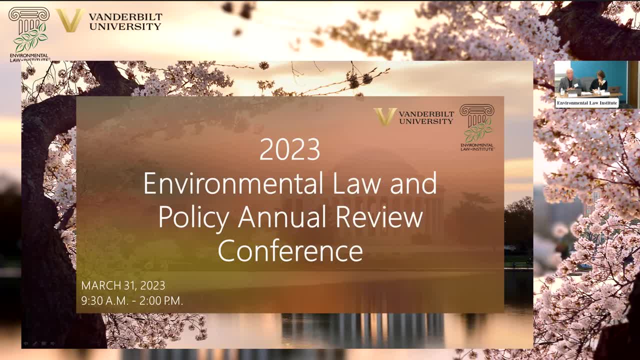 incentives for academics to write policy-relevant pieces, And I don't know about some of the academics in the room today, but I know that the first three or four pieces that I wrote, having come out of government, having come out of private practice, every one of my most wise 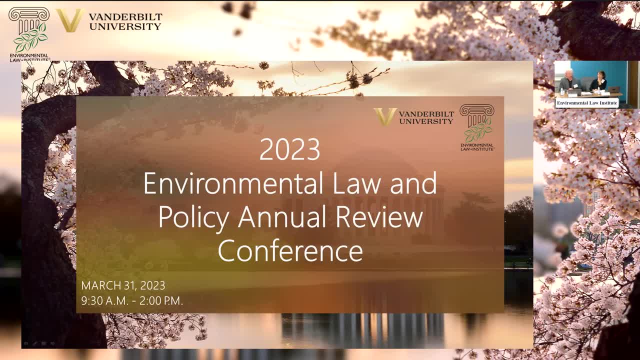 colleagues said: cut the last third of the paper. And what was that last third? It was where I said what you should actually do as a result of these really cool theoretical ideas I had, or cool empirical work, And that didn't seem adequate to me And it seems in the long run to create sort 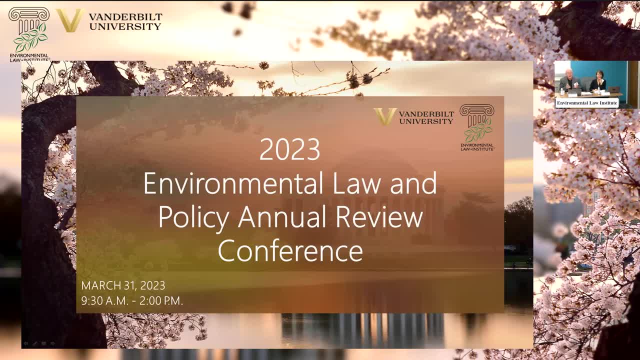 of an existential risk, Like what happens if you cut the last third of the paper And what happens if you're actually not making a difference. So another goal we have is to try to stimulate and reward feasible idea generation out of the academy and induce people, And you're going to see that. 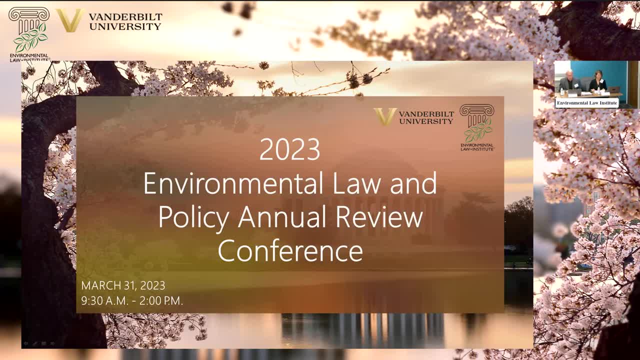 today, induce people to be able to generate those kinds of ideas and to want it to generate them. The third and most important goal of all of this- you'll see also throughout the day-to-day- which is that we want to provide a first-rate student journal right And a first-rate 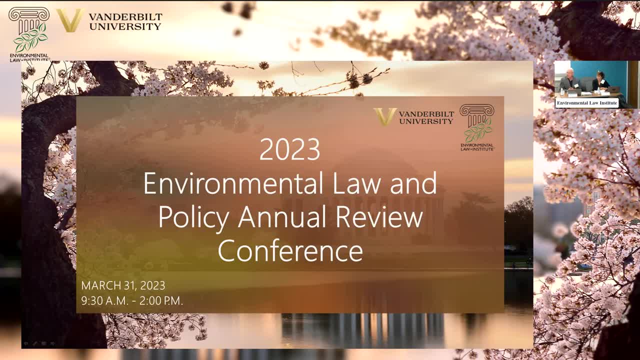 publication, with a first-rate publication, And that's what we're trying to do, And that's what we're trying to do with collaboration from ELI for our students, And so you're going to see students today making presentations, moderating panels, playing a range of different roles. The 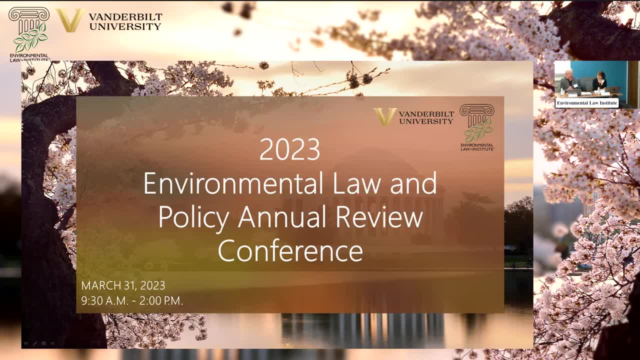 students are the core of what we do here And I appreciate you all coming to DC to do this and all the work you've generated through the course of the year. We select articles in ways that we'll hear more about in just a minute, But the idea again is to provide a journal experience for 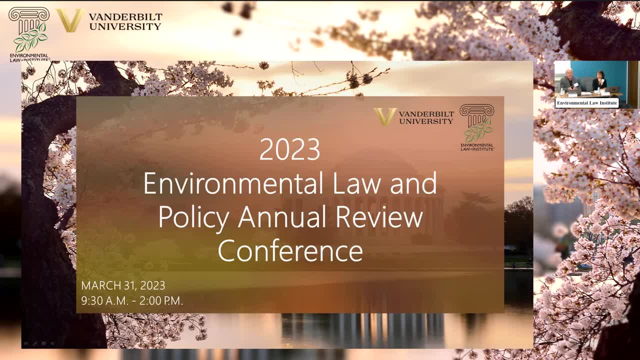 students, but also to give them the chance to have the kinds of experiences that new lawyers have: moderating panels, picking out articles, interacting with some of the key experts in the field- And we have many of them on the panels today, So that's where we're headed. 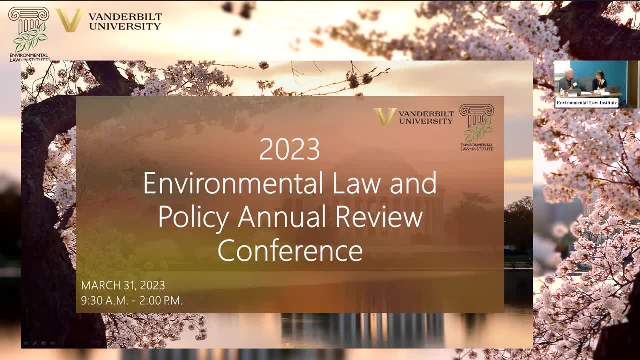 today And we're excited to do this. This is roughly 15 years that this has been going on now And we're really excited about the success. And I want to thank, while he's here, one of our first authors, JB Rule, who is my co-director on the Energy, Environment and Land Use Program, who's 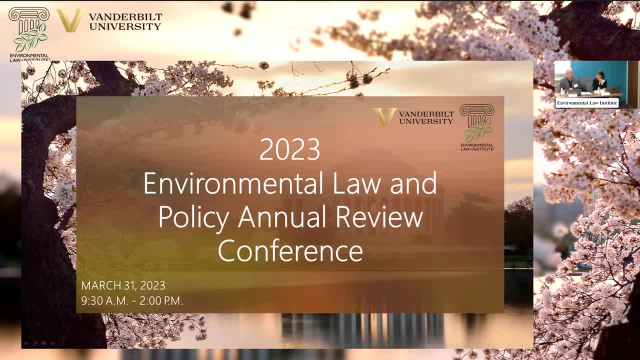 been a big supporter of LPAR through his time at Vandy And we do appreciate that Absolutely. All right, So we're going to hand it to Kristen Sarna, who is our superstar editor-in-chief and a Vanderbilt 3L, And she's just going to tell us a little bit about the process that got us here. 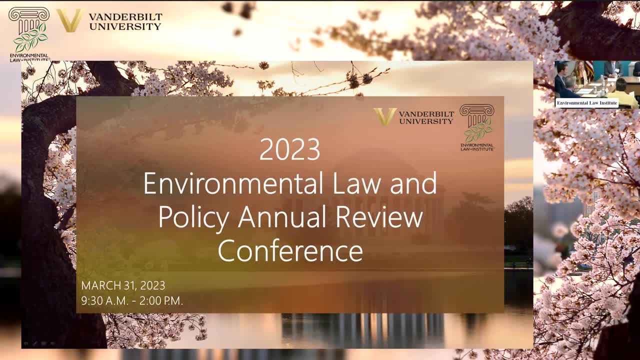 Yeah, Thank you, Good morning and welcome everyone. We are so excited to have you joining us today. Like Professor Briggins said, my name is Kristen Sarna and I have the privilege of serving as the editor-in-chief of the 2022-2023 LPAR edition. Before I jump into talking about 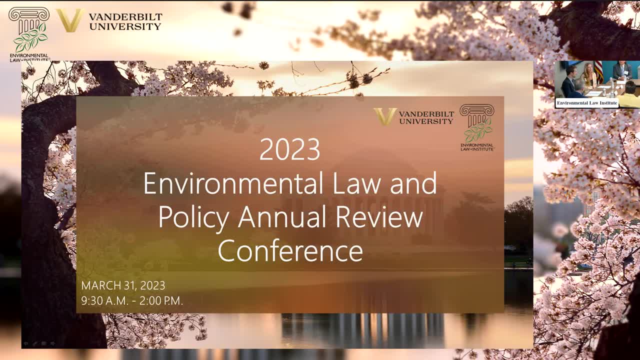 the article selection process. I want to say thank you to all of you for joining us today. I want to quickly thank the hard work of some individuals that made all of this possible. First of all, I want to thank our 21 student editors, who have worked so hard over the past. 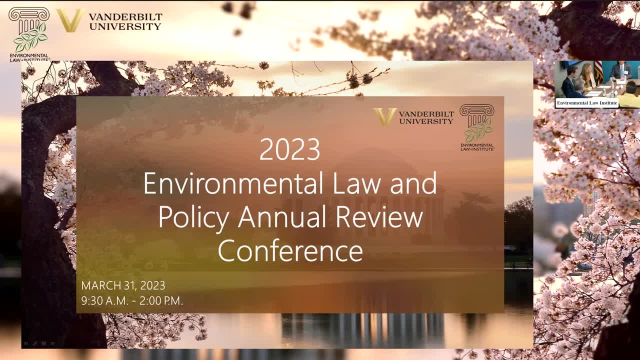 year to select these articles and prepare for this conference, as well as the work of Professors Briggins and Vandenberg and ELI Research Associate Tori Rickman. This wouldn't be possible without all of these people and all the hard work that they put into this conference and our upcoming. 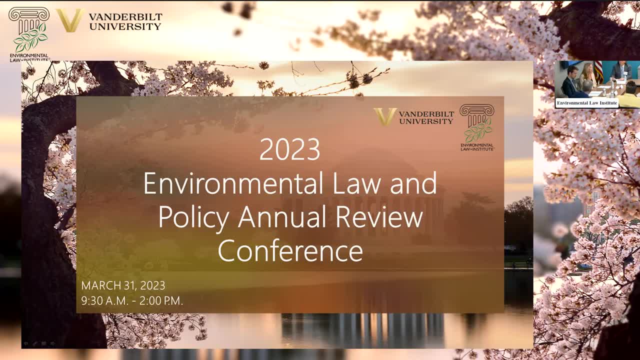 publication, And I also want to thank our advisory committee, Vanderbilt Law School and our environmental law institute. So before we get into our panel discussion, I'm going to briefly describe the LPAR article selection process that led us to collecting the three articles that we 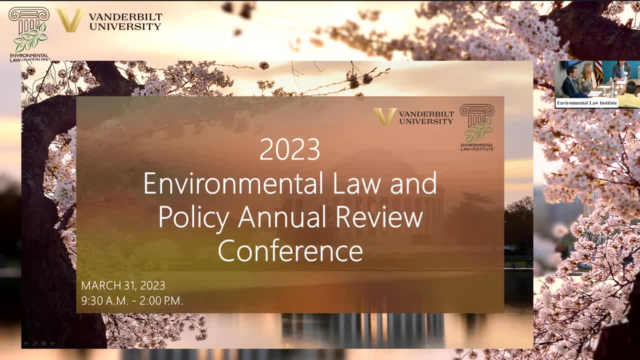 will be discussing during the conference today. LPAR is a joint publication with the Environmental Law Institute that takes place in the August edition of the Environmental Law Reporter. We republish in short and form, with expert commentary, some of the best environmental law and policy proposals and legal academic scholarship each year. 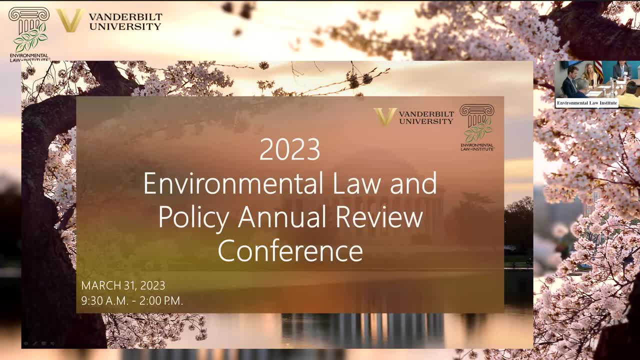 20 Vanderbilt Law School students typically participate in the LPAR process. Our article selection process begins by logging every article that mentions the word environment published in the Law Reviews of schools ranked in the US News Top 100, as well as a variety of 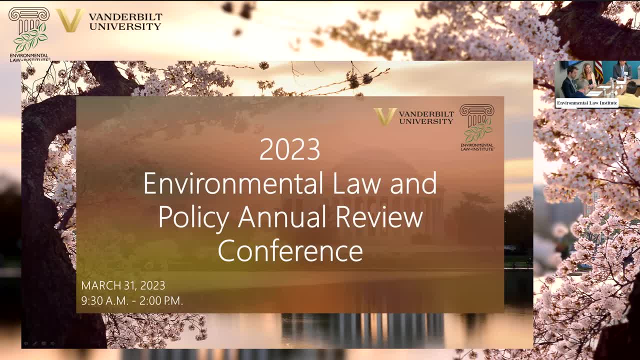 environmental law specific publications. This year, our students logged over 900 articles. We then screen these articles down to around 200 articles that discuss the environment in a meaningful and relevant way. After evaluating these article proposals based on our four LPAR criteria, which are creativity, persuasiveness, impact and feasibility, the articles are 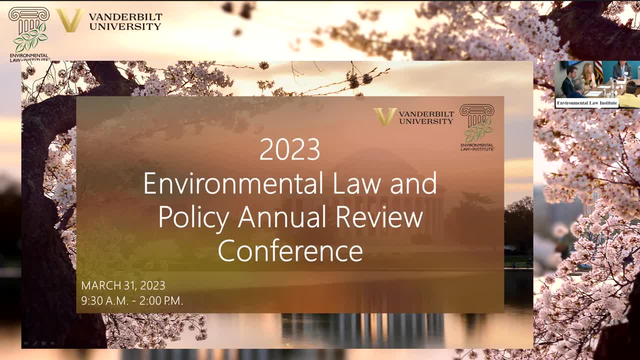 summarized by students and discussed by the entire class under the guidance of professors Breggen and Vandenberg. This process takes place over the course of two semesters and culminates in a top 20 list of the most exciting and innovative environmental law and policy. articles that we want to highlight. Our expert advisory committee works with the class to help. we'll monitor events, work on training, work on clinical research, speak about research and support our graduates in their field. This process takes place over the course of two semesters and culminates in a top 20 list of the most exciting and innovative environmental law and policy articles that we want to highlight. 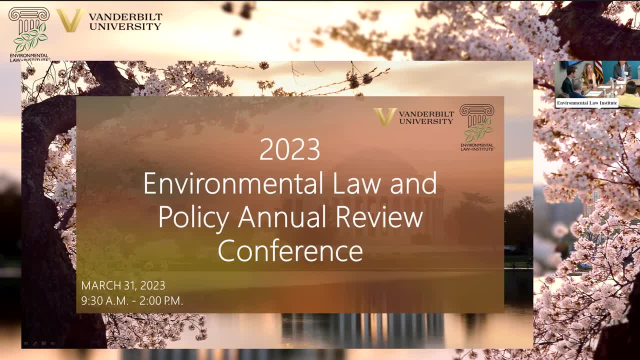 Our expert advisory committee works with the class to help proposed materials be used in the process. These articles include information and information related to the blackboard, social data, Francesca, digital learning and more. Our expert advisory committee works with the class to help narrow down that pool from 20 to just three to five articles that will be published in the August edition of ELI's Environmental Law Reporter. 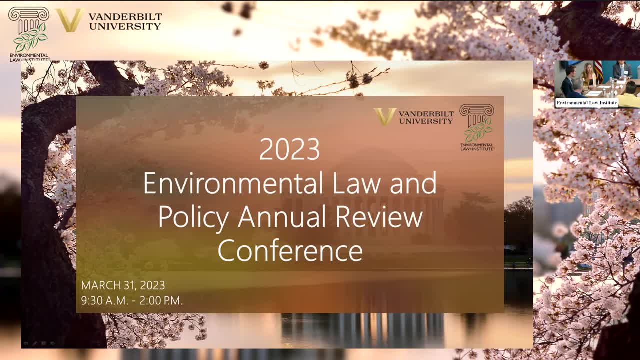 We are incredibly excited to be able to highlight three of those articles during our conference today. Thank you again for joining us and we hope you enjoy the conference. Thank you, Kristen, and thank you to our advisory committee. Some members are sitting in the audience, so thank you so much. 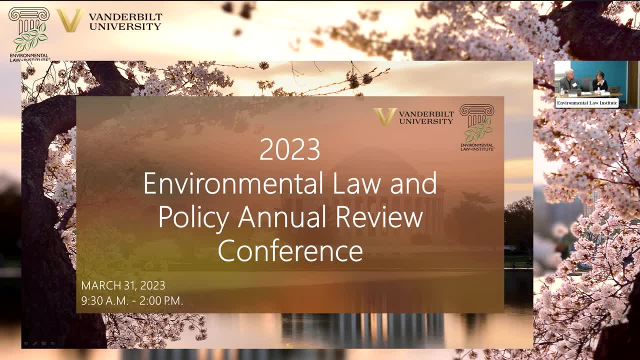 We really appreciate your input on the selection process. And before we get going with the first panel, Henry Woods, who's our development editor this year, is just going to do a little snapshot of what was in the pool, because I think it's really interesting. 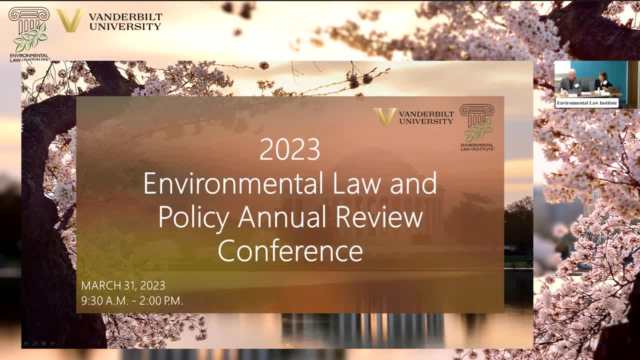 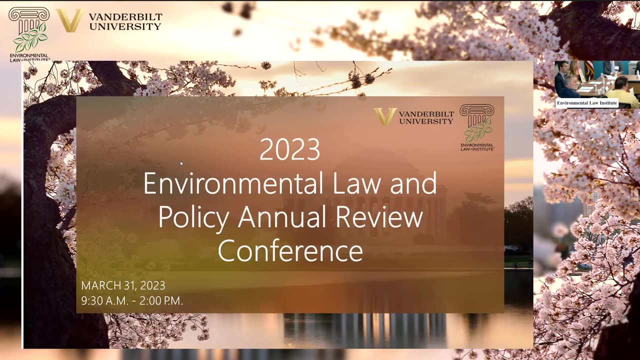 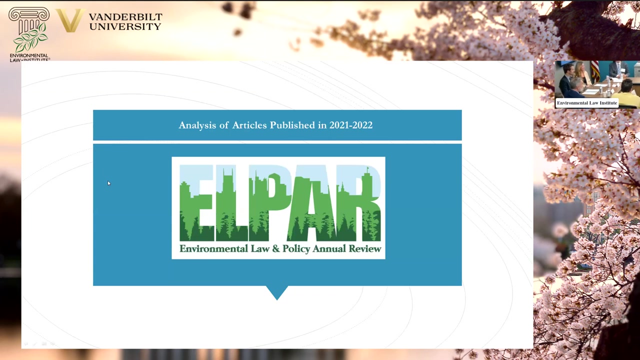 What was in the pool of articles. Yeah, thank you. You just tell Tori and she will magically turn that on Or not. You know, I'm just going to say: be patient. webinar participants, be patient. We have not done an in-person hybrid event in three years and I will tell you. we spent the better part of a whole day testing everything and I can absolutely tell you that something will go wrong. 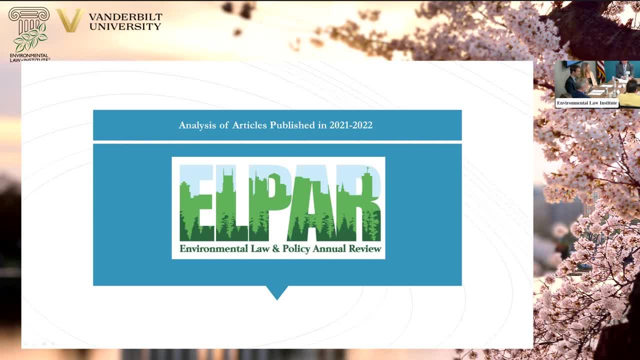 So be patient. Yeah, so good morning. My name is Henry Woods. I'm a third year law student. I've had the honor of serving as LPAR's development editor this year As part of my role to keep track of the Data and Trends in Environmental Law Scholarship. this morning, I'd like to give you a brief snapshot of the environmental publication data we have recorded this year. 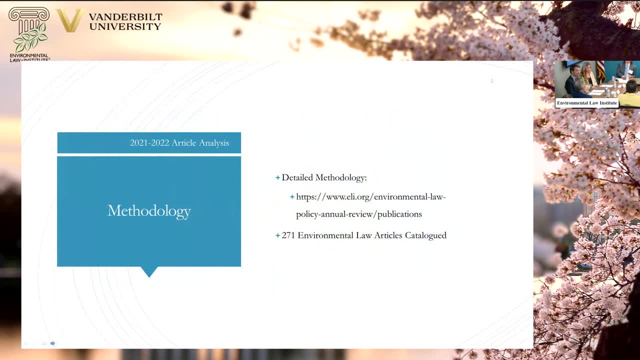 As Kristen described, we have established a methodology for evaluating articles and collecting data. If you're interested in a more detailed look at this process, the full information on our methodology can be found at the link on the ELI website. This year, we analyzed 271.. 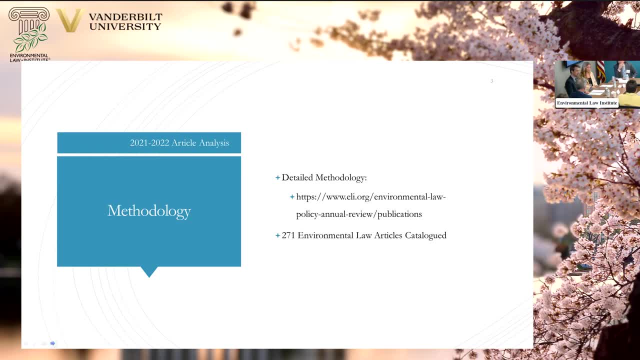 environmentional law articles. When members read through an article to assess whether it are environmental articles, they consider whether environmental law and policy are a substantial focus of the article and whether environmental topics were given more than incidental treatment and were integral to the main thrust of the article. 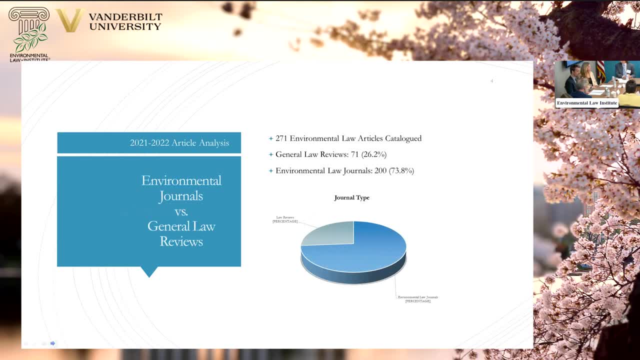 Of 271 environmental law articles, 71 came from general law reviews and 200 came from environmental law cultural items. Hundreds of articles about the environment analyzed들이 environmental issues such as exposure to novelhow We define environmental law journals as US-based specialty journals listed in the environment. 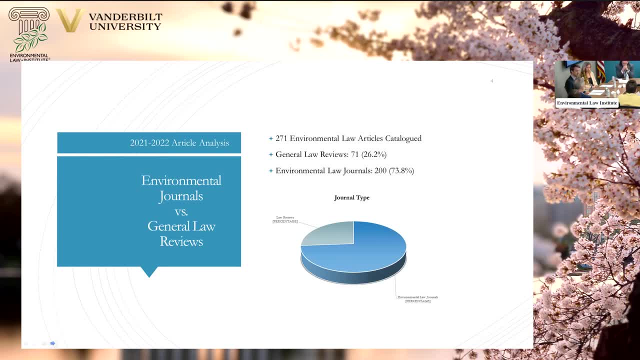 and land use, and energy and natural resources, subject areas of the most recent rankings compiled by Washington and Lee University School of Law. Additionally, as you heard from Kristen, only articles from law reviews of the top 100 law schools based on the most recent rankings by US News and World Report are looked at. 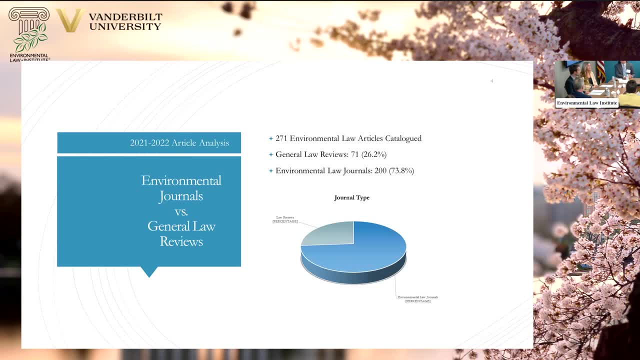 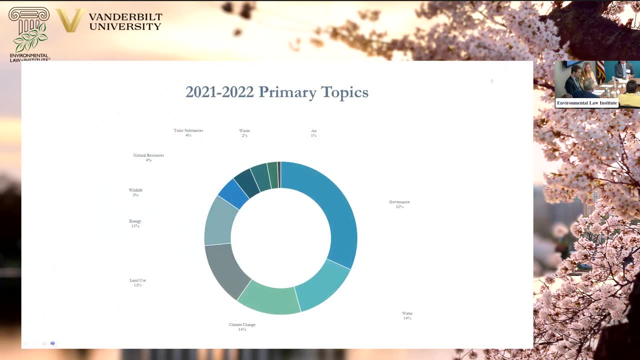 for inclusion in LVAR. We classified the articles into 10 topic categories, which are set out by the Environmental Law Reporters Subject Matter Index. These topics include air, climate change, energy governments, land use, natural resources, toxic substances, waste water and wildlife. 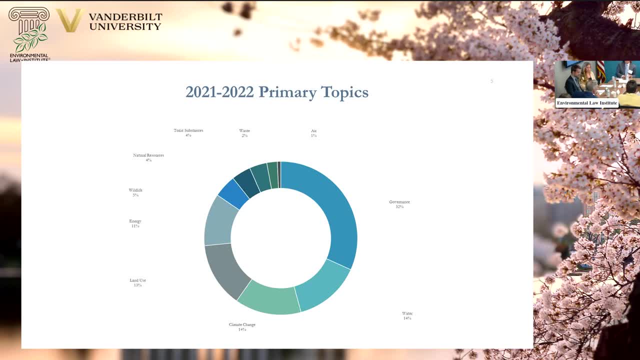 Articles receive a primary topic and also a secondary topic to the place. The environmental articles published from August 2020 to the end of the year are listed in the Environmental Law Report Subject Matter Index. Articles from August 2021 to July 2022 included 86 governance articles, 38 water articles. 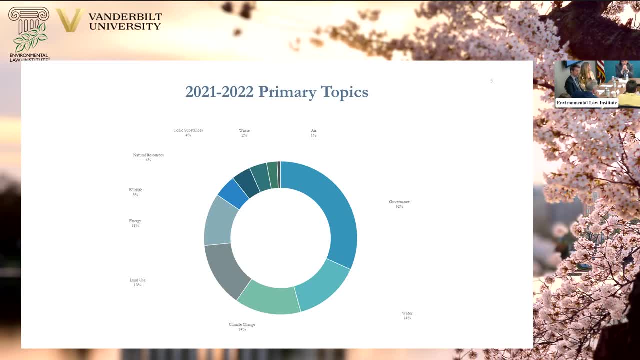 38 climate change articles, 37 land use articles, 30 energy articles, 13 wildlife articles, 11 natural resources articles, 10 toxic substances articles, 6 waste articles and 2 air articles. You can see each grouped by percentages here. 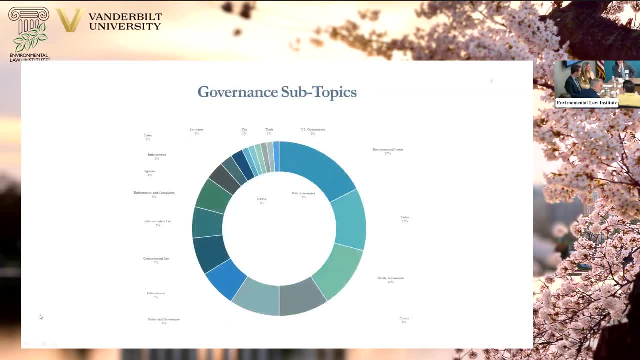 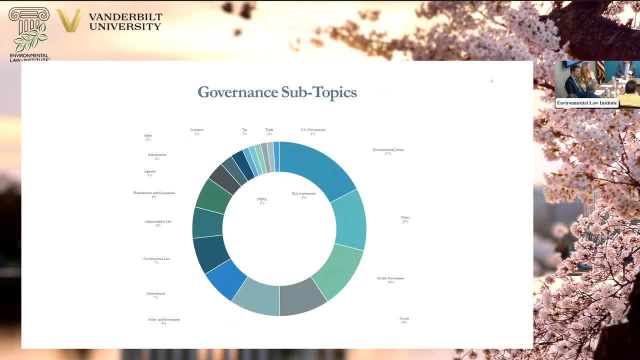 13 subtopics are included under other, with wilderness, infrastructure, estates, fisheries, pesticides and Clean Air Act being the most represented. Here we have examined the breakdown of governance articles from the 2021 to 2022 cycle, which is particularly salient as the governance category. 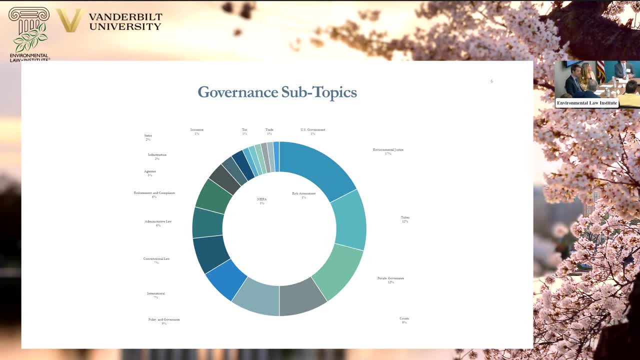 casts a wide net with 22 different subcategories. This year, many of the government's subtopics were consolidated and the private governance subtopic was introduced as well. That sounds like an important development. It is really interesting, though, like when we started this 15 years ago. 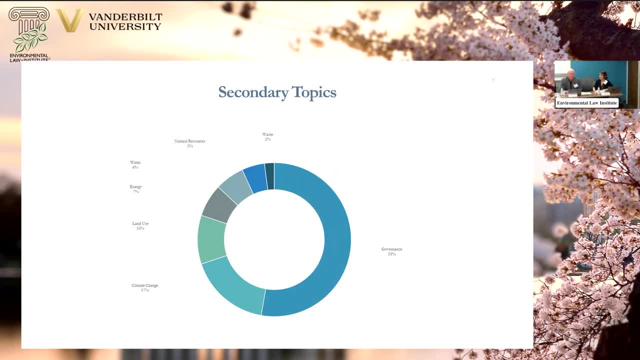 no climate change articles- right, I mean, it's been really interesting to watch it evolve. no energy articles. And for those of you who are afraid you might miss some of the substance of what Henry said, we do publish these data as a part of a summary. 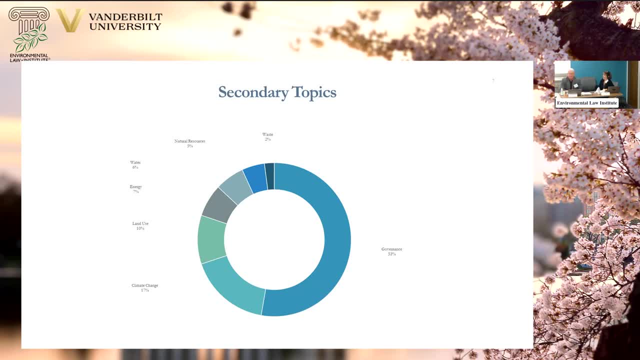 when the LPAR comes out each August, So it gives the students a publication opportunity and it'll have these data And the slides will be available as well. Yeah, so this chart tracks the secondary topics for articles where this was applicable, As many articles could be identified. 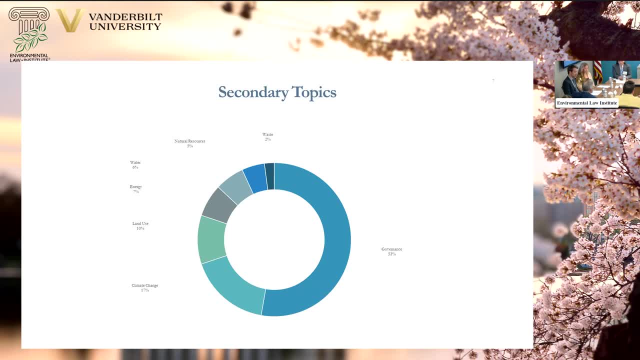 as falling under the broad net of governance, another topic, were equally applicable to the article. we labeled governance as the secondary topic, which is why governance is by far the largest secondary topics here represented. Additionally, not all articles had a secondary topic, This chart only representing 149 of the 271 articles. 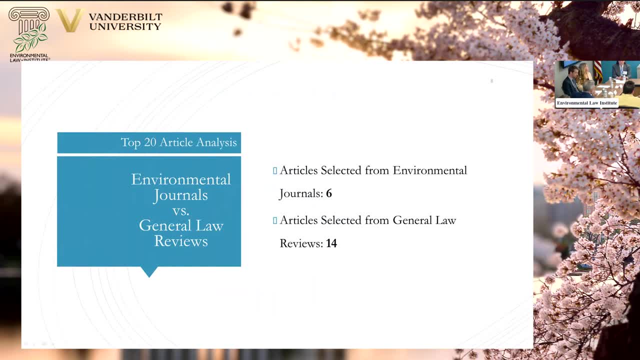 Out of our top 20 articles chosen for 2021 to 2022,, six were from environmental law journals and 14 were from general law reviews. Within this top 20, we had a range of primary topics, but the most common being energy. 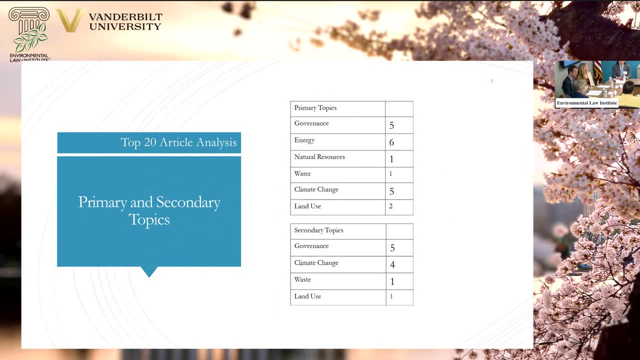 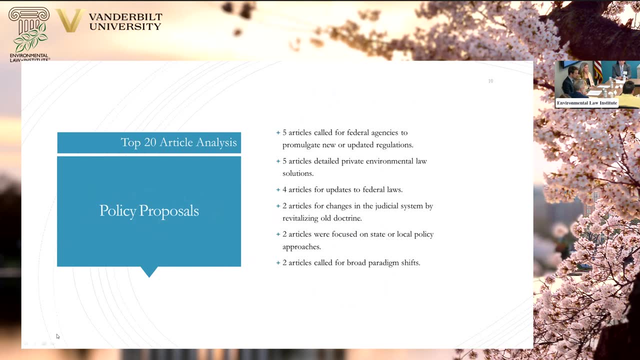 governance and climate change. You can see the secondary topics as well, although not every article had a secondary topic. as previously mentioned In our top 20,. two articles called for changes in the judicial system by revitalizing old doctrine. four articles proposed updates to federal laws. 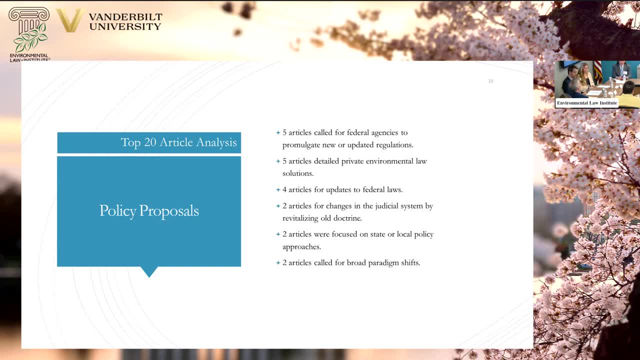 five articles called for federal agencies to promulgate new or updated regulations, two articles focused on state or local policy solutions, five articles offered private environmental governance solutions and two articles called for broad paradigms such as redesign, adaptation and response to climate change. 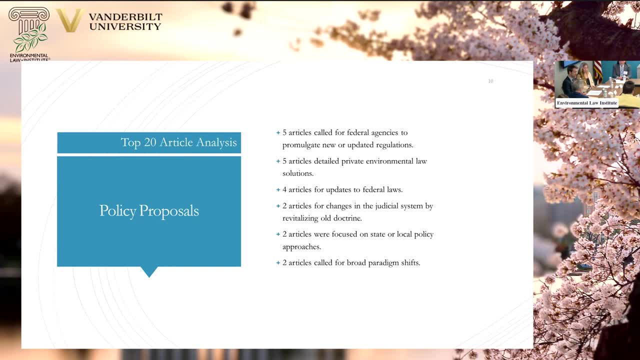 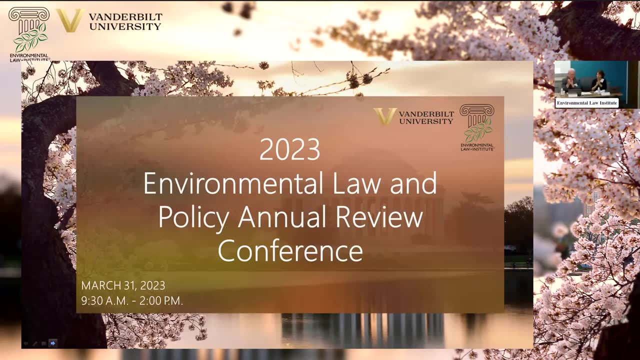 We had a great pool of articles to choose from this year and we're excited to discuss some of them today. With that, I'll hand it back to Professor Brigham Great. thank you, Henry, and Kristen and Mike. I do want to also just do a special welcome. 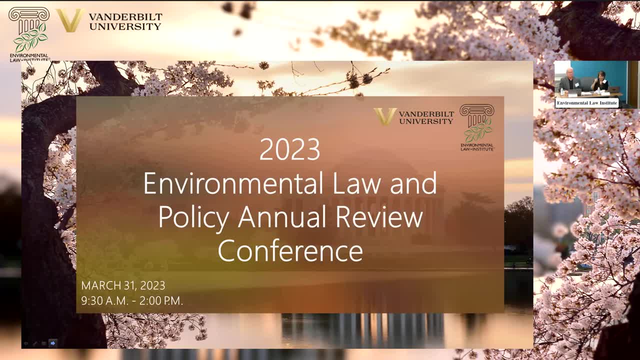 for the LPAR students and LPAR alum who are in the audience. It's wonderful to have everyone here and we also have some Vanderbilt students on the webinar. We really did just have a terrific class this year and just great, great discussions in class. 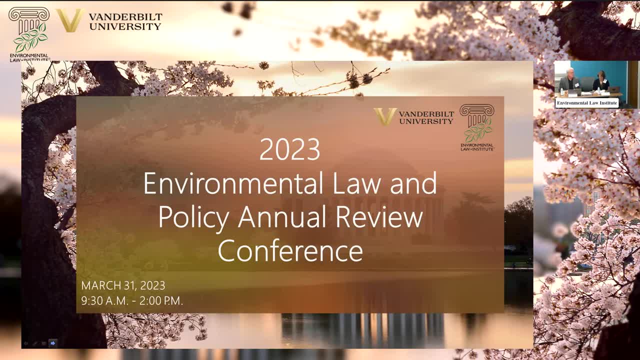 I do need to say a very special thank you to Tori Rickman, who is the research associate and has been working on LPAR for ELI. She's just basically did all the heavy lifting to get this conference together and did a terrific job. 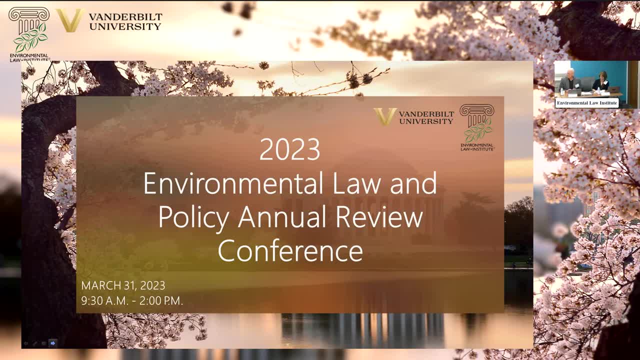 And also thank you to Colin Gibson-Tansel, our tech manager, who is on the webinar managing that, And I am not texting my friends. I'm texting the tech to make me sure that I'm talking to them. I'm texting the tech to make me sure that I'm talking to them. 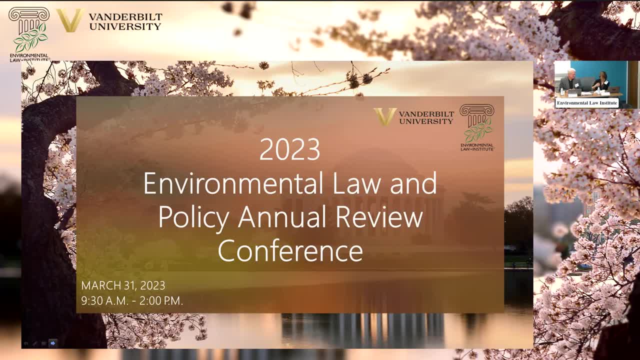 I'm texting the tech to make me sure that I'm talking to them. I'm texting the tech to make me sure everything's going okay on the webinar front as well. So basically, my job today is just to move us along as efficiently as possible. 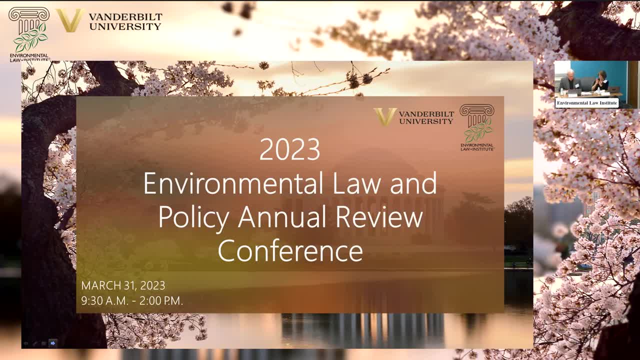 So the format for each panel is going to be as follows: We're going to hear from the authors, Then we're going to hear from each commenter, Then we're going to give the authors a chance to respond to what they've heard, which is always interesting. 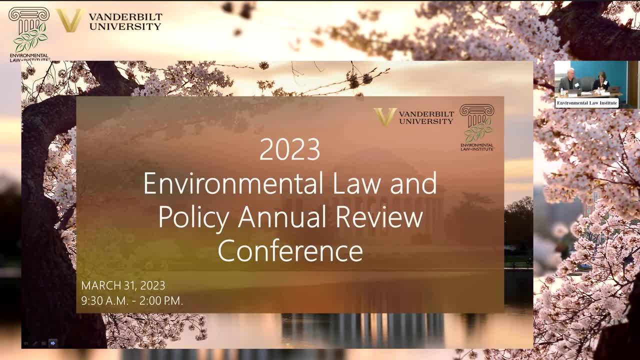 And then the LPAR student editor, who's going to start by introducing the panel, will also ask the first question And then we'll go to question and answers from the audience And I will try to go back and forth and take some from the webinar participants and some from the audience. 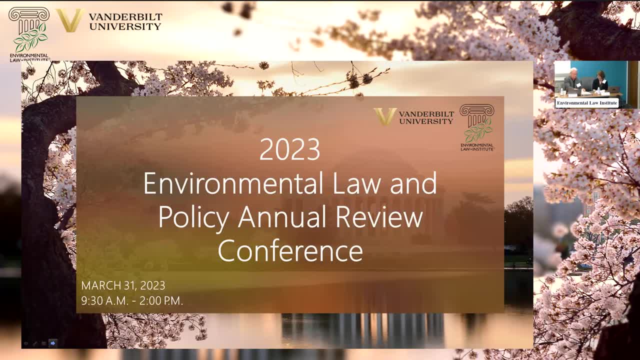 And I hope the speakers do not mind I will be making faces at them if they're running over- because we do have a very, really, really tight schedule today And the breaks are short And the reason they're short is because we don't want. 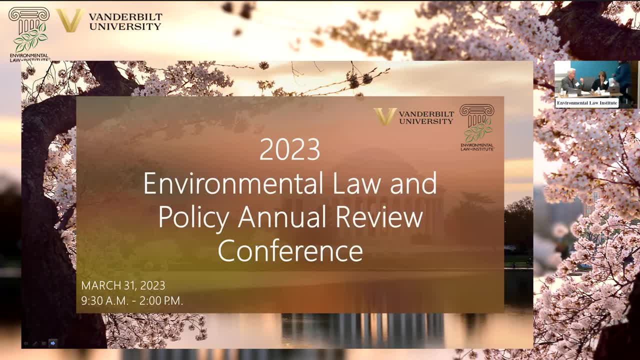 to leave our webinar participants alone for too long. But by all means, if you need to take more time, take more time. take more time. Come and go from the room as you need to. I know that we are on a tight schedule. 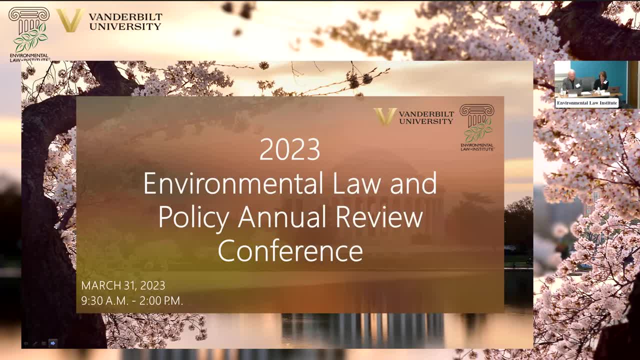 We have coffee and snacks in here. We're going to have boxed lunches later that you can pick up and have in your seat, And I hope everyone here will stay for the reception at 2 o'clock and get to meet some of the Vanderbilt law students. 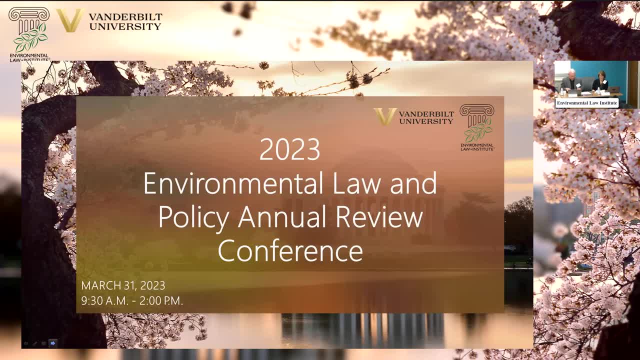 For those of you on the webinar, if you have any tech problems, use the chat And you will be able to communicate with our Tech Team, And I do want to. For those of you on the webinar, use the question box for questions. 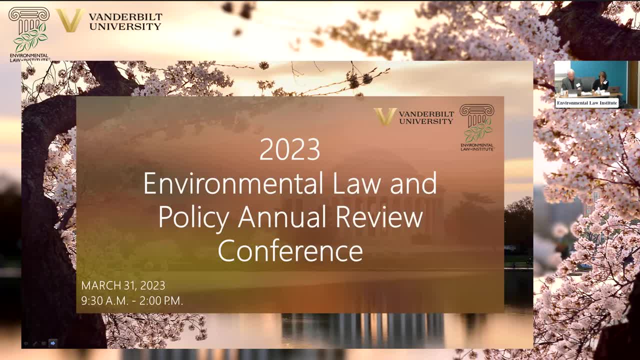 I'll be looking through them and posting some of them to our panelists. And, lastly, the audio recording of today will be posted on the LCAR website And, as I noted earlier, the slides will be available as well. So thank you so much for joining us. 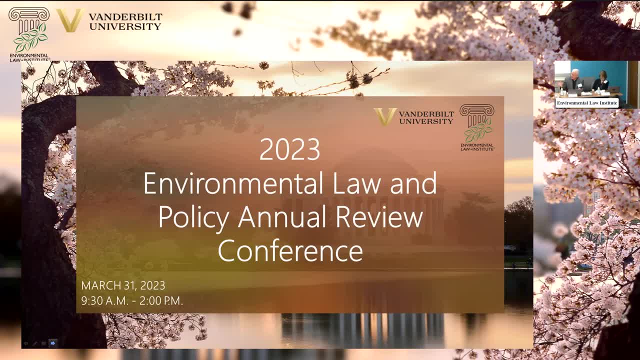 I think it's going to be a really interesting day. Do you want to say something? Can I just say that Hannah has the most amazing timing of anyone I've ever seen. I'm trying to look exactly at the right time In the audience. 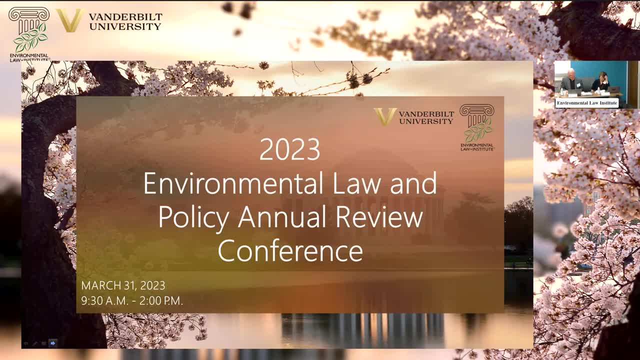 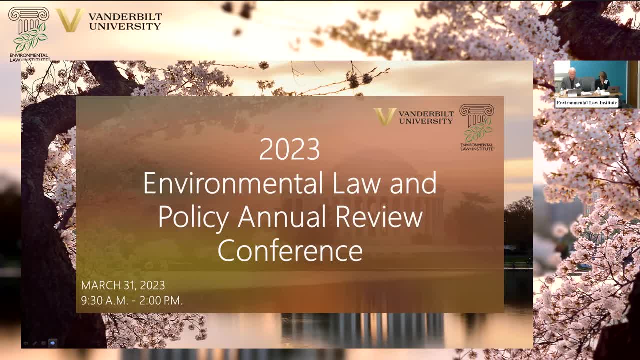 So I'm going to hand it over to Chris Burrows, who is the article editor and Vanderbilt Law student for this panel, And he's going to introduce: Oh, that's not going to work. See The best of late plans. There we go. 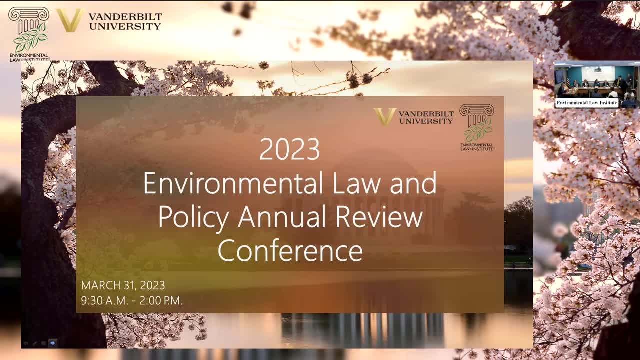 That's good. We practiced that too. You wouldn't know, This was an extremely popular panel and everybody wanted to comment, and so we ran out of students. The others will not be as good, Right? Hello and good morning. 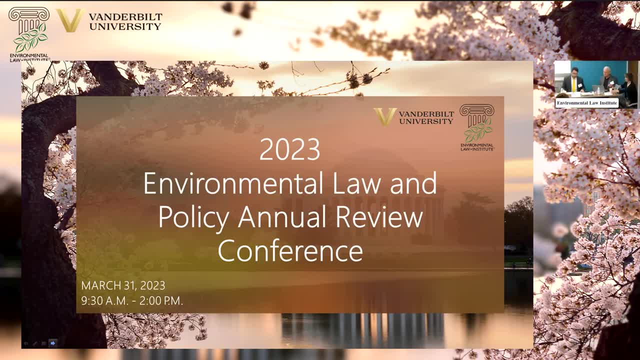 I'm Chris Burrows. I'm one of the article editors for LPAR and currently a third-year law student at Vanderbilt Law School. Today, it's my pleasure to introduce both the authors and the commenters for our first article today. Four Degrees Celsius. 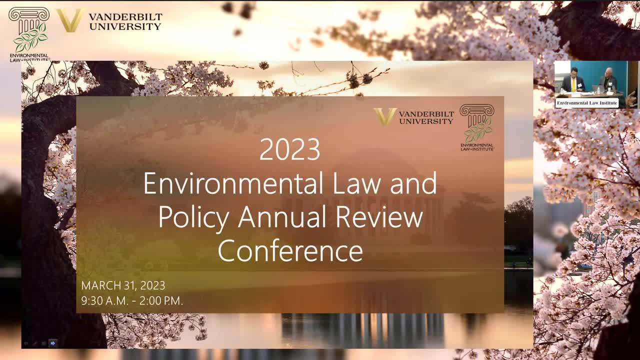 First I'd like to introduce our co-authors: David Daniels Allen, Distinguished Chair in Law at Vanderbilt University, as well as the Director of the Program on Law and Innovation and the Co-Director of the Energy, Environment and Land Use Program at Vanderbilt Law School. 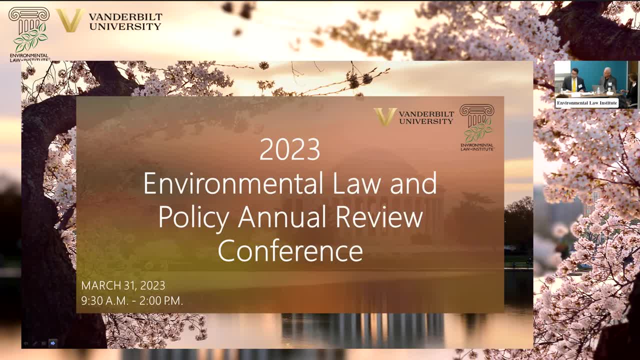 where he teaches several courses, including first-year property law, which I have the privilege of taking, as well as a seminar on climate change governance. He received his BA and JD degrees from the University of Virginia and his LLM in environmental law from the George Washington University Law School. 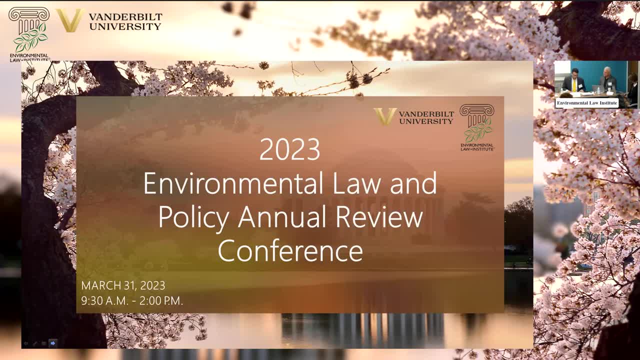 In addition, he holds a PhD in geography from Southern Illinois University. Professor Rule's influential scholarly articles relating to climate change, the Endangered Species Act, ecosystems governance and other environmental and natural resources law issues have appeared in the Duke, Georgetown, Stanford and other law journals and leading peer-reviewed. 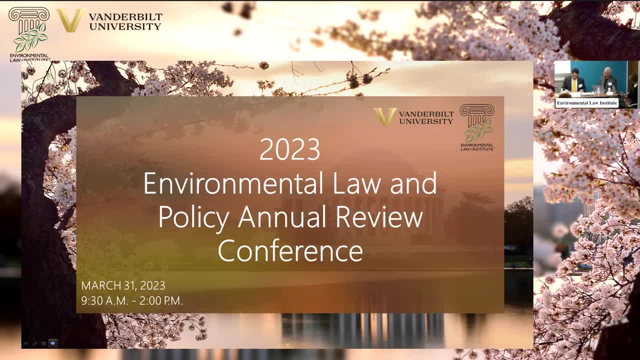 scientific journals. Robin Cundis-Craig is the Robert C Packard Trustee Chair in Law at the USC Gould School of Law, where she teaches environmental law, water law, ocean and coastal law, toxic torts, civil procedure and administrative law. 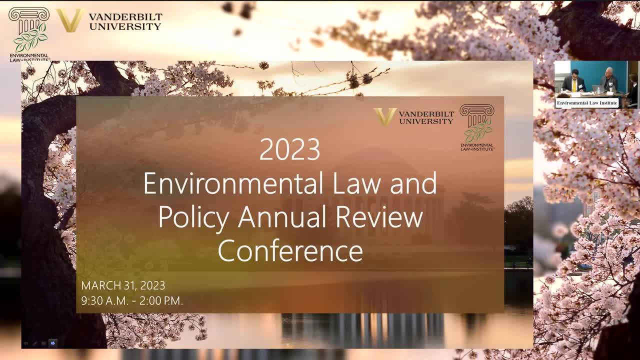 She received her BA from Pomona College in Claremont, California, her MA in writing about science from Johns Hopkins University in Baltimore, her PhD in English literature specializing in how the English Romantic poets write and write about science, and her PhD in English. 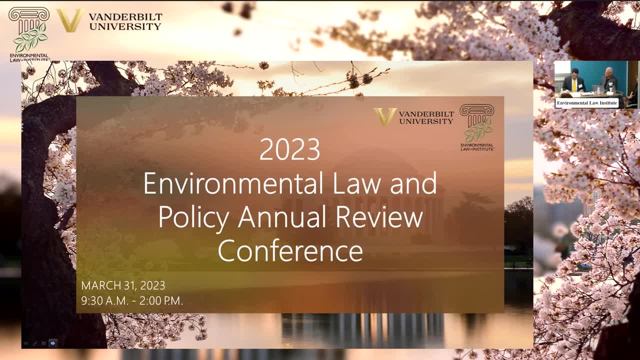 literature, specializing in how the English Romantic poets write and write about science, used contemporary science to explain social change from the University of California, Santa Barbara, and her JD summa cum laude with a certificate in environmental law from the Lewis and Clark School of Law in Portland, Oregon, my home state. 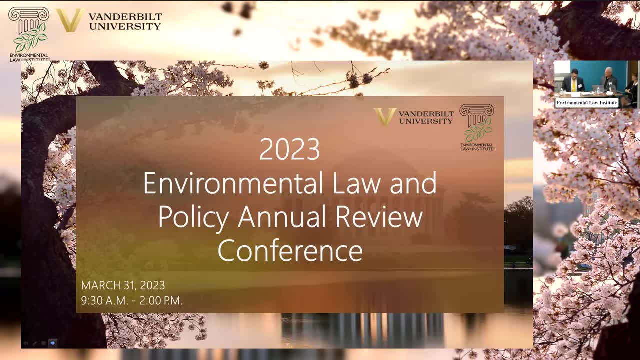 She is the author, co-author or editor of 13 books and has written or co-written over 100 law or science journal articles and book chapters. Professor Craig is an elected member of the American Law Institute and the American College of Environmental Lawyers and a member of the International Union for Conservation and Nature's. 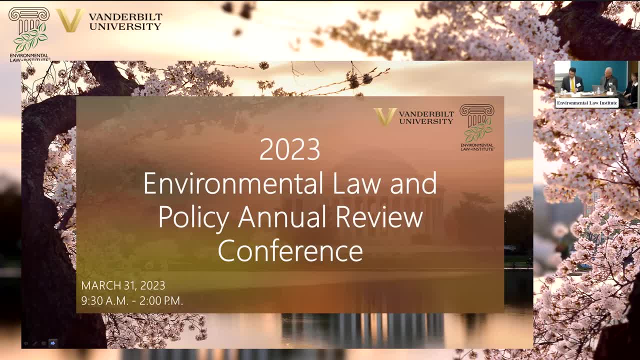 world commission on environmental law. and next i would like to briefly introduce our distinguished commenters this morning. uh, starting from the end there. um, dr rod schoonover is the ceo and founder of the ecological futures group, an organization dedicated to examining ecological disruptions: implications for national and global security. he is also a senior associate of the 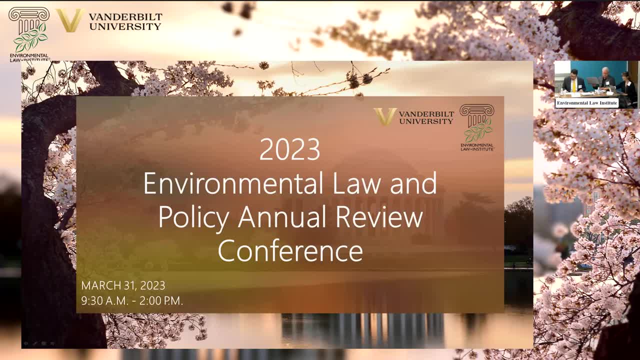 center for strategic international studies and adjunct professor at georgetown university, where he teaches climate science. he earned his phd in theoretical chemical physics at the university of michigan, where he studied complex systems. dr schoonover previously served for a decade in the us intelligence community as the director of environment and natural resources at the national 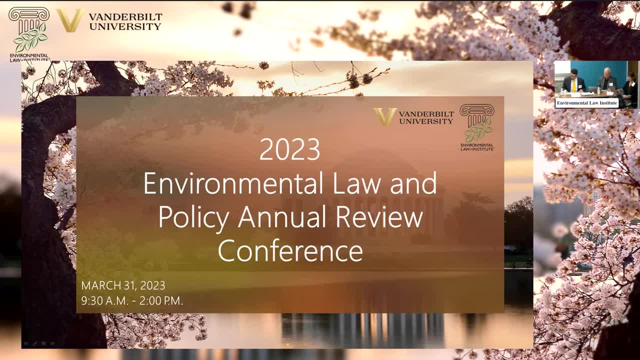 intelligence council in the office of the director of national intelligence and a senior scientist and senior analyst in the state department's bureau of intelligence and research. carlos evans is currently the director of the office of environmental quality and sustainability for the city of dallas, texas. he received his ba from the university of michigan and his jd from 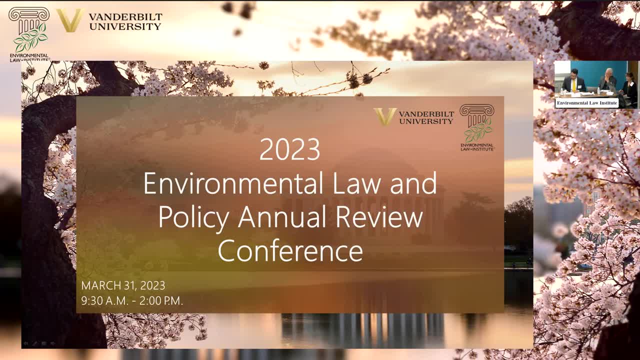 howard university school of law. prior to starting his current job in 2022, he spent two decades as an attorney at the us environmental protection agency. his areas of expertise include air and cleanup enforcement, and environmental sustainability and resilience. he has also worked as an attorney at the us environmental protection agency. 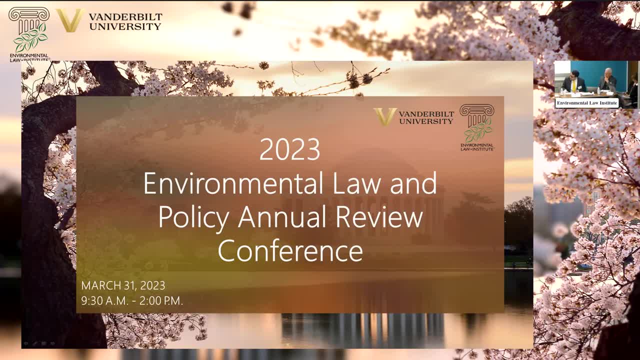 and environmental justice. hannah vizcarra is a senior attorney at the non-profit environmental law firm perfect justice, based here in washington dc, where she advocates for and defends strong federal climate action. she received her va from pomona college and her jd from georgetown university law center. 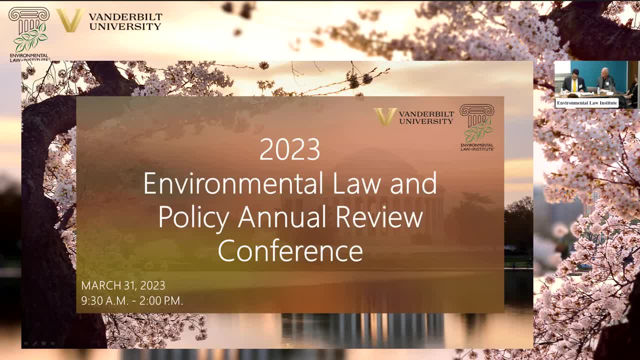 before joining earth justice, she was a staff attorney at harvard law school's environmental and energy law program, where she analyzed federal climate, environmental and energy regulation and policy and studied private sector responses to climate change. she previously practiced environmental law with two national law firms, where she worked on complex environmental litigation compliance. 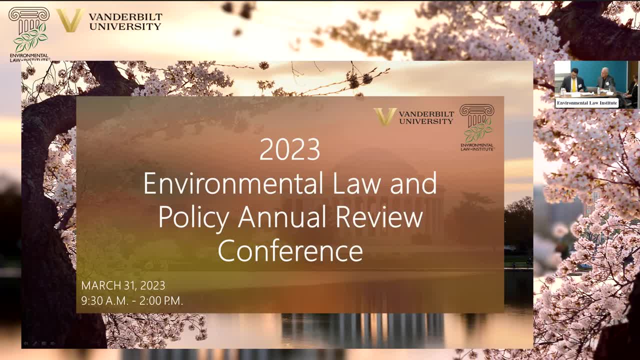 and transactional matters. and lastly, dr joel shiraga is the senior advisor for climate change adaptation from the in the office of the administrator at the us environmental protection agency. he received an a? b in geology and mathematics and physics, along with an ma in economics from brown. 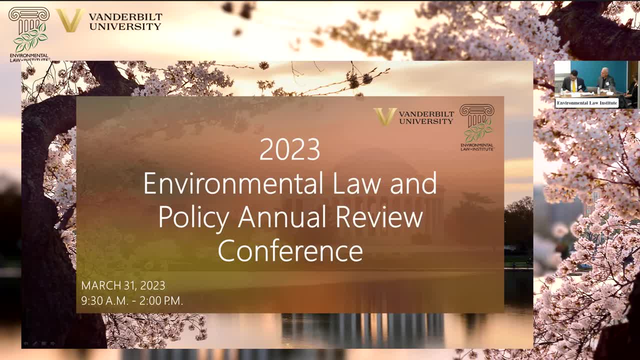 university and a? b in geology and mathematics and physics, along with an ma in economics from brown university, holds a PhD in economics from the same institution. a central focus of his work is supporting states, tribe territories, local communities and businesses to prepare for an increase in resilience to the 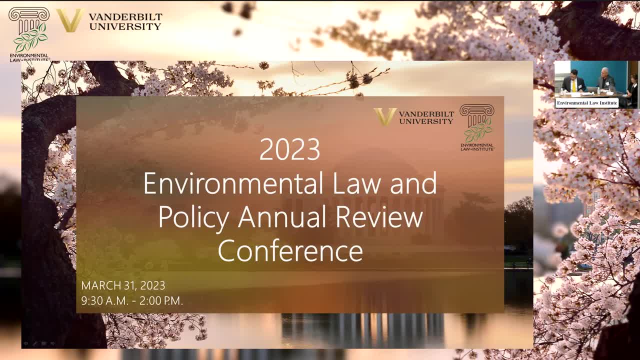 impacts of climate change. dr shiraga led the team that developed epa's new climate adaptation action plan and was also a lead author for the intergovernmental panel on climate change, which was awarded the nobel peace prize in 2007.. in december 2015, dr shiraga was honored with the 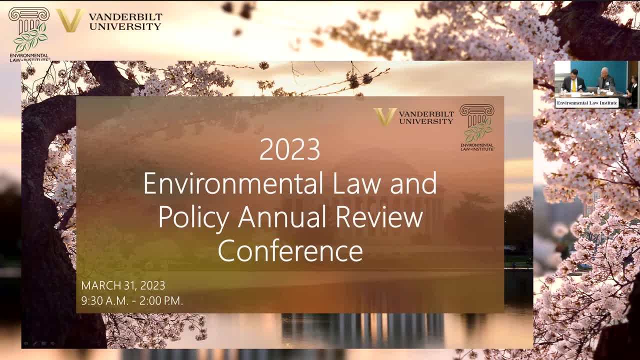 ац was parties that developed the us climate adaptation action plan and is a political award, the highest honor given to career members of the federal senior executive service. thank you, chris. as you can see, we have a real group of underachievers here. we're handing over to. 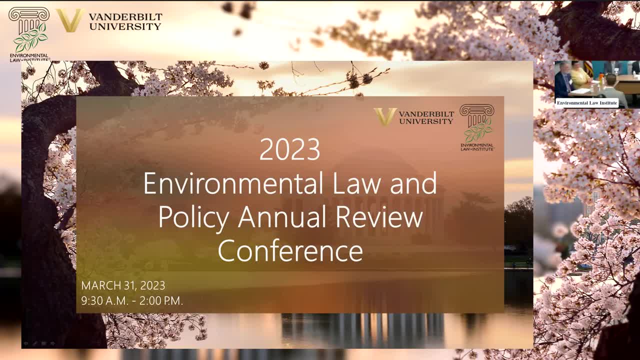 professors rule and describe. thank you, thank you well. okay, we're starting the day with doom and gloom, but first, on behalf of both of us, thank you to lpars for organizing this event and the article selection and editing process. lpar is truly the true sense of the unique student. 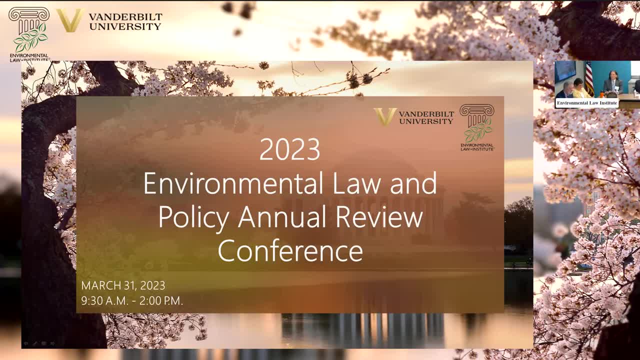 experience in legal education. there's nothing else like it, and i think it's really uh very distinctive and rewarding for our students. i see some of the former lpar students uh in the audience. uh also thanks to mike and linda for creating lpar and sustaining it so ably and of 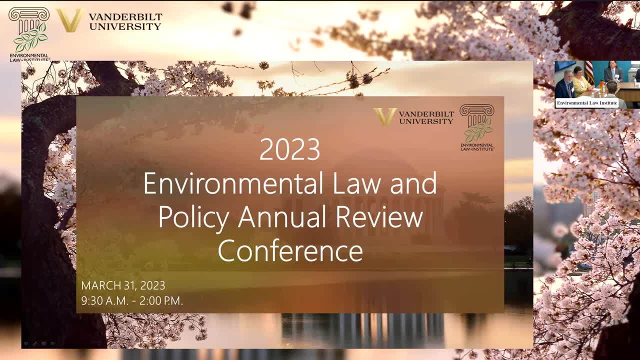 course, all the students knowing how much thought and effort the lpar team puts into their article select and editing process, it's a tremendous honor to have had our article selected, thanks also to eli. it also is a truly unique institution in environmental law and policy. it is a long 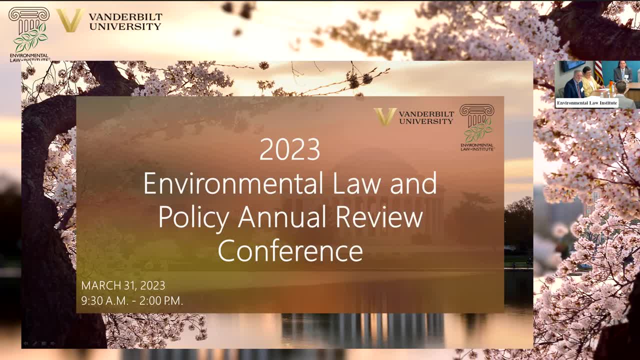 provided a robust place for convening, elaborating and innovating. thank you also to the panelists, and first thanks to my co-author. both enjoy writing the kind of scholarship that connects with lpars, and a lot of us have a tremendous interest in what it's like to be part of the green. 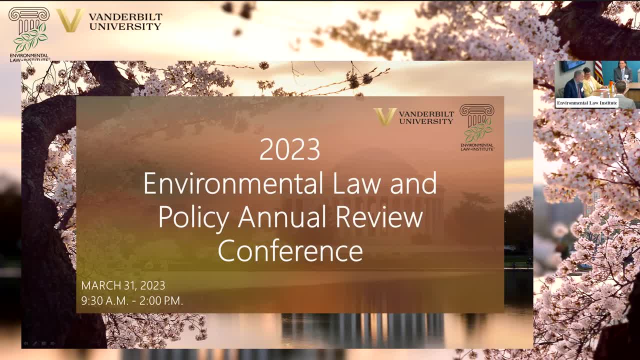 student engagement program and being involved with the informatic stakeholders in the school of law and policy at least in a very unique way. and first of all, thanks to lpars for putting together this drei-part document, as well as the first screening for the pre-Isabel ziel and the second screening for the student. 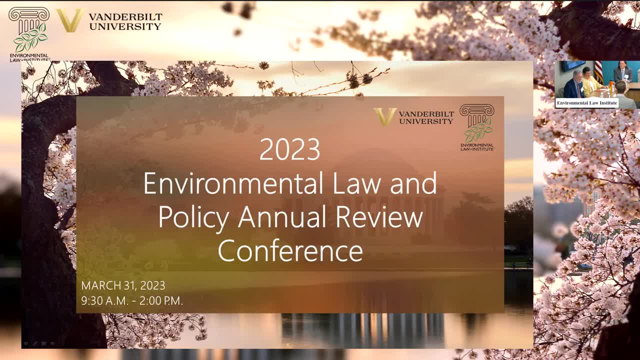 engagement program and the third screening for the student engagement program, and those, of course, are both excellent students. it's a wonderful opportunity to help them come together and talk about the world of instruction. thank you so much. the lpars is a great place to be and we look forward to your visitation, as you can see yourself as a student at lpars, as well as the 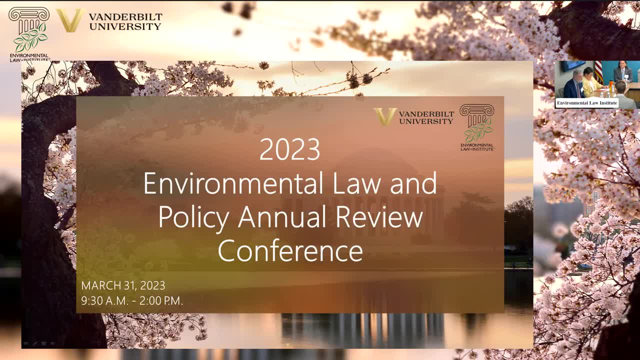 team got pushback, some of it aggressively, The idea being that promoting adaptation would lead to complacency and undercut mitigation policy. Our position was: hey, climate change is already here, The need for adaptation will be inevitable. But that resistance had led to what 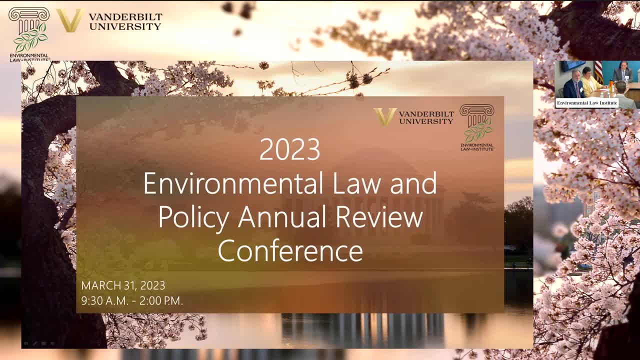 we call an adaptation deficit. We needed to start thinking about adaptation planning and policy fast. The resistance softened And I think by 2015,. it's fair to say there was a robust dialogue in legal scholarship on adaptation policy, But actual on-the-ground planning. 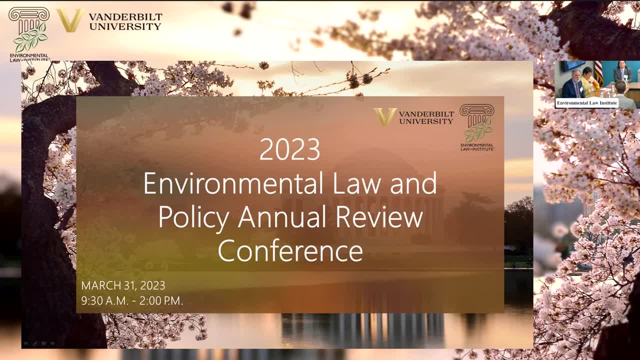 was still getting off to a slow start. Looking back on that pivotal year, the Paris Agreement ironically helped lead what we call decoupling of mitigation and adaptation policy, in the sense that both became locked on the Paris Agreement's goals of keeping warming. 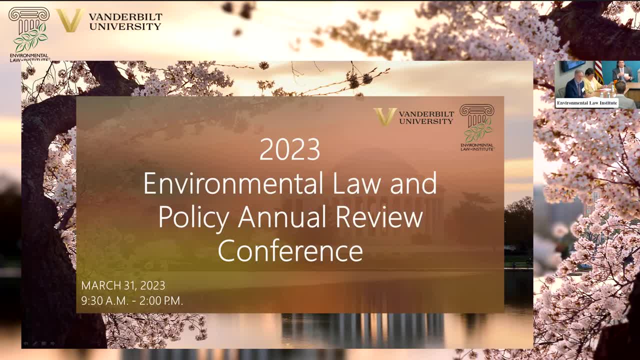 to 100%, 1.5, at worst case under 2.0. But those internationally committed goals for mitigation, it made sense to use them as a platform for building adaptation scenarios as well. I think it's fair to say also that the sense in the United 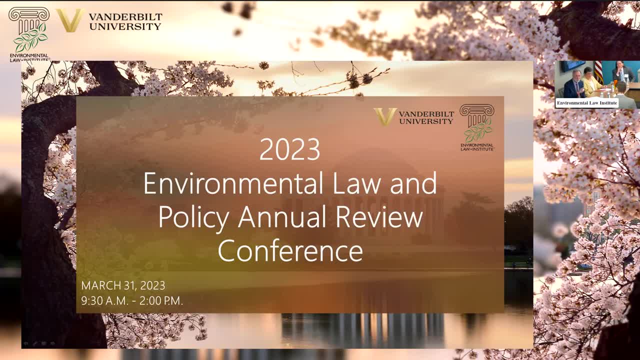 States was: we're going to be dealing with climate change, but it's going to be a lot worse elsewhere. In fact, the extent that climate migration was a policy topic, it referred to people leaving other nations, more distressed nations, And I think it's important to see climate refuge. 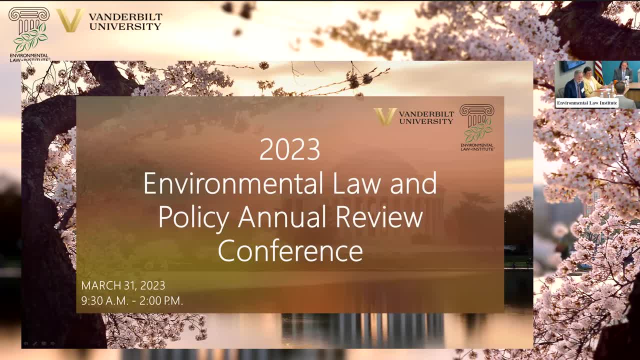 in the United States, Most adaptation planning at the federal, state and local levels fit into what we call an analytical climate group or in situ climate adaptation. The idea was that for a strategic blend of resisting threats such as sea winds, building resilience through better flood management. 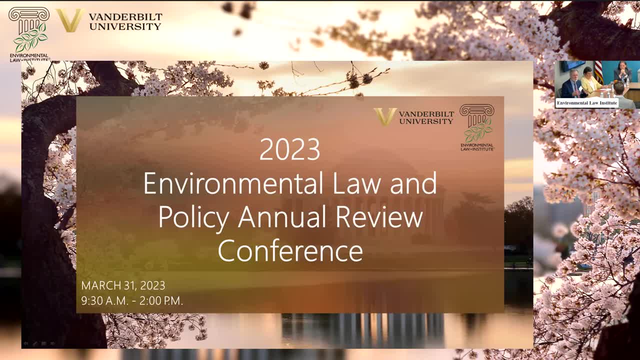 and to a much lesser extent at that time, managed retreats such as pulling back from coastal areas. We could deal with climate change in situ and keep communities basically intact. Some local plans did discuss more extreme scenarios but really did not put that to the test. 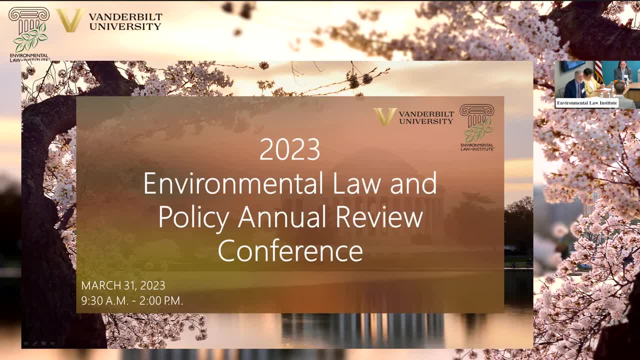 in their actual planning and policy By 2020,. if you were like we were long sunk climate science, digging into the climate science in the most prominent scientific journals, it was clear that the chances of achieving 1.5 degrees- 1.5 degrees- 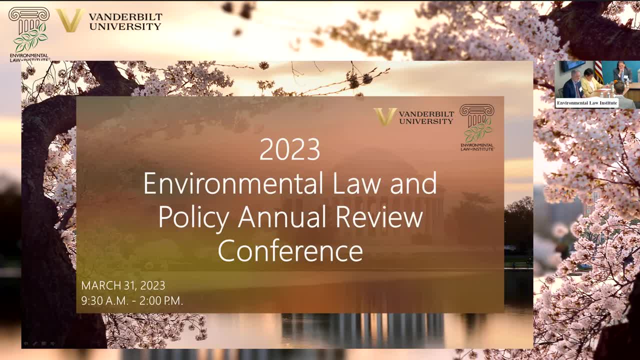 in the most prominent scientific journals, it was clear that the chances of achieving 1.5 degrees in the most prominent scientific journals, it was clear that the chances of achieving 1.5 degrees centigrade as our upper level were approaching zero. 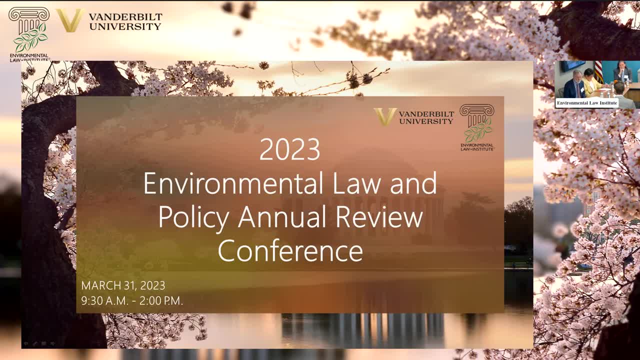 And the probability of blowing past 2.0 was rising and likely already passed. more probable than not Depends on you know what you read and what you believe, But in any event the climate change goals in the Harris Agreement were diminishing in probability. 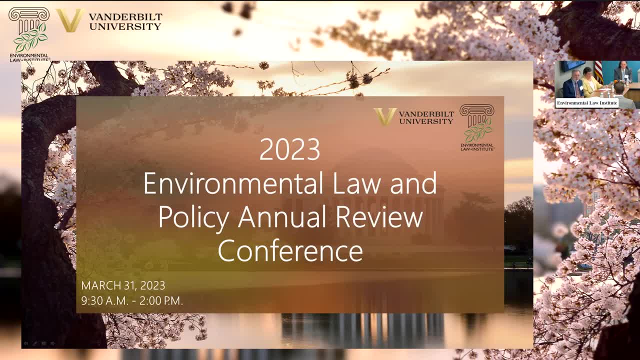 Well, that was the premise for our paper And we expected some resistance to that conclusion from our law professor colleagues and other readers. So we devoted 13 pages of this article to making the point using the best science and synthesizing it and translating it into policy. 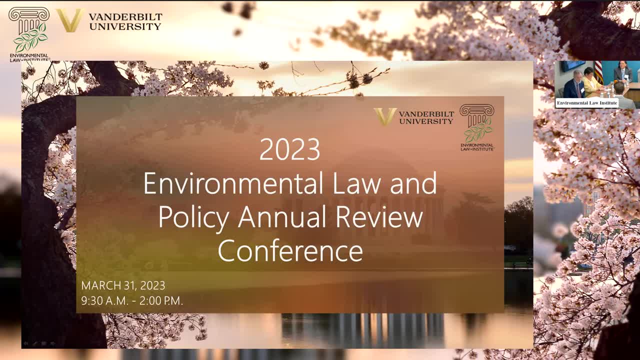 To make the point that we need to begin thinking about it beyond two different sea worlds. We worked in great detail through the current state of science, emissions, climate conditions, carbon budgets, emissions trajectory and the latest research on climate sensitivity. You know one of the footnotes. you know one of the footnotes. you know one of the footnotes. 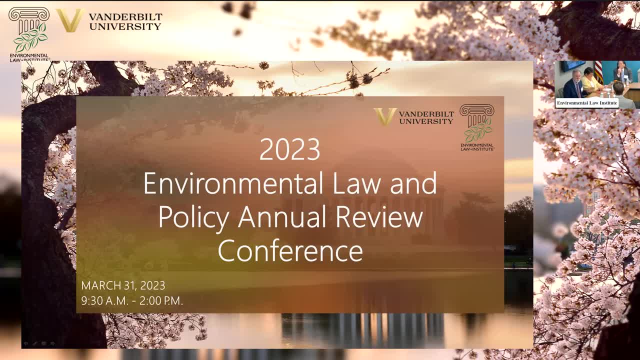 we suggested that. well, maybe in 10 years that part wouldn't be necessary anymore, because we'd either be living in a 1.5 degree C world already or that would be a given. And last week's IPCC report. 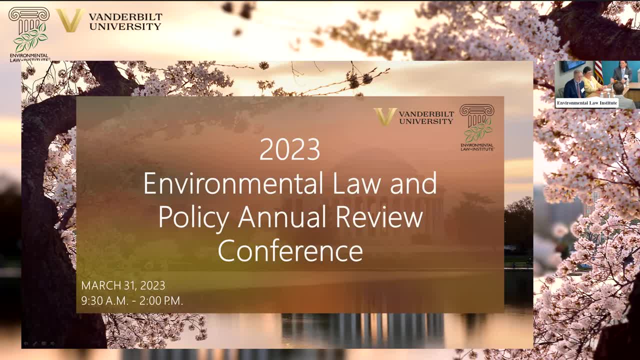 at least on the 1.5 degree C world suggests that that would be the case, and it would save us a lot of work. So I do commend the LSAR students who edited our article for condensing that 13 pages into two paragraphs. 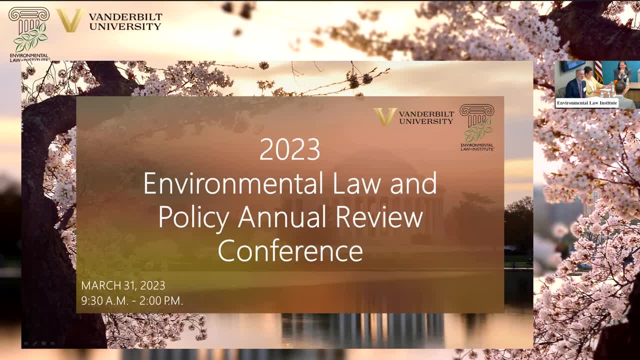 Point, there you go. So, in short, there seems to be little debate with the last sentence of that now shortened discussion. Barring rapid global political, social and technological transformation, we will be fortunate to limit temperatures by 2.6 degrees centigrade. 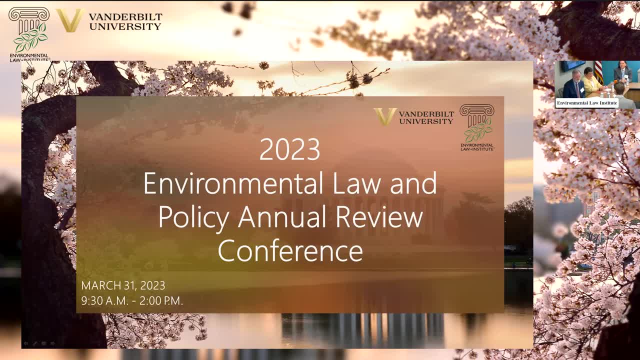 Possibility of reaching four degrees centigrade cannot be ignored. But taking that as a starting point, the central arguments of our article is that mitigation policy and adaptation policy must be decoupled. Allow adaptation policy to actively engage beyond two degrees C scenarios. 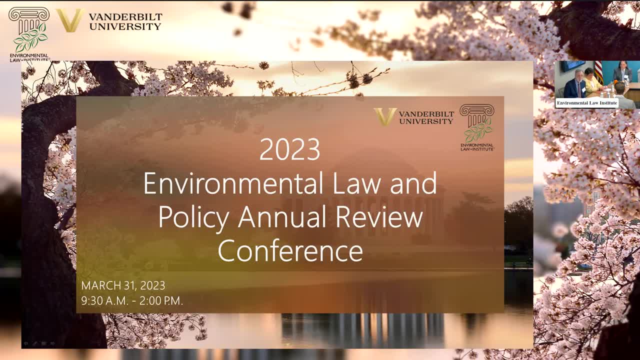 without giving up on below two degrees C scenarios as the motivation for mitigation policy. We're neutral in the article on whether the 1.5, 2.0 targets should remain the stated mitigation goals. That's a complex question but we're anything. 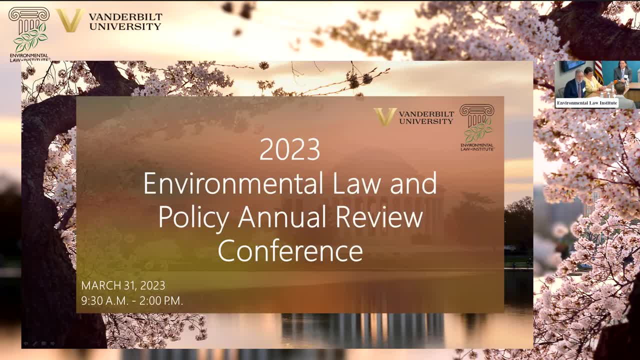 but neutral in the article on whether adaptation policy needs to move on and begin planning for extreme disruptions that swamp the resilience retreat strategies. In particular, we need to consider how we will adapt to how we adapt, in other words, through migration and other decisions. 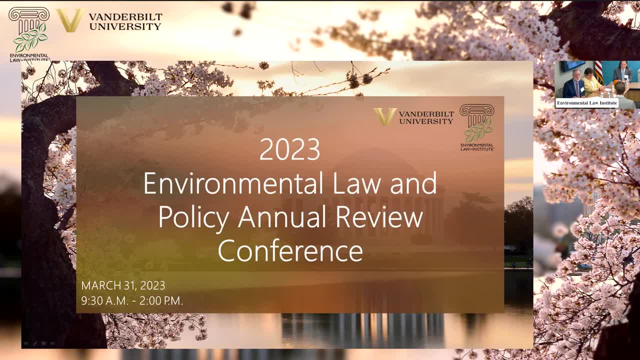 So we're not just adapting to climate change, We're adapting to human social adaptation to climate change. So with that, I'm going to turn it over to Rob, sehr gerne, to outline how we envision to have adaptation policy design And our proposal. thanks, Rob. 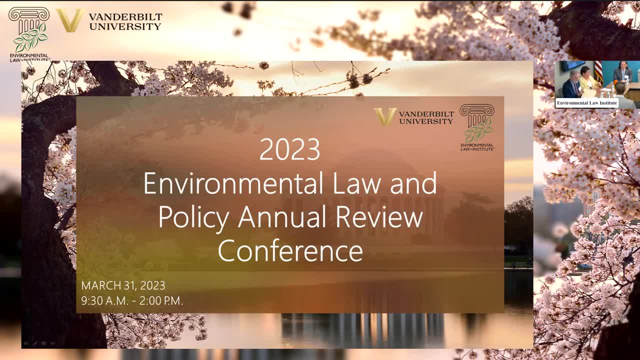 All right, well, thank you, JB. I wanna echo JB's thanks to ELPAR, to In Vancouver, to our commentators, And I wanna add one last thank you, which is to the Minnesota Law Review that agreed to go with a three character title. 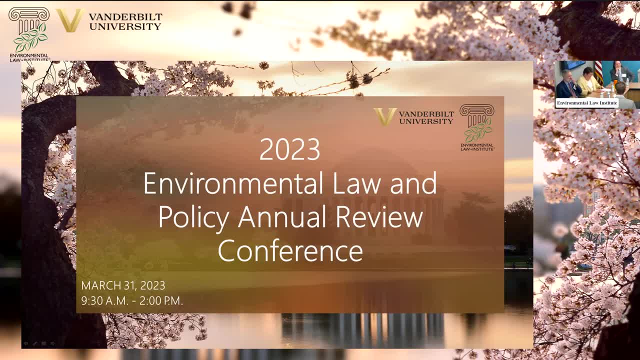 So that was something JB and I ensuite agreed to early on, and it was nice of them to do that. But so, picking up where JB left off, you know governance of and during extreme climate change will increasingly become more difficult And that 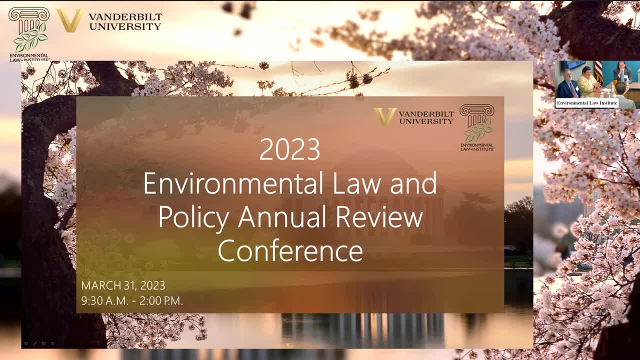 was one of the main points we wanted to make, And to try and take a first stab at imagining what that governance is going to have to be grappling with what it actually looks like on the ground to try to be successfully governing everything that's changing all at the same time. 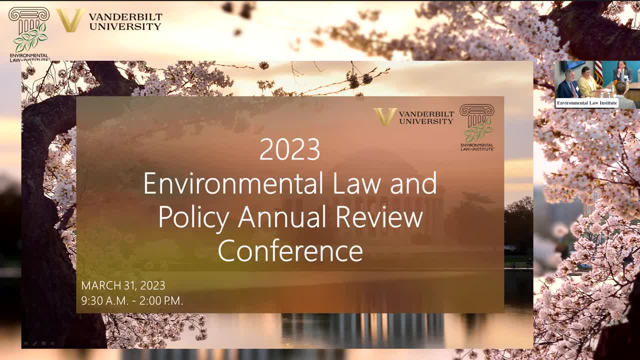 As JB mentioned in passing, we settled on migration as kind of a focal point, as a common thread that came up among everyone who's trying to envision this future, And it's kind of a universal thread in the sense that it's not just humans that will be moving around, but other species and ecosystems as well, And it's kind of a universal thread in the sense that it's not just humans that will be moving around, but other species and ecosystems as well. And it's kind of a universal thread in the sense that it's not just humans that will be moving around, but other species and ecosystems as well. 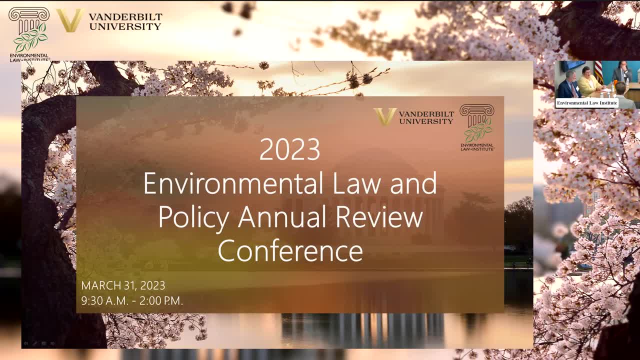 And so everything is in motion. all at once, However, as JB also mentioned in passing, we changed the focus from international migration, which is immigration, human rights, international law issue, to hey, we're going to have a lot of movement just within the United. 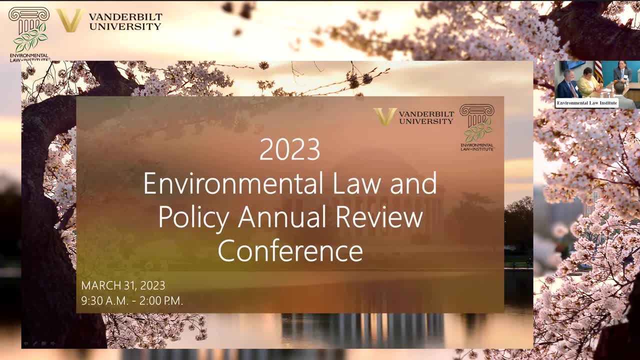 States. Let's keep this at the United States level and think about what that actually means. So governing this world requires moving beyond the three R's of resist, resilience and retreat into something we call redesign, adaptation, which means re-envisioning where people need to be, where they're probably going to try to be being. 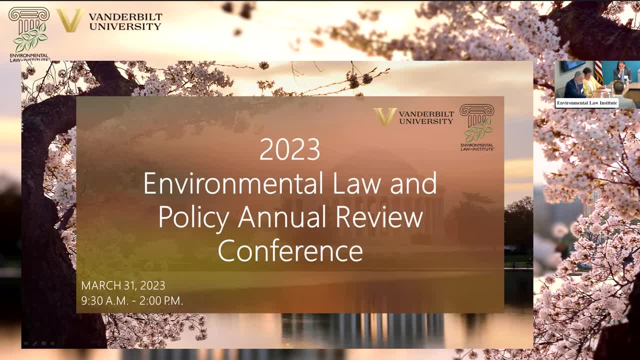 movement of population, changes in land use, changes in your natural resource base, changes in economic production, and the list goes on. So everything needs to shift. We need to be housing people in different places. We need to have the infrastructure in place to do that. Oh and, by the way, while we're doing all this, we should be 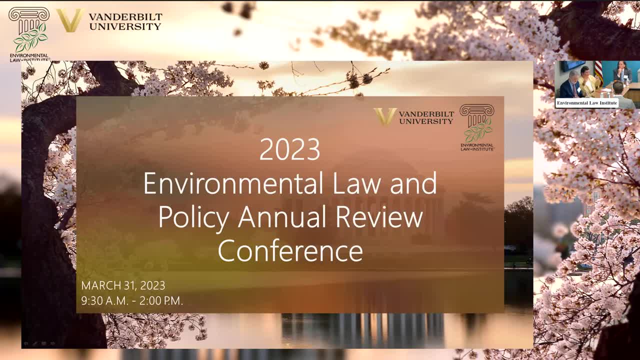 leaving some corridors open for the other species that are trying to adapt to the changes that are going on. So that was kind of our vision. And one thing we wanted to remind everyone of in this article is environmental law and policy have decades now of developing and developing. 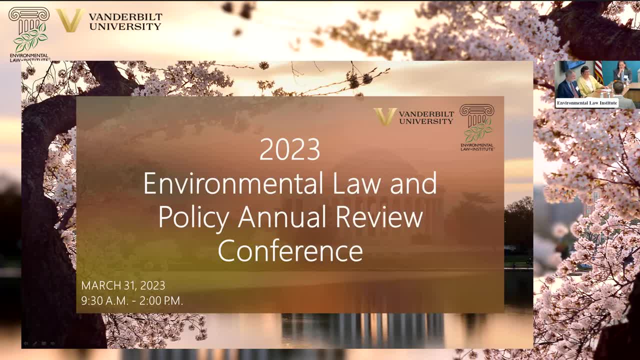 some pretty cool tools. It's not like we're going into this challenge without some ideas of tools we can put in place. So our scale ran from laissez-faire to federal preemption and mandates. Laissez-faire: we're thinking in terms of market signals and particularly we focused on insurance. 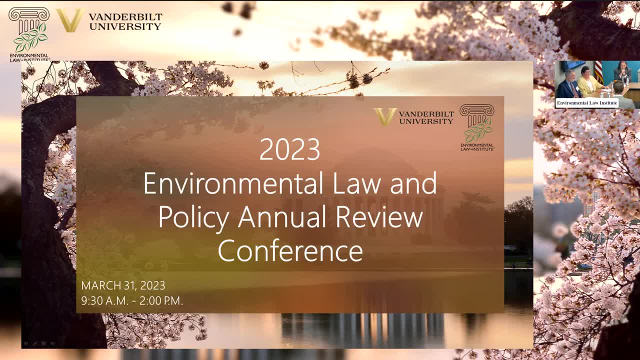 Insurance signals could already be driving more adaptation policy than they do, But our problem so far is that governments rush in where insurance companies fear to tread and keep insuring risky behaviors that are not money makers. So that could be a great starting signal for the adaptation process is when insurance companies say it's time to leave. 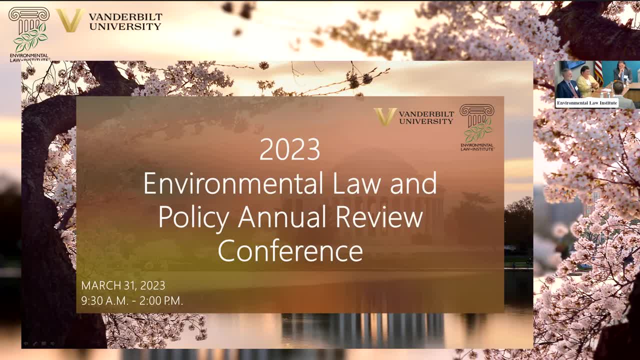 Probably everybody else should agree with that. We then got into planning tools in terms of needing to think about spatial rearrangement, Spatial rearrangements, infrastructure needs in different places, infrastructure decommissionings in certain places, and directed research by economists, by social scientists, by psychologists. 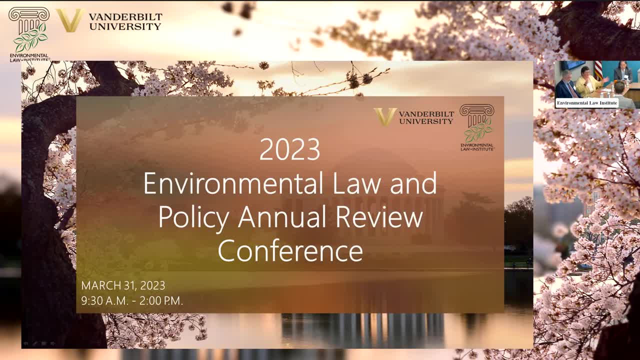 and, of course, by engineers and hard science, to figure out where the problems are that we need to solve. From there we get into prodding, which goes with reinforcing that insurance policy. We get into the insurance signal, Tweaking our disaster relief, which we don't think will stop- In fact I think it shouldn't stop- but it can be tweaked to promote adaptation goals rather than leaving everybody in situ. Review subsidies and remove the perverse incentives that we have all known for decades are in there. Add some tax incentives, perhaps. And perhaps the most controversial recommendation we came up with is: we may have to go back to land use. We may have to go back to land use. 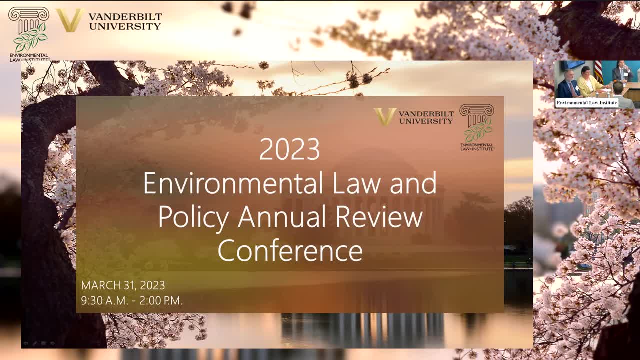 And perhaps the most controversial recommendation we came up with is we may have to go back to land use, Because where federal lands and national parks and things like that, all the places we treasure need to be- might be different than where they are now. So you know, one very effective history has proven mechanism for getting people to move where you want them to be is to give them free land. 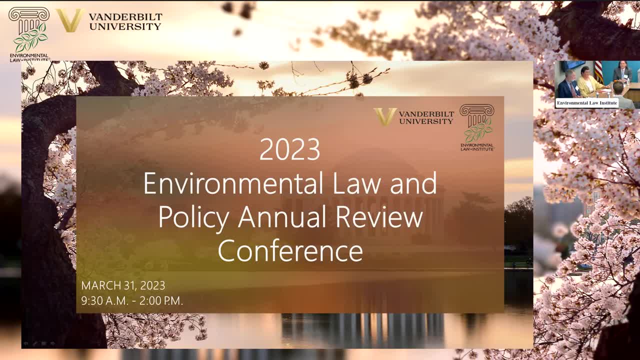 So and then, like I said at the end, our preemption and mandates. If you're talking about national scale rearrangement, by definition there's going to have to be a heavier federal hand in this local government, local government's plan for in situ adaptation, in part because that is where they have governance control. 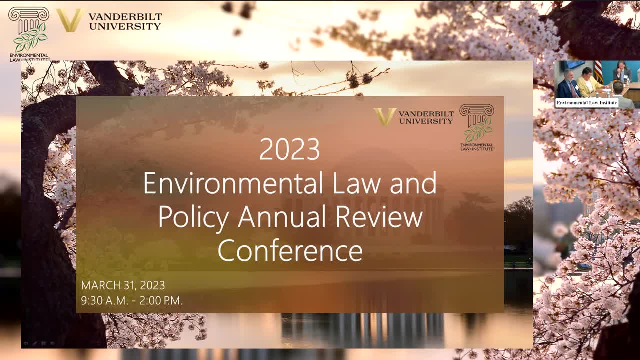 And so we need a heavier federal hand in all this. Our models in thinking about this tended to come back to the Dust Bowl, migrations and the ramp up after Pearl Harbor for World War II And the various public works programs going on in the Great Depression. 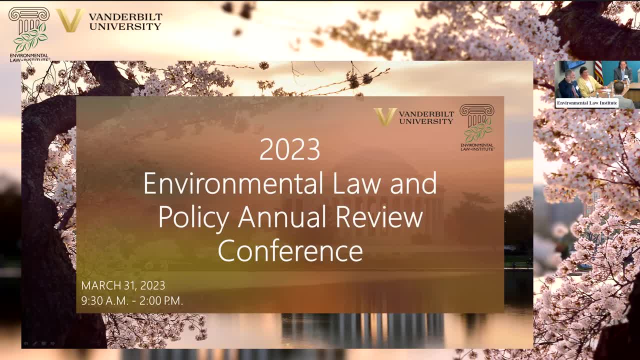 But another series of public works programs and social support mechanisms are going to be necessary as well. So our policy recommendation- I do realize we're coming up on the end of our 15 minutes- is that we need to engage in anticipatory governance. 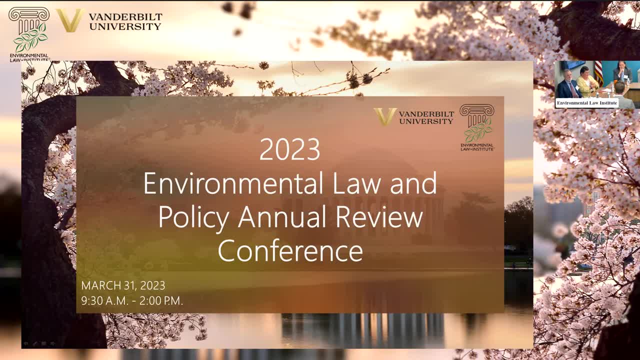 Thinking about what the governance needs are going to need, Are going to need, Are going to be 10 years, 15 years, 20 years, 50 years from now. Anticipatory governance is a growing field of governance research And we think that should be aided by a new, intensely interdisciplinary 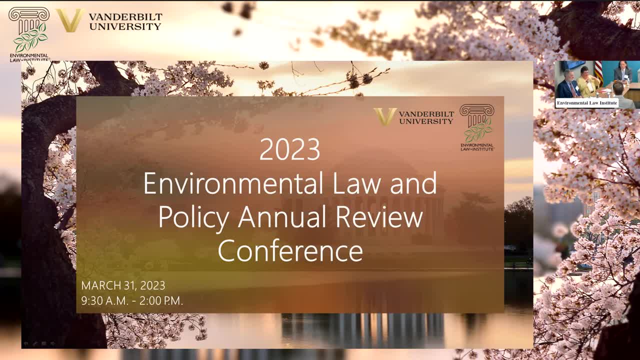 And when we say intensely interdisciplinary, if you can think of it, they should be involved in this group. Jamie and I had the great pleasure Being in an intensely interdisciplinary group working on adaptive governance issues in the context of water. It helped tremendously to have some psychologists in the room. 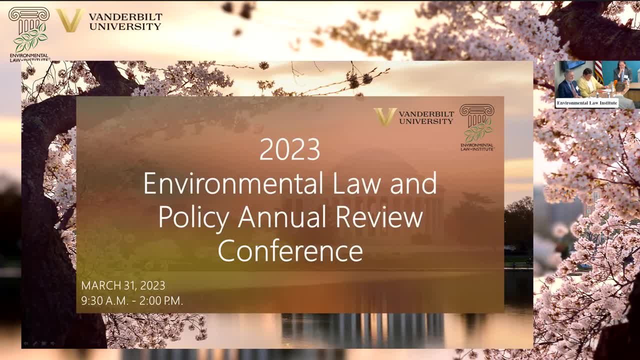 And some social scientists So intensively interdisciplinary nonpolicy making body. We thought that was important. You don't want the people doing the evaluations to be the ones that are subject to the policy. We thought that was important. You don't want the people doing the evaluations to be the ones that are subject to the policy. 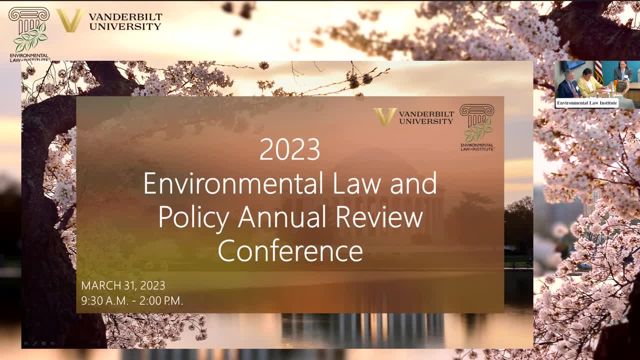 So we're looking at a number of different ways to do that. So we're looking at a number of different ways to do that In many different ways to understand the politics of making the final policy, of all Who are basically sitting around dreaming up all of the different ways the future play out. 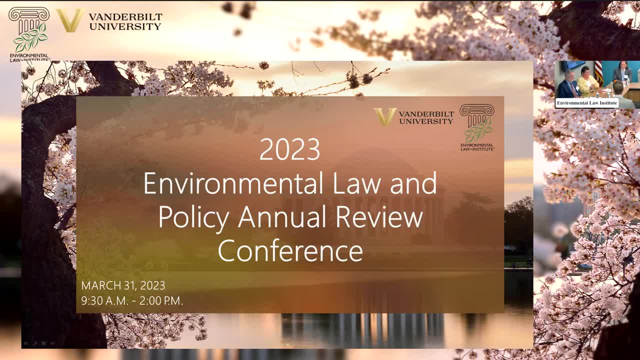 Both in terms of how climate change impacts the United States, But also how human beings are something to that. Are we going to have panics? Are we going to have orderly moving around? Are we going to have armed insurrections in some parts of the country? 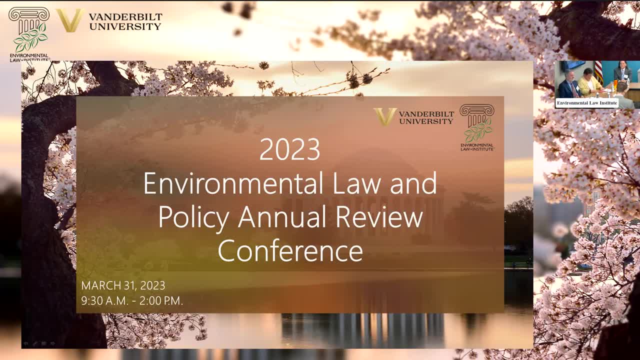 All of that needs to be governed. Like I said, part of the consideration, so that we can come up with various scenarios of how our future might unfold and what governance responses are going to be needed. and are we going to- which is almost certainly going to be true- are we going to need different kinds of governance? 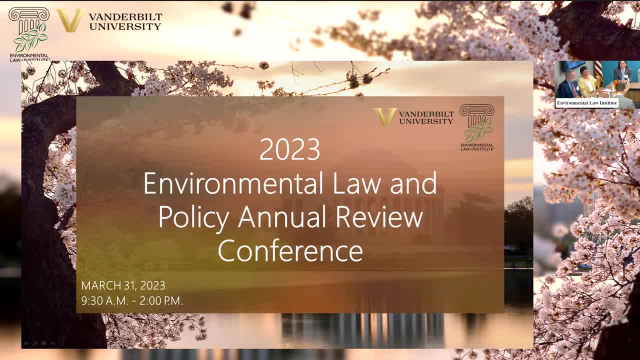 responses in different parts of the United States to achieve different adaptation goals. So that's a summary of where we ended up and that was our recommendation, And you can see why the article was picked because it's thoughtful. no, I mean really thoughtful. really thoughtful analysis and recommendation. 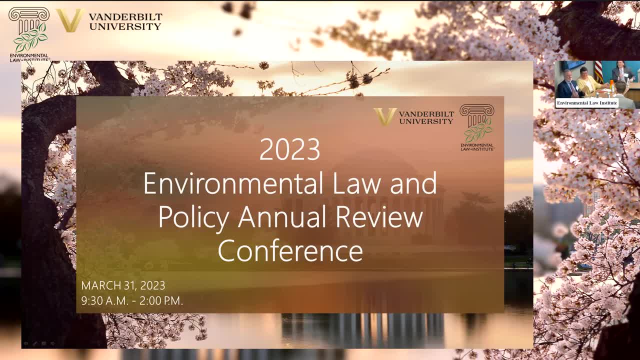 Can I add just one thing, Just to emphasize: about six months after our article came out, a team of client scientists published an article in PNAS, one of the most influential journals, essentially saying the same thing, from their point of view: That we need to actually start designing scenarios of beyond two degrees C, because we're likely 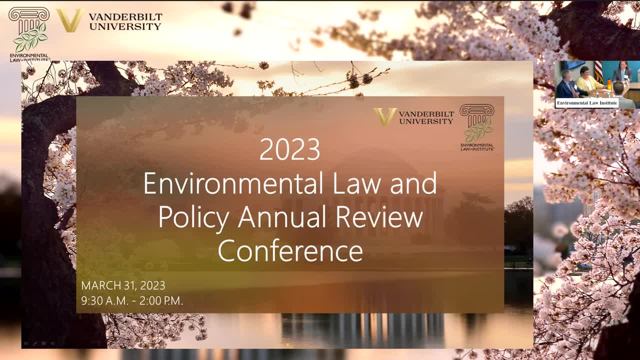 headed there And we had a little exchange of letters. Their idea for how to do it was a little different to ours, but you know pretty much the same. you know a lot of common ground, So it's just interesting to see this also coming from the climate science side as well as. 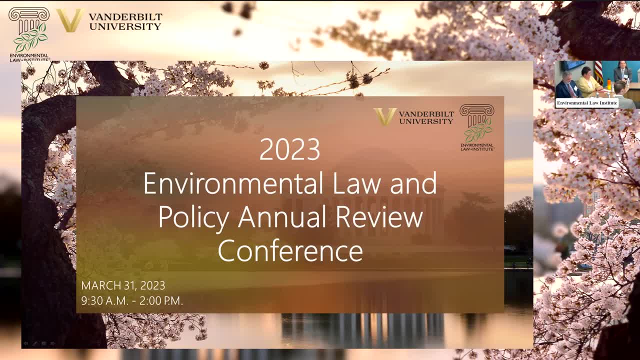 the policies. Wonderful, thank you. So we're going to turn now to Carlos Evans in the city of Dallas, to give a little bit of a talk, A little perspective on this. We're going to get a lot of perspectives on this. Yes, good morning. 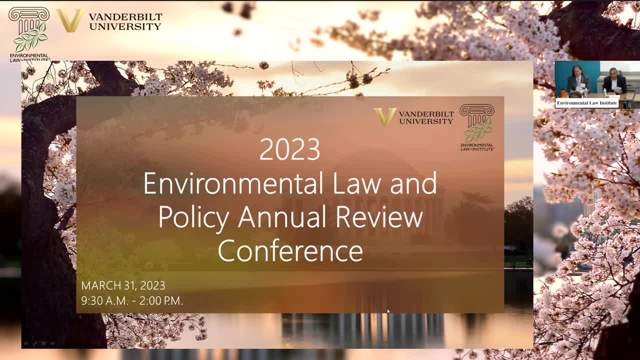 So Carlos Evans, city of Dallas Department of Office of Environmental Quality and Sustainability, And this is a very complicated and intriguing topic. As you know, city of Dallas is an inland city, So this topic is going to be different for inland cities versus coastal cities, right, 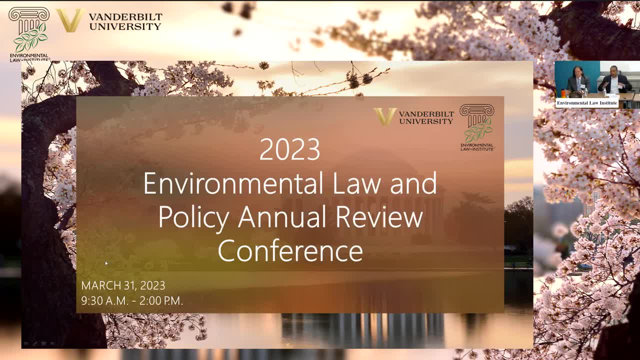 So for the city of Dallas, we are focused on realizing a sustainable, resilient and equitable city of Dallas, right, And if redesign adaptation means for us to get more federal funding as we accept more domestic migrants, then that may be a good thing. 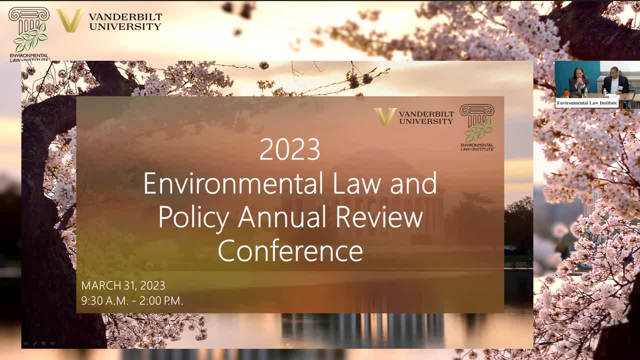 If redesign, adaptation means that we're asking the city of Dallas residents who love their city to go to Oklahoma- and most are not necessarily fond of Oklahoma- then that's going to be a completely different issue, right So? but anticipatory governance. 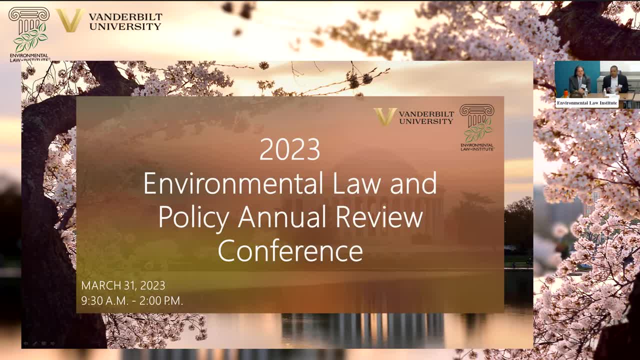 You know if there's a federal agency planning this out and providing policy recommendations to council members, and you know so. for example, my role is I provide recommendations to our council members. We have 15, 14 council members and a mayor. 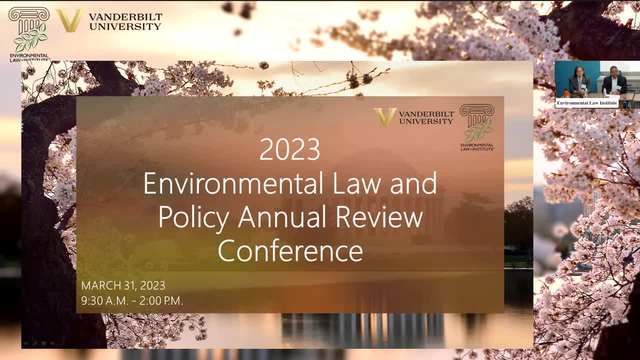 If I'm up there telling them: look, this federal agency is saying- and I don't know what that was, but it's saying and it's saying in 15 to 20, 20 years, you know we're going to have to move to Oklahoma, you know that provides some data and scientific cover for me to say that. 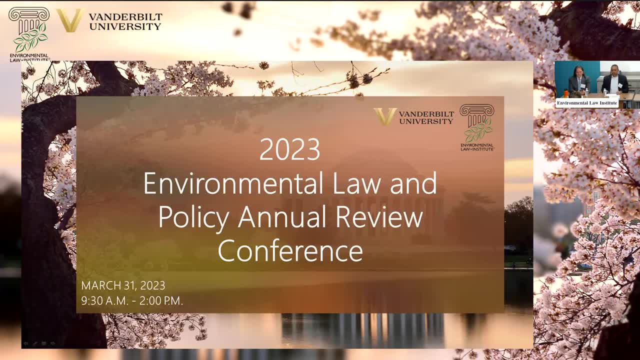 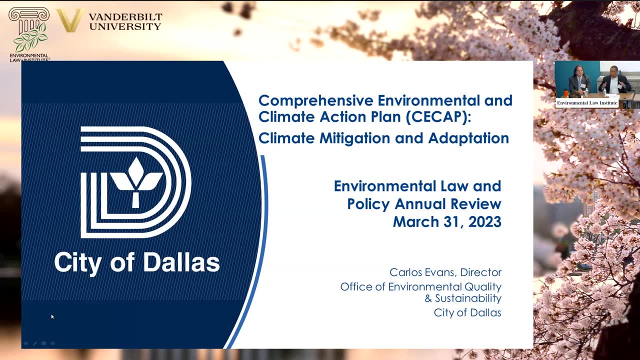 But I don't know if that's going to go over well, So but let me run through some slides just to show you where we are right now. Again, we're focused on sustainability, resiliency and equity. Go to the next slide. 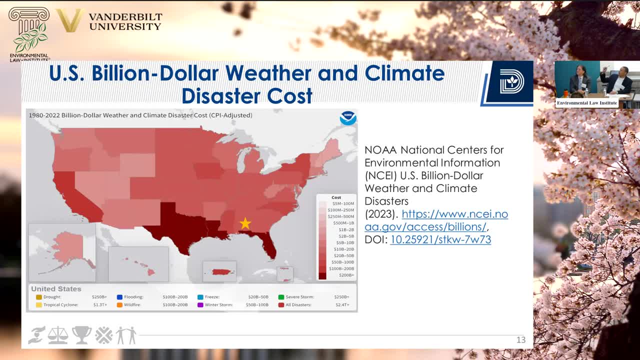 Next slide. So just to remind, and I don't know how the star got on a different state, but the star got on Texas, But anyway. so just to remind everybody, Texas is number one in the wrong way. So we're number one in a billion dollar weather and climate disasters and number one in cumulative cost of climate disasters. 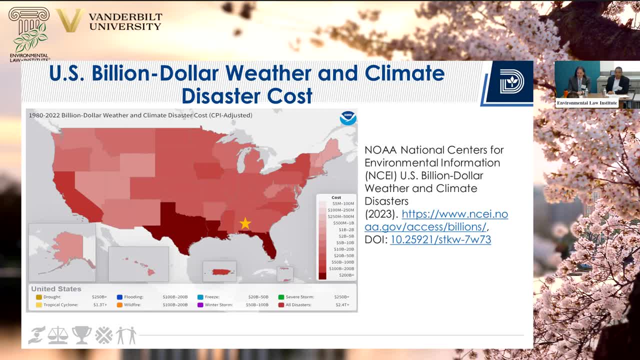 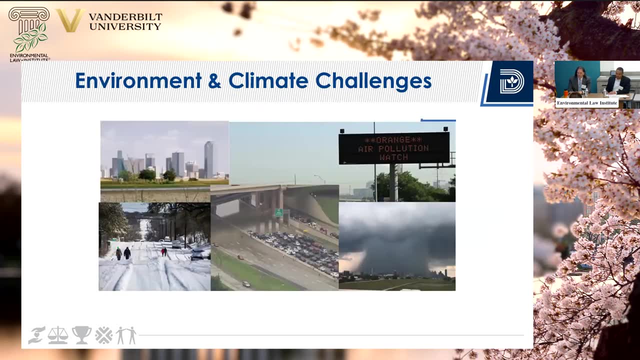 Since 1980 were approximately around $380 billion in costs from climate and weather related disasters. Next slide: As you know, Texas suffers from extreme heating during the summer seasons, extreme freezes during the winter seasons. You may recall 2021 extreme weather. 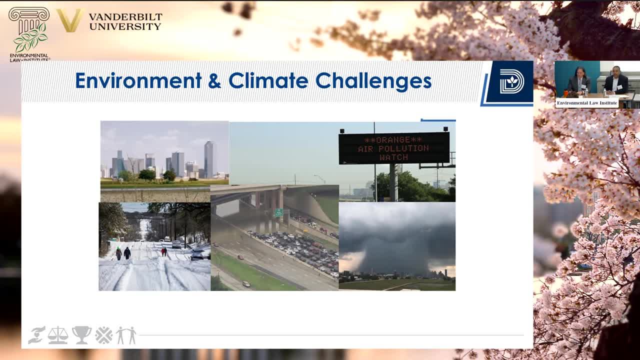 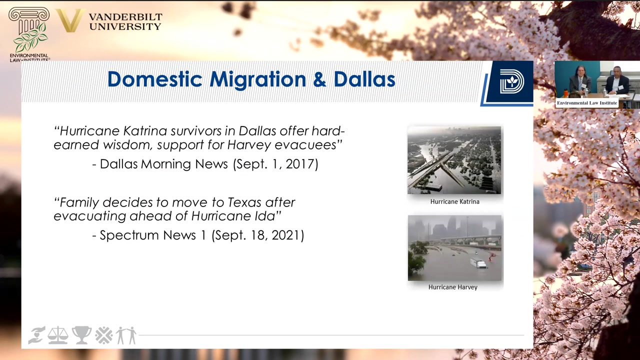 a winter storm, Yuri, where this whole state lost power. Hundreds were frozen to death in their homes, without power, electricity and heat. These are some serious and real issues for us, And the floods are more severe as the year progresses. As I alluded to before, the city of Dallas is a destination. 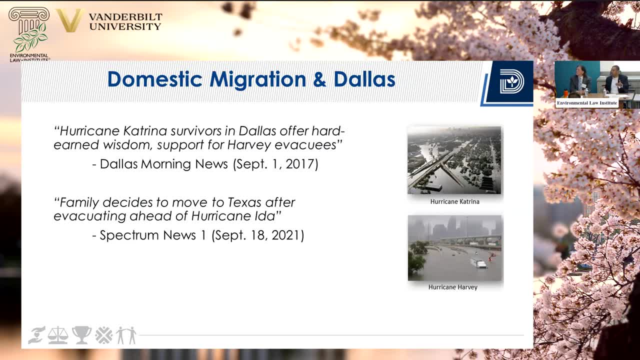 city for a lot of inland residents. Because of Hurricane Katrina, Rita, Harvey, a lot of folks are coming from the Gulf Coast to the city of Dallas, One of the reasons why the city of Dallas is growing, as well as headquarters to a lot of corporate organizations. Next slide. 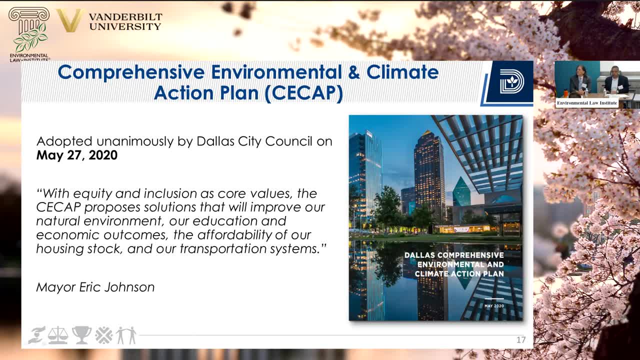 So the city of Dallas approved unanimously in 2020 a comprehensive environmental climate action plan. Again, we're focused on climate mitigation, climate adaptation, improving environmental quality and environmental justice. Next slide: Eight goals. We like to say it's everything from A to Z, from air quality to zero waste. 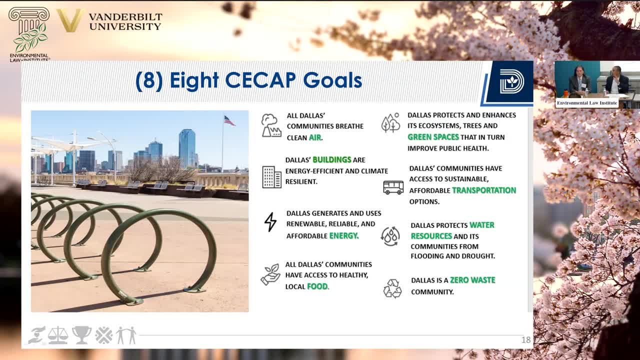 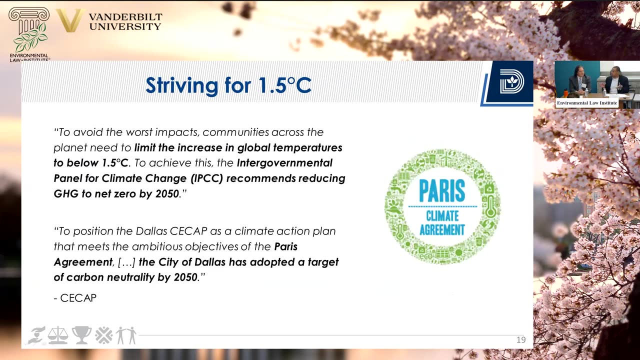 Talking about buildings, energy, transportation, water quality, air quality, access to local food, access to healthy and local food, and the like. Next slide: Sorry, I'm trying to give a few minutes. We're still striving to avoid 1.5.. One of our arguments- I wasn't there. 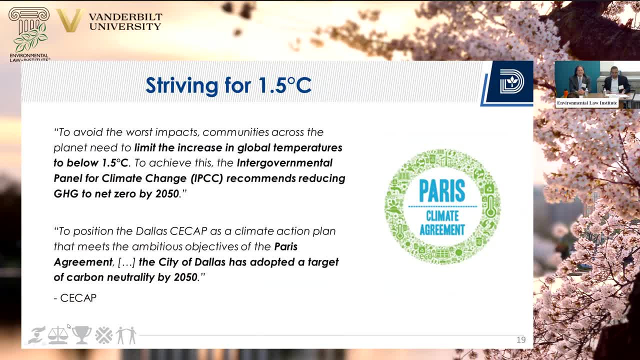 at the city I was at, EPA Keep C-CAP was passed, But one of the arguments for this was: look, the science says we need to avoid 1.5.. That was the scientific backing for our climate action plan. We have you know now that. 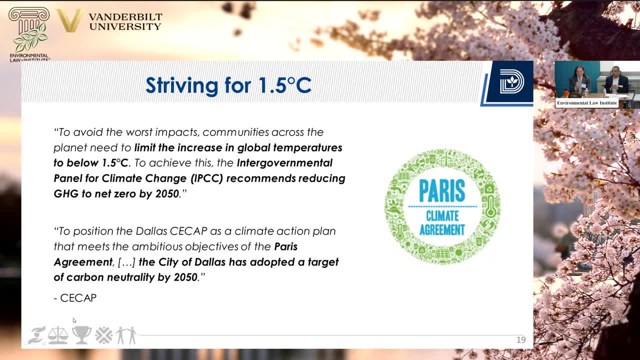 the IPCC report. latest IPCC report came out. we have not briefed council on that, But I think, regardless of whether we're talking about 1.5, 2.6, 4.0, the council members are going to say: 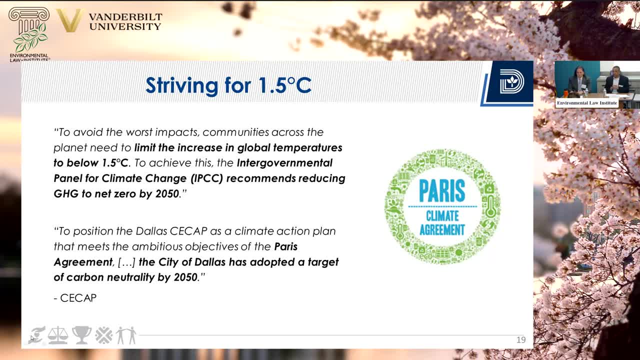 look, I need to advocate for my residents who want to stay in the city of Dallas, whether that means, you know, focusing more on adaptation or focusing more aggressively on both mitigation and adaptation, I think they just want to stay. they want to make sure that we stay in our city. 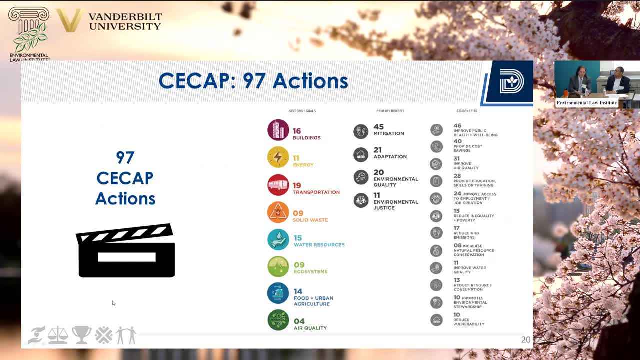 Next slide. So we have 97 actions Again. so you see a focus here. We have 45 mitigation actions, 21 adaptation actions, 20 environmental quality actions and 11 environmental justice. I think you see the essence here being. 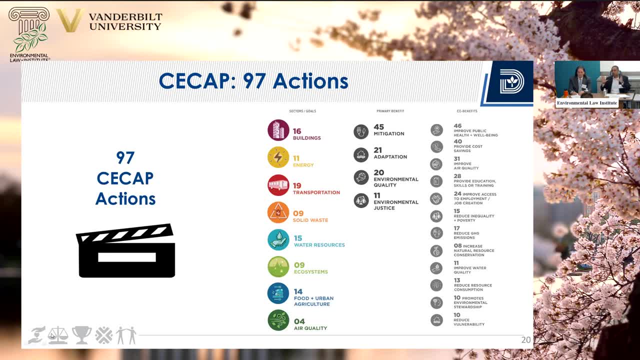 1.5.. We're trying to get to net zero greenhouse gas. Our general goal is trying to get to net zero greenhouse gas emissions by 2050, consistent with the Paris Climate Agreement. You know, again trying to be more aggressive in mitigation so we can meet our climate goal. Next slide: 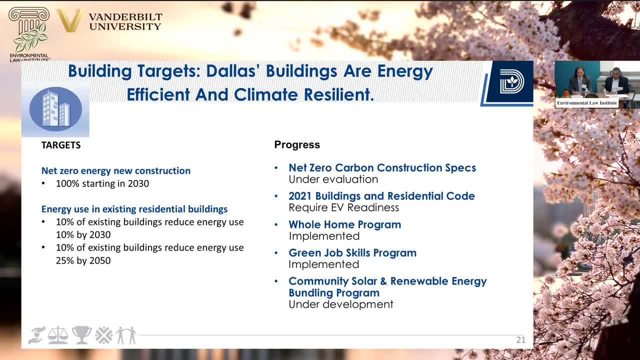 So, just running through some of kind of where we are status right now, we're trying to work on net zero carbon construction specs. That's still under evaluation. We're trying to work on net zero carbon construction specs- That's still under evaluation. We're about to adopt some of the 2021 international construction codes. 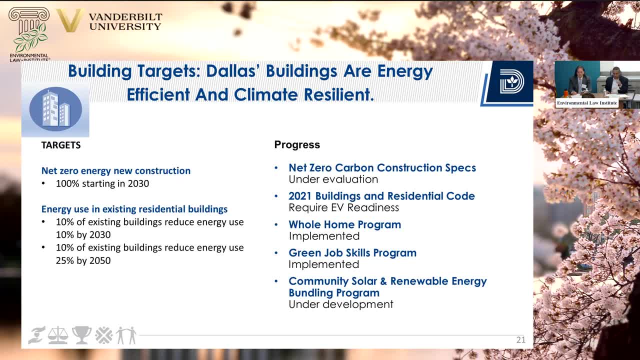 including some requirements for EV readiness and solar, which is not on the slide. We have a whole home program which provides our residents with information on weatherization, energy efficiency and renewable energy programs and projects available to them. as residents within the city of Dallas. We just launched our green job skills program, So this is if you're a contractor within. 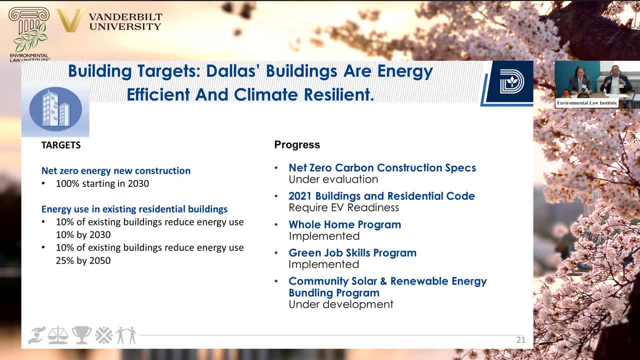 the city of Dallas. you're going to be able to get a job in the city of Dallas. So we're going to just launch our green job skills program. So this is: if you're a contractor within the city of Dallas and you want to get your weatherization certification, we will pay for some of your. 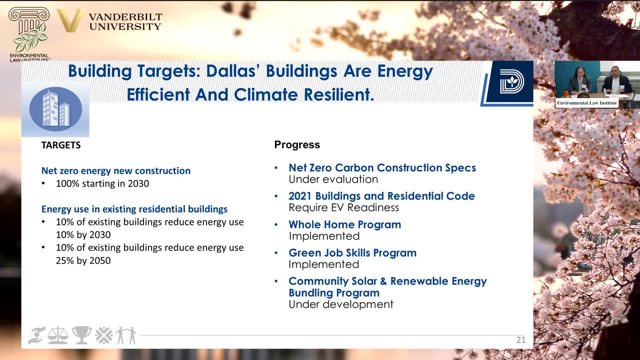 we will pay- Well, we'll pay- for 50 people, some of their, some of the courses so they can get their weatherization certification. And we're still working on our community solar. Well, we're trying to develop a community solar project And we're looking at bundling programs for renewable 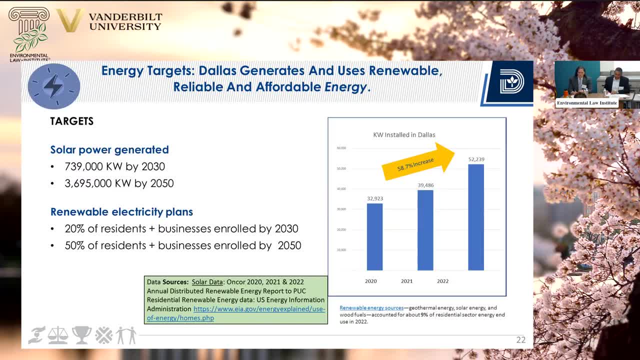 energy Next slide. So we're we're we're trying to work on net zero carbon construction specs. We have approximately 52,000 kilowatts of installed solar. That's a 58.7% increase since 2020.. 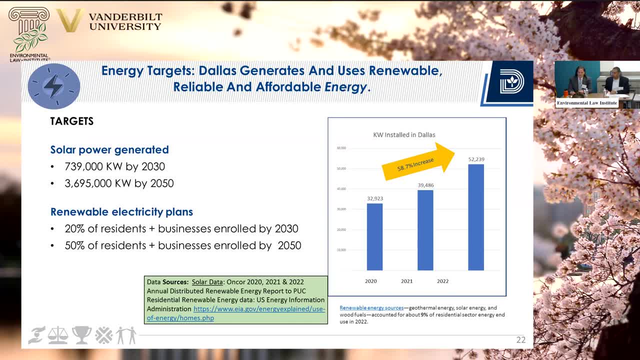 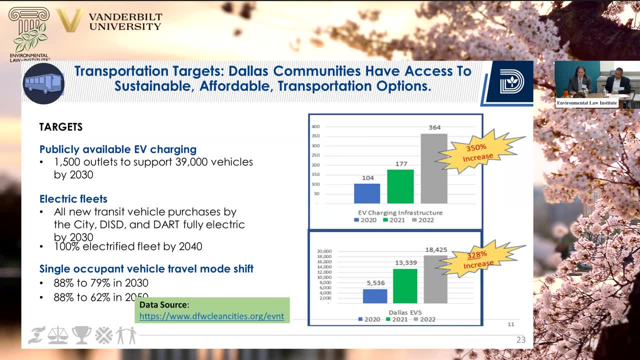 We're not Austin, We're not other cities on the West Coast and East Coast, but we're making progress Again. this is our third year implementation of our climate action plan, but we're getting there. Next slide Again. we're not Austin or San Francisco or anything like that. 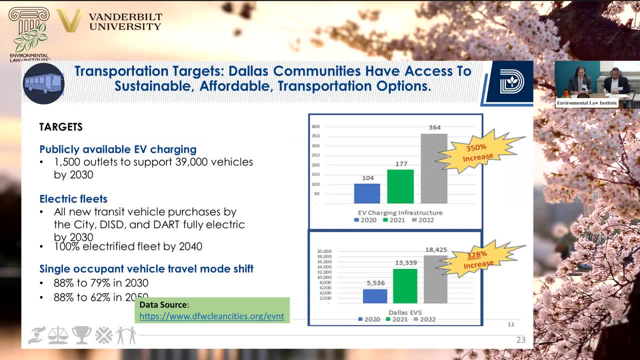 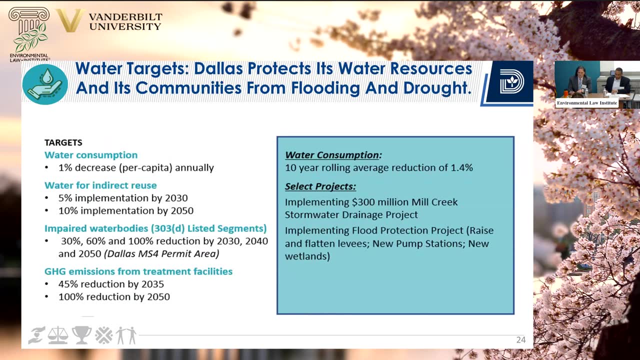 but we have approximately 360 EV chargers and approximately 18,500 folks driving around in EVs thanks to Teslas and other products. Next slide, When we talk about infrastructure and resiliency. a lot of money is being poured into our water infrastructure, stormwater infrastructure. 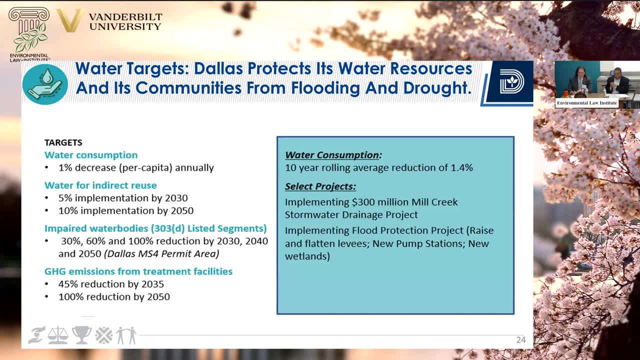 We are implementing a $300 million Mill Creek stormwater drainage project On the east side of Dallas. a lot of flooding concerns So essentially the Dallas Water Utilities has burrowed or created a storm, huge storm drain from East Dallas to West Dallas to get that water into the Trinity River. 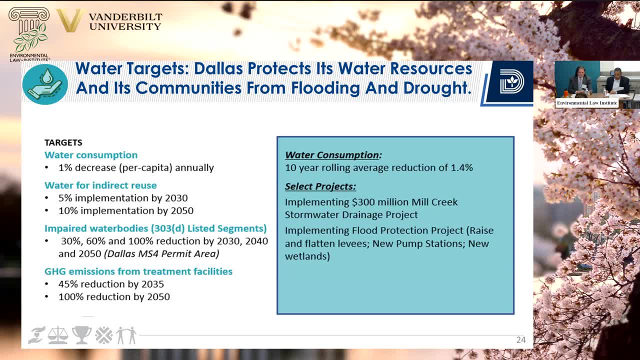 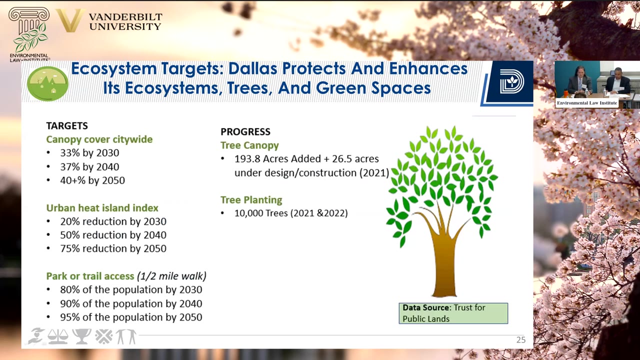 So that project is underway and almost completed. We're also implementing a $230 million flood protection project that raises and flattens levees. We'll be operating new pumps, pump stations and creating new wetlands Next slide. We've planted approximately 10,000 trees in the last couple of years. plan on doing more, but we're getting there. 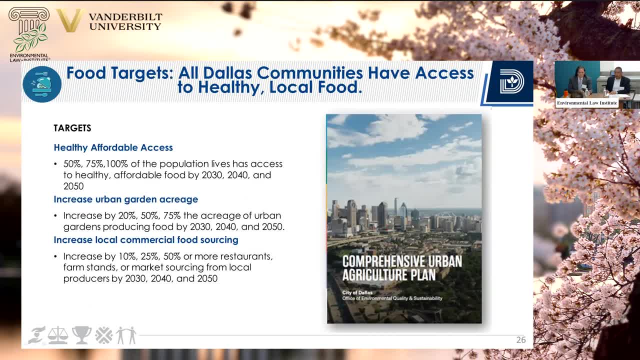 Next slide And we just launched a comprehensive urban ag. the city council just approved a comprehensive urban ag plan. We have about 15 acres of urban ag acreage in the city, trying to expand that so that we can significantly, significantly, significantly improve the water quality of the city. 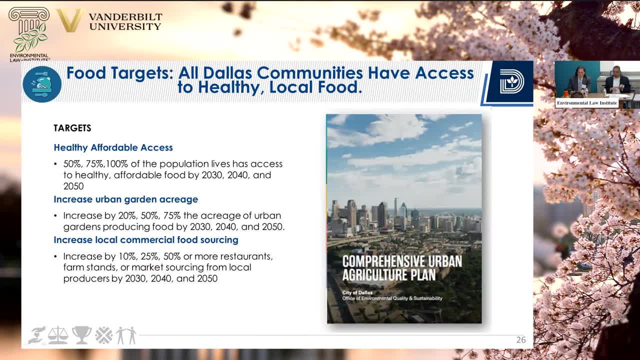 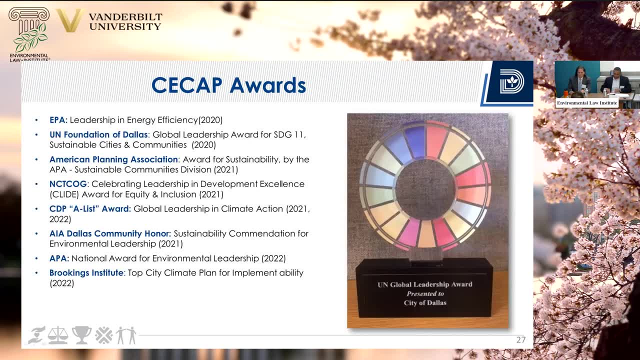 Next slide And we think that will impact our food supply. once we do, that will focus more on food consolidation, distribution and market opportunities. Next slide. So we're again three, three years in. we have some awards. got to say Hey. 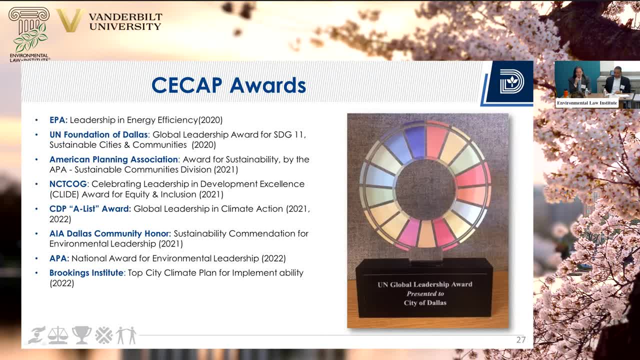 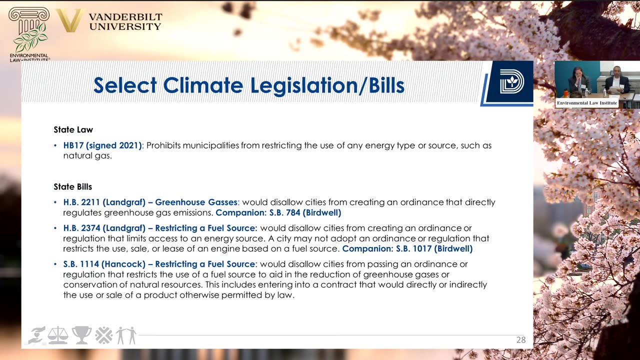 What the latest award is saying. we have a totl climate plan for implementability, And so that's awesome, That's a lot So, but again, Yeah, So we're in Texas. So what does that mean? that we have some real political realities from the state legislature. HB 17, signed in 2021, says that we cannot favor any energy types. 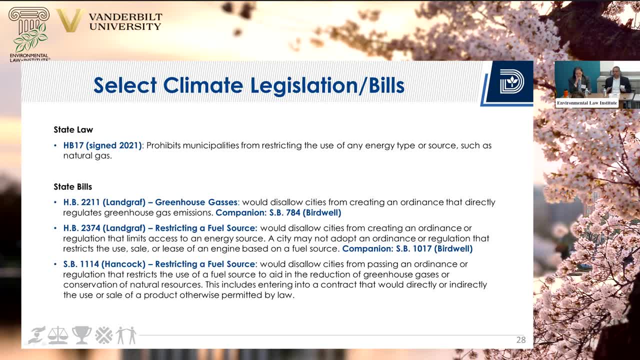 Right, so that's huge. that's not so. California and other states. you know they say, you know they're focused more on electricity, etc. renewable energy. as a city, we can't, we can't favor any one type over another And there are many bills currently going through state committees trying to make sure that we do not regulate greenhouse gas emissions or favor a fuel source. 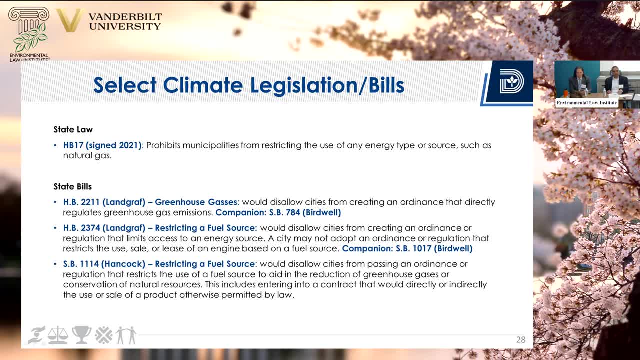 So this one of this, one of the one of the reasons why this came about- is in December, and some of our council members on our environment sustainability Council Committee prioritize transitioning gas powered landscape equipment to banner battery and electric powered landscape equipment. They want us to work. 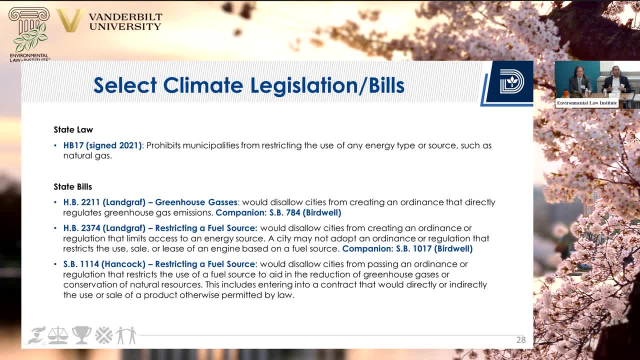 We're tasked for bringing a plan before them in June to transition out the entire city by 2027 is talking about city operations, talking about businesses- major, medium, small businesses. we're talking about residents. if you live in the city of Dallas, you're supposed to be getting battery powered battery powered equipment. they want to put together a plan for the entire package by 2027. so you know, in theory that would require a. 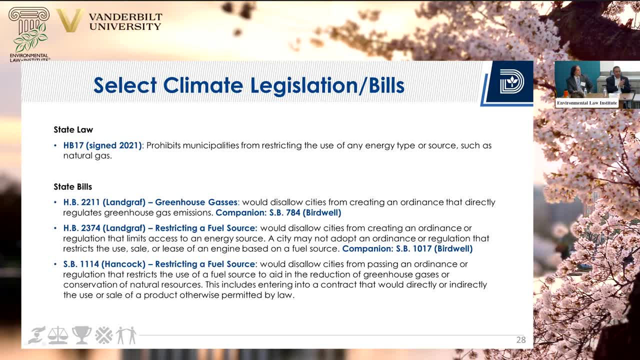 Institutional, Institutional, Institutional, Institutional. And so that's one of the reasons why, and also the other reason why many people are concerned about this is because of the various issues that that that's the issue strategy I mentioned earlier. obviously, Your city has very decentralized programs. your buybacks and your, you know things of that nature and your ordinances. 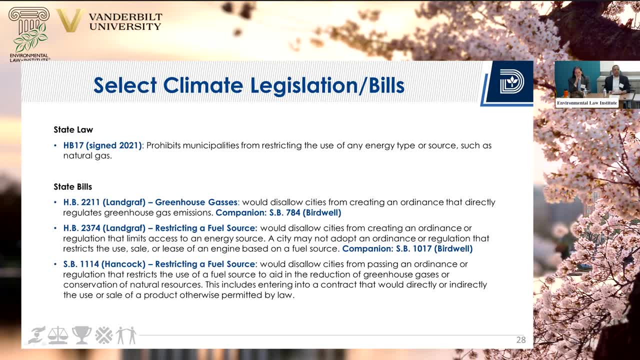 Well, private sector has a lobbyists, and so what do they do? So now we have a number of bills in Austin saying that, well, we don't necessarily support this. So that's one of the reasons why you see some of the bills and the Austin or state let tis the state legislature. 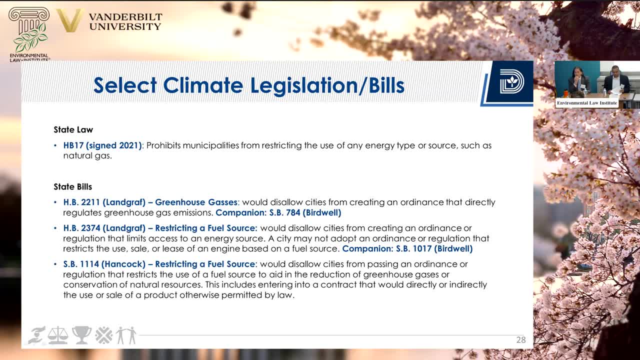 emissions and kind of being neutral on the municipal level. So, all told, just going back to I'm not sure how much time I have. Did I run over? But you're good, Take a couple more minutes, All right, Especially about those awards. 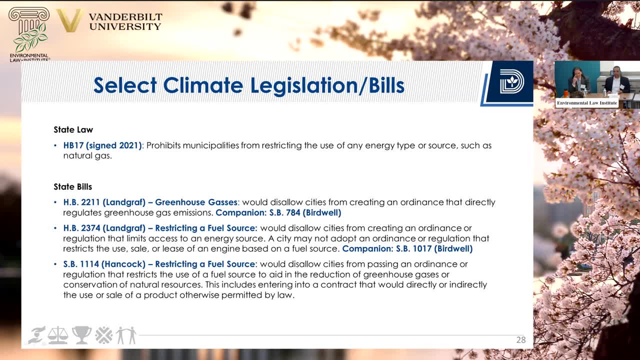 So again, so I mean it's a very complicated, I mean it's a very, very fascinating topic and I love enjoy reading it and just thinking about it. To me it comes to feasibility on the local level, because obviously they say politics, all politics, is local When you work for city. 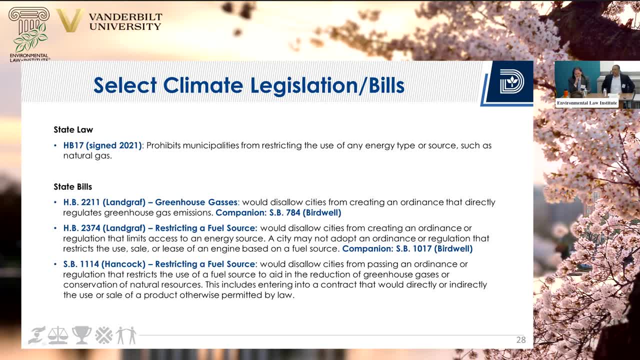 council it's really local And they are, and we have districts right, And so each council member is representing a district and they're focused on their districts, So they don't want to have to go to their residents, who have perhaps have been there for generations, and say, hey, 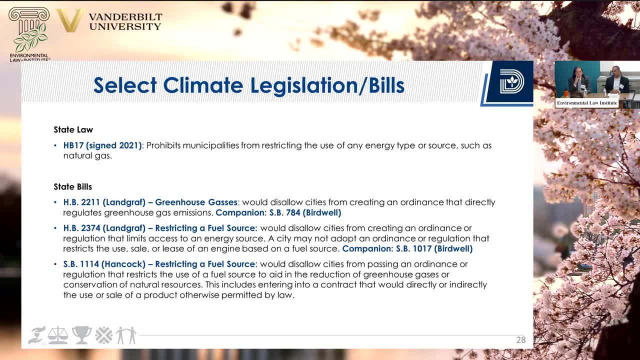 we love, you know, we know you love your TCU, Texas Longhorns, Texas A&M, but you know, go be a Sooner, you know. So that's, it's an interesting, interesting topic for discussion, But again, if that means that we're a destination city, now again, if I'm Houston, 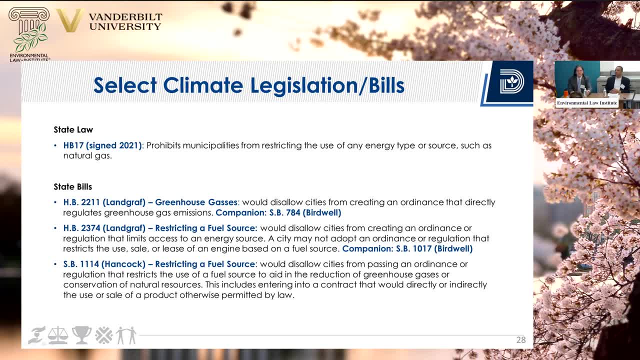 if I'm the director of the Environmental Department of Houston. that's a completely different story than you know. that's much more drastic and dramatic and you've been identified already. So if you're New Orleans, you know you may be. you know, you know this may be coming. 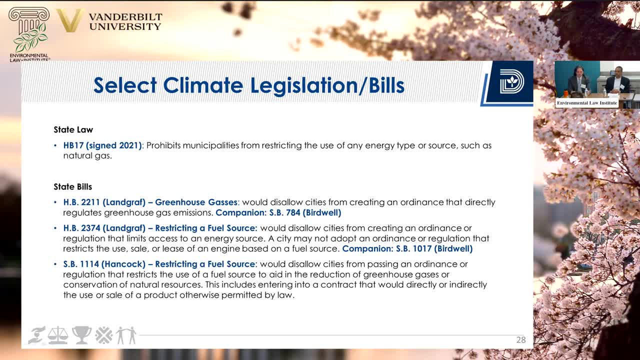 because you're losing land, land mass already. But you know this, this concern about migration has not been identified, I think, for the city of Dallas. We're used to being a destination city for domestic migrants, So so, just, I guess it depends on where that line is, you know. 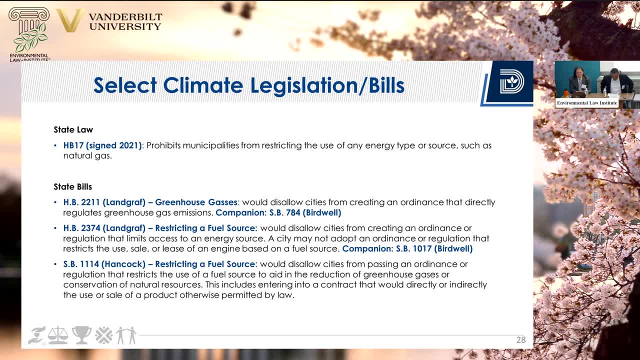 where folks will be living. Yeah Well, thank you, It's so. it's really interesting just to hear how this plays out on the ground. right, And I think what you said is so important about you're not San Francisco, because I work on the grounds in Nashville quite a bit and it does not matter what San Francisco's. 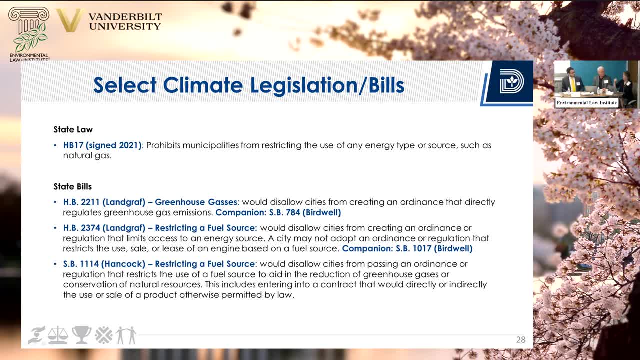 doing, People do not care and they just go. yeah, but when Dallas is doing it, it makes a difference, And that's part of why I invited you, because we look to Dallas, you know quite a bit And I think it's just. 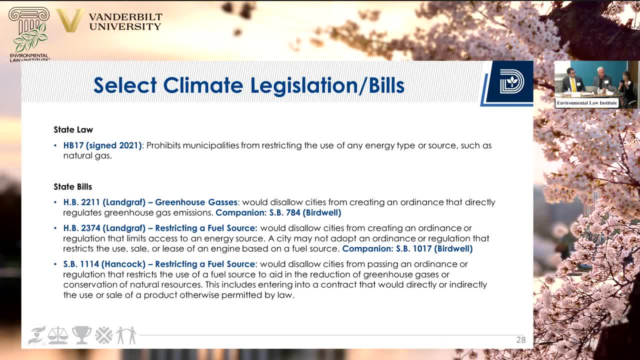 really important to remember about this dynamic of you know, blue cities and red states, and what you're trying to navigate in terms of getting things done, whether it's mitigation, you know, or or adaptation. So thank you, And we are going to move next to Joel Strider from EPA. 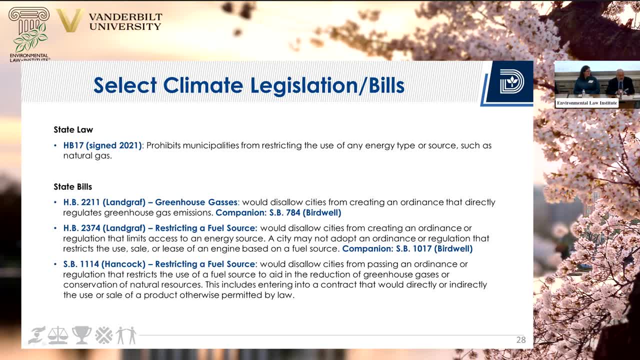 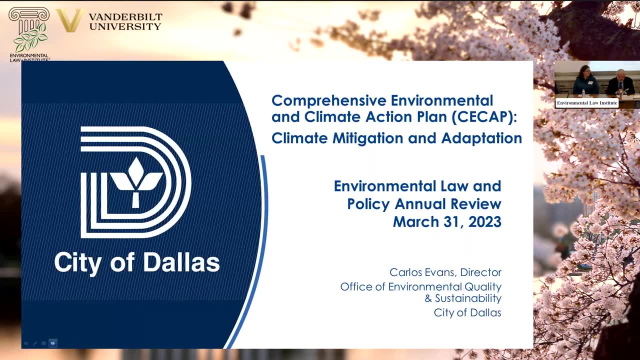 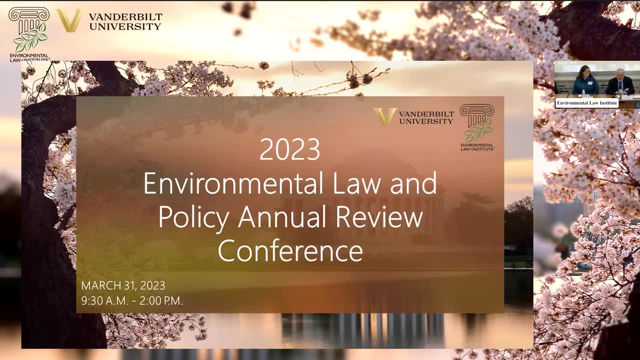 Well, thank you very much. Good morning everybody. It really is a privilege for me to be here, And Linda and Michael thank you very much for this opportunity. I think the introduction and the introductory remarks suggested that we're starting this conference with doom and gloom. I'm going to try to bring a note of optimism and opportunity to the 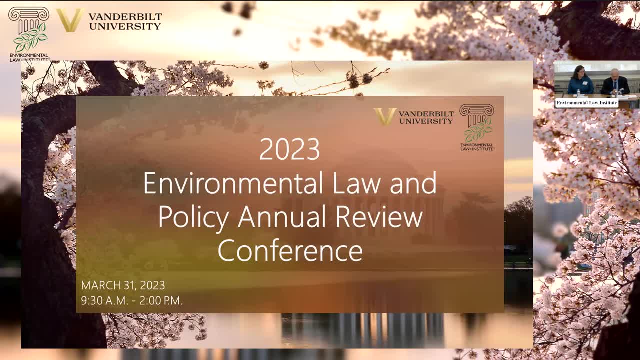 discussion. JB and Robin have written a very, very thought provoking article and a very important article, And thank you for writing this, this paper. As they acknowledge in their article, the Earth's climate is changing at an increasingly rapid rate, now outside the range to which human 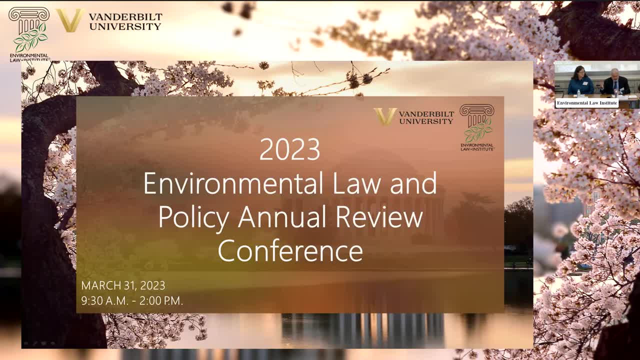 beings have had to adapt to in the past And realistically, as JB's suggested, achieving the goal set in the 2015 Paris Agreement of limiting global warming to 1.5 degrees centigrade, which the Intergovernmental Panel on Climate Change estimates will actually occur sometime around the first half. 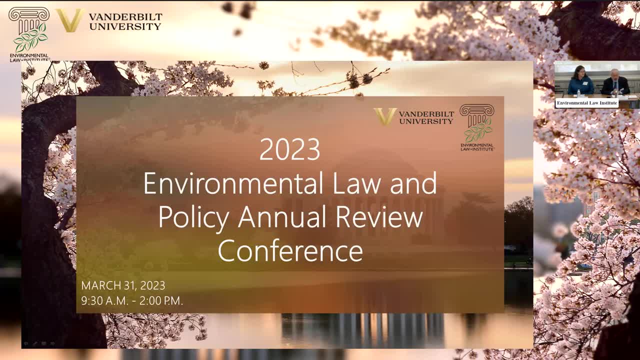 of the 2030s, which isn't that far away folks, will be unattainable without drastic actions to reduce greenhouse gas emissions And in the absence of any additional efforts to reduce emissions even more existing and currently planned fossil fuel. 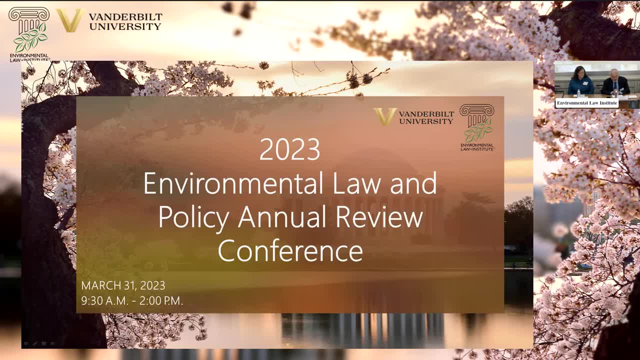 infrastructure will produce enough greenhouse gases to warm the planet roughly two degrees centigrade this century, And I have to applaud the importance that JB and Robin place on having concurrent governance efforts to both mitigate emissions of greenhouse gases to slow the rate of climate change and slow the rate of warming. 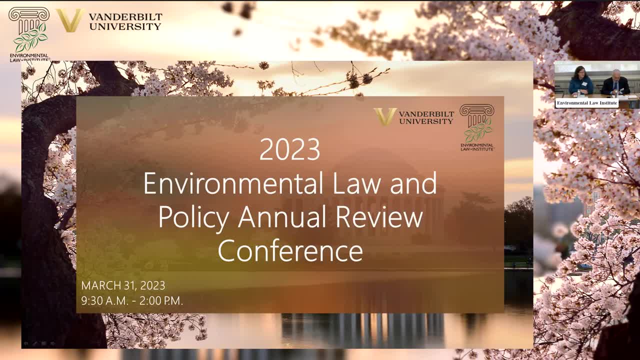 and anticipate adaptation to prepare for inevitable impacts. But, as you've heard, JB and Robin go a step further. as JB said, and I'm going to quote you, they argue that, barring rapid global political, social and technological transformations, we will be fortunate if we're able to limit temperature rise to two degrees centigrade. 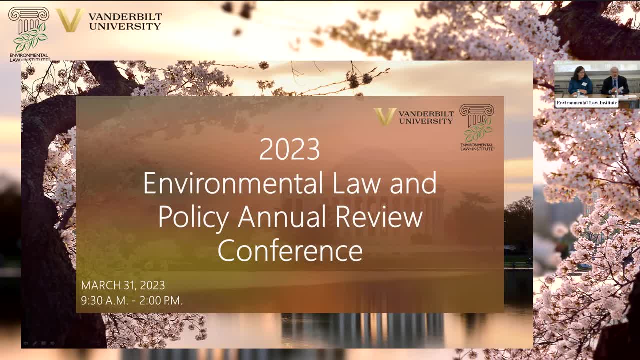 and the possibility of reaching four degrees centigrade can't be ignored. Clearly, reaching a four degree centigrade the world would have potentially catastrophic impacts, catastrophic consequences. However, to put it in perspective, as noted by the IPCC's newly released AR6 synthesis report, 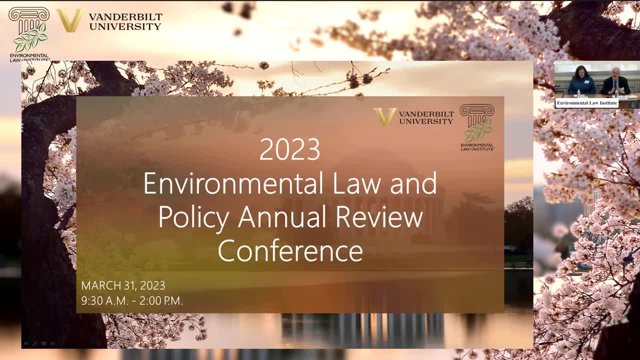 many of the most dire climate scenarios once feared by climate scientists, such as a four degree centigrade or more world, now look a little more unlikely. A lot of nations like the United States are investing more heavily In clean energy. you just heard about Dallas and wow, I'm impressed. 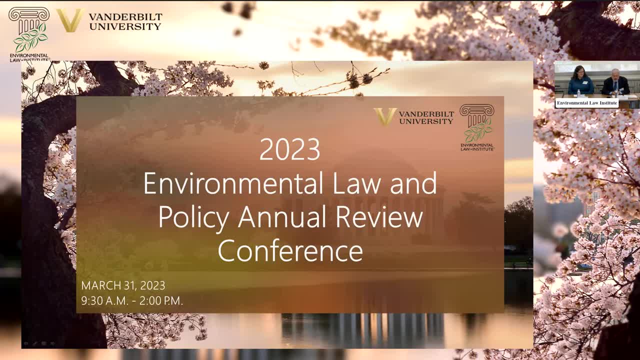 But nations are investing more heavily in clean energy, which has become much more cost, competitive, and at least 18 countries, including the United States, have managed to reduce their emissions for more than a decade now. However, whether or not one believes a four degree centigrade world, 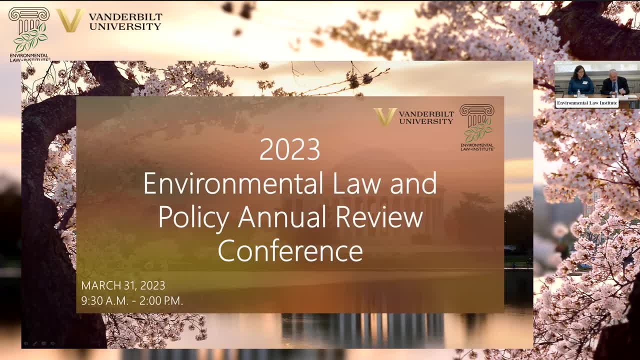 is likely, investments in low-energy energy will not be entirely necessary until a one degree centigrade global warming will begin. And so here's some of this non-reliable data that I hold and deal with. The first step is to look at what the global climate problem is and to look at the role of the global climate. 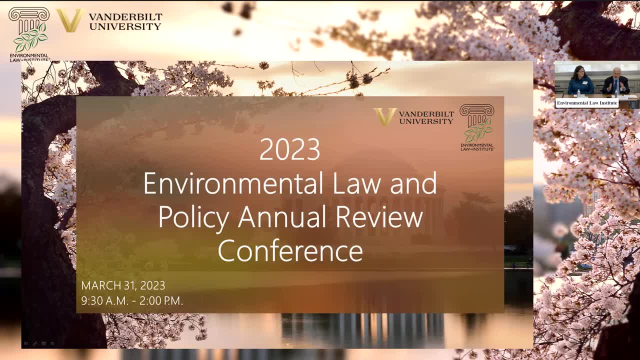 in the future. The most significant role in this global climate problem is to look at the economic impact, the social impact and the economic impact and the global level of climate change that is on this planet. The second step is the economic impact on the global climate in the future. 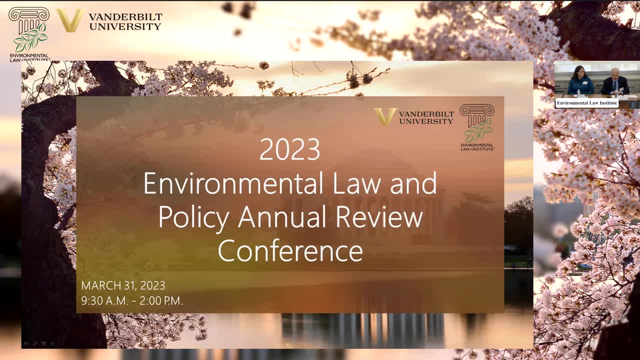 exists and whether it has been exceeded already depends on the individuals, the communities and ecosystems. you're talking about their geographic location, the particular climate risks they are facing And I want to emphasize- and the values that they hold about the things that might be. 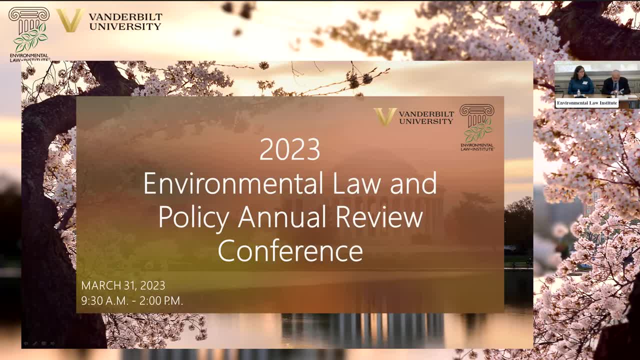 lost And I would suggest to you- Robin referred to the discussion they have about migration, Which is very real. I would suggest to you, for example, that the tribal community of Shishmaref in Alaska, whose elderly sadly recently voted to move their entire community to another location. 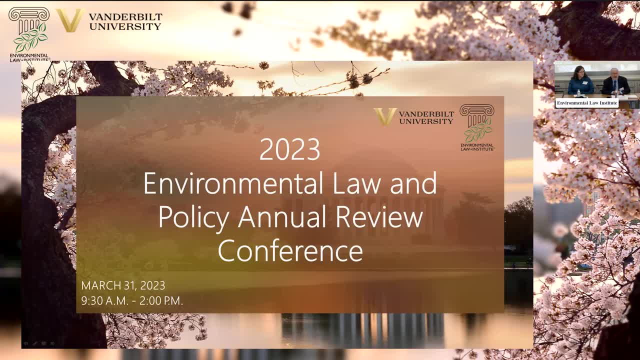 despite the precious cultural resources that they are losing, would say that they've already passed a critical threshold. The bottom line is: impacts are already occurring and thresholds, both physical and socioeconomic, are already being exceeded. I want to be clear. I'm not saying this to disagree with the points. 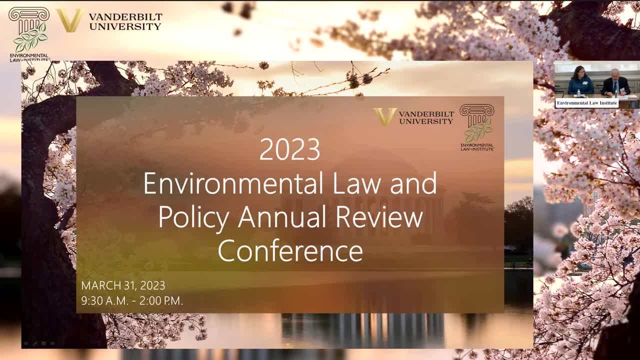 JB and Robin have made, but rather to strengthen their argument that these trends have significant implications for governance and law And to reinforce that engaging now in anticipatory adaptation is the best chance we have of avoiding a breakdown in democratic governance. Governance, Anticipatory adaptation. 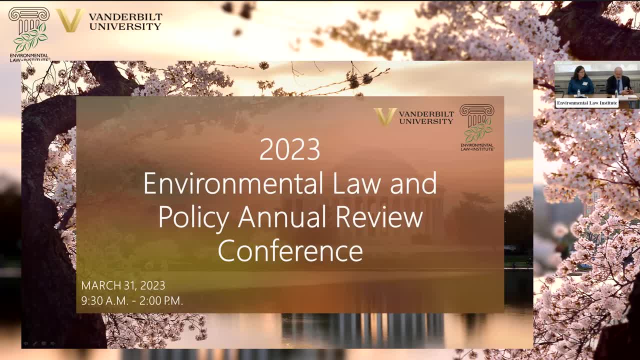 adaptation is smart government And it's also smart business. The real question- and I was thrilled to see the toolkit that you have in your paper- the real question is: how do you do it? Given their focus on four degrees centigrade, JB and Robin recommend reorienting adaptation policy for 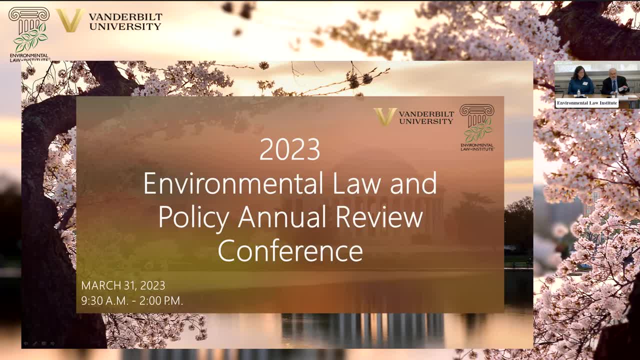 anticipatory redesign away from incremental adaptation that is carried out largely at local and state levels, local and state scale, And I think that's a great point, And I want to hear your views on the reorientation of this policy by a more regional and national And I agree. 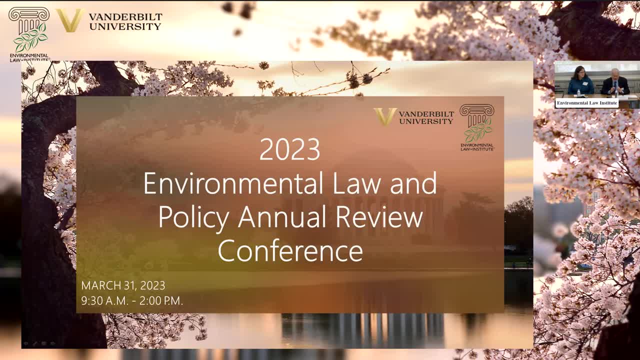 I would suggest to you as a bit of optimism here and opportunity. I would suggest to you that this reorientation is already beginning. I'm pleased to say that many of the items in their toolbox for redesigning adaptation are already being implemented in the United States by the federal government. 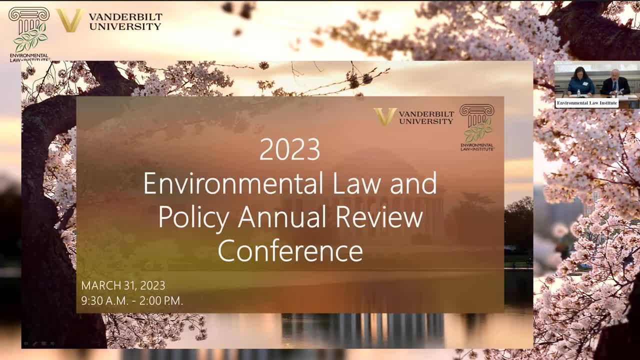 by federal agencies like EPA, and by the private sector, the insurance industry, for example. President Biden's executive order on tackling the climate crisis, which he signed the first week he was in office, as well as landmark legislation like the Infrastructure Investment and Jobs Act and the Inflation Reduction Act, put these mechanisms 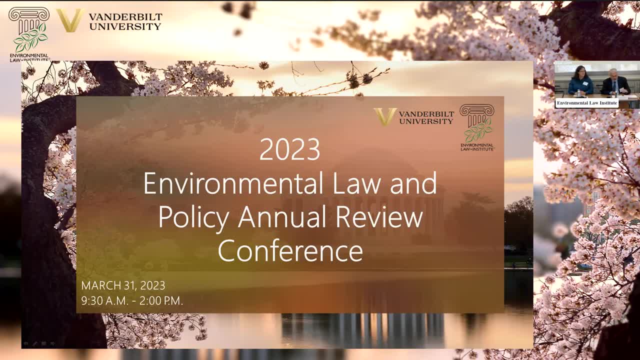 at the national and regional level in motion. We've just started. There's still a lot to do, but it's happening. For example, JB and Robin highlight the value of letting the market direct investments in adaptation in the right ways. We've already been seeing that happen Again. 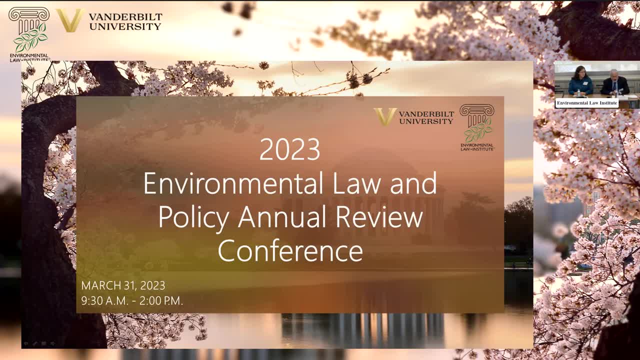 reflecting off of your example of extreme events, NOAA has reported, as you just heard from Carlos, that since 1980, not just Dallas but the whole US- has incurred over $1.5 trillion in damages from weathering climate disasters, each of which cost at least $1 billion. So that's an underestimate. 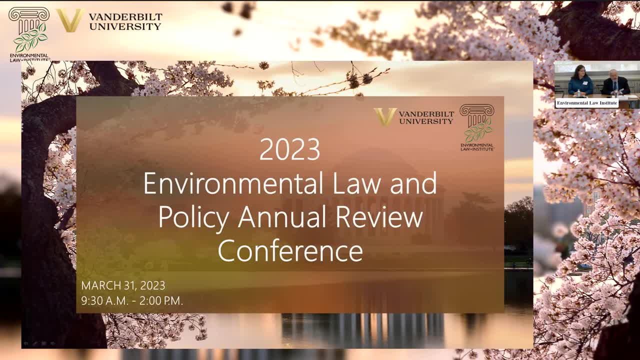 What's so telling about that? Well, the economic impacts have become so severe at this point that the vulnerability of local communities to future impacts is now influencing credit ratings for municipal bonds. And I got to tell you, cities care about that And, trust me, the markets care. 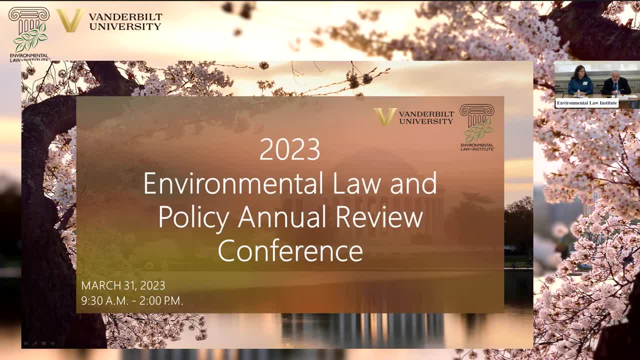 JB and Robin also argue that planning and prodding by the federal government to guide private actors to make climate-smart decisions and investments is critically important, And I agree. They note, for example, that there is considerable agreement that the US's basic infrastructure 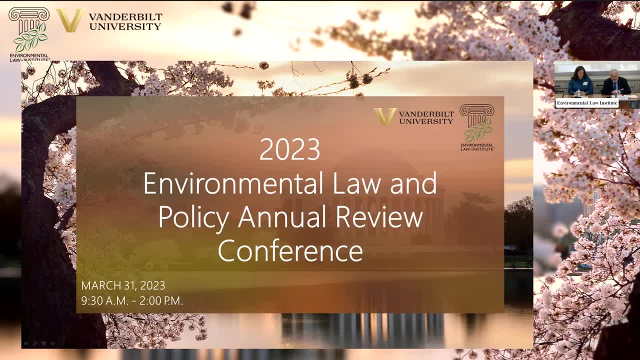 already warrants increased investments. That is why the Infrastructure Investment and Jobs Act of 2022 provides billions, billions of dollars for federal agencies like EPA to provide resources to states, tribes and local communities to invest in infrastructure, with a concurrent focus on advancing environmental justice. And I want to tell you that a huge and people aren't aware of. 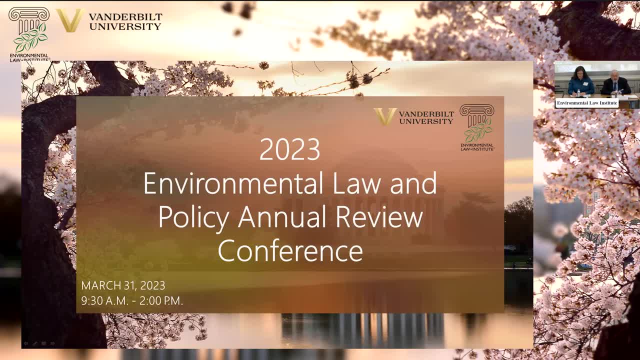 this yet, but a huge focus is being placed by all federal agencies on ensuring these investments lead to outcomes that are resilient to the impacts of climate change. For example, EPA, which received $50 billion from the Infrastructure Investment and Jobs Act criteria are now being integrated and included. 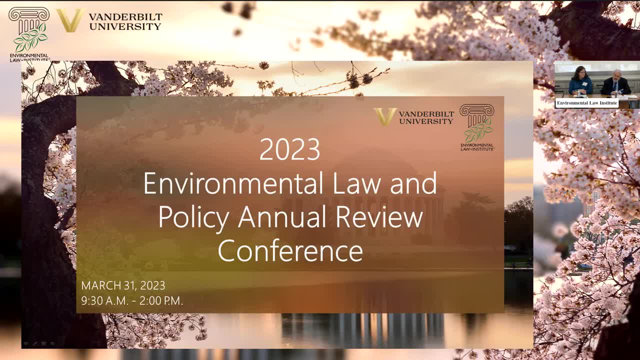 to incentivize climate adaptation in the various financial mechanisms we have for distributing those funds. But we're not starting there. We're also providing the technical support to the recipients of those funds to empower them and help them make climate-smart investments. It's not 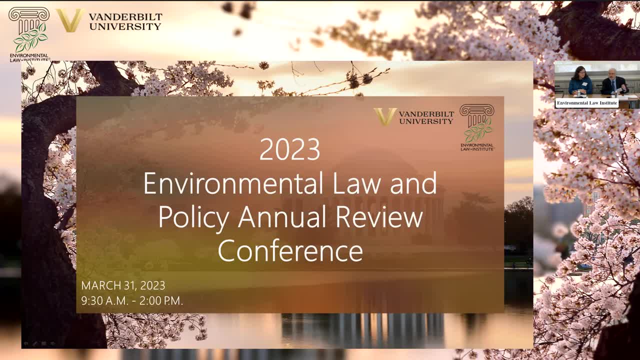 just enough to write checks, but I've got to tell you what we hear from middle- to smaller-sized communities and tribes is: we need the technical support to understand how to make climate-smart investments Very quickly. JB and Robin also emphasized the need for investment in research. 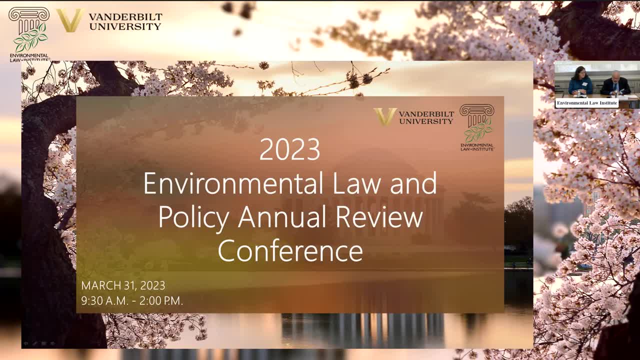 to better inform adaptation decisions and to provide the necessary tools that we hear from communities to help them make climate-smart investments. So we need the technical support to understand how to get the right information back to those communities that they need- In fact, the US. 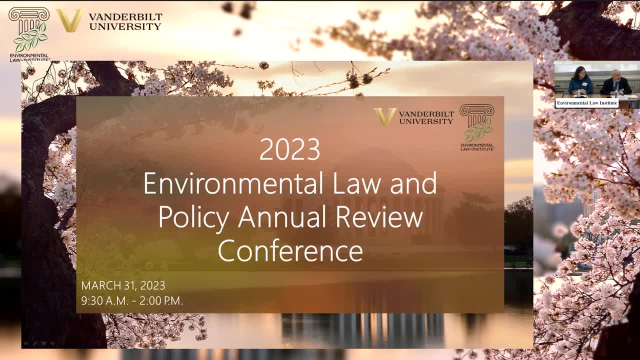 Global Change Research Program is doing that, producing things like the National Climate Assessments that, in fact, are required under the Global Change Research Act of 1990 in order to provide timely and useful information to support decision-making. By the way, the evolution of that, 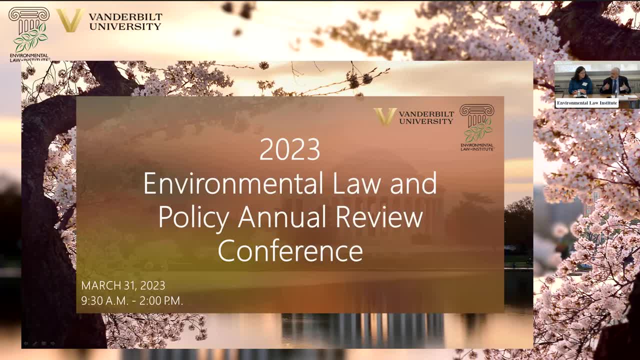 research program towards providing useful information in a timely fashion for decision-makers. global change research program. In addition to them, many federal agencies like EPA, NOAA, DOE and DOT are making significant investments to produce the tools and technical support and information needed by decision makers in the public and private sectors across the nation. 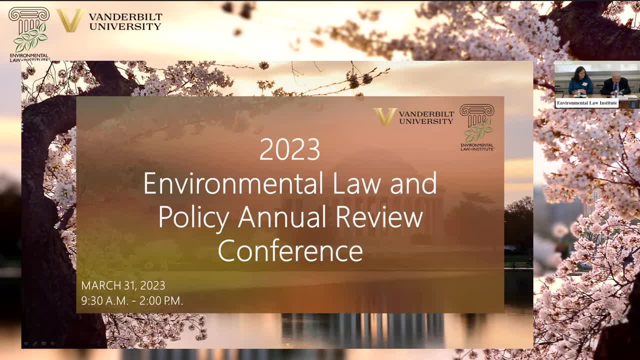 If I could just take a couple more minutes. Robin and JP also discussed the need to create a national foresight system for adaptation planning And to show you, as has been suggested, how quickly things are happening now: Just last week, the Office of Science and Technology Policy. 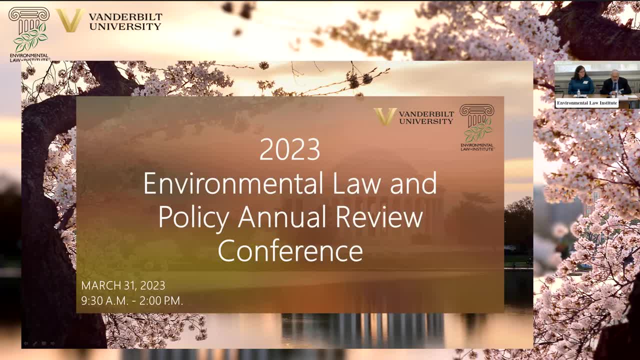 released a report outlining the development of a data-driven climate services system by the federal government, a coordinated federal government that will provide the types of services a national foresight system needs to provide. We're just starting And it isn't going to be easy, but we are moving in that direction. 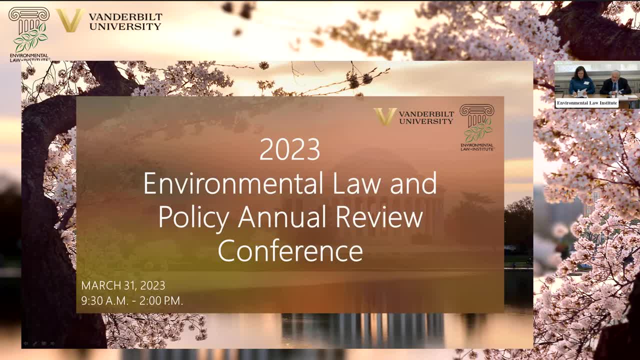 And finally, Robin and JP talked about the need to develop programs that create paying jobs and provide training and adaptation skills, And again, that is already underway across the federal government. For example, agencies like EPA and DOT are already developing and providing training for people and communities across the nation to increase their awareness. 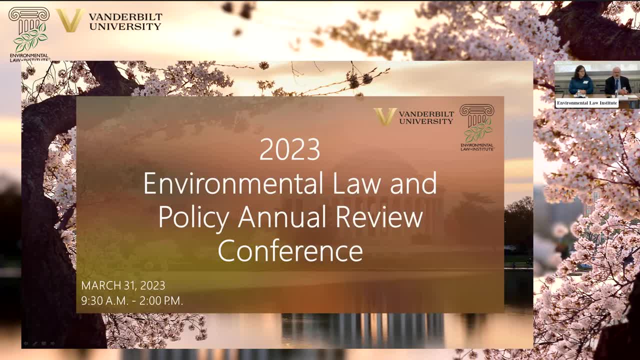 about the challenges of climate change. It's a very important part of the process, as we've already discussed, And that's why climate adaptation even matters for the things that they care about on a day-to-day basis, And then to train them on the implementation of adaptation strategies. 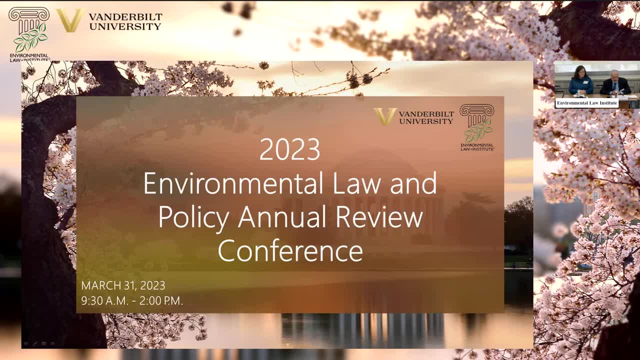 So, to conclude, I have to say I shared JP and Robin's concerns about the increasingly scary risk posed by climate change and for the importance of having concurrent governance efforts to both mitigate greenhouse gas emissions and adapt to climate change. Let me just quickly interject. 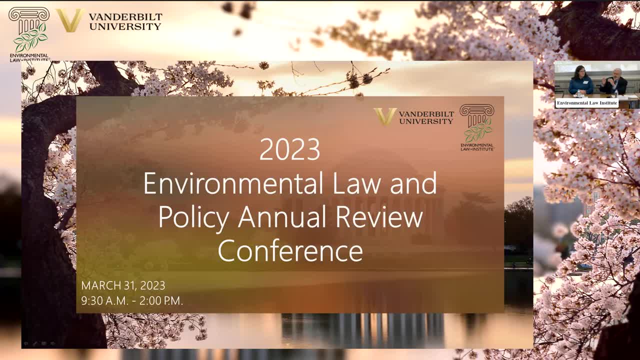 quickly interject. I work on the adaptation side. So much, Davey, of what you said about our experiences, which mirror each other, from 10 years ago, 20 years ago, 30 years ago, where adaptation was a dirty word, It was viewed as a diversion from mitigation. We live in a different world now. 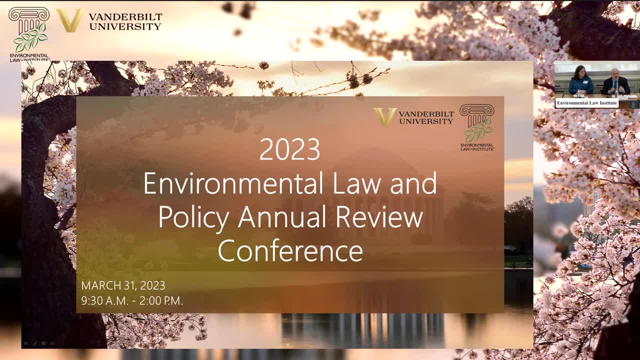 thankfully, and it's still evolving. But let me be clear: any smart climate change policy must consist of both mitigation and adaptation. You need to go hand in hand, And I would simply argue in conclusion that, whether or not we feel a need to prepare the 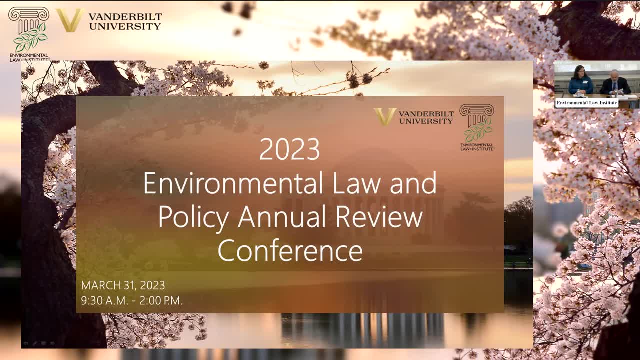 nation for a path to a four degree world or beyond. we can and are already taking significant steps to develop a robust national foresight system for climate adaptation And we need to continue doing so and we need to do it fast. With that I'll stop. I just want to point out: 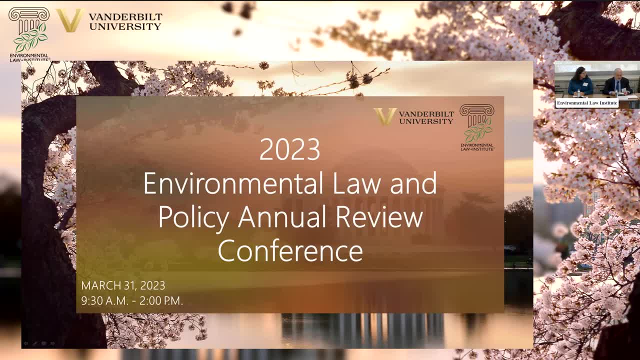 before we move on, that being a Nobel laureate qualifies you for two extra, And I love a panelist who actually starts this stuff. And thank you also because I think for so many of us who work on these issues, it's easy to despair. And thank you for pointing out that. 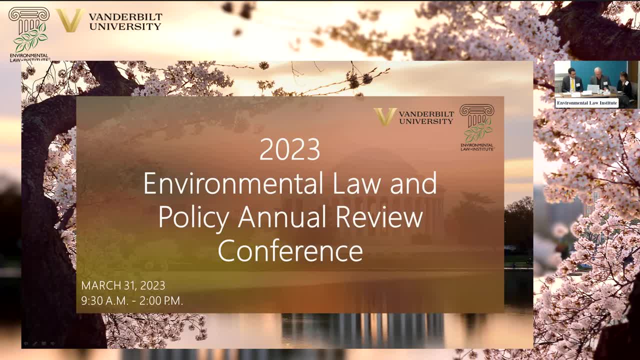 there is some momentum going at the federal level, So thank you for those comments. I want to just take one second and remind the webinar participants to look in the chat. There are instructions for how to switch your screen so that you will be seeing the speakers, not just these lines. 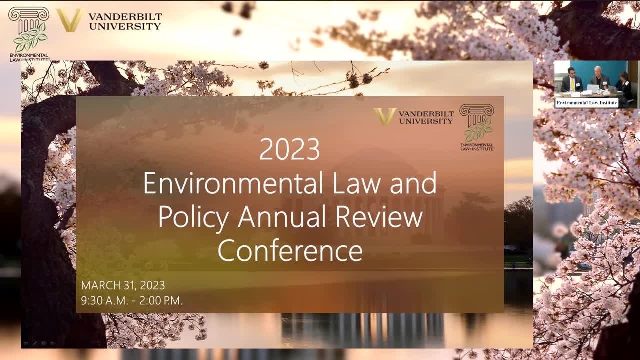 So we have over 150 participants, including people around the world, as far away as Nepal. So yeah, so we're going to hand it over now to Rod Schoenover. Hi everyone, Thank you for the invitation to organize this, Thanks to the panelists. I read this article of great, great zip code: 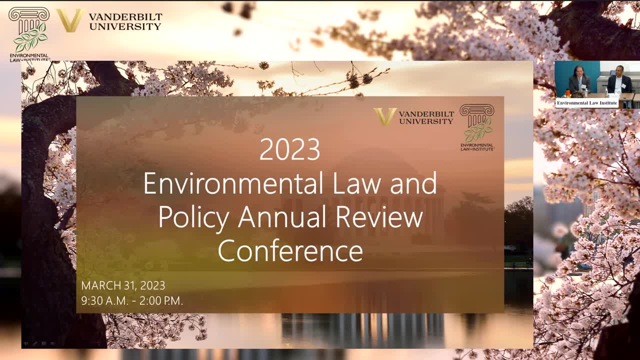 Thanks to the panelists. I read this article great, great, great. I read this article great, great. I read this article great, great, Great. And any other questions And any other questions interest. I read the full Minnesota version as well. I thought it was very intriguing And 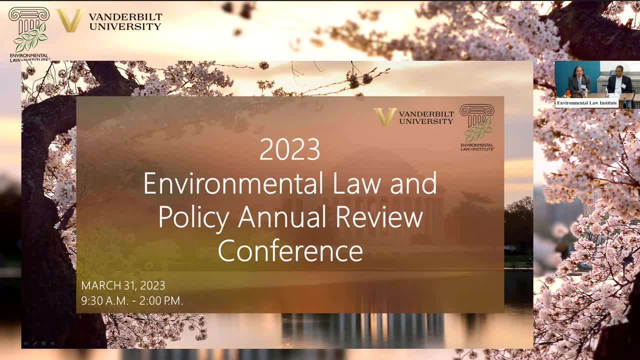 coming to this topic as a scientist, as a complex systems physicist, and also as someone who worked in the security community for quite some time, including at the State Department as the Paris Agreement was being constructed. I tend to be an optimist on many things regarding climate change. 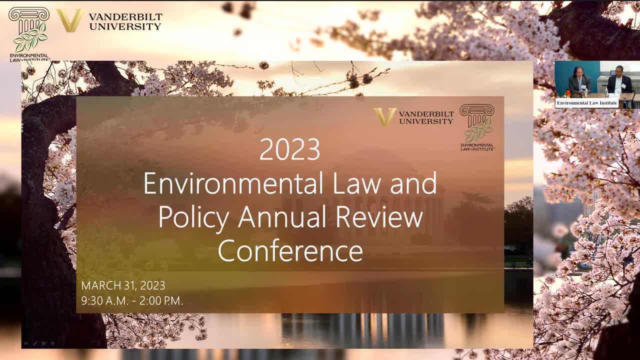 However, I'm going to really lean into doom, Because what we're really talking about, and the title of the paper that I offered up, is really the dangers of underscoping risk. I don't know what it is, But what we're really talking about is risk assessment in many of these categories. 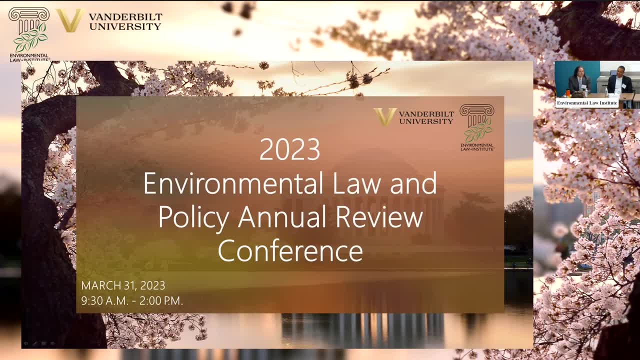 So, basically, institutions and models that don't evolve and step with changing conditions cause problems. They no longer serve the institutions and people that are in line to serve And at times they can actually be part of the problem. And so I saw this in the National Security when I saw a lot of resources. 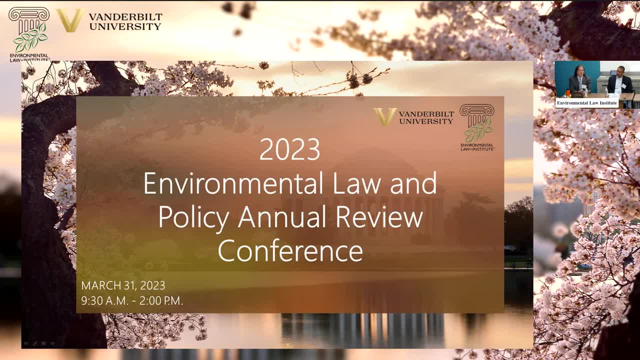 the doctrine and architecture becoming increasingly misaligned with the reality of the planet on which we live. And I think, in terms of the conclusions that JB and Robert come to in the paper, I think they arrive in sort of the same place, that, especially in light of cascading change tipping points, I think they argue effectively. 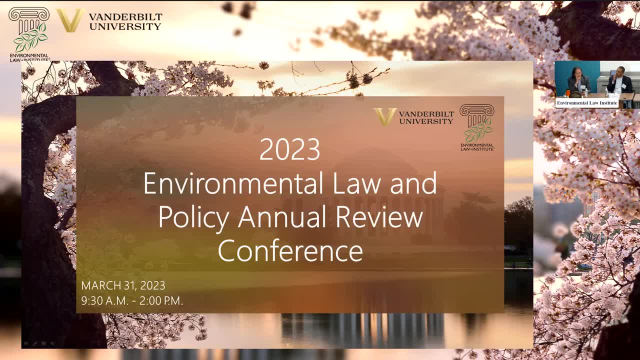 that governance measures will fall short if institutions don't adapt and embrace. We've already talked about it. It's the real possibility of two degrees Celsius. A lot of people, when you close the door in the scientific community and the security community, will say two degrees, has long been conservative. 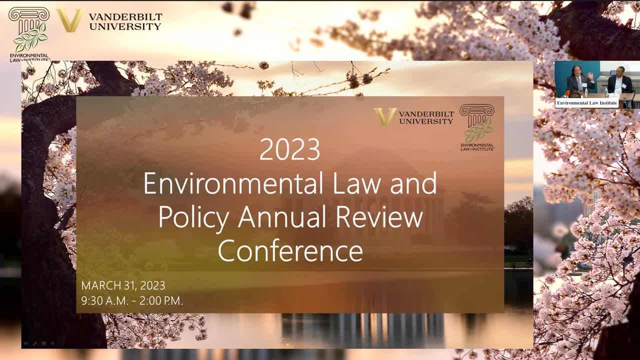 It's one thing to talk about it as something as a target for the multinational, multilateral institutions to aim for. It's another thing to as a target for how we structure our society And so the world that I'm, I'm most recently a part of the security community, is quite pragmatic, quite realistic. 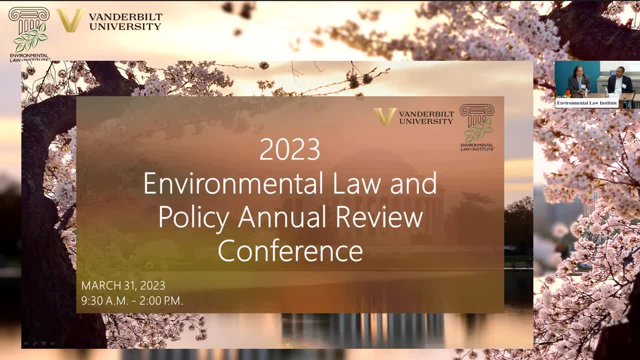 And they want to focus their attention on realistic targets, And so I think the authors are keenly aware that discussions of four degrees Celsius bring out criticism of being doomous. I think some critiques that. Yeah, I think sometimes that critique is fair when we are trying to communicate to the public. 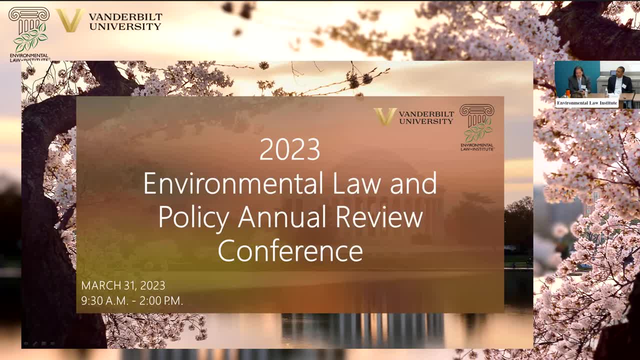 about temperature targets But, as I said, it's clearly long been too conservative for adaptation planning In the IPCC report. I'm going to pull out another quote, And that's all. pathways that limit warming to two degrees Celsius involve rapid and deep. 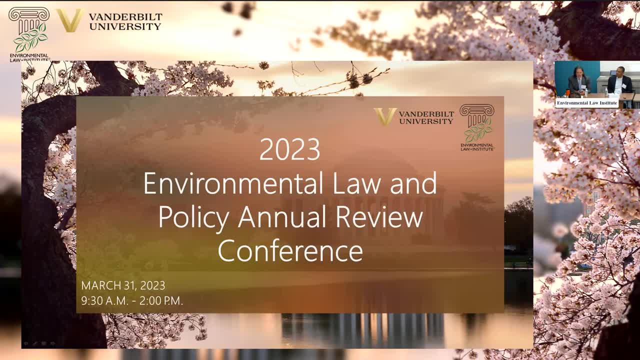 and, in most cases, immediate greenhouse gas emissions in all sectors this decade And those emission reductions are happening. but in physics we talk about vectors. We have to have speed and direction. We have the direction, We don't have the speed. 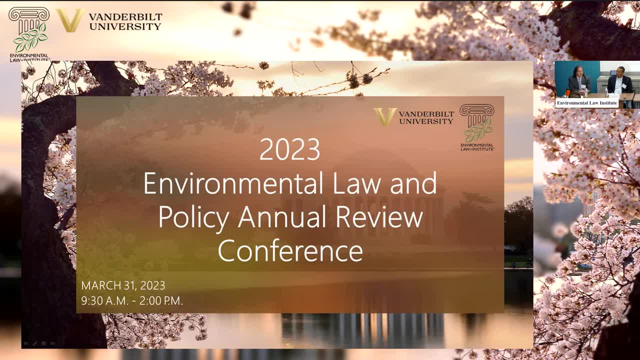 And I don't. The flip side of it is The flip side of that statement is what happens if we don't have transformative change, Because I see incremental change and I see a lot of it and it's good, but it's not transformative. 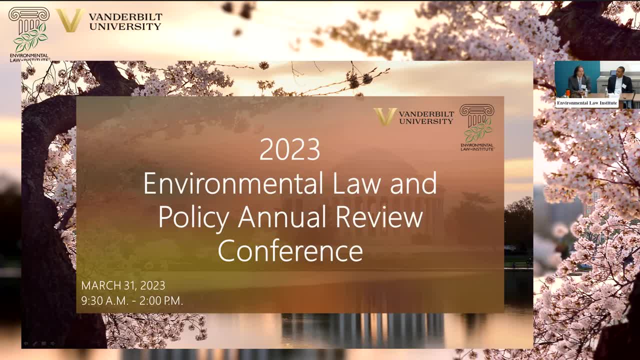 And unfortunately, in the United States we also have a political system in which two parties don't agree on the problem nor the solutions, And so it's hard to separate the scientific, technological piece from that. I think it's Any intended planning that's predicated on assessing the risk of a certain target, especially. 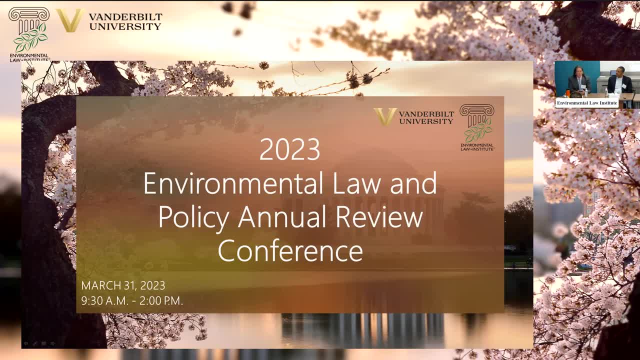 when it's something like two degrees, the danger of low-balling, the risk is high. So we don't do this in our normal life. We have a career-changing. We have a career-changing. We have a career-changing Meeting somewhere downtown, especially somewhere we don't know. 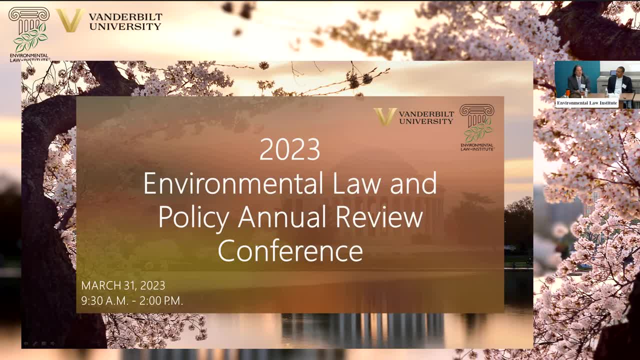 We don't try to time it exactly. We build a cushion Because this is So. planning for two degrees Celsius is bad policy for adaptation, And so I think that's something that the military does: builds It assesses, not the worst case. 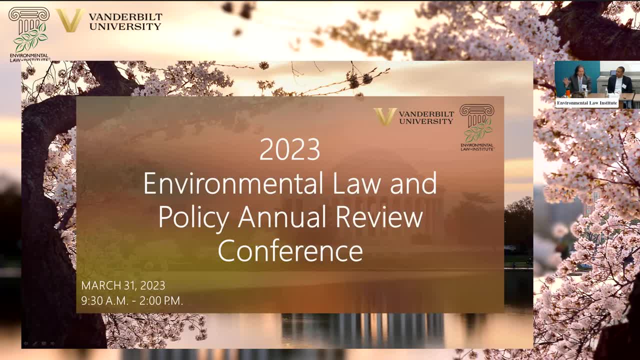 Possibly, But a bad one, And uses that in terms of many of its risk assessments. I think a highlight of the article was the invocation of, And really extension of, the anticipatory governance concept. I think it's Even in times of relative stability, it's a good idea to identify risks in advance. rather, 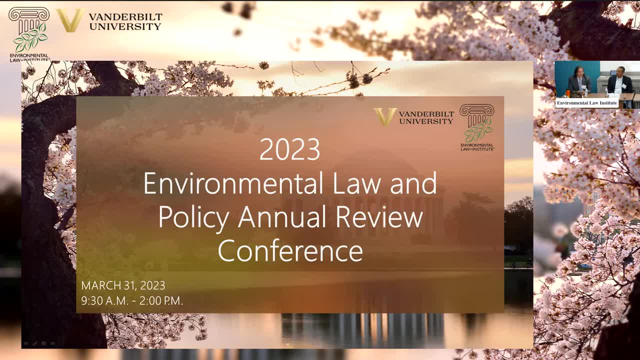 than being hit by it. It's a good idea. It's a good idea to identify them and trying to respond Right. Reactivity never leads to good outcomes or not optimal outcomes. It often leads to maladaptive responses and outcomes. I really like the author's use of redesign in the discussion, especially the focus on 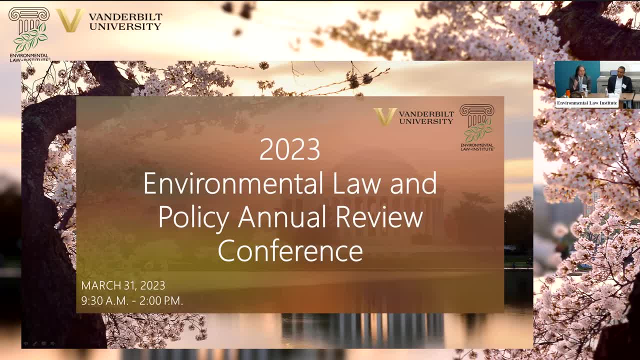 sociological, societal pieces of our resilience. And I could talk a lot more about the strengths of the paper, but I want some critiques. I want to critique the paper a bit, if I might. They call for the development of enhanced foresight capabilities. 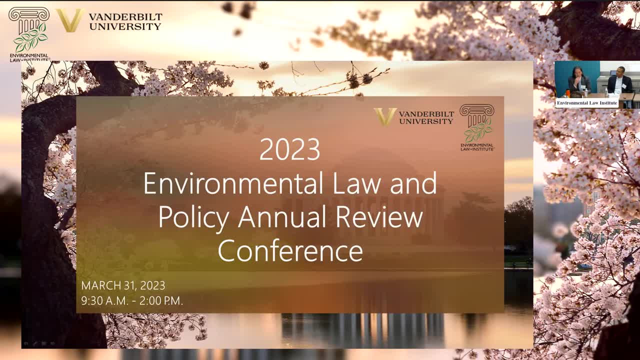 This is a part of the intelligence community I worked on for quite some time And this is greatly needed. There's no question We should temper our foresight expectations, Since the systems we're looking at, As the authors have in many ways, are unforecastable. 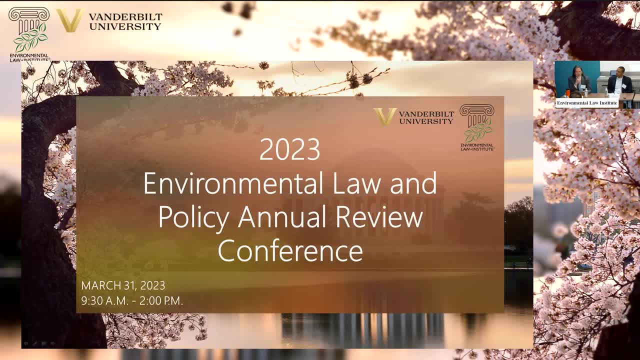 And more data doesn't get you more foresight. And that's not to say we shouldn't found the problem, but we should temper our expectations. As someone who worked on infectious disease and pandemic risk planning foresight, You know I think it's important to bring up COVID and argue maybe if we had appropriate foresight. 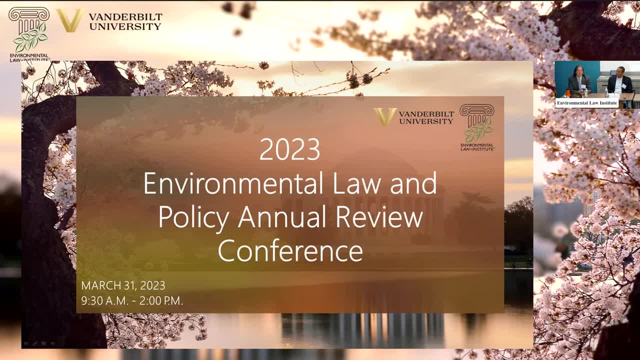 we might have had a better response. The counterargument is: we had foresight in SARS-1,, MERS- you know a number of other. In fact, I myself wrote in the annual threat assessment the word coronavirus as a threat. 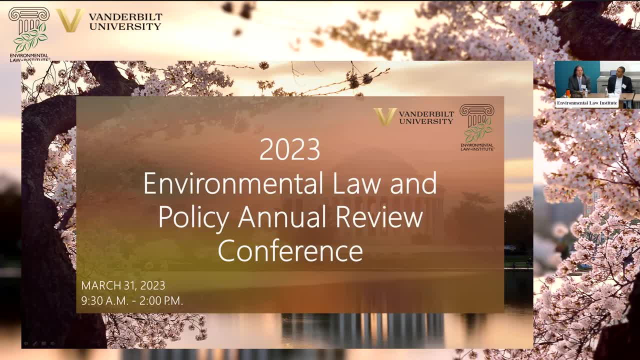 three years before it happened, this latest coronavirus. So foresight in itself, and again the authors say this isn't enough. You also have to make the decisions on that foresight, And so oftentimes we don't put enough effort into enhancing decision-making right. 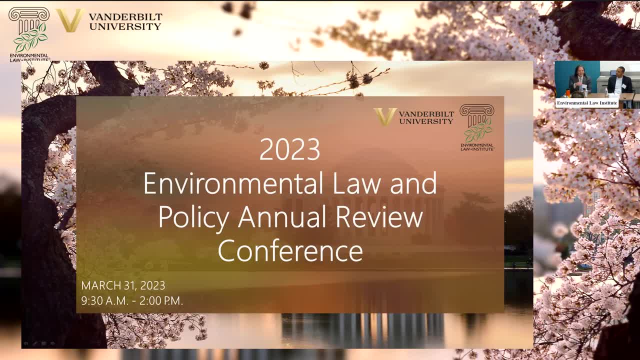 All the warnings in the world aren't going to help Unless you actually get it Right, Unless you actually get that decision part. I think probably for me the most problematic part of the paper- and it's actually the part that is the most interesting- is the title and the thesis behind it, the four degrees. 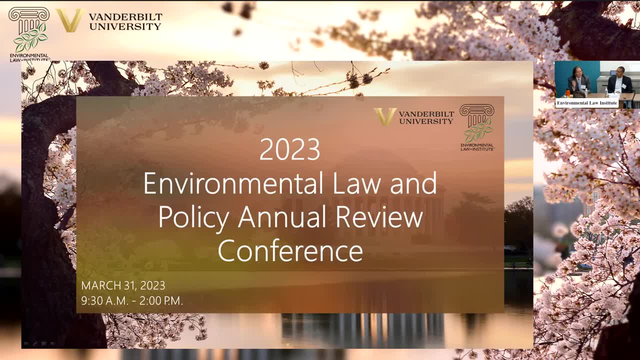 Celsius, And it's not because it's too doomy. It's because when you attach the danger of pneumonia- Right, The danger of a moment- onto a temperature, you're actually missing other really incredibly important thresholds, right? This is nothing that the authors don't know already. 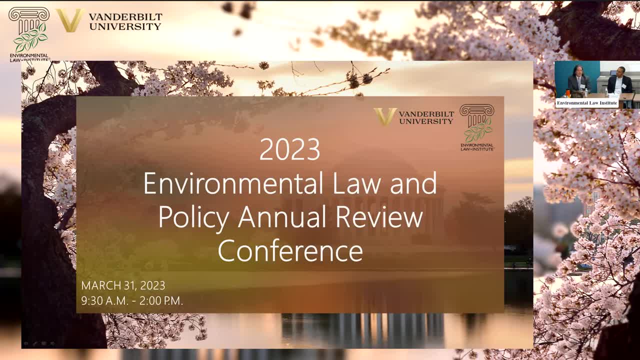 And I really liked the treatment of tipping points in the article. But the systems that the climate community models in their Earth system models don't contain, And I think that's the most important thing. They're just the most important thing, Because that's the most important thing, right? 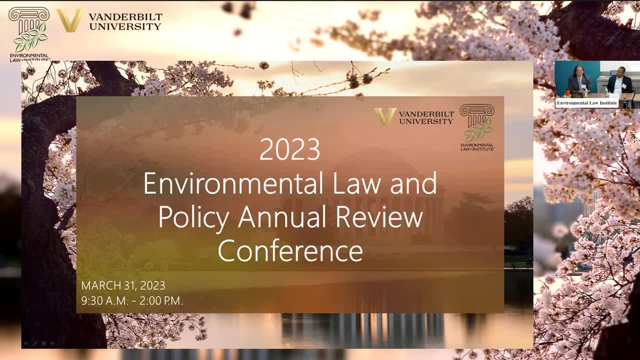 Because they don't really take on many of the things that are happening. They don't really take on the dangers of soil toxification right Or most of deforestation or you know a lot of the things that have happened in the other. 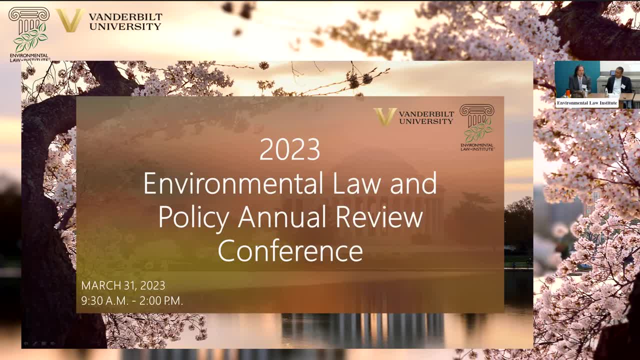 planetary boundaries that are not climate change, that greatly affect the vulnerability of human systems to climate change, Right. A lot of the things that the tipping points, that temperature can push us over, they can also be pushed over by other things that are happening, right. 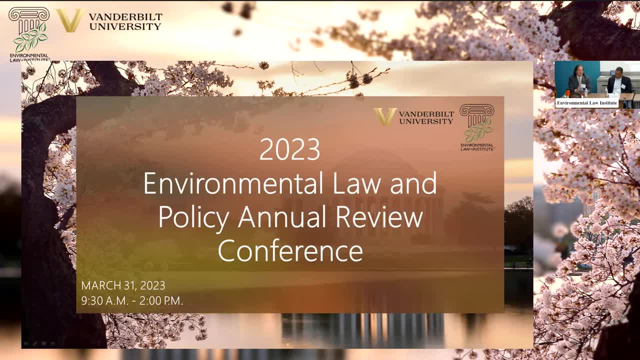 Nitrogen and phosphorus overabundance, for example. And so four degrees Celsius- provocative, I like it as a title, but we're in danger of passing a lot of these tipping points at two degrees Celsius, And so let's not think that there's a. I mean intellectually, we can talk about four. 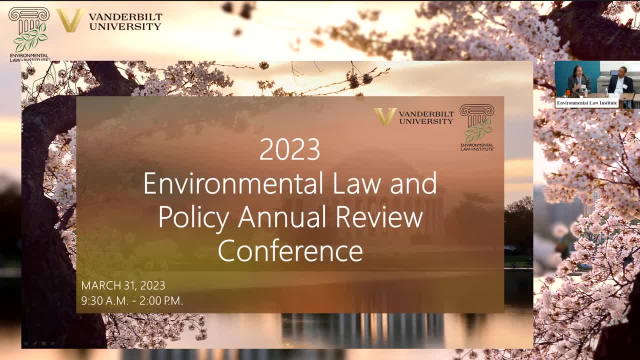 degrees Celsius. as long as we internalize, we're in a lot of danger well below four degrees Celsius. And then, lastly, I would say, you know, the politics of the moment are important in terms of, you know, and this is not a critique of the article, it's a contextualizing comment. 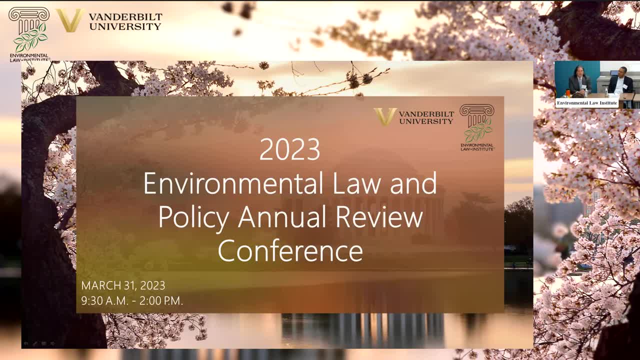 We have a poll Public in which that is to me, seems to me to be quite vulnerable to influence campaigns of all stripes, both foreign and domestic, of which creates enormous challenges to governance. It's hard for me to see a trajectory where the population of the United States, where 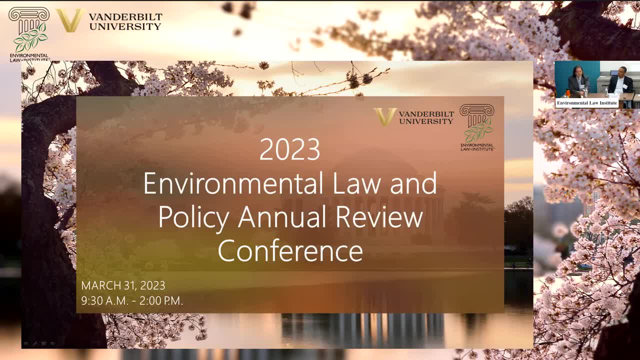 we sit now Moves to a place where anticipatory governance is not seen as a very unwelcome, maybe highly intrusive set of activities by either the government or industry. I mean, it's clearly the right thing to do, but I worry that we're underscoping the real. 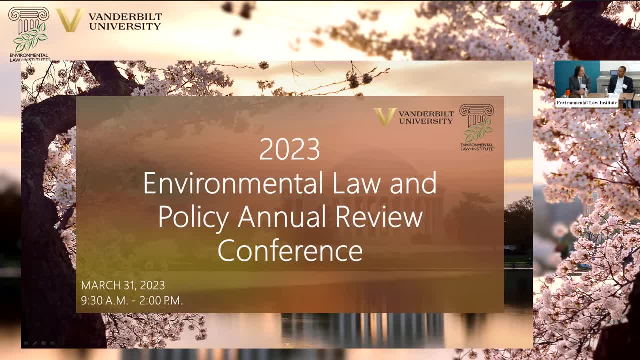 risks of doing that as well. That's it. Well, thank you, And you're right, that was very sobering, but also very, very thoughtful. Thank you for those comments, Hannah. you're up next. I will clean up here a little bit. 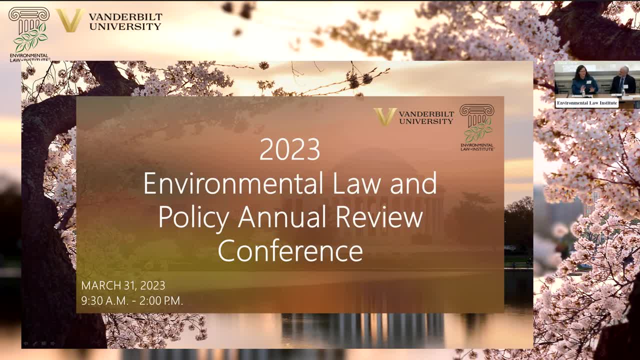 I am also going to bring us a little bit back into the doom era, But as a practicing attorney, I also am going to kind of refocus us on the legal questions here. These have been really Excellent and informative presentations and discussions. Also, it's rare that I get to sit on a panel with both a sage hen and a fellow Texan. 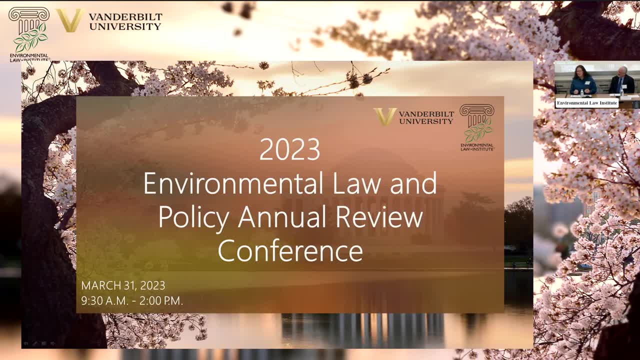 As an environmental lawyer, it's really cool that my undergrad mascot is a sage hen. But I have to admit I felt an increasing amount of dread reading this piece. but it wasn't. It's not because of the thoughtful explanation for why we should both recognize that. 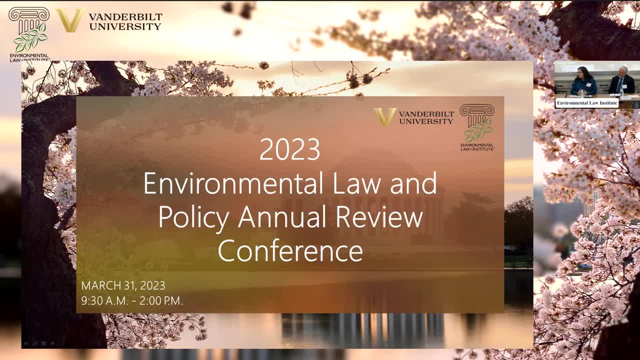 It's not because of the thoughtful explanation for why we should both recognize and plan for the possibility of a world that doesn't meet its current climate goals. It goes beyond two degrees and potentially up to four. You know, as we've heard with great eloquence, the communities in our country are already facing these risks. 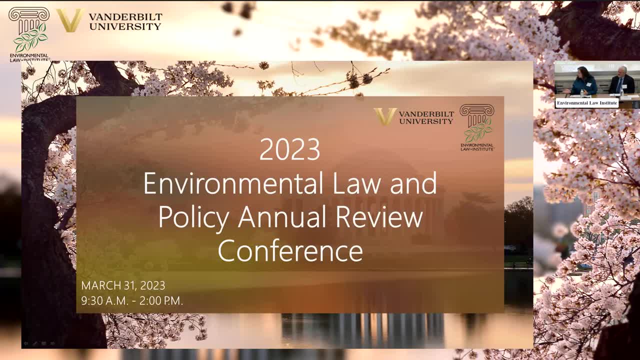 They're already facing these impacts and struggling with what it means for their cities, for their communities, where they're going to go. But rather, that dread came because, as lawyers are prone to do, I began to think about the legal mechanisms needed to achieve these goals of redesign, adaptation, as the piece walk through, the ideas, their ideas for needed future action. 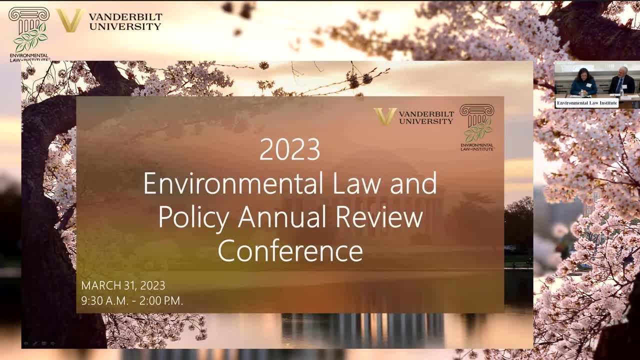 This wave of pessimism and dread came over me because I could not read the article without thinking about the current legal and jurisprudential trends that would impede even the earliest steps the authors have suggested. You know, as we've heard the- and the authors know in good detail, you know, our current approach to adaptation. 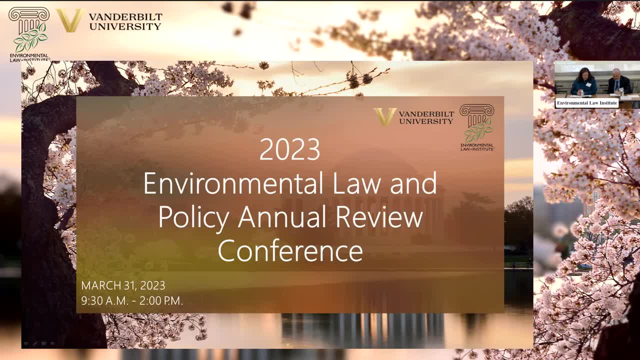 Besides in the in situ approaches and the three R's, much of that legal authority for adaptive action sits with local and state jurisdictions right now, You know, and they face competing incentives as we've heard some of before today and you know are probably are not well suited necessarily to be able to comprehensively plan for these larger changes. 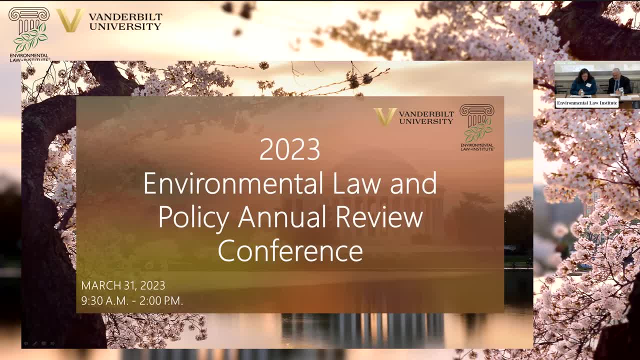 Each of the redesigned typologies discussed many and many of the examples of potential actions needed. We'll require the federal government to do big things and, you know, in ways that they haven't done before. You know, I appreciate the references back to prior, prior examples, but there are big distinctions between those and what's happening now and our current environment. 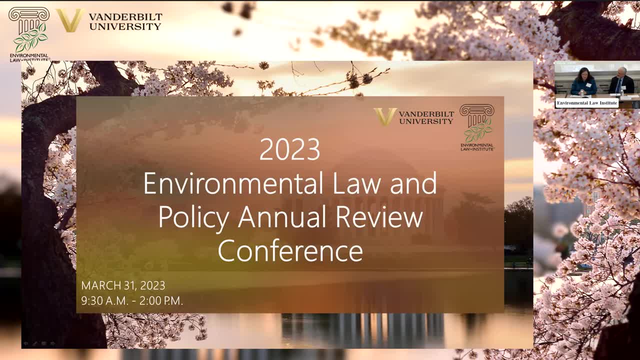 And using laws developed often without the foresight of for those needs, and ideally, Congress would act to address some of these shortcomings. But you know we're facing significant headwinds today. We're facing significant headwinds there. This has been alluded to already and it also is discussed in the paper, so I don't want to make this sound like like Jamie and Robin did not, did not, did not think about this. 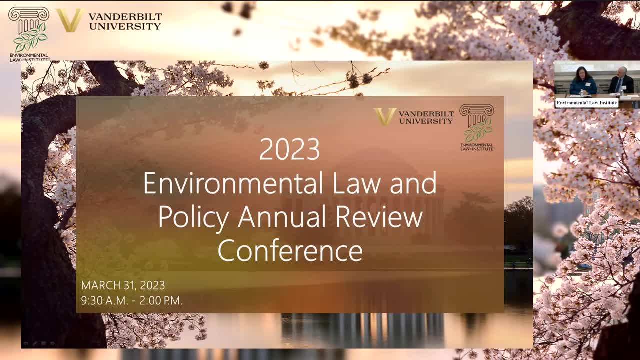 We're in the midst of an historic assault and federal authority to address hard problems, and particularly those designed to address climate change. This movement is the culmination of decades of work to clamp down on federal regulatory action and the courts, developing newly restrictive legal theories that they're that we're now seeing put into action. 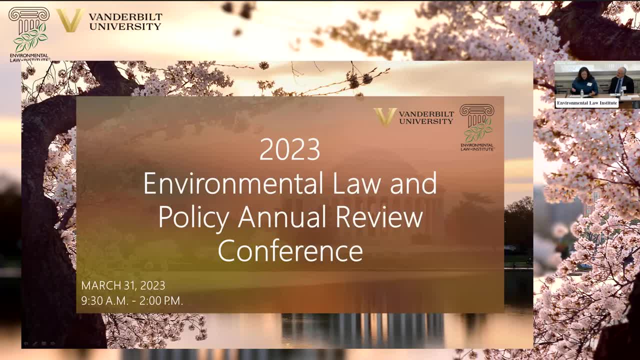 that we're now seeing put into action And aided by a reactionary political environment that we just discussed a little bit of, that limits the potential for congressional action and has spurred a rise in politically motivated legal responses to federal efforts to address climate change. You know, even the author's proposal on the the two degree foresight program seems relatively modest compared to the potential changes we will need to take further down the line once we enter these encounter, these cascades of change. 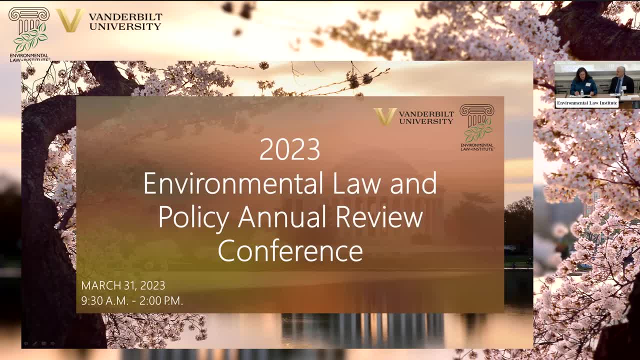 But even that seems disrespectful. But even that seems disrespectful And that, seems, is fraught in the current political and legal environment And that, seems, is fraught in the current political and legal environment. As I mentioned, JB and Robin are not blind to be its issues and they make a point of acknowledging them. They are somewhat optimistic that that some of these roadblocks will be overcome as the realities of what we face become more widely apparent. 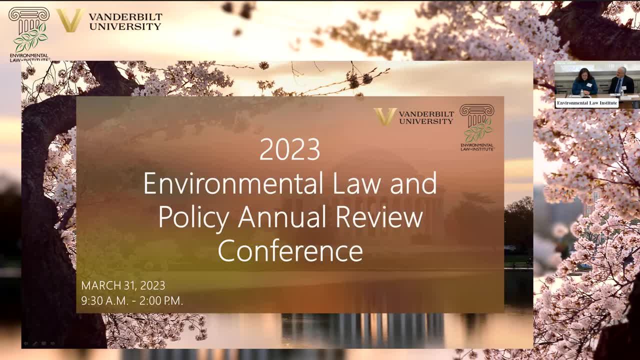 And to some extent I agree. political headwinds can shift quickly and stronger. congressional action may once again be a reality. However, I believe the more intractable, intractable problem is that of interpretation: interpretation of existing laws and the reimagining of the scope of actions the federal government can. 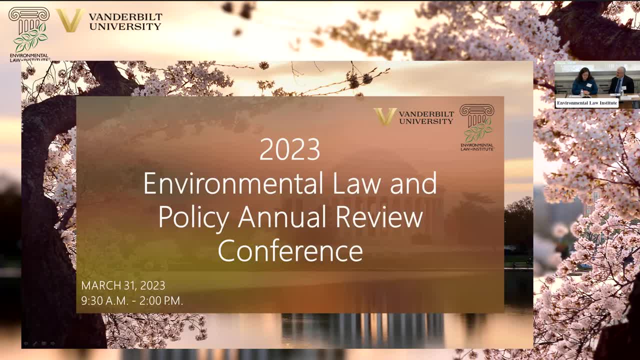 take, whether in Congress or in the executive branch. Our bedrock environmental laws and broader administrative laws are under attack by those who seek to significantly undermine the ability of the federal government to regulate and act in technical areas that require expertise and longer-term thinking, like climate change. The laws in the books today could be used to 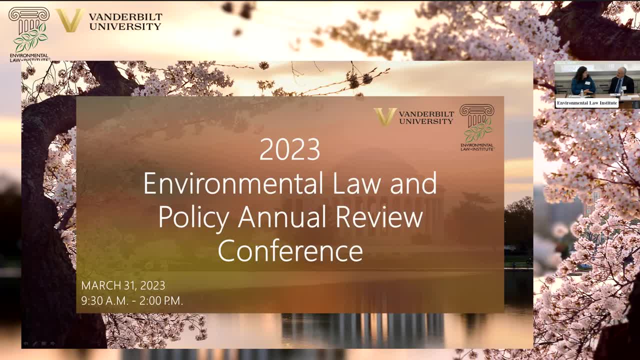 interest towards the necessary redesign and there's a lot of action going on at the federal level to try to do that, but they are currently being reinterpreted to limit the available action in the toolbox the federal government has, Like legal theories being used to undercut. 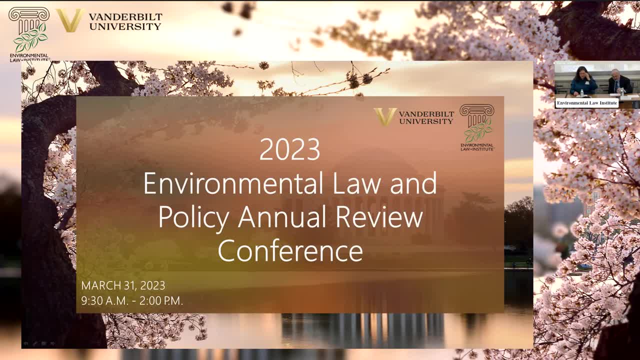 executive action. these legal theories being used to undercut executive action can also impede congressional action. I think we need to recognize the potential for how this can play out. These new legal doctrines, such as the major questions doctrine, could significantly alter the ways in which 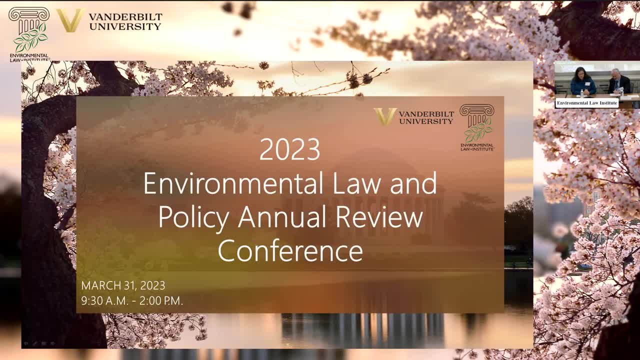 Congress can legislate to allow for agencies to effectively implement the goals of a statute In order to have any hope of being able to address the problems identified in the paper. should we exceed two degrees and move towards four? we must counter this legal takeover designed to 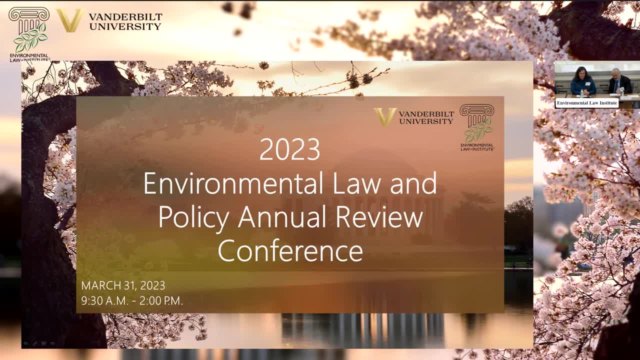 hamstring the administrative, state and governmental action. Doing so, I think, will require more than the national foresight system at this moment. That's an incredibly important piece of it, in whatever form it takes, but I think it requires a concurrent, dedicated effort to counter this. 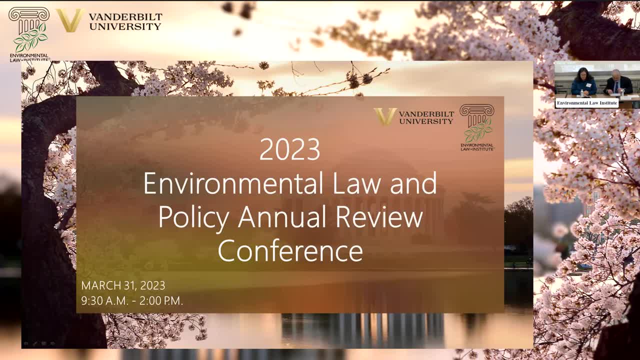 legal movement, this currently dominant legal movement that would make adopted governments harder, if not impossible. You know, essentially I'm trying to put a call to action out here to all the lawyers in the room and law students, because you know we are. we are talking about a legal 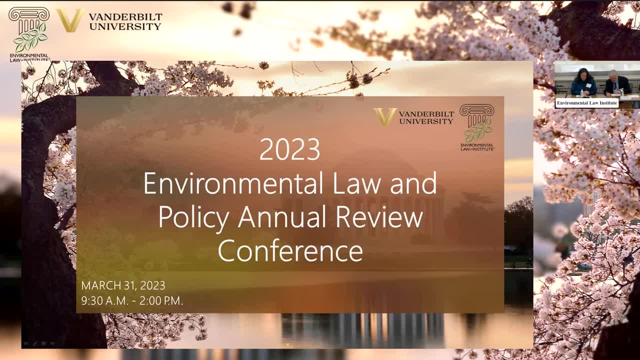 journal and legal implications here, And I don't want to be overly pessimistic. We've already heard about significant congressional and administrative actions that have been taking place in the last couple of years. They are bread and butter with what I do. for what I do, I focus on federal 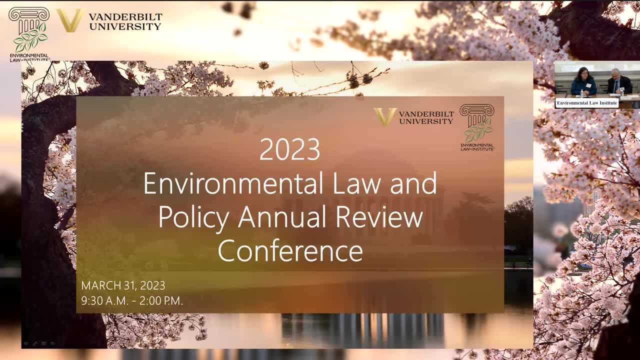 regulation and its implementation and, you know, ensuring that the courts don't undercut that action. You know, these incentives- some of the incentives that have you know been used to are being put into place through the Inflation Reduction Act and that came with the IIJA- are 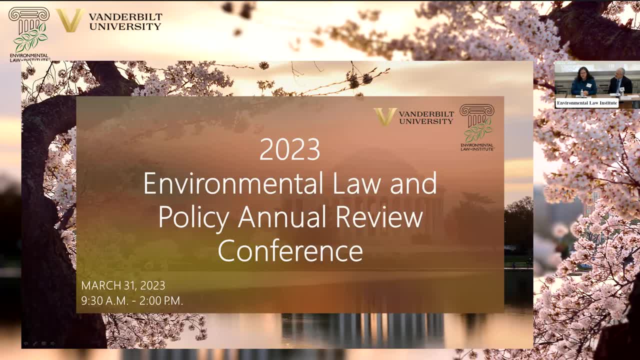 are part and parcel to to the just the ideas that we're in in this paper, but their success remains an open question. there's wonderful work going on in parts of the federal government right now and but it's you know- they also have to work their way through the courts. 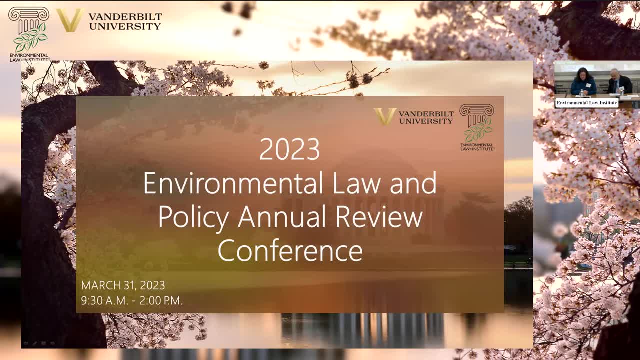 the extent of the impact of recent court decisions on the ability of federal agencies to do their jobs or congress to legislate in ways that allow them the flexibility to address hard and changing problems that we don't fully know yet. how that's going to come out, there's a slew of challenges to 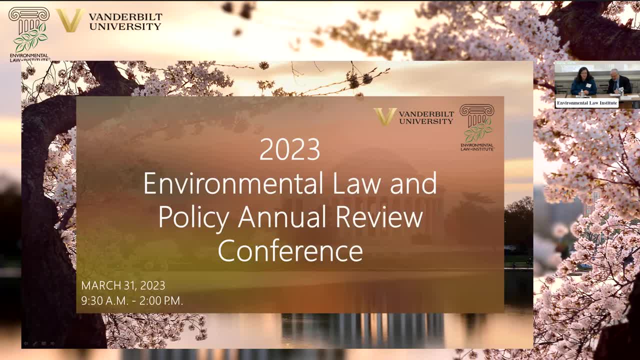 agency actions that will make their way through the courts in the next couple of years. some already are, are in that process at the moment- and these will define the scope of these limitations. so you know, as someone who focuses on this and many other attorneys out there who do, 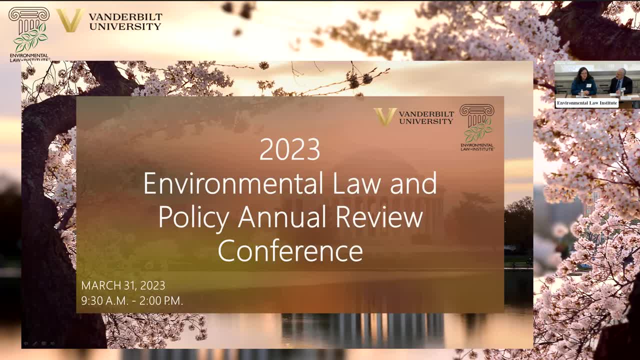 I think we're at a critical moment where we have to make sure that we're ensuring these, these wonderful moves forward and steps forward, have a place and continue to have a place in our governance. I wouldn't be able to do the work I do if I thought all was lost. I don't. what are lawyers for if not hard problems? right and 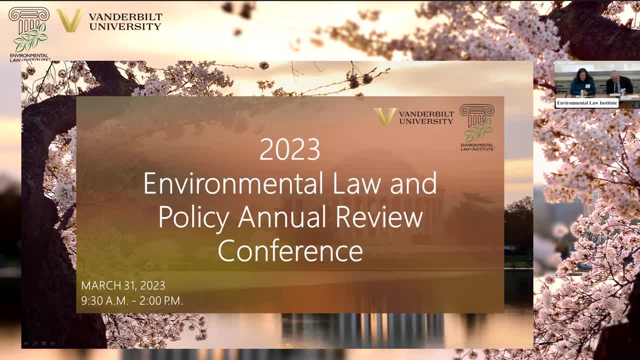 that you know. so, as someone focused on federal climate actions and how they fare in the courts, I see this as a call to action. identifying pathways to effective redesign, adaptation, and what that could look like in practice is incredibly important. and equally important is working to establish the legal precedent that will allow us to do so when we need to, and you know so reading this paper. 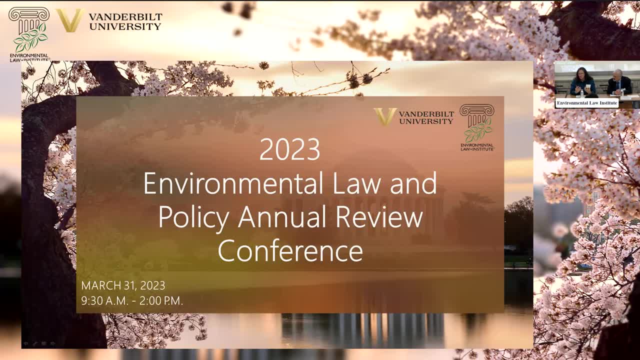 I just have this like big pull for urgency and moving that process forward. alongside the kind of adaptive- uh you know, thinking through the, the specific adaptive paths that we need to take. this requires a broader defense of the ability of the federal government to address climate change, pushing back and 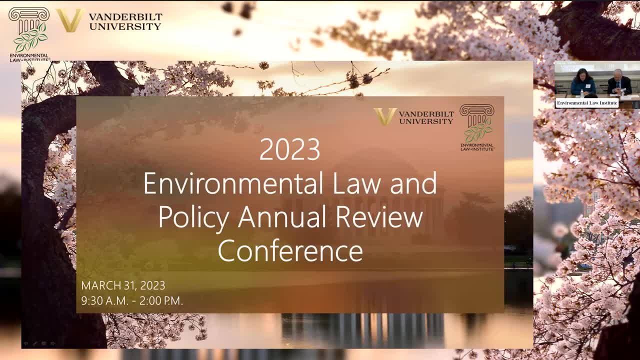 support on the current efforts to limit these actions and creative legal thinking about what legal structures must change to accommodate redesign adaptation. so I'll just you know, note. my final comment is that I look forward to the next five papers- the ones that they alluded to in their papers- that would outline more specific pathways to redefine adaptation, whether 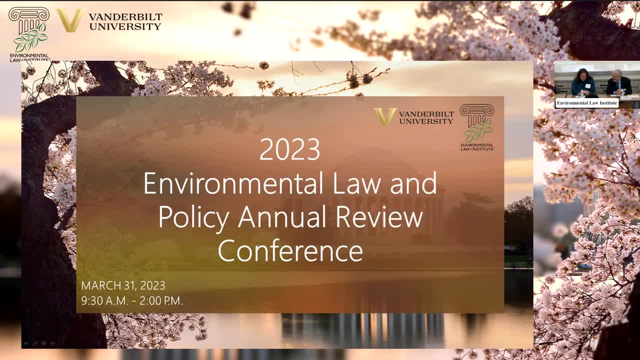 you're writing them or someone else and work with, and to working with other dedicated lawyers- hopefully many in the room. I think I'll just finish with saying that, JB and Robin, you have achieved your goal of, you know, getting the legal world's imaginative juices flowing and thinking about what this could look. 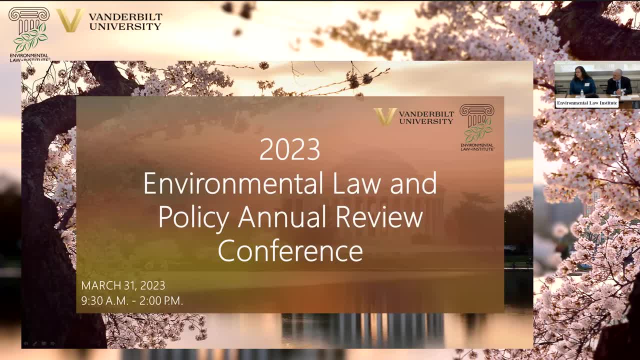 like um. you know, adaptation is a different problem than mitigation. I'm from Houston. Houston has a lot of adaptation problems, as the gulf coast and many other places in our country, so I want to thank you for your time and I hope that you have a great rest of your day. 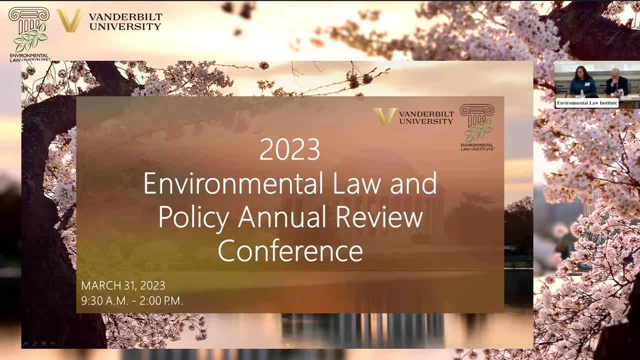 thank you. thank you for this and let you know, look forward to what comes next. I want to thank you for that perspective. so you two have been sitting patiently listening to all these comments on your work. do you want to take five minutes or so and in response, and then we'll. 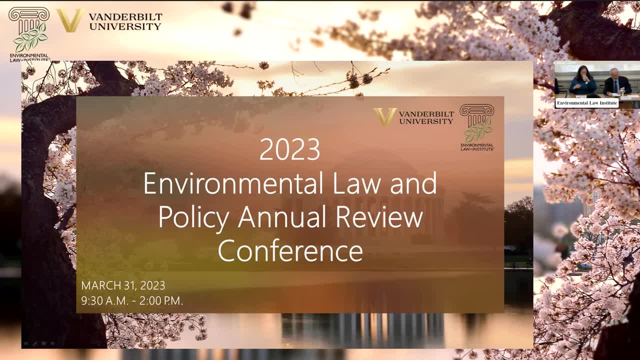 go to some questions and answers and reminding the webinar participants that they can put questions in the Q&A box. take off some of your thoughts. yeah, go ahead, I've got some more. let's go pretty quick. first of all, this fantastic, thoughtful and helpful comments on just this is what makes LPAR so great, uh, and it's such 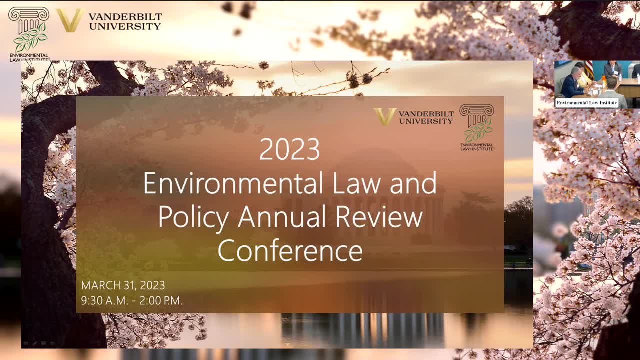 an honor to have our paper uh available, uh for this kind of conversation, uh, just quickly. so, Carlos, you, you've identified, I think, the real problems and challenge, but also why we need a national redesign thinking is that you know there are going to be inbound cities and outbound cities. 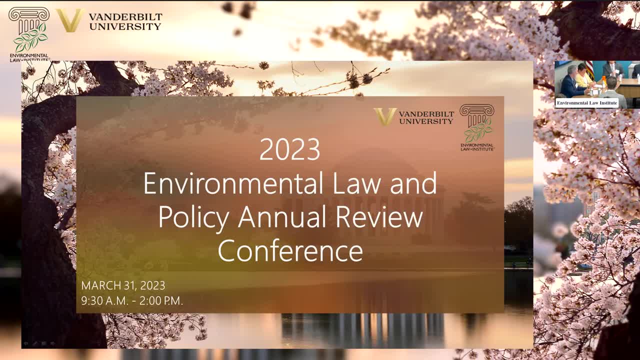 or areas right, and both need to plan and just saying you know, hey, we're going to be looking pretty good in Buffalo in 50 years. come on, do you really want millions of people showing up in buffalo's tours? and we're talking tens of millions. the Hauer study what we cite in the paper. 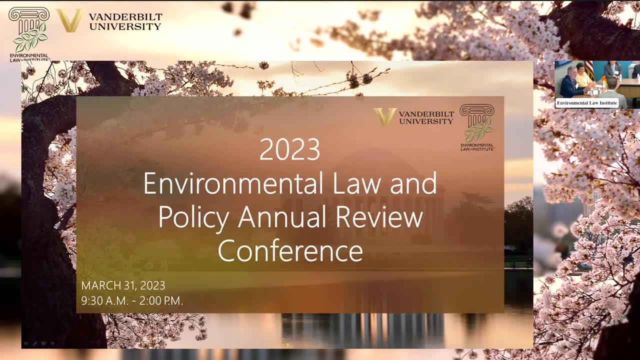 just from a few years ago. just looks at, uh, sea level rise as a as a force of mainstream decisions. that's 11 million people they project moving away from the coast, and that's not taking the drought. fly a lot biggerた. pursuit the Boynton Collider, five at one minute and then. so what are your thoughts? 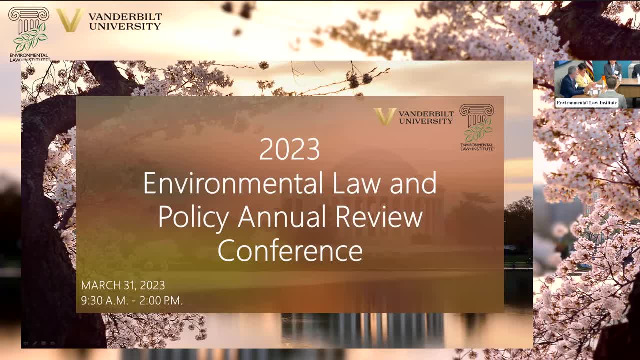 Avecwater over the 10,000etrical results. have you heard that there are a lot more instructions and drivers of migration? so we're looking at tens of millions of people in the next maybe 25, 30 years moving around, and that that can't just be chaotic, random, that we need to plan for that. so that's. 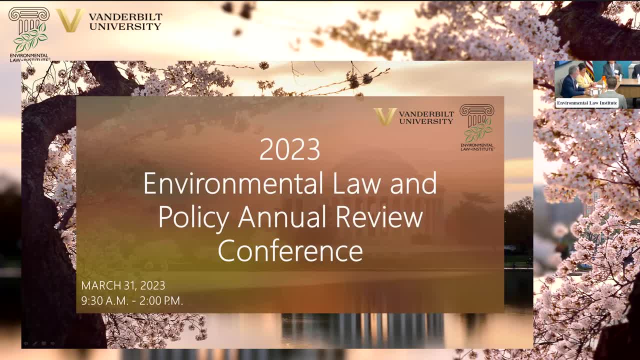 the motivation, and i think it's super hard for an outbound city to think that way, but at least this four-side agency would give that city the basis for planning ahead and understanding that we may be losing population, but we, you know how do we deal with that. but yes, i think that's. 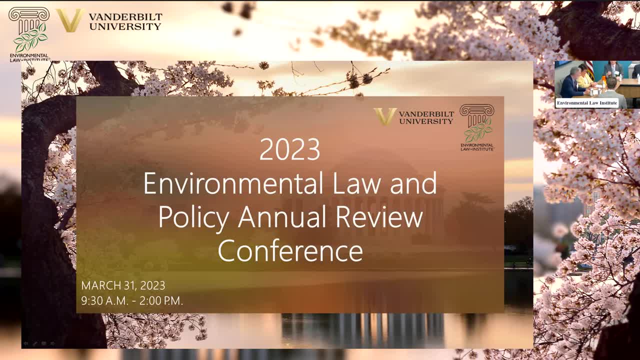 important. but, um, joel, uh, i'm very encouraged to hear about these developments. what i have to realize is, uh, we actually finished writing the minnesota law review paper in february 2021, two years ago. a lot has happened. uh, i don't think it changes the fundamentals of the paper or the thesis. 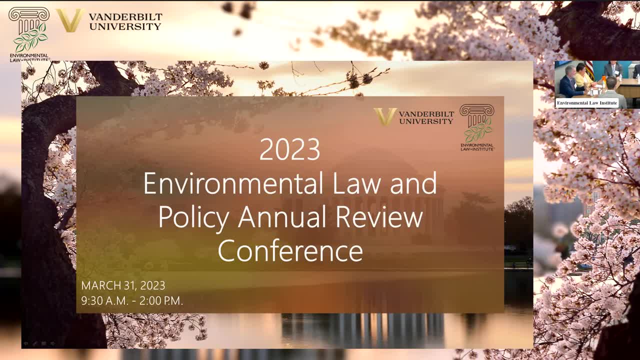 but it's great, on the one hand, to hear about what's happening and yet, as hannah points out, it's also some developments that are, you know, making it more difficult to think and implement creative uh policies. uh, rod, i love your uh, i'm going to talk. 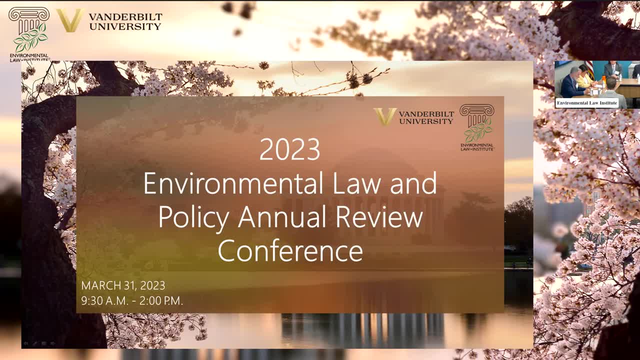 to you later about complex systems. it's a big research area of mine- but, uh, both you and hannah focus on this political reality. we anticipated that uh in our uh proposal for anticipatory governance and that's very much why we deliberately limited our really concrete proposal to a science-based 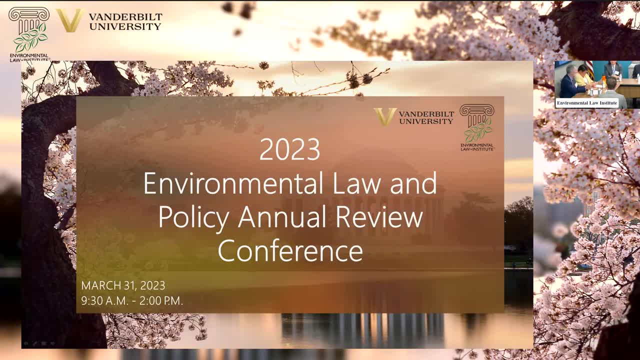 agency, kind of a usgs style non-policy, but providing the beginnings of really robust scenarios. uh, taking into account that there's no real way to predict a complex adaptive system like this, a global, complex system, but that science-based agency, maybe we could get that in without you know major. 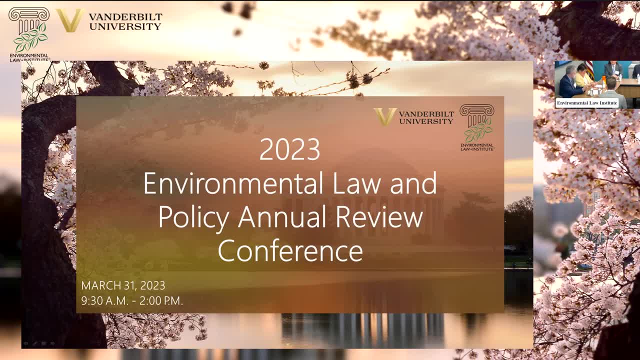 progressions, doctrine or big political divisions and get a start on anticipatory governance. uh, that would then provide the platform for that political moment. i mean they happen. the ira, you know, four years ago you said we're going to have this huge spending bill and so that's never going. 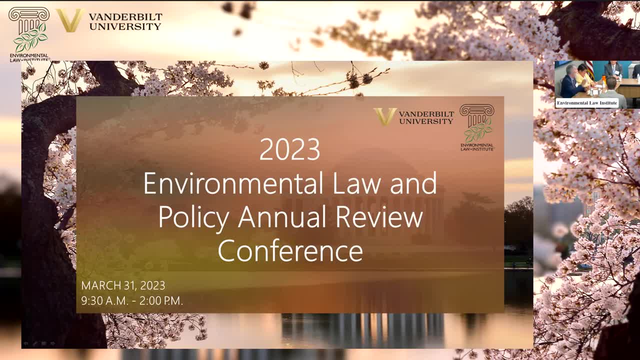 to happen. we took advantage of the political moment. we've got to get ready for that next political moment that might allow us to then implement or concrete substitute and just for governance at that national level. so fantastic comments. yeah, i, i think that's a great point and 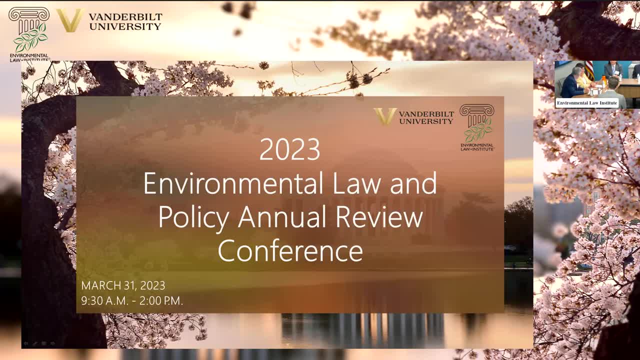 i echo jb's things. comments were fantastic. came from a lot of different directions, uh, but, um, we, we did, uh, uh, definitely recognize both politics and the law were going to be problematic. so, um, i i will let jb have the individual responses. i just wanted to take a couple minutes. 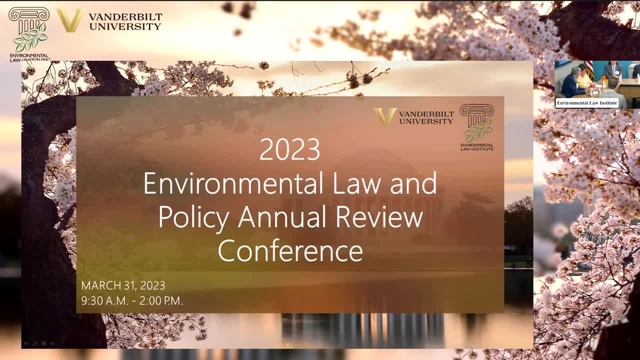 to throw out some more general responses and where i take hope from in all of this. so, um, i think, carlos, most responsive, responsive to you. one possibility of seriously thinking about a 4 degree c future, or worse, is you get serious about the mitigation and and that's one one way. 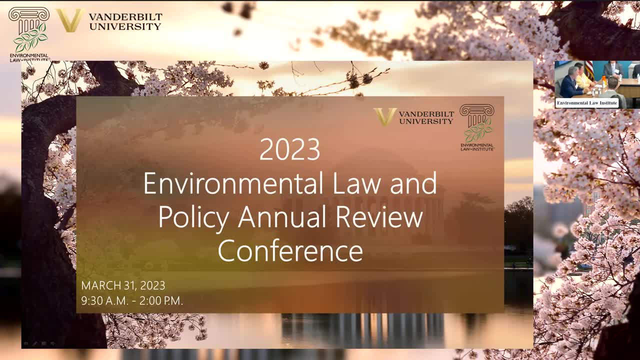 that these two, uh the decoupling, might in fact come back and reinforce efforts on on the mitigation front is if you really think about this feature- and jv and i both had days when we had to walk away from this paper for a couple weeks- i think there's a lot going on, going on right now with um. 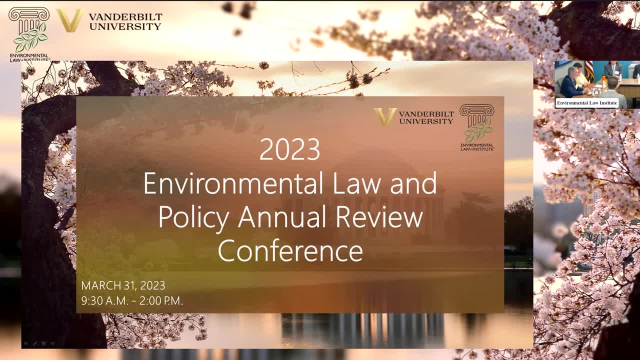 not the policy, but i mean i think the policy that would actually be for those couple hours and just you know, uh, digest, uh. but if you really really think about it, it's hard not to get serious about taking mitigation seriously. can i just add one point on that, because i totally 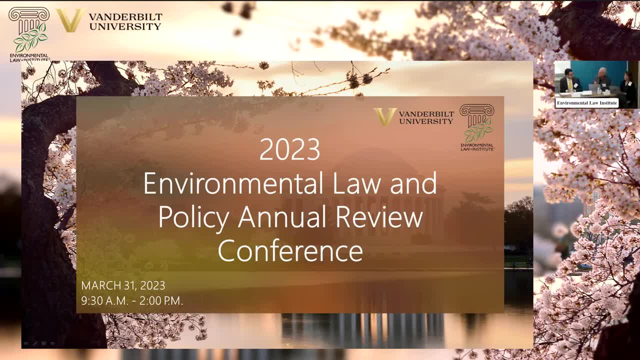 agree with you, and one of the reasons i think people early on were pushing back on thinking about adaptation is consistent with some of the research that we've done with social scientists- that if people just hear about adaptation and think it means the solution, then they become less supportive of mitigation. so it's so important to talk about adaptation in combination with 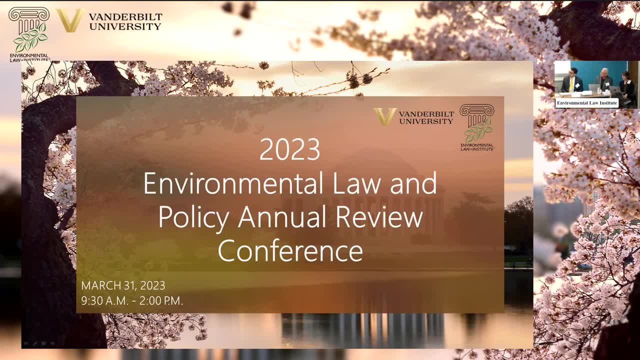 mitigation. i think your point is essential there, right? so, um, and then the the last point i'll just leave with, on a sense of hope. um, and this goes to the legal part, it goes to the politics part, it goes to why we want to be primed to do the right thing when the next moment comes. 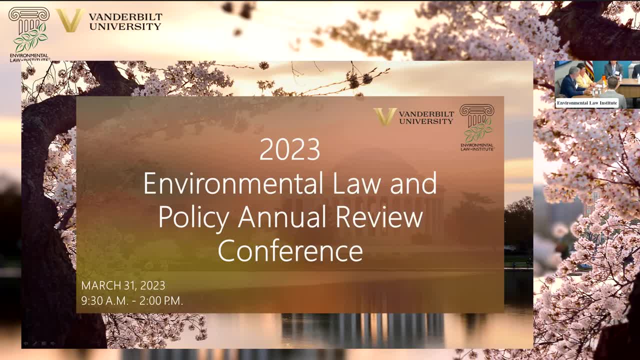 is. you know, in the background of all this, we are poised and in my humble opinion, over d4, a generational shift in who's in government. um, and i'm saying that very carefully, but i mean it hasn't transitioned the way government has normally transitioned. and when i look at my students, when i look at the people in our children, the kids in 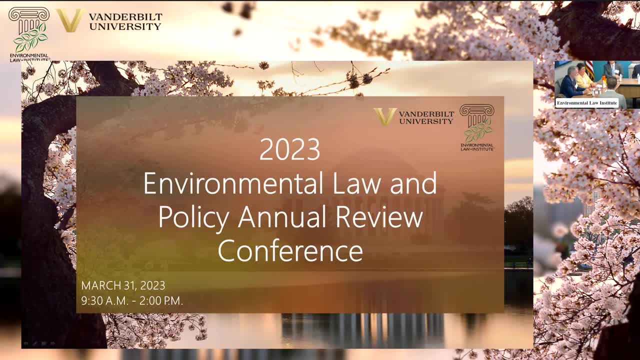 our children's trust. uh, what they are accomplishing, uh, in europe. uh, what they are trying to accomplish in the united states. if you read, uh, the district court opinion in the giuliana case, if you read the dissent in the giuliana case, there are judges who get it and there's a generation that's about to take over that. 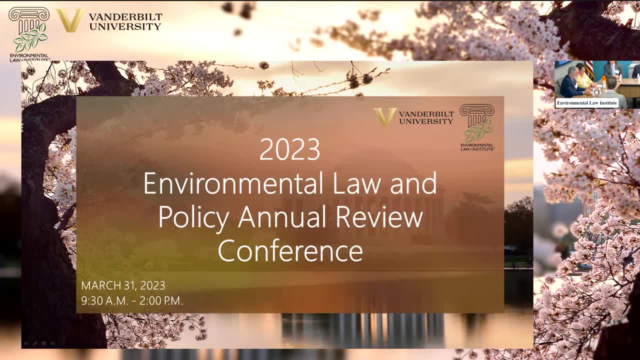 gets it, and the sooner they come into power, the better off we're all gonna be. so, um, that's that's where i take a lot of hope and and that's where i see that moment coming. is we're like: so we're about to have a profound generational shift. 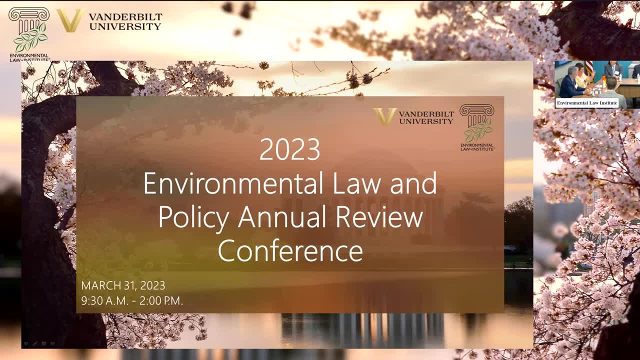 in governance and it's going to skip a couple jen, it's going to skip me, um, but that's fine, uh, but um, you know, i think that that's all. there's a lot, a lot to be ready for anticipating that, and the more, uh, the more we've thought it through, the more that we have this foresight that can say okay. 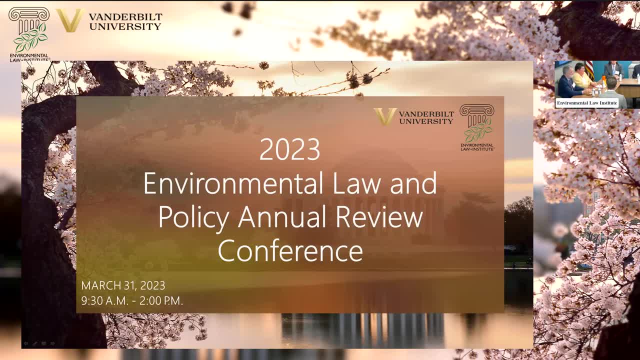 you're ready here, here's what you need to think about. uh, i think there's room to be hopeful there. so i think that's the first question to the panel, yeah, and then we'll go to the audience. uh, so, uh, professors, um, as anna vizcarra mentioned, uh, with the administrative state's scope. 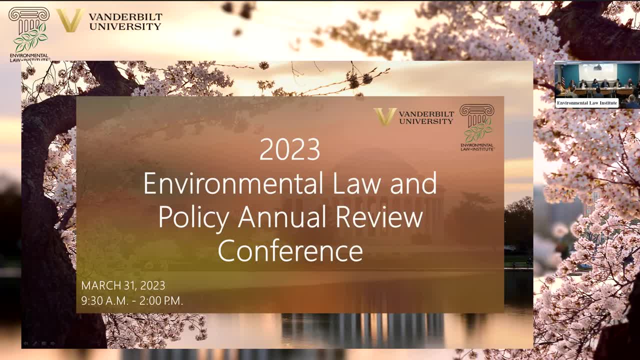 significantly curtailed by precedent, like west virginia, vpa and uh with congressional gridlock, rendering um most decisive legislative action uh difficult, although we did hear about some progress uh on that front. um, how would your proposed um new national foresight bureau reliably sort of ensure that all this um 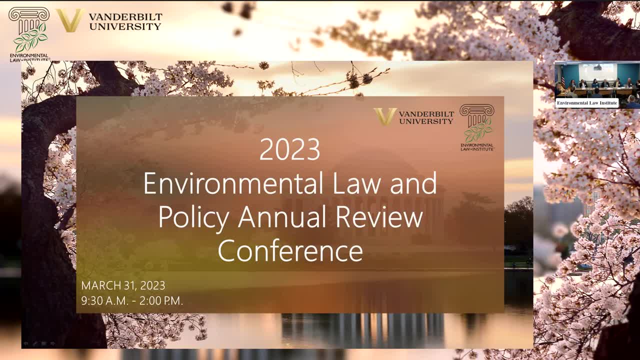 this data is translated into actual actions sort of at the state and local levels. now we heard about sort of new uh advances, mostly in the inflation reduction act and the infrastructure bill. a lot of that seems limited to these sort of subsidy programs and sort of beneficiary pays uh programs, which seem to be the only things that. 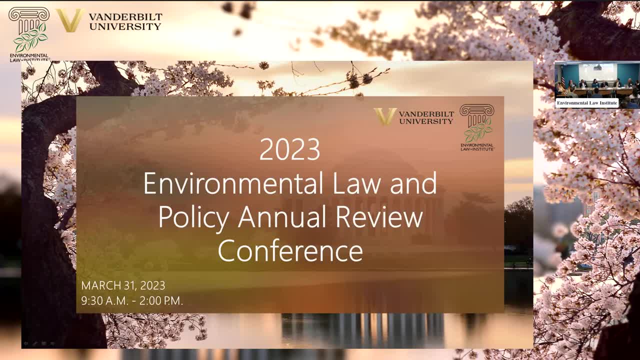 are getting through congress right now. um is that sort of enough to implement that? or you know what's. what are the options going forward to prevent the sort of underscoping of risk and to address the, the fundamental um change that we need, that doctors can look for addressed? 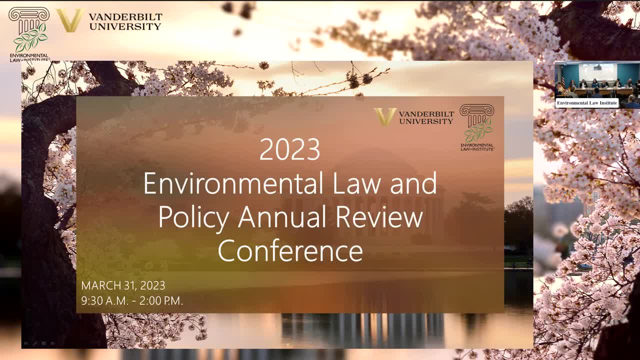 i'll just start by saying: if there is no political will, there's no political will. um, and emphasize again, the point of our recommendation is to have the information ready to go when, when there is political will to put it in place. uh, but that said, um again, we do see change when major events happen, and as this becomes, 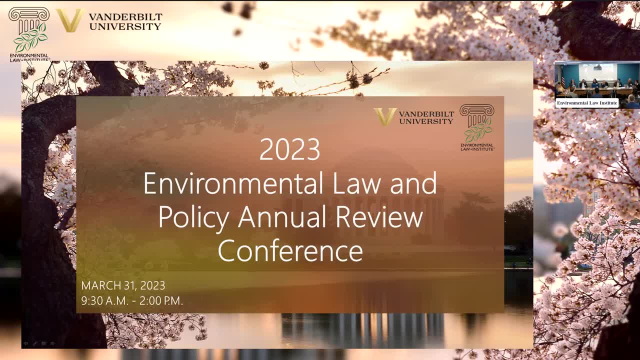 more and more of reality. um, you know, i'm at the end of the colorado river. if you don't think, that's not a daily discussion in los angeles, uh, about what that means for the future of los angeles, uh, it really is. and and um, you know, phoenix has gotten. 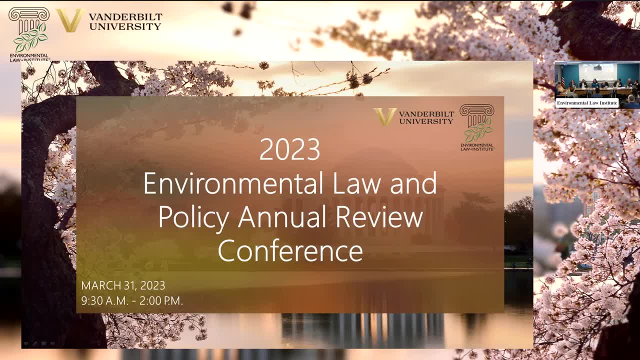 record days where planes can't take off or land because it's too hot. uh, you know those kinds of things when they start. we're having a really weird winter this year. i mean, how many weird winters do you have to say where it's like, okay, we're just going to be normal? um, uh, but you. 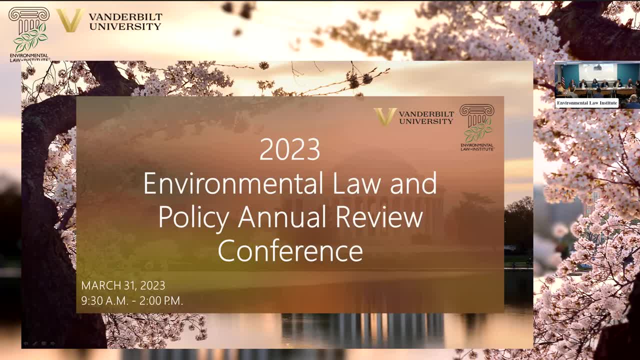 know, eventually people do have to respond and we, um, you know, on the administrative law front, jp and i made this point in a different article- we wrote together: uh, we made up administrative law the first time we can make it up again. they could do what we uh needed to do. it's not, you know. 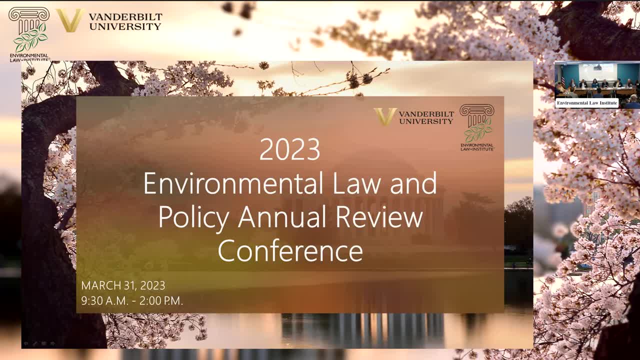 uh, it's not written on tablets and it can't be done. it's not written on a tablet, it can't be done, it can't be changed. law is a human institution. it serves human ends. uh, and when we need it to change, we have been more than willing to change it. so, yeah, uh, and like i said, that's just a matter. 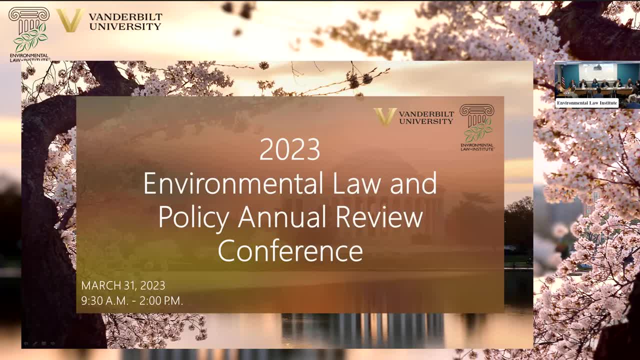 of getting everything lined up so that when the political moment is there, it can get done. you know i'm going to give a chance for any of the panelists. this is an incredible panel. does anyone want to just follow up on anything they heard from other panelists? um or responses. 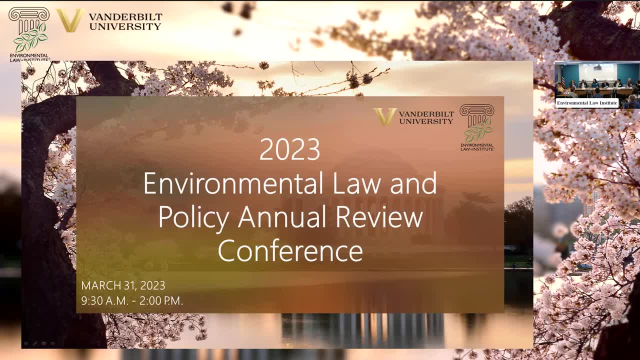 from the audience and then we'll get to the question, i guess. i guess i'll speak to focusing on like seriously getting to mitigation and adaptation. i don't know if that means because we're just trying to do both, um, but so is the whole country with an ira. that's a good start, but we need a whole bunch of money. 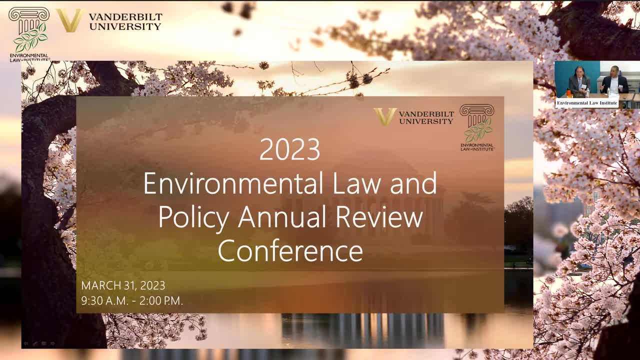 on both sides and we haven't really talked about equity. like, how do you, how do you really focus on equity in the right way? um, you know, does that mean, you know, you know, The city of Dallas gets favored now versus other cities on the Gulf Coast? 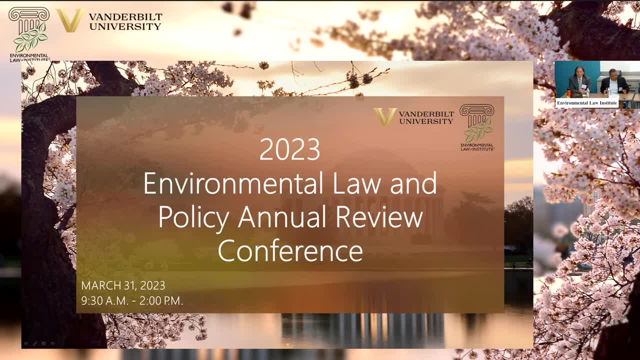 Are we choosing winners and losers with the federal funds now so that in 20 to 30 years the cities of Dallas could be more resilient and accept, you know, the domestic migrants? I mean, that's a tough political call. You know, there's an interesting comment from a webinar participant that says: I feel the mantra should be climate change adaptation, mitigation and resilience. 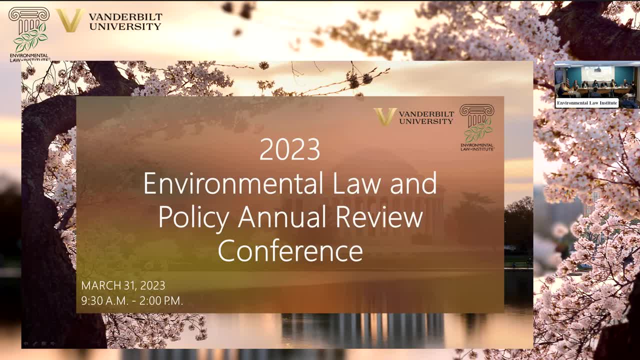 The resilience planning and policy and governance is advancing farther and faster than the first two. Any, yeah, Rod, Yeah, real quick, just in terms of the politics at the moment, I actually think it's unfair to saddle, you know, the authors and the paper on that particular point. 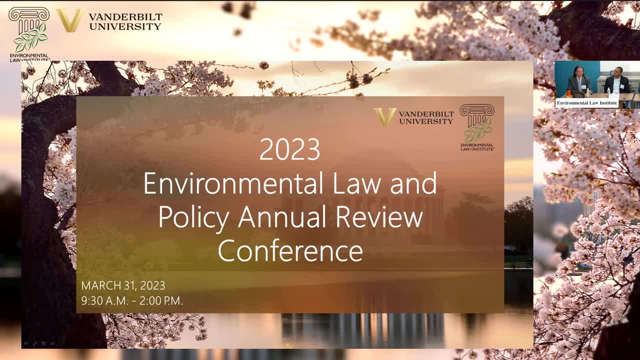 Because that is somewhat out of the control of you know, there's a different force going on here, But I do think it's important to identify two things, And one is when you assess risk and when you scope risk, that information itself as an element of risk, which the intelligence community that I was a part of had a hell of a time dealing with. 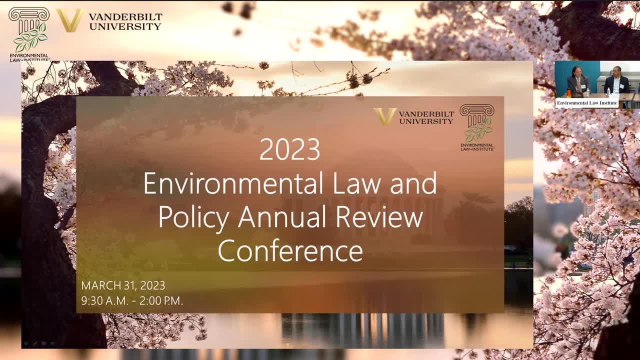 And one is when you assess risk and when you scope risk, that information itself as an element of risk, which the intelligence community that I was a part of had a hell of a time dealing with, But it is a significant piece of governance, It's a significant piece of risk. 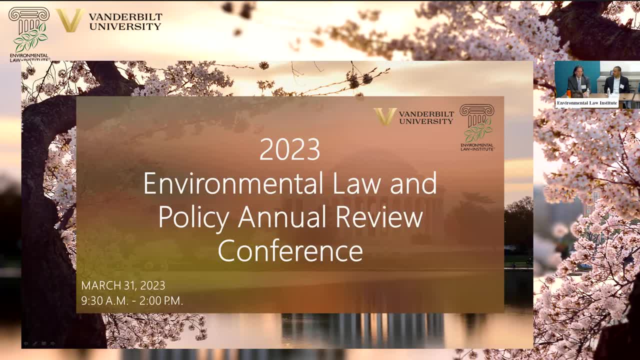 And we our legal structures. I'm a lowly physicist so I hesitate to talk about legal structures, but it seems like we don't have many levers at all to address the information integrity question. And second, it's about what we're talking about, which is the basis of the global system. And so I think that's a question that I'm going to be asking, and I think that's a question that I'm going to be asking, and I think that's a question that I'm going to be asking, and I think that's a question that I'm going to be asking. 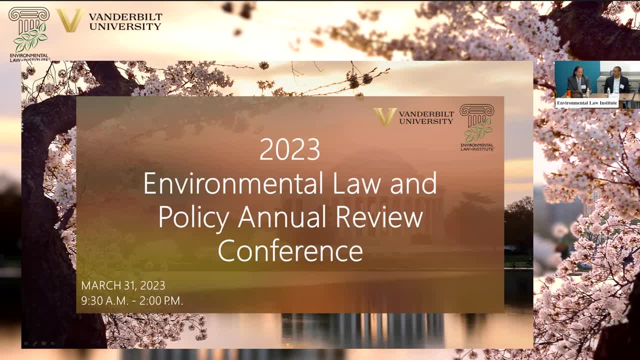 scoping risk in the national foresight bureau, um which you know i had when i was inside a government. i argued for such capabilities that were domestically focused. um, i think one thing that we have to be very uh thoughtful about is how we scope risk there as well, and, historically, 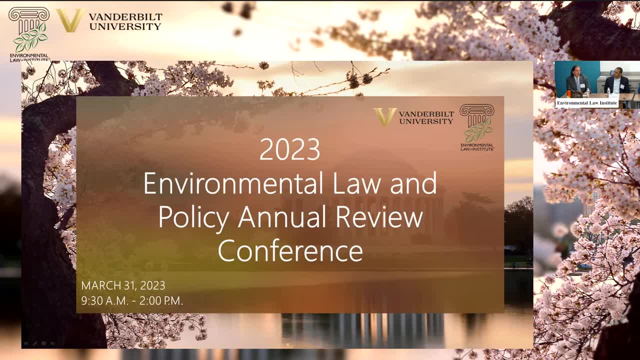 the way that we talk about the impacts of climate change and if you just start rattle off the things uh that you know- storms, heat waves, sea level rise- are you actually capturing the risk of climate change when you go through an especially abiotic, uh meteorological list of stressors, when the 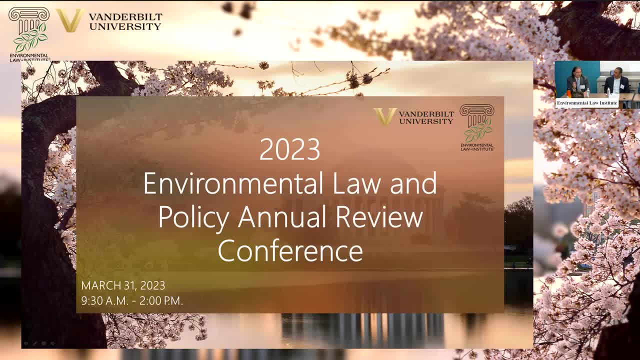 temperature of the planet is changing. it's no longer an environmental issue. this is a planetary control issue, right? anything that's temperature dependent has the ability to be moved right, and that's every chemical, biological, ecological, industrial, agricultural process. it's it. it moves beyond weather, right, and so it might be that the most 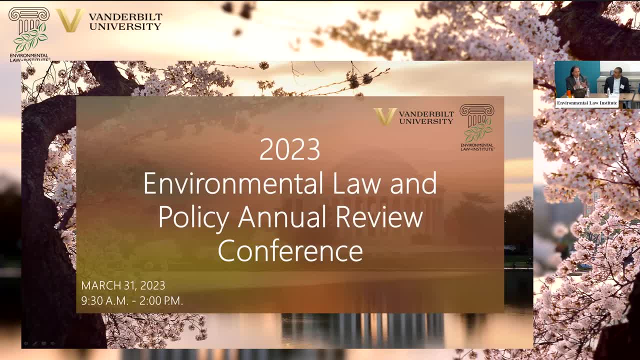 important stresses that come about from climate change are infectious disease patterns and uh, antibiotic resistance, uh and uh production. right, and so you know. historically, many communities have started with sea level rise and in storms, but we know a lot more than we used to and we can assess risk a lot better than we used to. there's a paper just shortly. there's a. 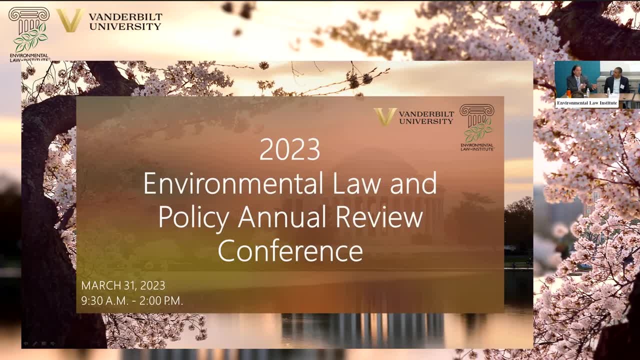 paper, uh, that came out two years ago in nature, climate change, where the authors identified 467 pathways by which climate change affects people. right, and so when we look at a few of those, we're not seeing the entire story. i do, um, i do think on the legal and political question. i think it's important to to some extent. 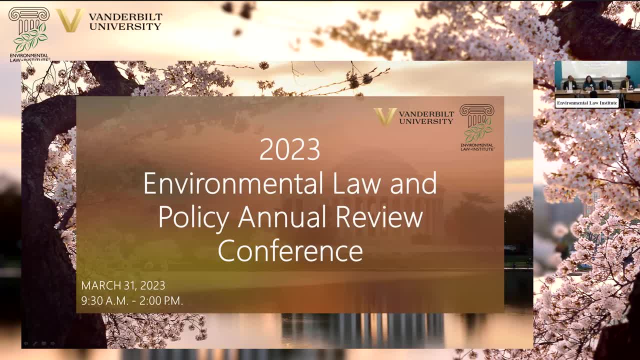 decouple those. you know- robin talked about new generations- and, and you know, very motivated folks looking at this in a different way. the political will can shift relatively quickly, um, and even even with you know the the realities of where administrative law came from and where it could go. 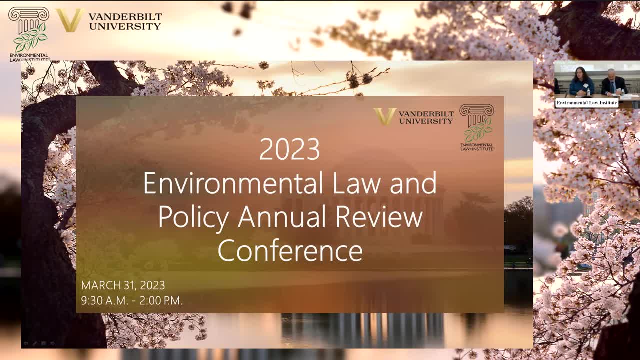 uh, i think we're in a moment where we shouldn't lose sight of the fact that we're in a moment where decisions being made now in legal jurisprudence can significantly slow down these potential. these potential, you know adaptive governance approaches and so you know, i view that as 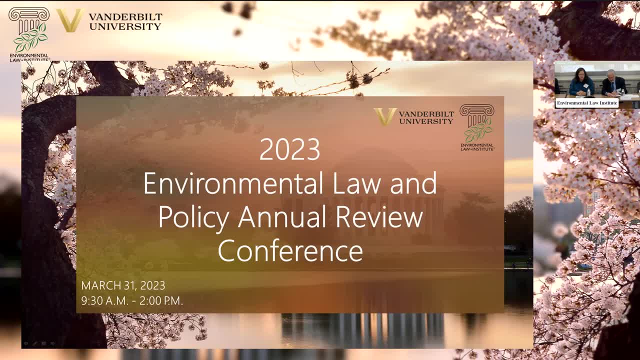 a real call to action for lawyers to make sure that they're engaged with these fights, that we're limiting the damage there so that we can quickly move forward when necessary. um, because Even if the political movement is headed one way that may be different than the current moment, you will still have these legal decisions on the books, judges in place that are following them and that will outlast the broader political structure and feeling. 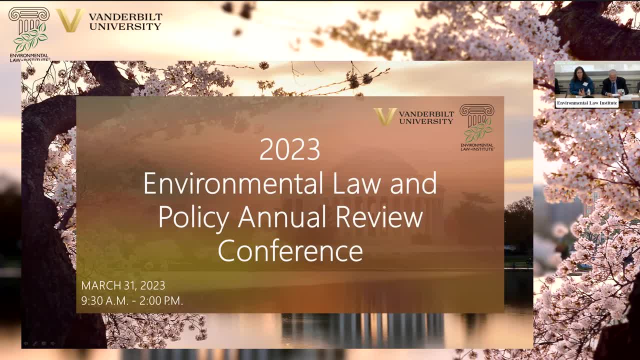 And so we have to, we have to grapple with it, We have to limit the impact to the extent we can and figure out new ways to address the legal issues and work with Congress to do so when necessary. So I just want to sort of emphasize that I see this as two sort of parallel structures, also parallel, also sort of separate from the identification of the need and the problem sets, which you know is incredibly important as lawyers, not 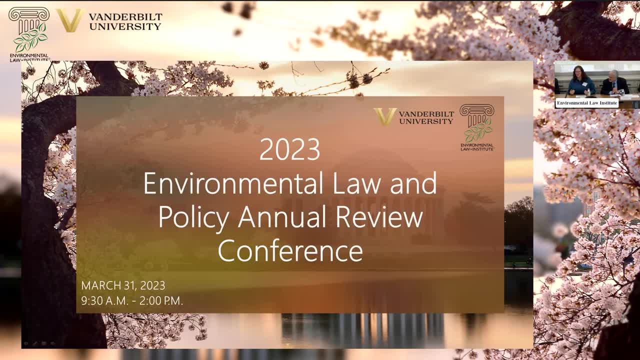 physicists, not, you know, scientists. we need somebody else to tell us what those are so that we can start thinking about those legal structures and how we address them. Yeah, while we're on that track, let me put a third pathway on the table, which is the Environmental Defense Fund. thinks about private governance as proof of concept. 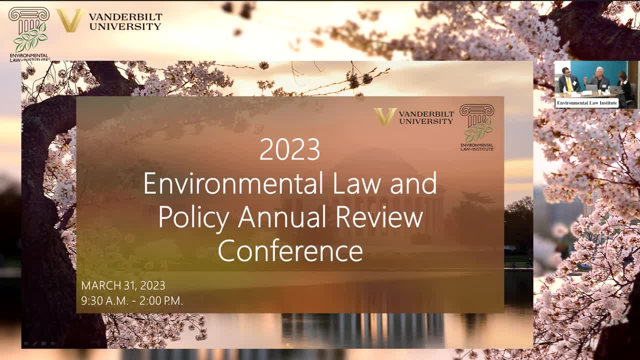 And one thought: you all did a really nice job. I think of noting that possibility and then saying you're going to dive into public. One thought would be: we get Vanderbilt, we get USC, maybe we get a major foundation and we start actually building the organization. 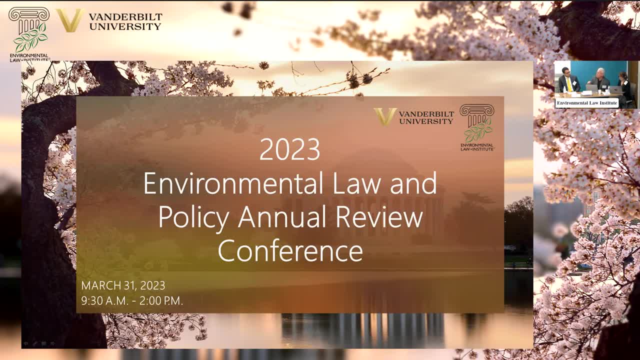 and the organization And the plan that you're talking about for the time when the political system is ready to bring it in, so that we have something up and running that can begin to do what you're talking about. And let me just say that, lastly, I've been working with physicists for 20 years in the academy. I've never heard one put the word lowly before the physicists. 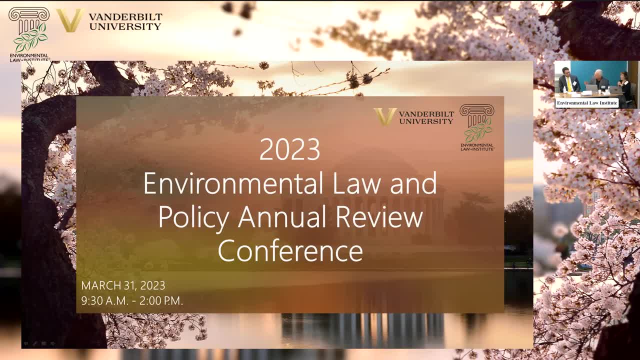 I just want to say we've got a remarkable panel here, remarkably modest given their talents We do, and I think we needed another hour, clearly, but we need to wrap up. So what I'm going to suggest- because the people in the room did not get to ask questions- if you all wouldn't mind hanging out maybe in that corner for the next five, 10 minutes and answering questions- we'll set this up while you guys are doing that. we'd appreciate it. So we're going to take a 10 minute break. we're going to get back on time because of our webinar is in process. 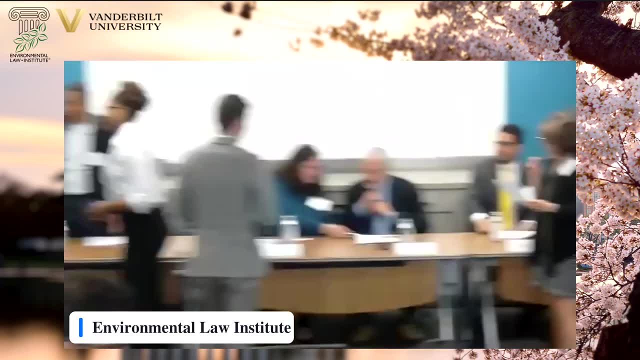 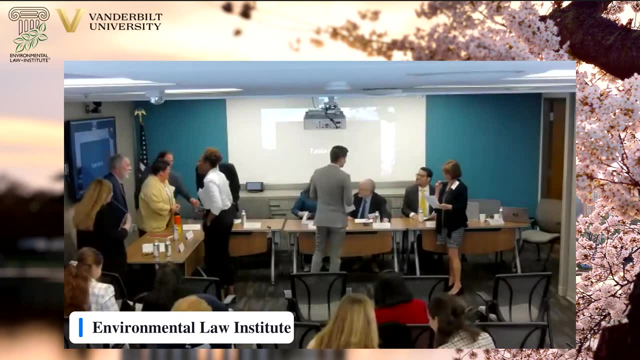 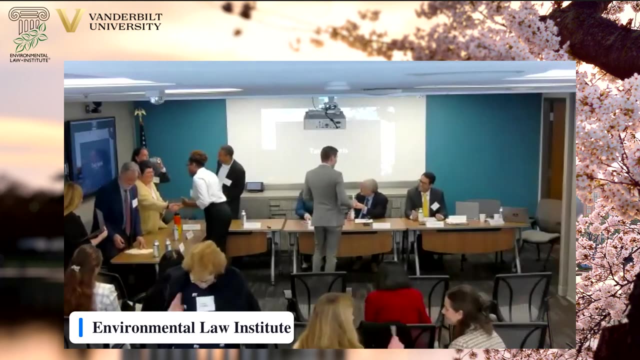 Webinar participants. the feed is live throughout. we can't turn it off, so you may want to mute your sound for the next 10 minutes and turn it back on when we start. Great piece. I'm going to go back. Yeah, looking forward to being back. 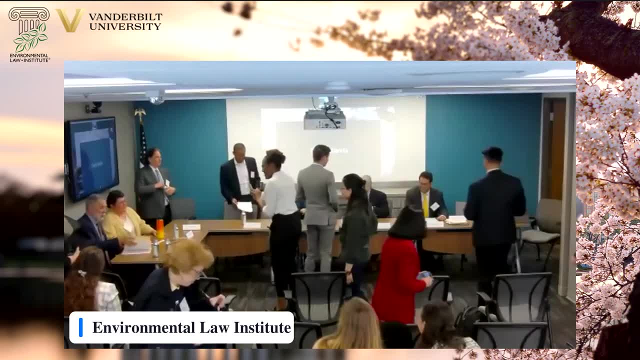 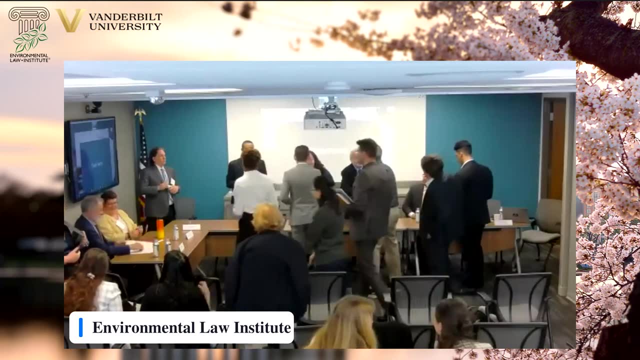 Yeah, Yes, All the time. He's the one I'm the winner. Yeah, Yeah, Yeah, Yeah, Yeah, Yeah, He's a good man. Hi, Oh, my name is Aiden Aiden. I haven't seen you in a very long time. 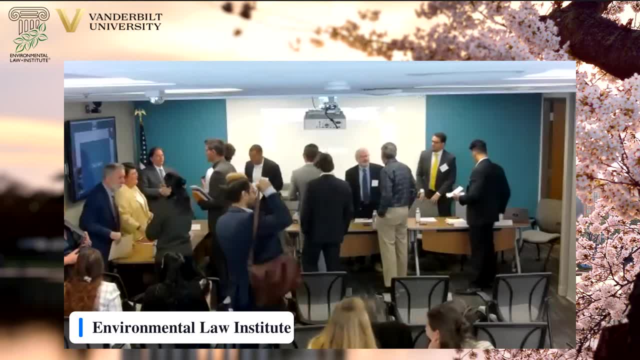 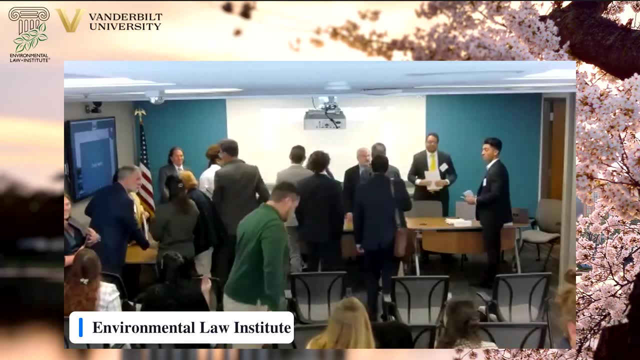 We met at Georgetown Law at the moment and your experience in particular. I thought there was a lot of discussion. We seem to catch up sometimes. I think we're going to have to figure it out, the kind of jurisprudential barriers that are getting to you, and now they're going to allow us to make that happen. 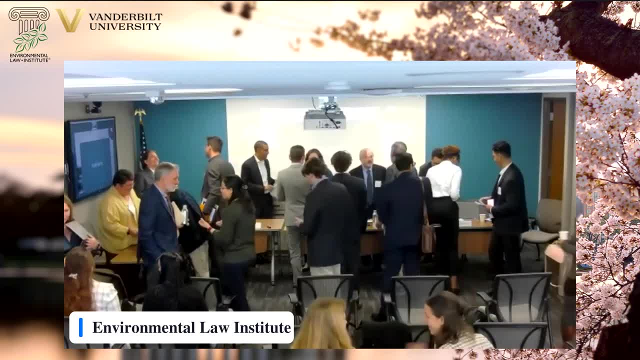 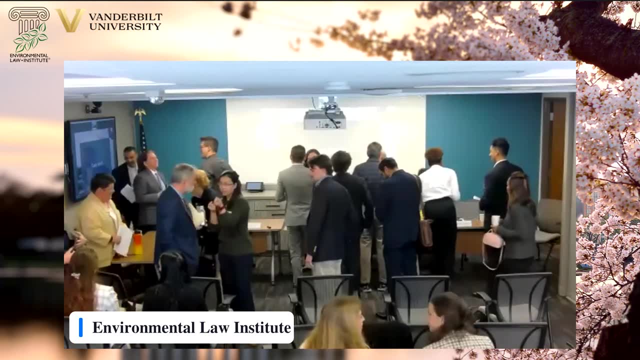 That's what I really wanted to talk about. Thank you, Thank you. Yes, there we go. Oh my gosh, that's great, Great, Thank you. All right, I thought we had time. Thank you, Thank you. 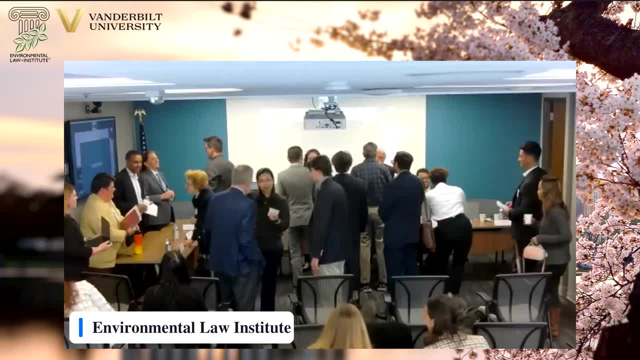 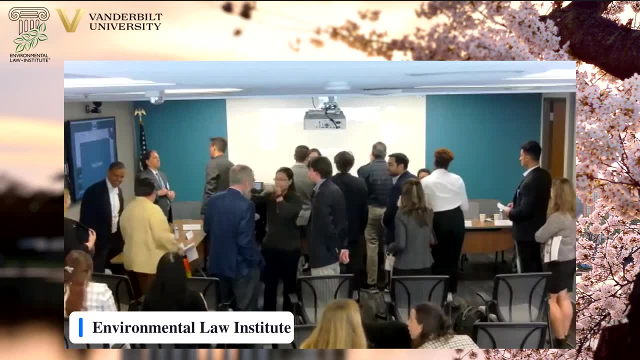 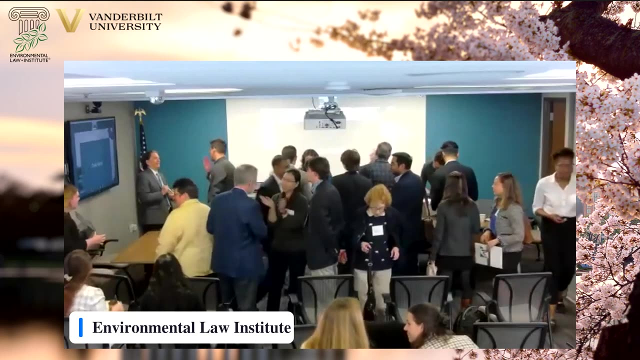 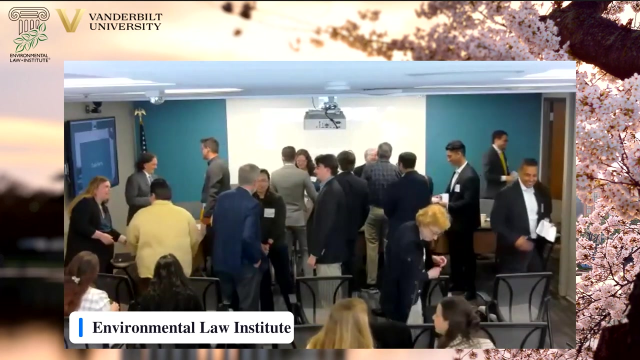 All right, Mike, how are you? Thank you, Thank you. So we have gotten a couple of letters in the chat which kind of gave us a bit of a big jump. This is Michael, So thank you, Go ahead, James. 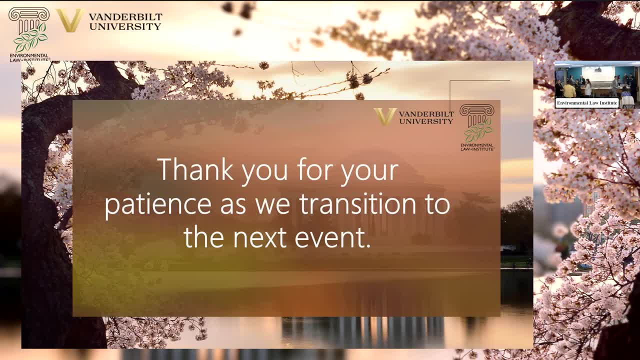 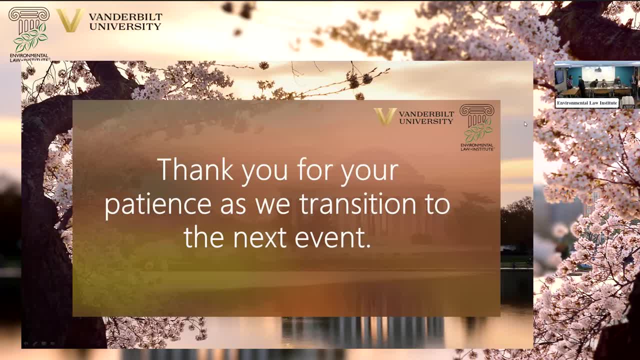 We make sure. Yeah, there we go, Finish, Finish. Okay, wow, That's. that's part of your soliloquy that I was going to try and put in your hands. I had a chat, GPT, write some comments for me. 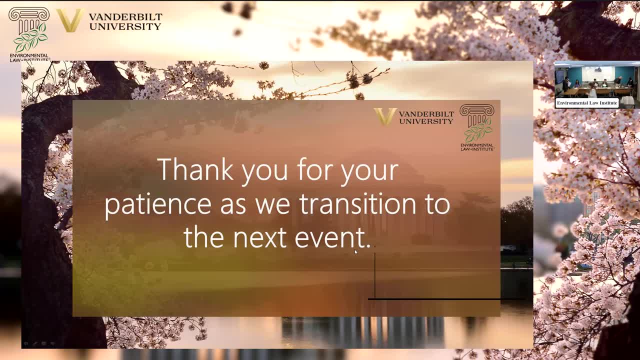 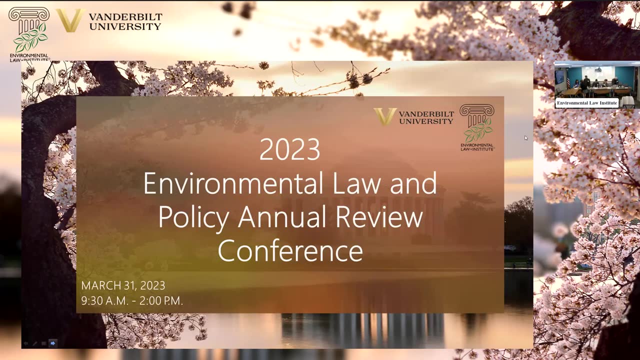 Because the last week or two I've been like everything that I was thinking like I know rendered irrelevant as humans, and everything I've been thinking Welcome back. All right, everyone, Welcome back. I'm Linda Bragan. I'm with the Environmental Law Institute. for those of you who are just joining us on the webinar or here in person, 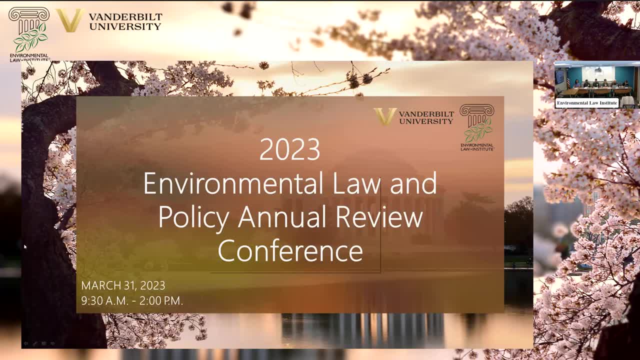 And we are going to get started, But I want to remind the webinar folks that you should put questions or problems about technology in the chat And you should put your questions for the panel in the question box. And if you're having any trouble getting your questions in the chat box, 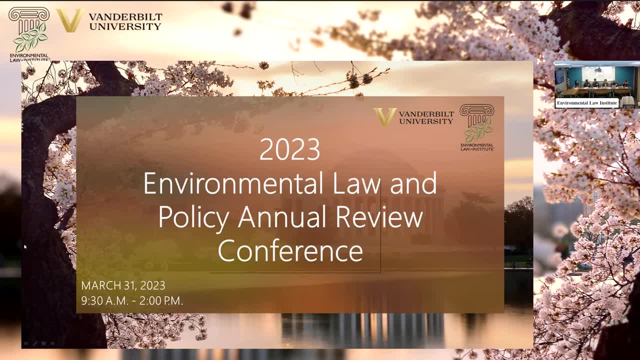 And if you're having any trouble getting the screens to work, there are instructions in the chat, because you should have your speakers front and center, not the placeholder screen, as you're watching the webinars. So we're going to go as fast as we can. 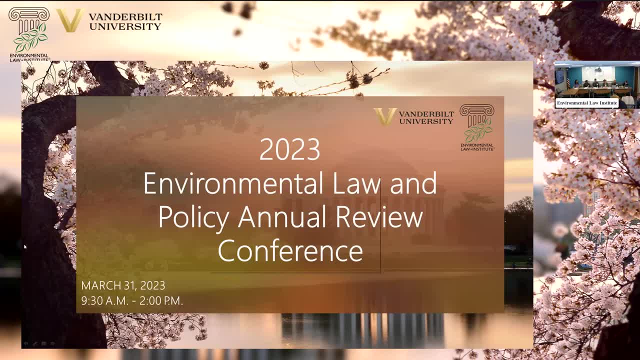 And we may go a little bit over, because we started a little bit late And I want to make sure we do have time for questions. So I want to start by introducing third year law student Tosia Harris, who is on remotely with us today. 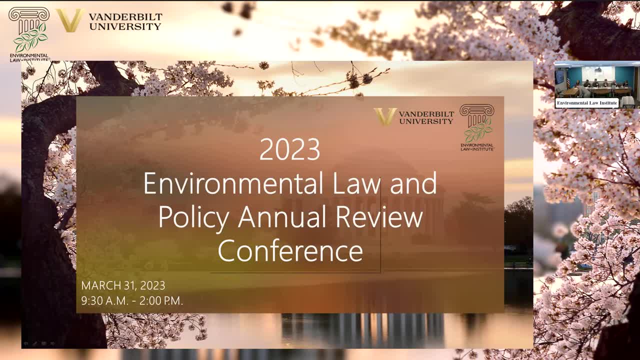 She was the article editor. She's from Vanderbilt Law School for this article And I am going to hand it over to Tosia to introduce our panel. Thanks, Professor Bragan. As Professor Bragan has said, my name is Tosia Harris and I'm a third year law student and LPART article editor. 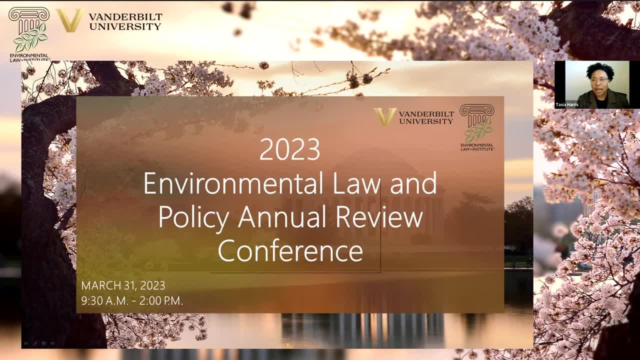 I'm excited to facilitate this panel discussion of the article How Algorithm-Assisted Decision-Making is Influencing Environmental Law and Climate Adaptation by Sonia Jaya. Sonia Jaya is a professor at the University of Minnesota. at the University of Minnesota, Sonia Jaya is an assistant professor at the University of Baltimore School of Law and external research affiliate of the Environment and Democracy Group of Central European University's Democracy Institute. 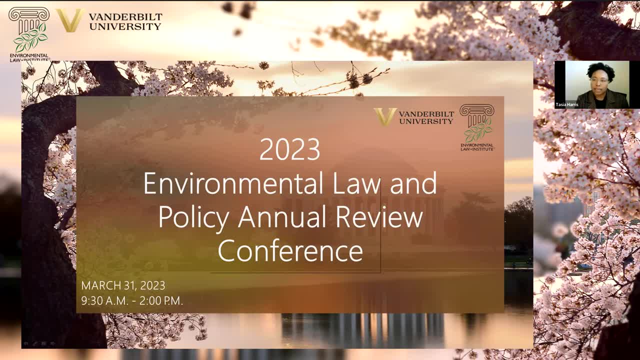 Sonia Jaya's research interests focus on the overlapping areas of environmental governance, environmental law, technology and society, Asking how environmental law and institutions can sustainably adjust to rapidly changing biogeophysical conditions And societal demands associated with climate change, And what the consequences are for equity and democratic participation. 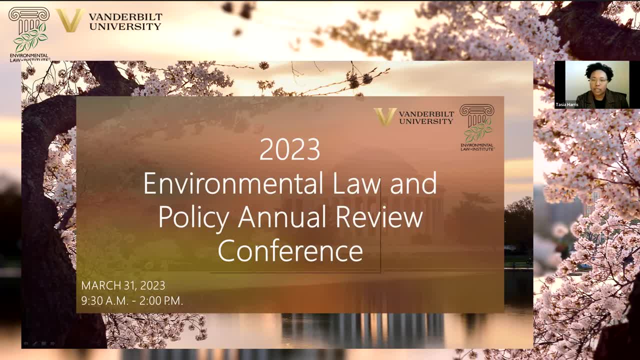 Her approach to these questions draws on her interdisciplinary background in geography, water policy and law, as well as her practical knowledge of energy regulation. Before University of Baltimore Law, she worked in energy regulation at the California Public Utilities Commission And was the research lead for the Water, Energy, Climate and Sustainable Development Committee. 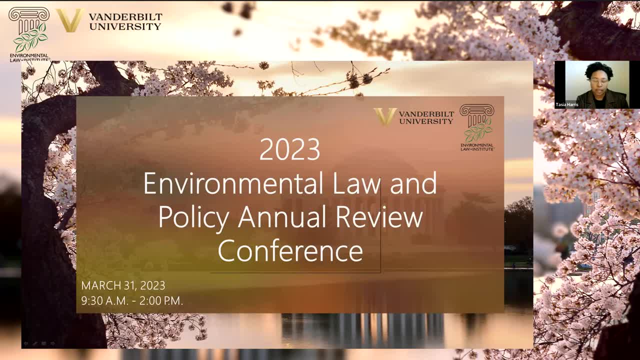 And is the research lead for the Water Energy, Climate and Sustainable Development Committee. And was the research lead for the Water Energy, Climate and Sustainable Development Committee At the California Energy Commission. Jaya holds a PhD in geography from the University of Arizona. 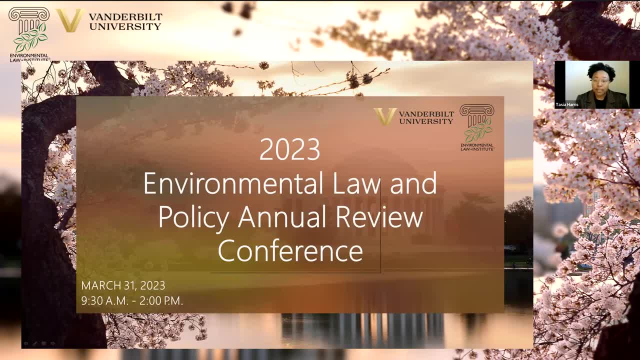 A master of science in water science policy and management from the University of Oxford And a JD from UC Law, San Francisco. Joining Professor Jaya is panelist Keith Dennis, Senior fellow at the US Department of Energy. Keith is an expert in energy and climate policy. 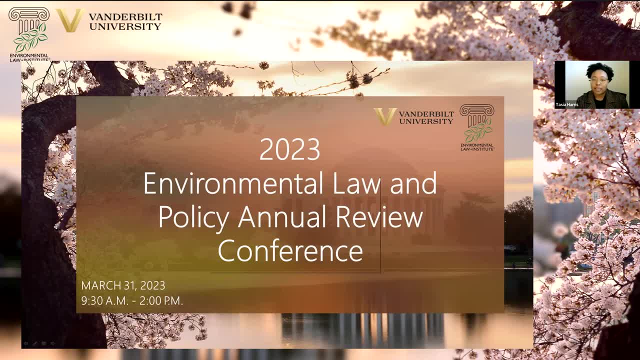 Nipah and international law. He has experience advising and litigating multi-billion dollar infrastructure projects, negotiating in dozens of international environmental agreements, including the Paris Climate Agreement, and developing net zero energy housing. Keith holds a JD from Georgetown University, an LLM from the London School of Economics and Political Science and a BS in. 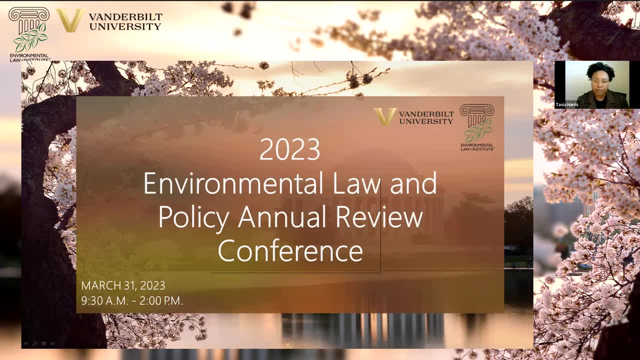 communications from the University of Nebraska-Lincoln. We are also joined by panelist Mohit Chhabra, technical lead and advisor for climate and clean energy at the Natural Resources Defense Council. Mohit provides analysis and strategic guidance to policymakers and other stakeholders at the state, regional and national levels. He is currently working on redesigning. 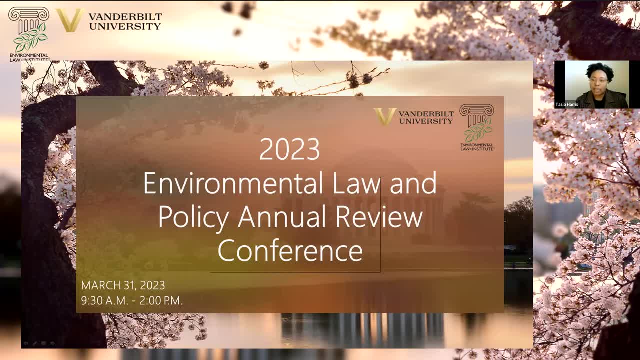 electricity pricing to facilitate decarbonization and enhance affordability, developing cost effective pathways to reduce greenhouse gas emissions and pollution from California's energy sector. and serving as a technical advisor to other regional teams. He holds a master's in civil, environmental and architectural engineering from the University of Colorado, Boulder, and a 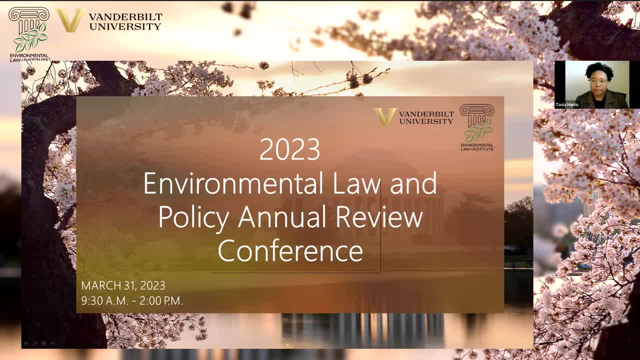 bachelor's in mechanical engineering from the University of Pune in India. Lastly, we are joined by panelist Debra Gorman, president and CEO of the Greenlining Institute. Debra has over 25 years of experience in nonprofit and private research universities and over 10 years of private sector. 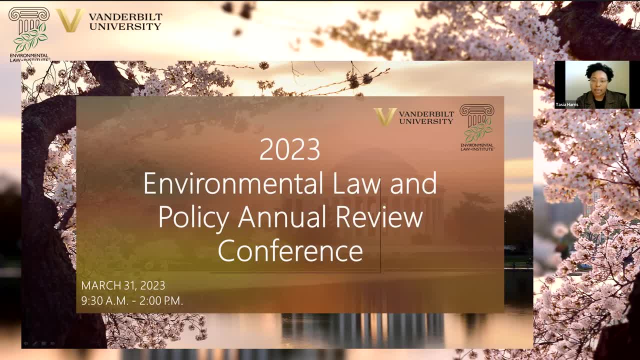 business development expertise. having worked in investment banking, international infrastructure development and engineering. She currently serves on several advisory boards, including: the Federal Reserve Bank of San Francisco Community Advisory Council as a 2023 chair. the California Organized Investment Network, which serves as a national model to provide leadership in increasing 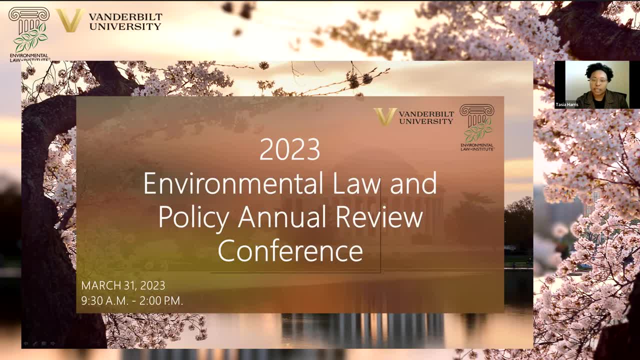 insurance and the California Organized Investment Network, which serves as a national model to provide leadership in increasing insurance industry investment and understored rural communities throughout California, and the nonprofit insurance alliance board of directors. Debra received her BS in management sciences and her MBA in finance from Stanford University. Thanks, Going back, to Professor. 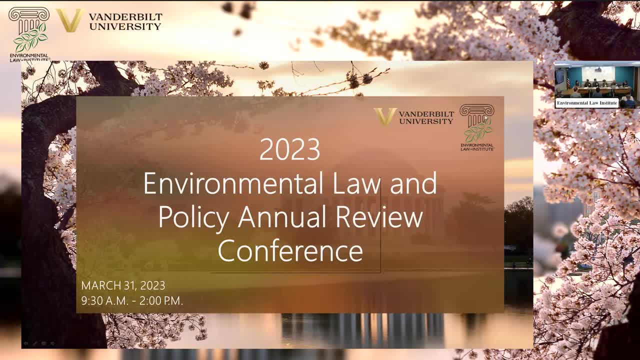 Britton- Great. Thank you so much, Tatia, for being with us remotely and we are going to kick it off. Sonia, tell us about your article. Great, thank you, I'm delighted to be here. There should be. 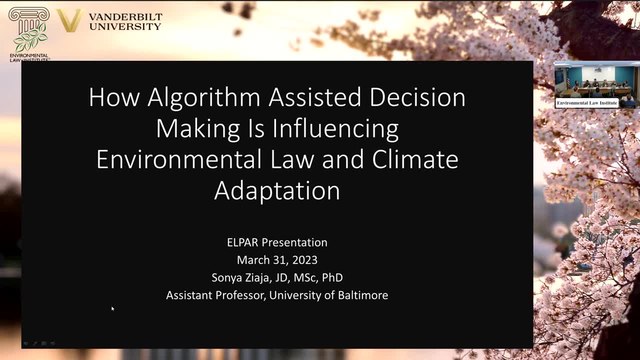 slides. i think, yep, great, otherwise would be really different presentation. um, i want to first thank uh the environmental law institute and vanderbilt. i'm so glad to be here to share my paper and i'm honored to be uh among your panelists. so thank you so much. um, so a lot's happened since. 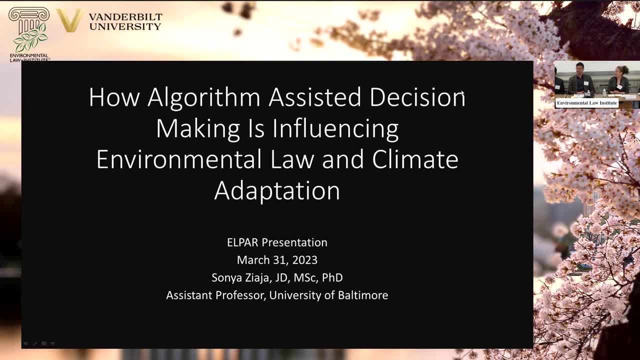 i wrote this article and we'll get into that a little bit. i'll try to keep this pretty short, so next slide, please. thank you. so the takeaway first, uh, on the next slide- is that algorithm, algorithmic tools, are really just forum for environmental decision making in the first panel. 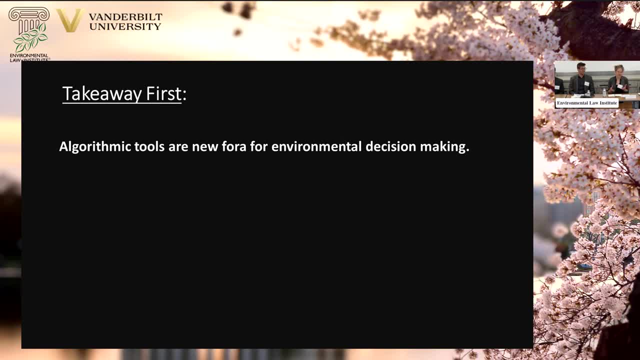 we talked a little bit- or rather, the panelists talked a lot, uh, about the kinds of tools that we need for climate adaptation, and we're thinking about those as kind of like, yeah, tools that they fit into democratic processes, and then there's kind of an output: what my paper is. 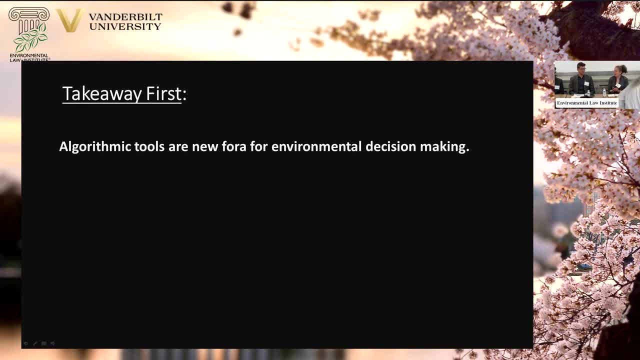 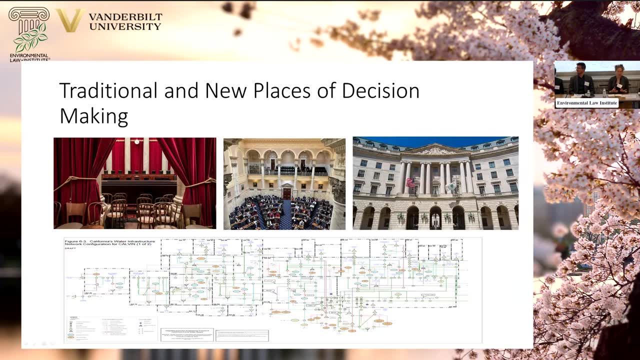 really challenging is that idea that these are something separate. uh, so i'll go through this argument. next slide, please. so when we think about forum for decision making, we're used to thinking about like legislatures, maybe courts, if you're a lawyer, uh- and administrative agencies. but when you 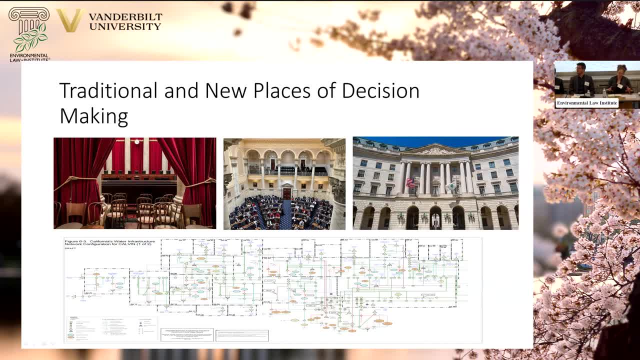 see at the bottom of the slide is a schematic uh of an optimization model and how that views the water system in california, and i'm suggesting that this is also a forum where we can kind of start to think about this and understand it in a more participatory way. next slide, please. 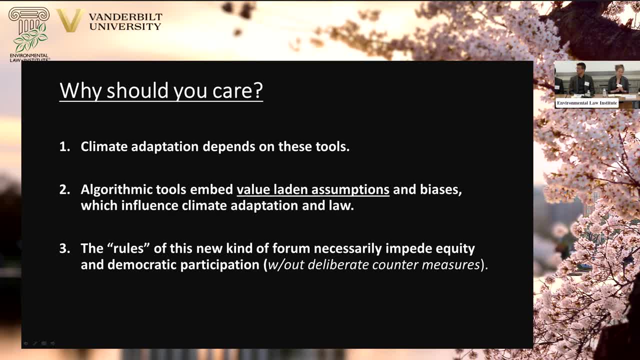 so why should you care about this? first, climate adaptation absolutely depends on these tools. secondly, algorithmic tools embed value-laden assumptions and biases which influence climate adaptation and law. and the third reason is that the rules of this new kind of forum necessarily impede equity and democratic participation without deliberate countermeasures. 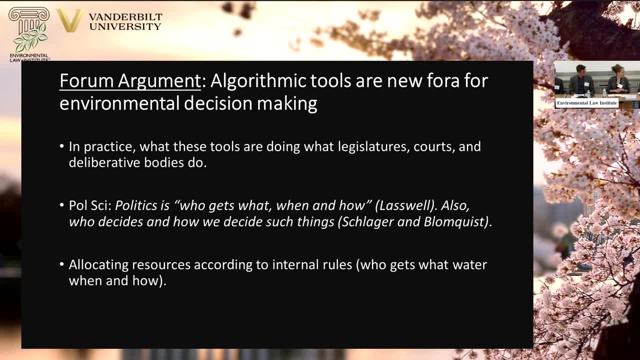 next slide, to the extent you can speak loudly for the problem. no, and i'm sorry, but it's, you know, one of these complicated hybrid things. but you know, the microphone is going to the webinar feed. it's not amplifying right now and so, to the extent you can- i don't right- i'm going to try to treat you guys. 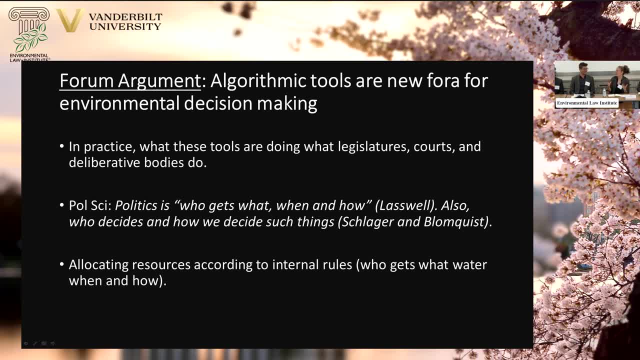 like one else in the room. yeah, my apologies if you can't totally hear me, but i will do my best. thank you so much, linda. all right, so here's the forum argument. uh, in practice, what these tools are doing is what legislatures, courts and deliberative bodies do. so from political science we know that. 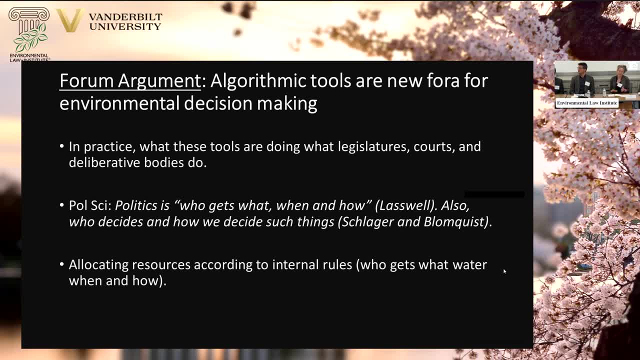 politics is who gets what, when and how, and it's also who decides and how we decide such things. so what these tools are doing are really allocating resources right. these are mostly optimization models that i was looking at, but there's also other kinds as well. um, according to internal rules. so who gets what, when and how? next slide. 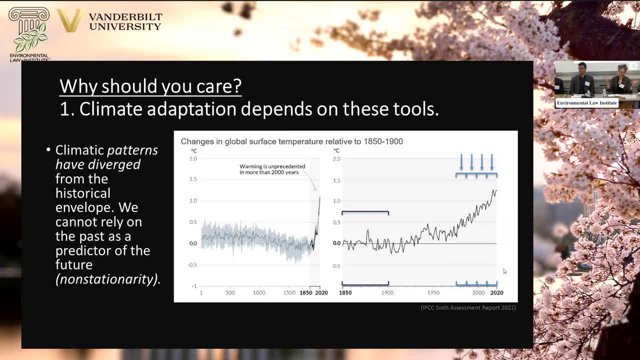 so climate adaptation depends on these tools, as you, this audience likely knows much more about than than you know broader audiences. climatic patterns have diverged from the historical envelope, so we can't rely on the past as a predictor, uh, of the future, right? so here on. 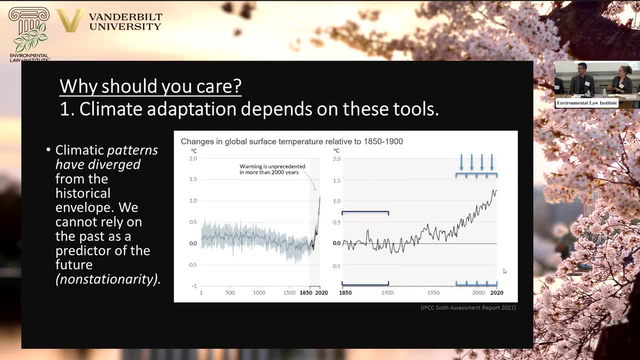 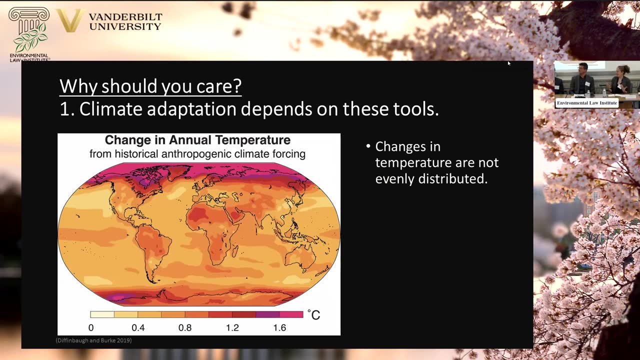 this graph you can see changes in global surface temperature from 1850 to 1900 and then later on. this is from the sixth assessment report, so it's a little bit dated. next slide: okay, these changes are obviously not evenly distributed. next slide: thank you, tassia. 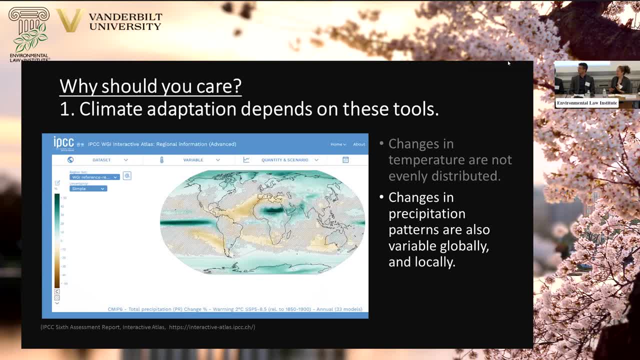 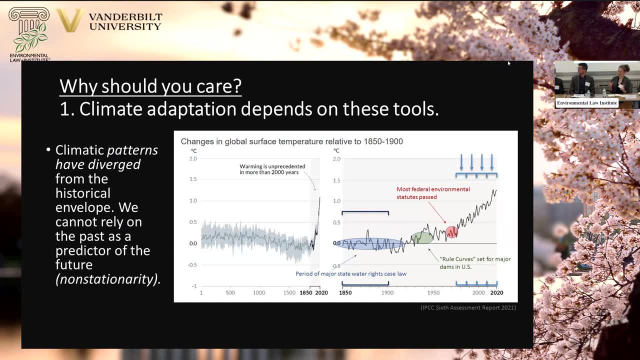 changes in participation patterns also vary dramatically. next slide, please. why this is a problem is because when we developed our laws and where climate is going now. so if you look at this graph, you can see the major period of state water rights law in the united states. all kind of happened when things were pretty stable. right rule curves for major us dams. 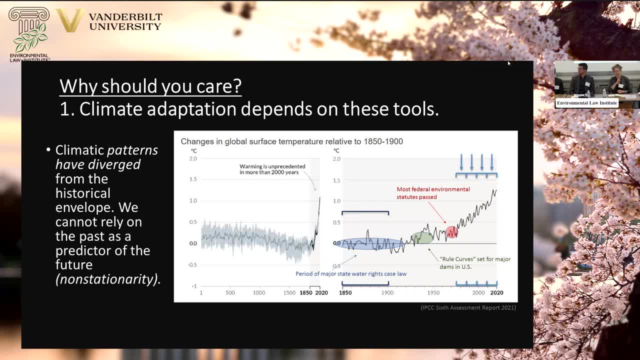 these are, uh, excuse me, subheading us army corps of engineers in order to decide how much water you can keep and when to release it. those were set kind of in the 1950s, kind of mid-century, last century, uh, but things have moved on since then. okay, next slide, please. that is an example of a rule curve. 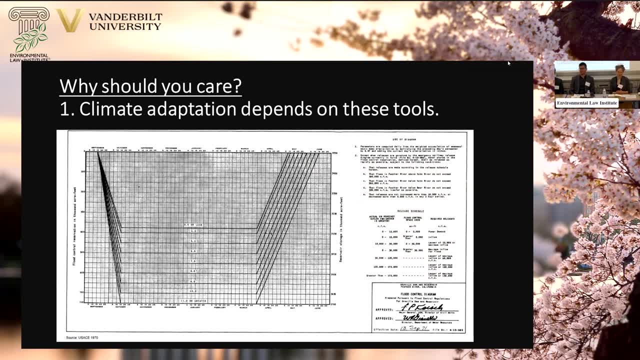 these are really important for dam operations. so this is for hydropower, for flood control, making sure that there's enough water for everybody. obviously. this is something that is crucial, uh, when you're talking about climate adaptation, in terms of who's getting water and when, um, these were done with slide rules in the 50s, with very, very limited historical data. so 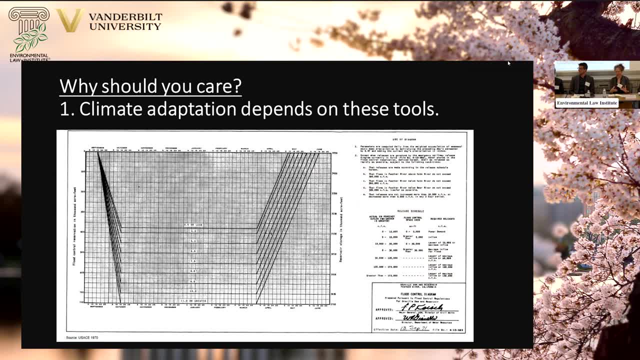 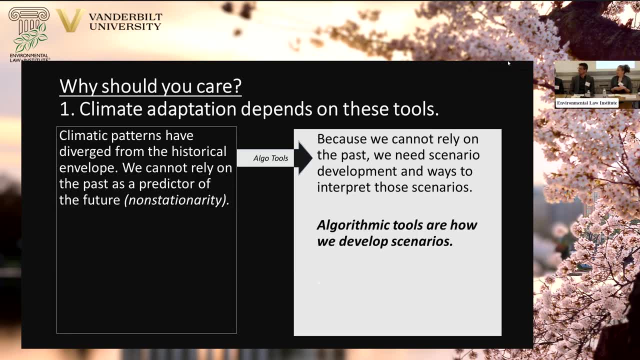 if we're going to adapt climate change, as discussed in the first panel, we need to change how we're thinking about some of these laws and planning next slide all right. so climatic patterns of diverge- right, we talked about that. algorithmic tools are what helps us, because we cannot rely on the past. we need scenario development. 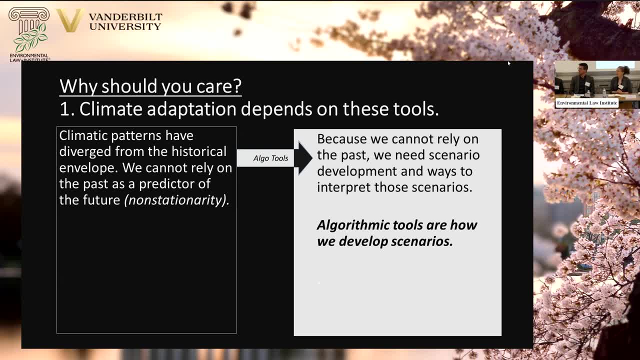 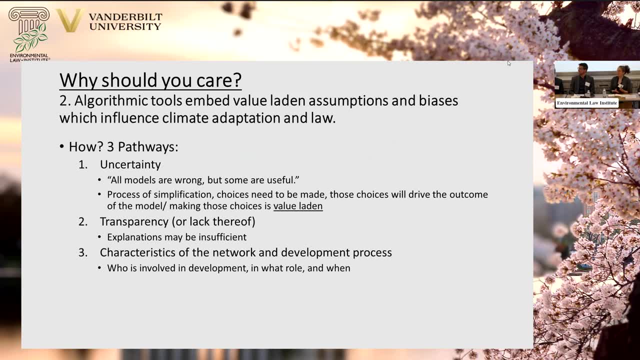 uh, in ways to interpret those scenarios. next slide: algorithmic tools, though, embed value-laden assumptions and biases which influence climate adaptation and law, so i want to pause from what's on this slide briefly to let you all know that the btc is an organization that works with the university of america to help young citizens. 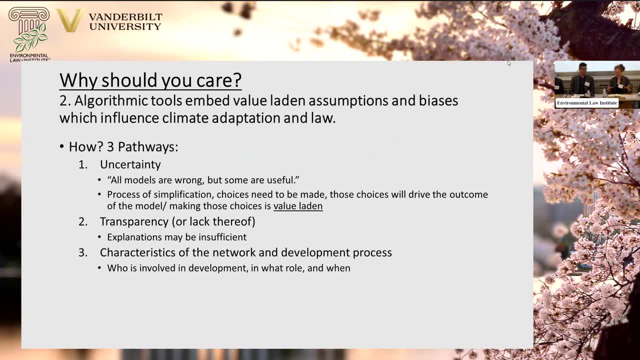 bring their own future challenges into their communities and learn from the attest um sort of um, and then i'll let you go into it. Algorithms are just programs for what steps to take when right. So okay, here's how value-laden assumptions and biases kind of get baked in. 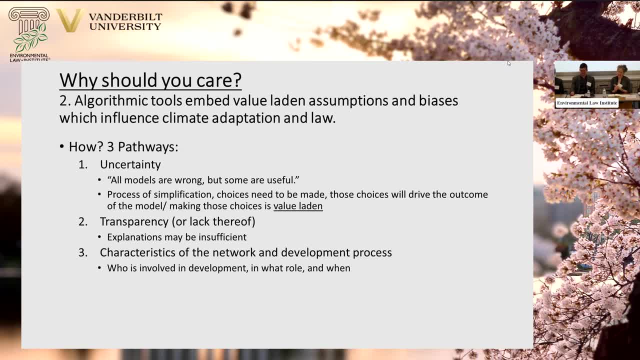 So my article talks about three pathways. The first is uncertainty. So all engineers say this: all models are wrong, but some are useful. This is something that they know right. But there's a process of simplification, Choices need to be made, and those choices will drive the outcome of the model. 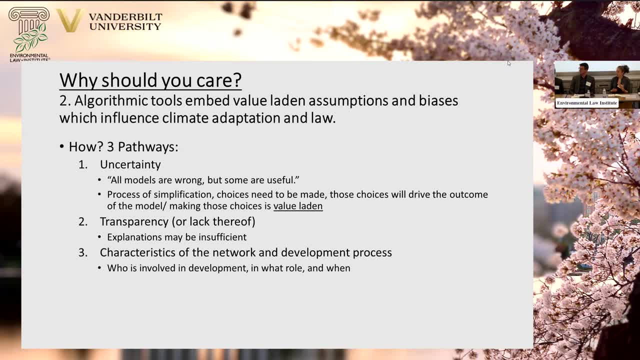 Making those choices itself is value-laden. Secondly, transparency: Explanations might be insufficient, right, If we have something? again going back to chat GPT, which I really shouldn't do, but taking that as an example, if you know, the company behind it said like: 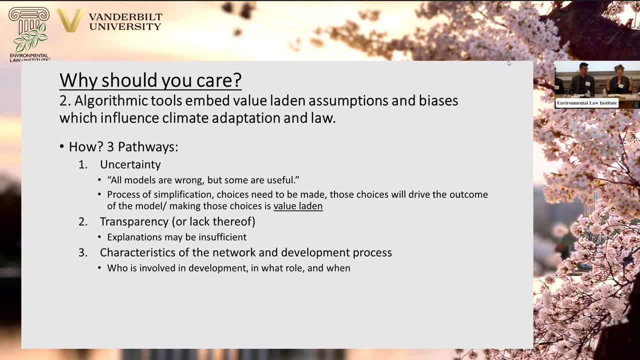 look, here's our code. Here's everything that we did. There are very few people in this room, and this room is packed with experts who would be able to understand that. right Information doesn't necessarily mean that there's a capacity to understand it. 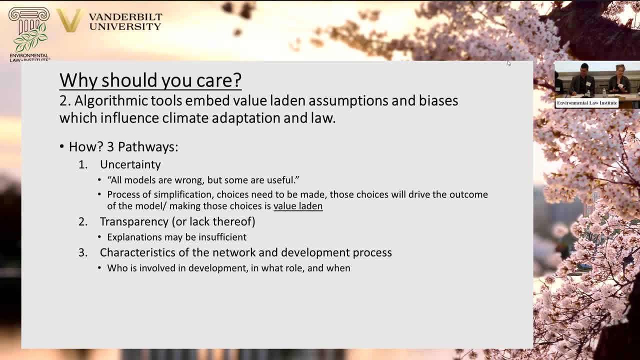 Third, the characteristics of the network and the development process. So you know these are tools, just like law is a tool, So they're tools in their form. But who is involved in that process of the development? In what role? 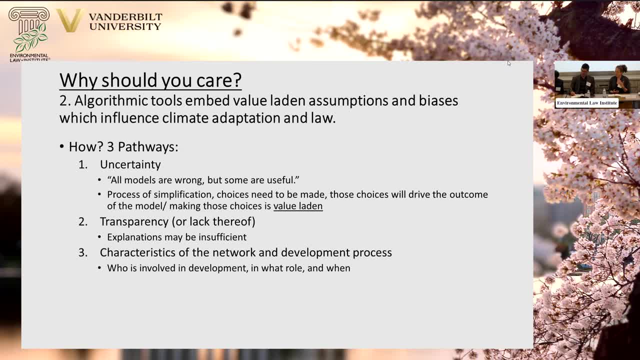 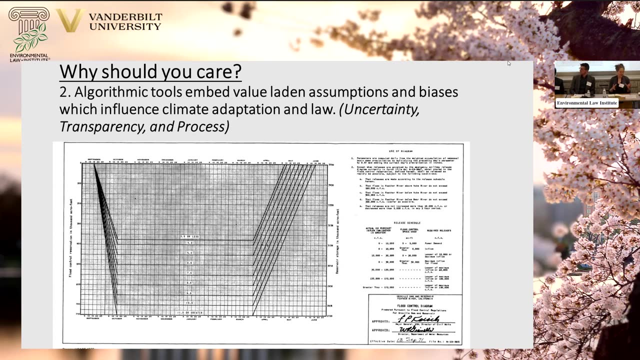 And when they have that role also influences what kind of assumptions are made in the program itself. Next slide, All right, So going back to this rule curve example. so one of the tools that I talked about in my article is this program called Inform. 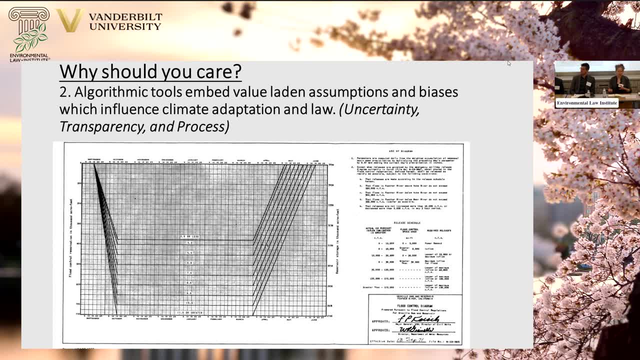 And Inform is used to regulate reservoir operations across a river and kind of combines a couple of things and includes you know, interesting climate scenarios And it turns out it does it a whole lot better than humans do. When I spoke to the developers of that program, one of the things that they said that they 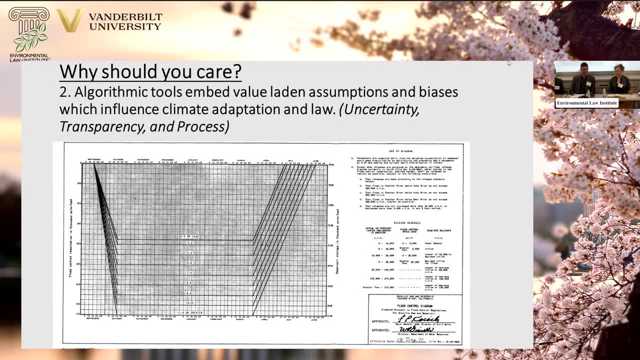 did was they went out and they interviewed existing dam operators. What they found out from existing dam operators is that they actually would diverge from what they're technically, legally allowed to do. So they incorporated that, that divergence right, That normal practice that people use, and incorporated it into the model. 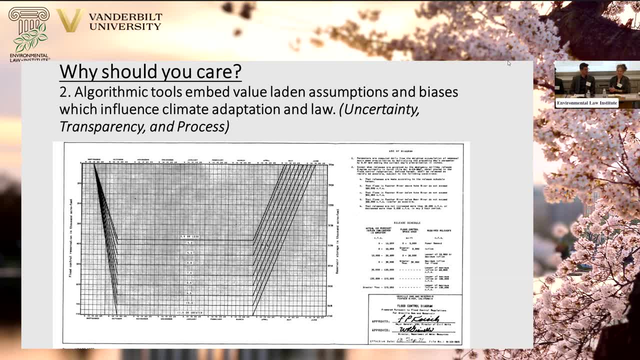 But at this point no one can remember, including the developers of the model, what it was that people were doing. that was different from what was on the books, right? So you're losing something in there through that translation. Next slide, please. 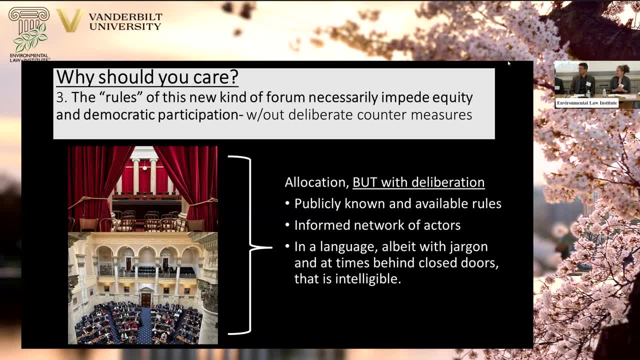 All right. Finally, why should you care? So the rules of this forum impede equity and democratic participation without deliberate countermeasures. Here's what I mean by that In our normal kinds of forums, right when we're thinking about courts or city councils. 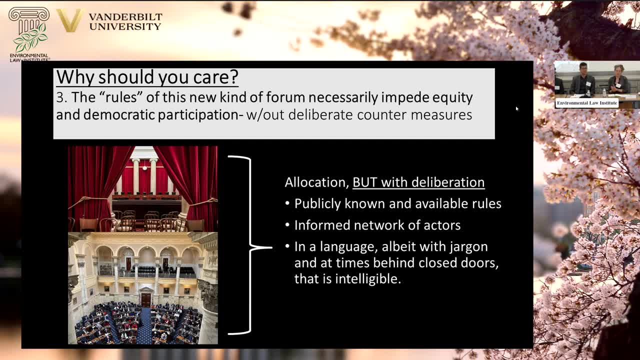 or legislatures. there's allocation, but it's with deliberation, It's publicly known and available rules. There's an informed network of actors in a language, albeit with jargon and at times behind closed doors, That is intelligible. 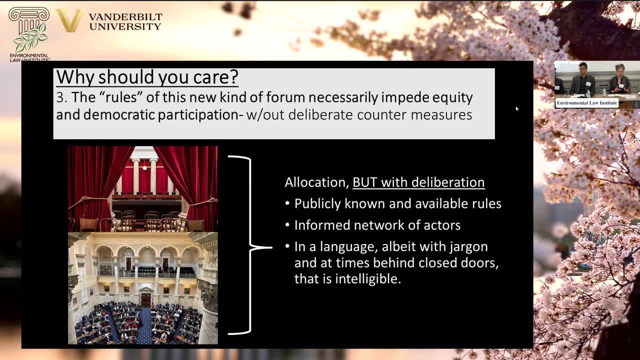 So, even though we might disagree with how those politics are playing out, it's all being done in a language that we No one can contreat and can critique, And there's an entire world of experts, many of whom are sitting next to me, who understand. 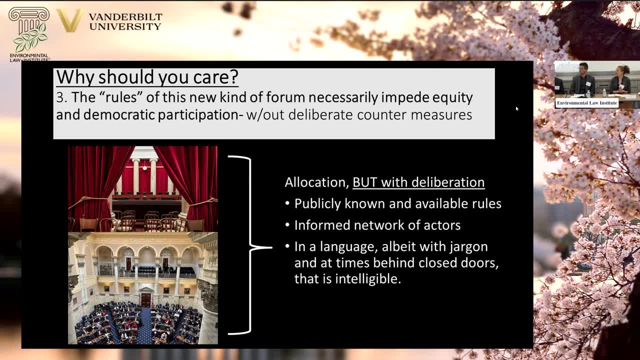 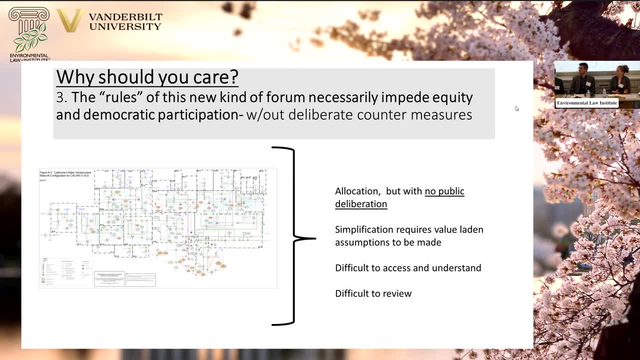 that and can help translate it to the public. Next slide, Excuse me So, with algorithmic decision-making, what we have is allocation, but with no public deliberation. There's a simplification which requires value-laden assumptions to be made. 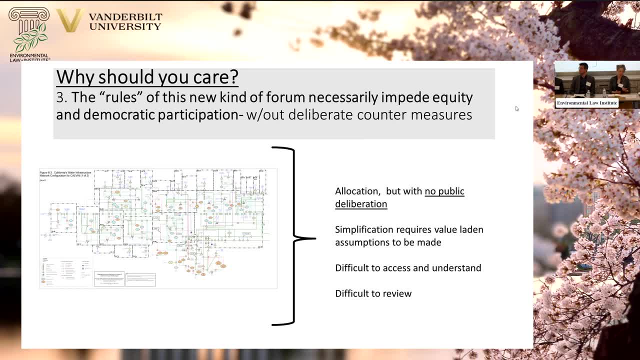 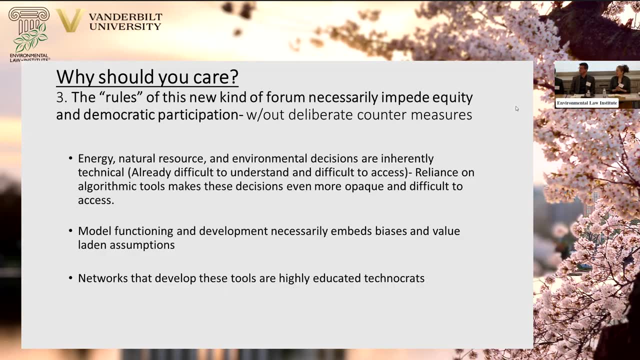 It's difficult to access and to understand, Which makes it really difficult to review Next slide, please. So energy, natural resources and environmental decisions are already inherently technical. They're very difficult to understand. My mother is a very smart person. 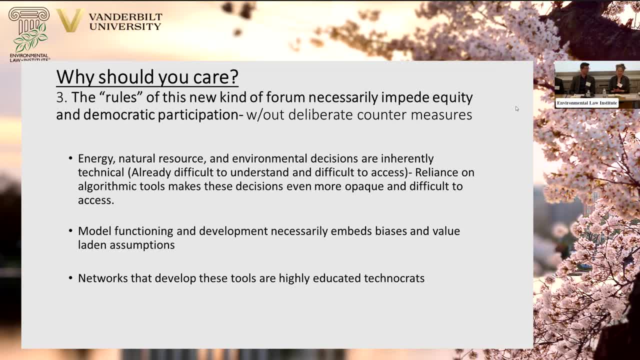 I try to explain to her what I do. There's, you know, only so much traction you can get there. There's a lot of expertise that's needed. Reliance on algorithmic tools makes these decisions even more opaque and difficult to access. 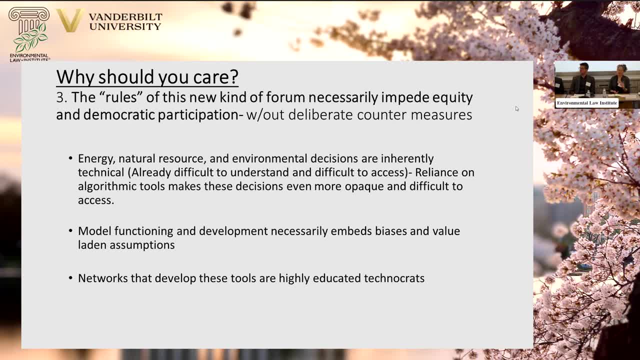 Model functioning and development necessarily embeds those kinds of biases and evaluating assumptions that we talked about, And the networks that develop those tools are highly educated technocrats, which I don't mean disparagingly Those are. they form really important parts of society. 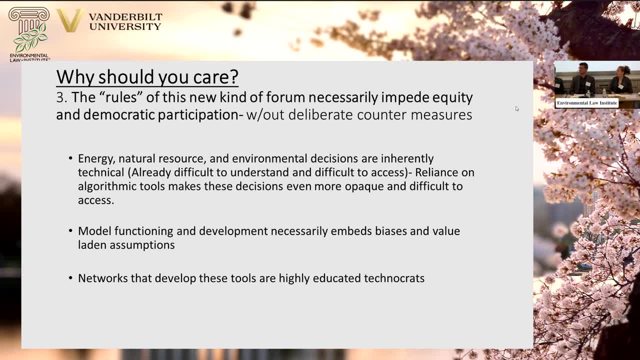 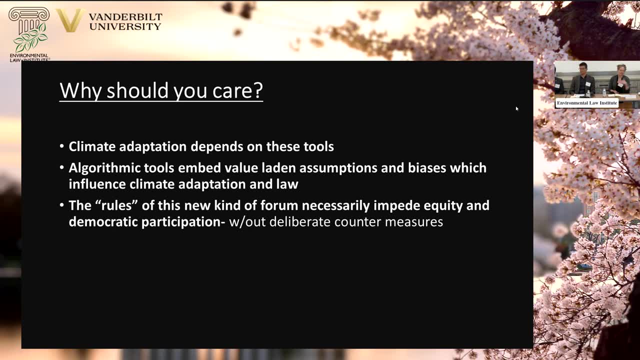 but are not representative of society as a whole. Next slide: Okay, so quickly to repeat myself: you should care, because climate adaptation depends on these tools. They're embedding value-laden assumptions by the kind of nature of themselves, And then those rules might actually undermine legitimacy. 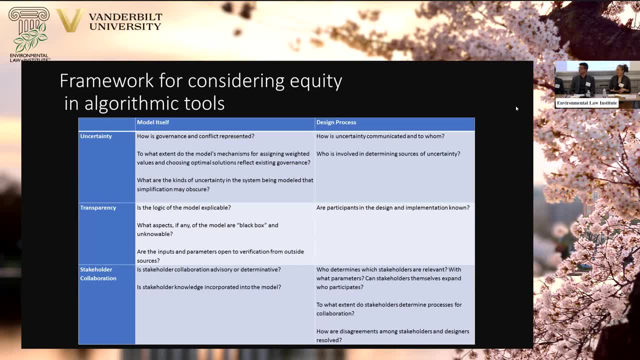 Next slide. So what I do in my paper is to try to open this up and create, at least as an initial step, a framework of questions that people who are interested in climate adaptation, who are in kind of advisory roles or who are kind of participating in these processes 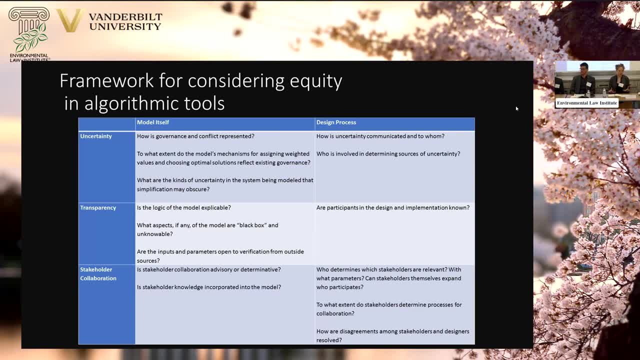 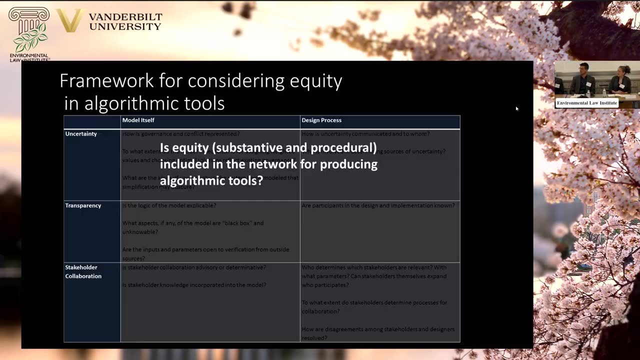 can start to ask to open up these models to more democratic and equitable processes. So I divide this up into questions that have to do with the model itself and the design process, And it goes through uncertainty, transparency and stakeholder collaboration. Next slide, please. 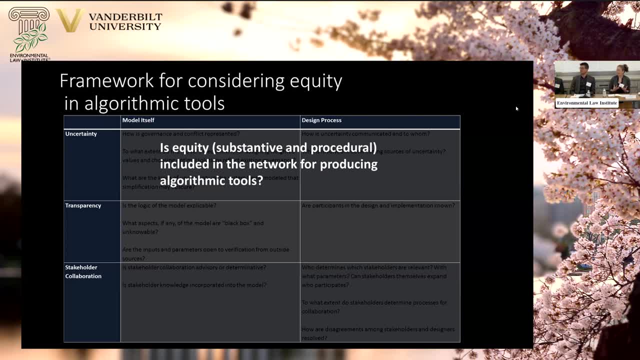 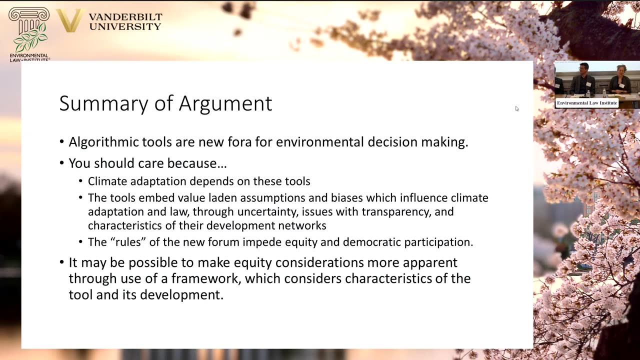 But all of these basically come down to this, which is: is equity, whether it's for our community, substantive or procedural, included in the network for producing algorithmic tools? next slide, please. so just to summarize the argument one more time: algorithmic tools are basically a flora, right? 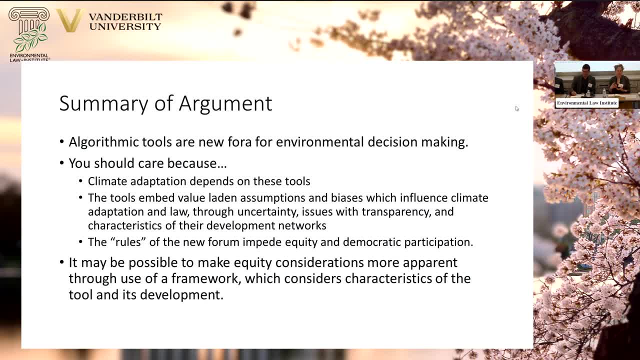 they're, because they're making these kinds of allocation decisions and then humans tend to follow those. we should understand these in a very different way than we have been. we, you should care, because really these aren't going away. we need them so much, just as, uh, the first panel had mentioned, but because of the nature of them, we need to. 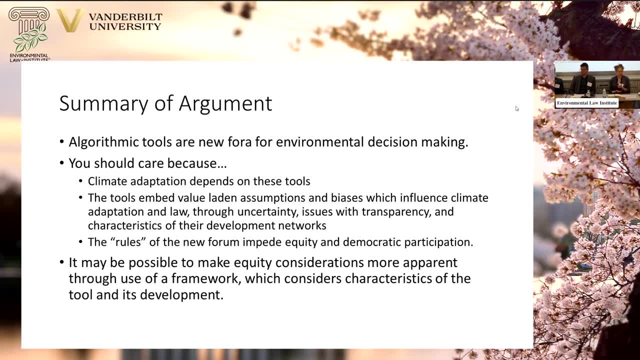 develop better systems for understanding them and to bring them back into line with, you know, what i think are still, uh, democratic values, although that might be changing in the united states. okay, it may be possible to make equity considerations more apparent through the use of this framework, which considers the characteristics of both the tool and the development. 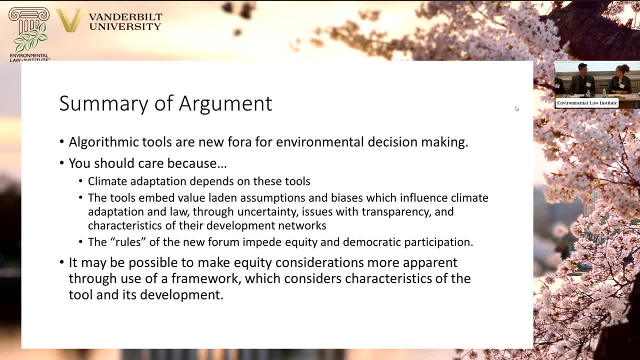 so with that, thank you very much. i'm looking forward to questions and discussion, and thank you for treating us all like 1Ls or people who do not like your mother. um, because i do think this is so important. the students can vouch for this when we read this: 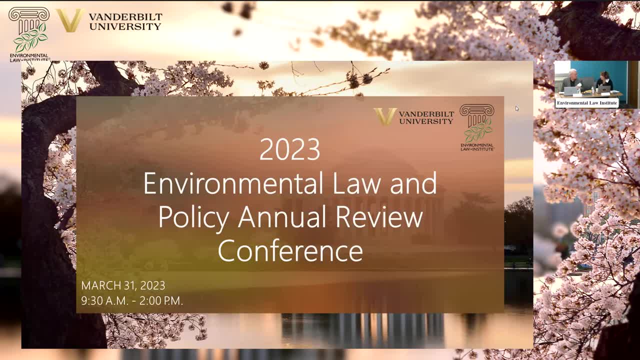 article. i was very excited because i hadn't in. in you know the decades i've been doing this, i really had never focused on this, and yet i focused lot on public involvement and we have a lot of discussions about equity and this is almost invisible. So thank you for writing the article and for explaining it to us in a way that at least 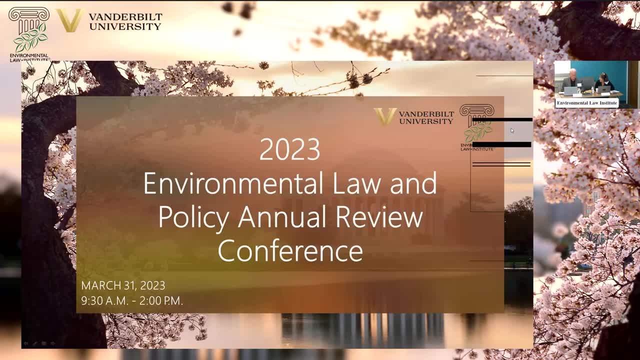 I could understand, and hopefully your mom And Keith. do you want to jump in here? Sure, Thank you. So thank you, Professor, for the article and for the explanation. Now I've read the article several times and I feel like this was still fantastic, Like the sort of curtains have fallen. 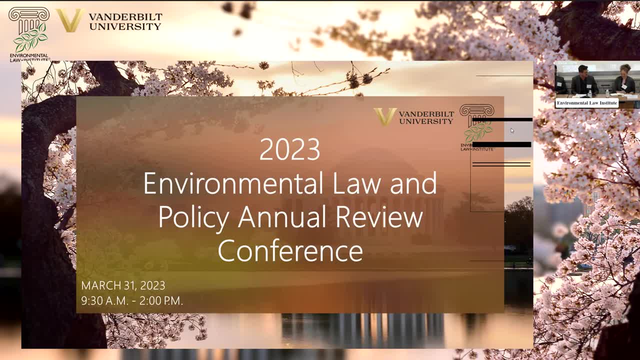 away and I'm like, oh yeah, So additional little epiphanies going on. in particular, I like your emphasis in the presentation of talking Sorry, And then in my points I just want to say if anybody on the panel, if anybody in the audience here has any questions at any point. 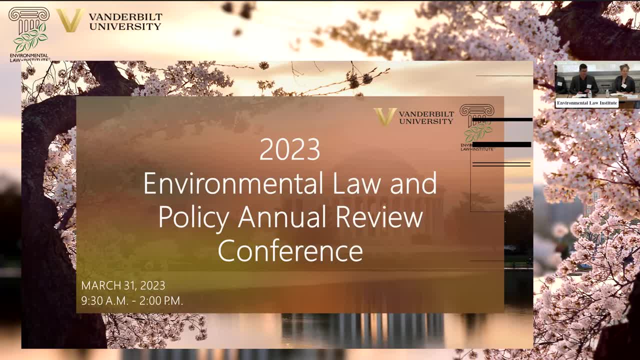 feel free to raise a hand, interject at any moment. I'm more interested in responding to questions than I am in the audience, So thank you. Um then, then just going through my points, but I had a few main points to make. 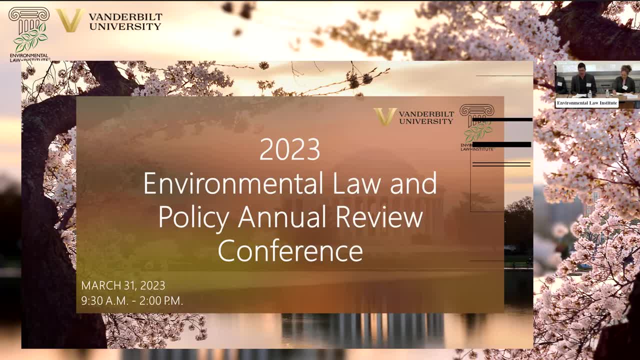 which a new one was that, uh, I really uh appreciated your emphasis on thinking of these algorithmic tools as as a forum for for decision-making, and we need to think about it in that way. Um, and, in thinking through that, I did want to emphasize a few of the points that 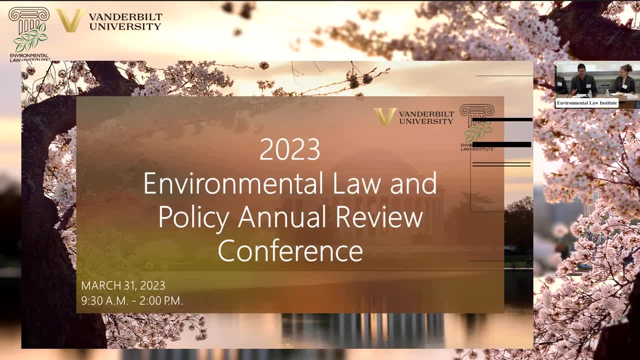 you made there. um, that that really stuck out to me as I read the article- And I think I've read it through several times, And the first one was: you know you talked about this- What, what do I think at one point you asked the question: what algorithms have to do with it? 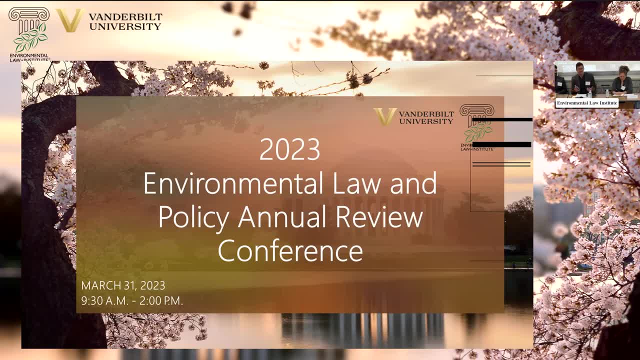 And from my point of view, it's. it's everything everywhere is sort of some sort of algorithmic based decision-making, as you said, from like down to a recipe that we're doing, but also, um, working in the office of policy at the department of energy, that our office is full of. 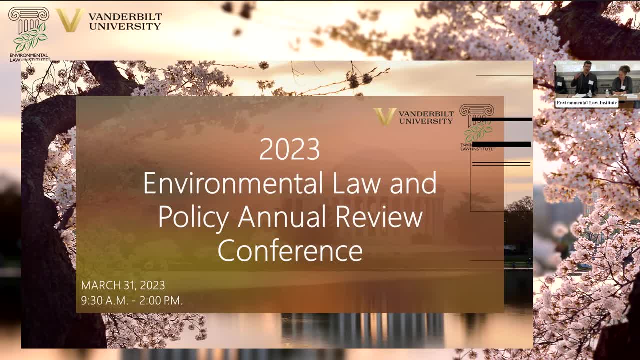 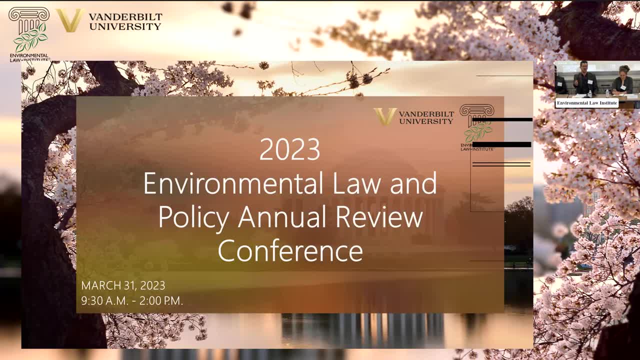 with national renewable energy laboratory, the experts Oak Ridge national laboratory, the sort of people with the supercomputers doing this modeling, are then working with folks in our office who are both helping develop the models and also translating the results of them for sort of policy relevant things, And so for me it feels like everything that I deal with every day is 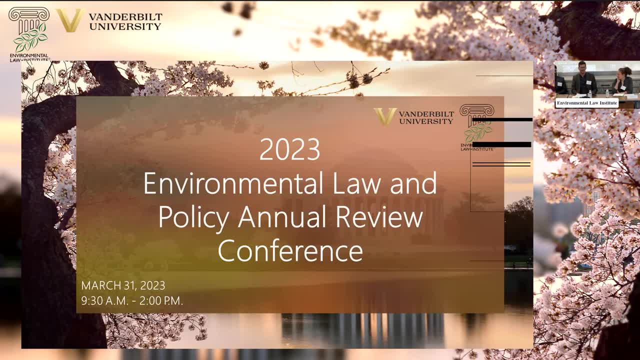 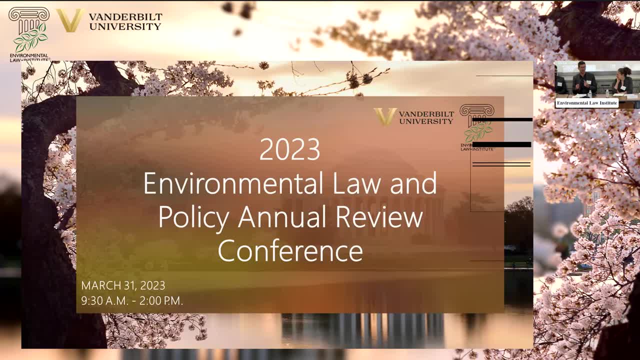 of all of this for one: put things into place, More people will come in. I think for surfaces we're starting to get really effective. Yes, like, figuratively speaking, already. Yeah, Yeah, All of the scientists in the university of Maryland. 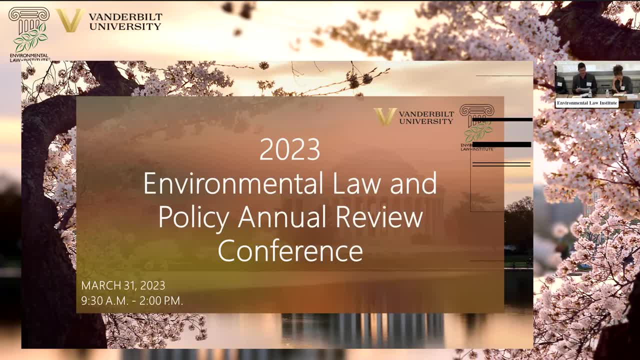 So hands off, hands off, actually, yeah, Um, in terms of other ska on this topic right now, there's a lot of. I've never, ever read it before. Um excellent Ins pregunta um um thank you, Thank you. 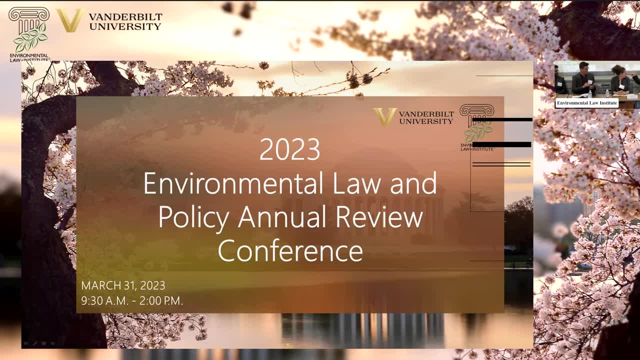 Thank you, and chat gpt. but hey, but don't worry, we have chat gpt responses. yeah, so they can talk about how drivers but they uh- and i will refer to this a couple of times because it is um interesting- and i did have a little bit of that uh sort of crisis of confidence in this last week of thinking every 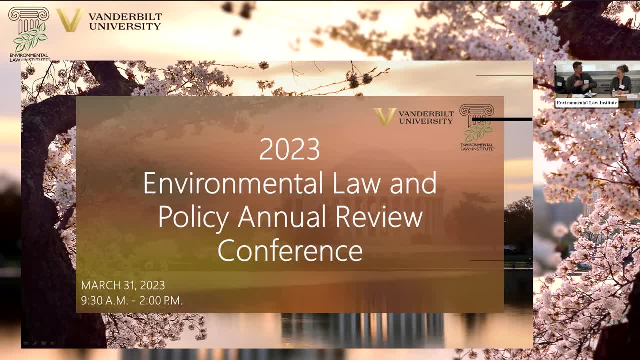 all of my observations are just: it's all superseded by this thing that's out there. now that everybody's talking about that, this is a fantastically complex algorithmic model. when you stop and think about it, it's the sort of chat, gpt and things like that that we're seeing in the news. 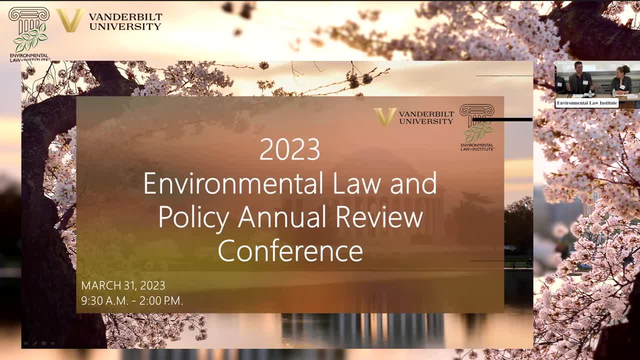 are one particular sort of you talked about. the sort of machine learning is something people talk about with algorithmic networks. it's only one element: chat, gbt, in these large language models, they're just one kind of additional tool that we have. i like to think of going back, uh, 10 or 15. 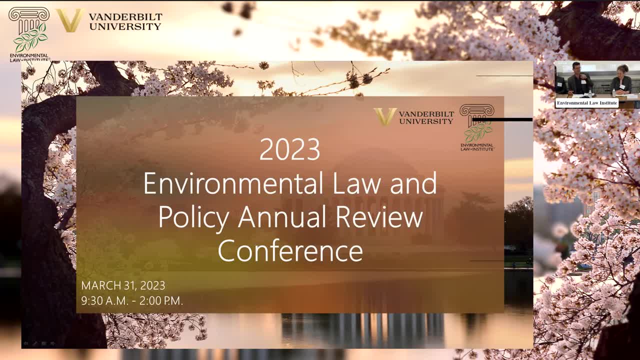 years when ibm's deep blue first beat uh master chess champion, and i forget gary casper. um, and you know in the headlines are then getting computers are taking over, the sort of the computers you know can now beat our chess champions. well, it turns out, the thing that could reliably beat a computer playing chess. 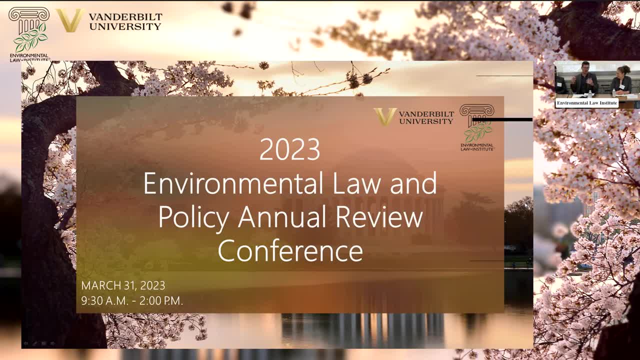 is a person in a computer playing chess, and so that that it is to keep in mind. even as these get more complicated, they are still tools for us to be used, at least for a little while longer, before they, uh, before they take over completely presumably. um, but one thing, another thing to 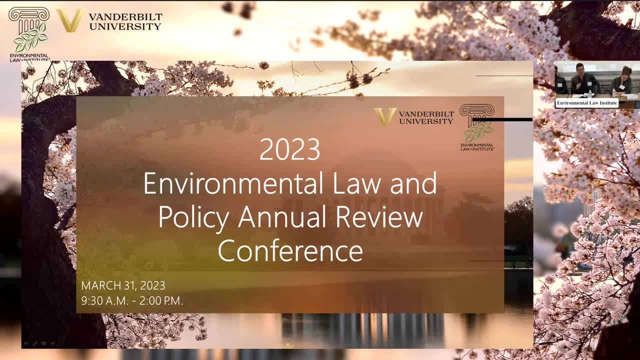 think about in terms of the algorithmic decision making is in the research tools that we use and have used for a decade or more, that we may not think about how it's screening what we're receiving, the information we're getting. we think about sort of facebook, um, you know, tick. 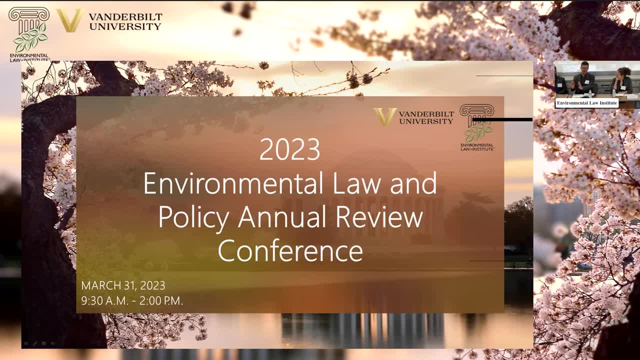 twitter, the way those algorithms work to feed particular content to people, and there's been lots of writing about that. but even something is just your basic google search and thinking about, am i actually getting a sort of objective view of the research here? i had an experience again. 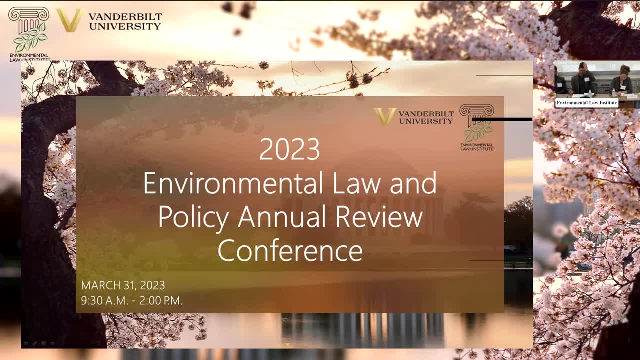 about 10 years ago, where i was working on a project, where i was working on a project, where i was working on a project related to the keystone xl pipeline that was proposed to be built from the us to uh, from canada to the us, and i was trying to research something on a specific oklahoma law. 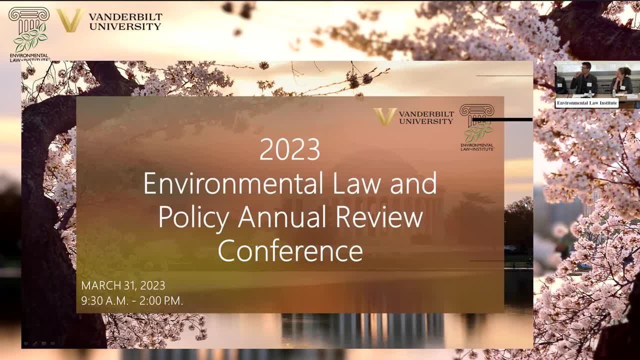 about pipelines and i was using google for it and no matter what search terms i put in about oklahoma, public utilities commission, i just would get 10 or 20 pages of keystone excel pipeline stuff and i finally figured out after about an hour of wasted time that i needed to log out log. 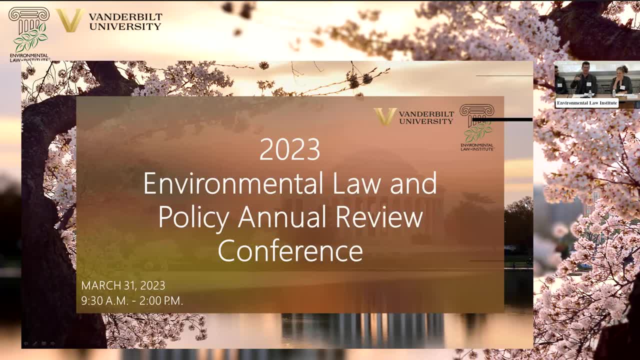 into a different browser without being logged in and then did the search and it popped up the first time and i thought, oh, it's just. this thing has learned that it's that this guy really likes this pipeline and just keep feeding him as much as he will get there and he'll click on it all um. so anyways, to be aware of all those, 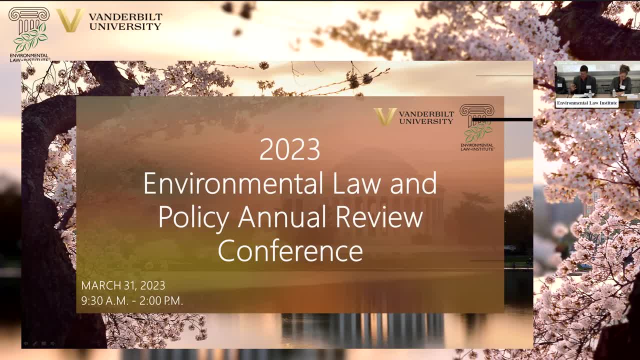 different places where we're now being influenced in um what we're being fed, not just by the specific tools, but the other ways we get information um one point relating to both unseen. i'm now see that i'm babbling too long, so i'm going to start going quickly. one point that i wanted to make related to both uncertainty and 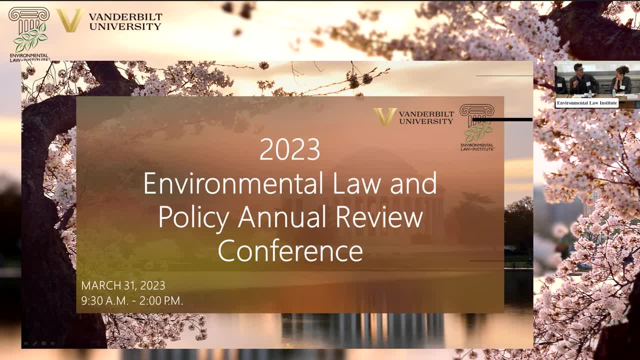 transparency. that both highlights the difficulty in this area for an additional example and was one of the ways that i thought a scientist best cut through that uncertainty for me previously. the first one is that in you mentioned several other places where algorithmic assisted decision making is being used, perhaps more directly, as just algorithmic decision making like. 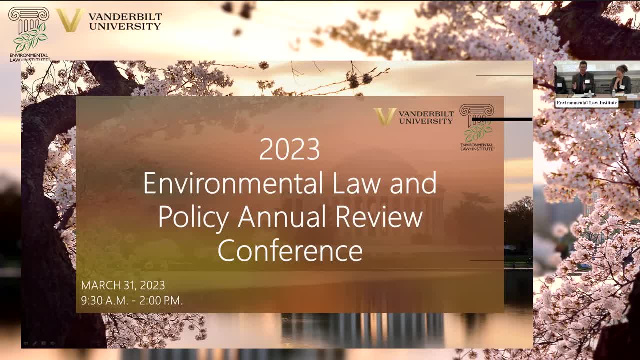 what comes out of the models, just automatically doing something. many states um, and in particular i know in nebraska, my home state, the welfare benefits the agency has contracted out to a contractor that is using their algorithm that's just determining, sending out benefits letters, benefit denial letters from. you know, this is not an insurance company doing it, this is the state bureaucracy. 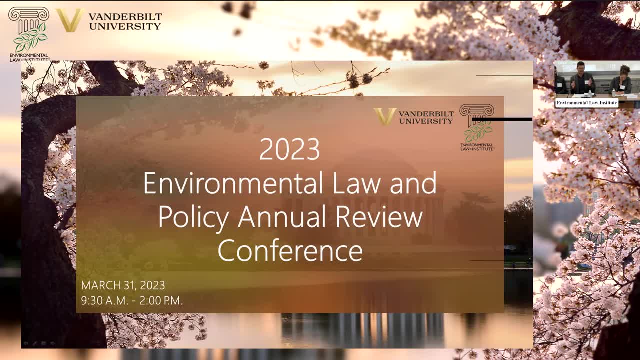 doing it through this company. um, i was talking a couple of years ago with an ngo in nebraska who's very concerned about this, worried about the transparency of it, and they were working, you know, through the public information laws to try and get access to the information that was being sent to. 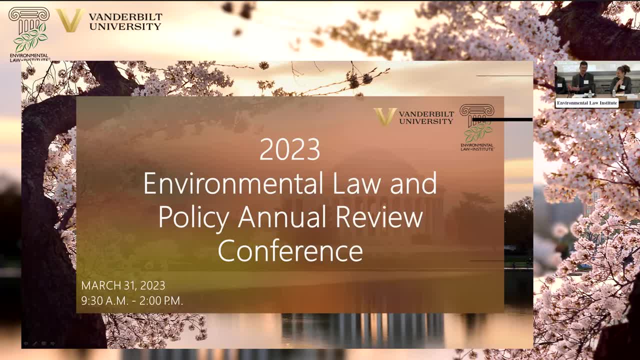 access to just what the code was, what the thing was, and they were running into problems with, uh, the company saying it's proprietary, it's not subject to the public interest law. so they were fighting that battle. but then they came and they were talking to me because they were like: okay, 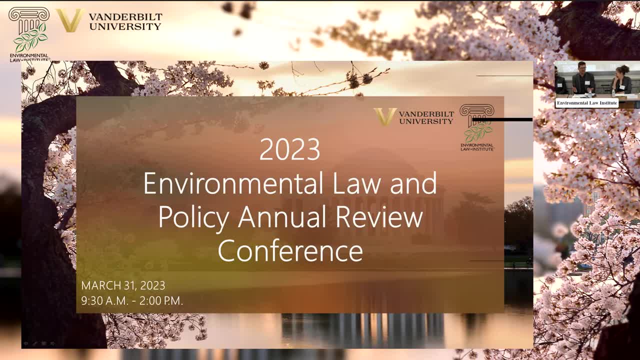 what if we actually get this stuff? like we, we're a bunch of public interest lawyers- like how are we going to make any sense of what's going on there? um, and it just highlights that, and it it is the. and, of course, my answer was: well, i can put you in touch with some data scientists who can help you. 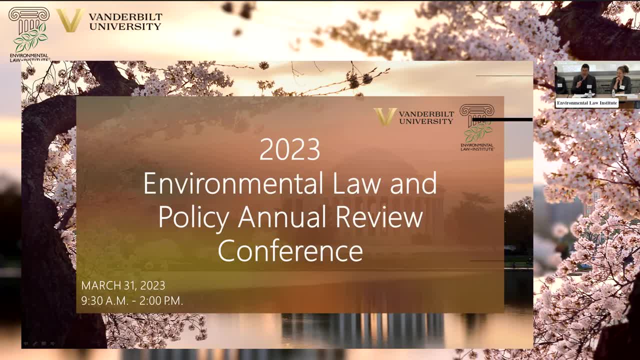 because i certainly can't do it either. but, uh, one example where this has been best explained to me was in a previous life, before i started working on climate issues. i did a lot of work on oceans, uh issues and living marine resources and working with um scientists doing population levels of fisheries. so you're trying. 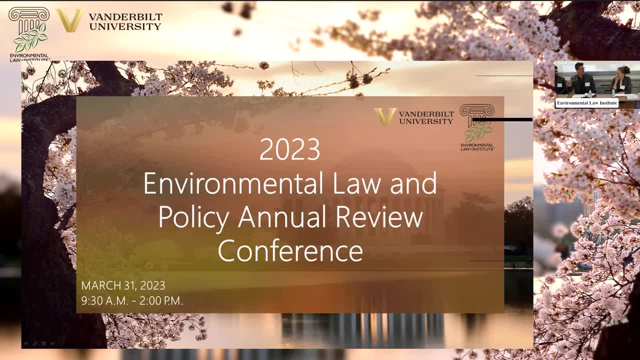 to manage high seas fishers, figuring out who can take how much fishing per year that will not impact the stock levels, and we were, you know, pressing our scientists and asking these questions and asking them what we should do in the negotiations, and we're going to be able to do that, and then we're 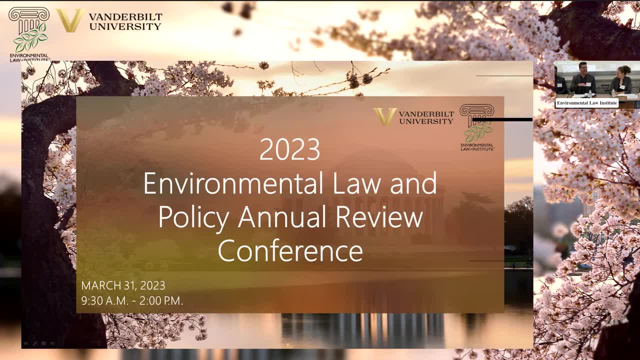 going to be able to do that, and we're going to be able to do that, and then we're going to be able to do that. so i'm talking about very important, like scientific questions. so i know, just imagine you need to be left in this position for a year, but you can't get that out of your grasp. 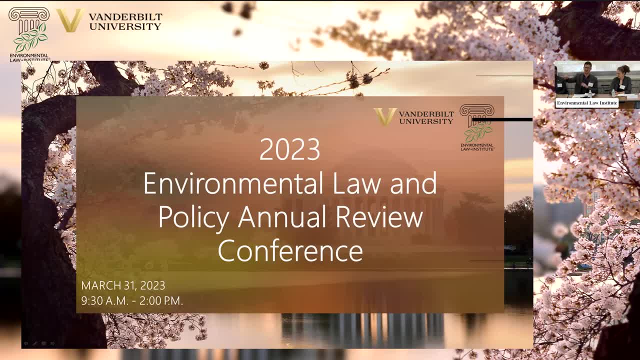 right, so and so um for a year. i really think that what we want to do is make sure that this- i'm trying to be here, you know, as as united i think you know we really want to have, as a function of all civilizations and both right um, the important investigation that so in schools. 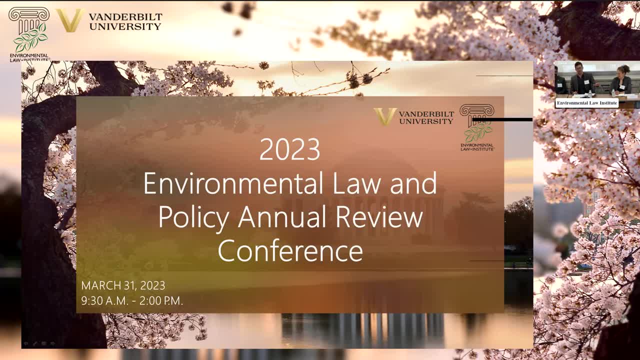 um, uh, for e-sports, and so, if you can see me as a blogs site, i'll literally insert the link-up there. but, uh, but at the end of it, you know, uh, they'll be able to get that answer into the législ�es match-up class. um, so there's few things to understand. i can't say. this is: 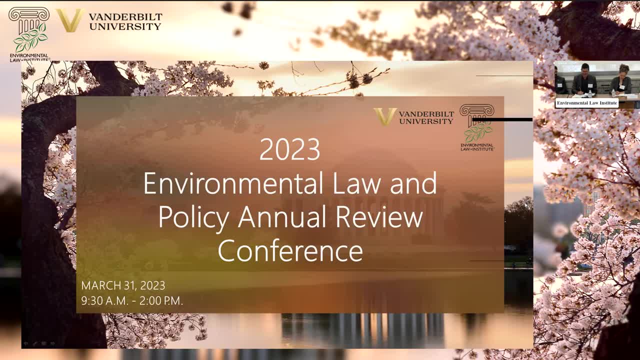 answer, And that is the which brings those still to even that information and the point that you make about the value-laden assumptions that can go on in the algorithms, both in the input data, which is a big issue in this area, also because you think of, for citing new transmission lines. 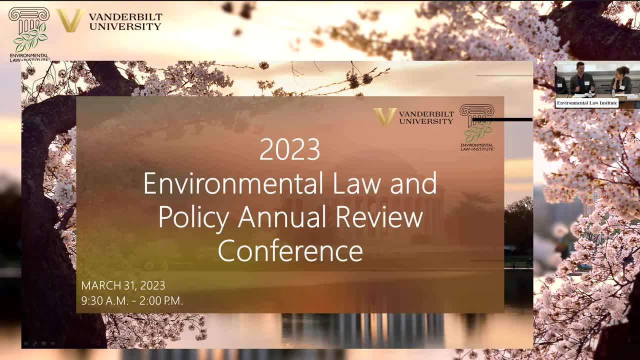 that we need hundreds, if not thousands of miles of them to help decarbonize, as a key piece, citing pipelines, any linear infrastructure. the citing will be done by an algorithm that is going through and figuring out a least cost solution for the developer, And it will do least. 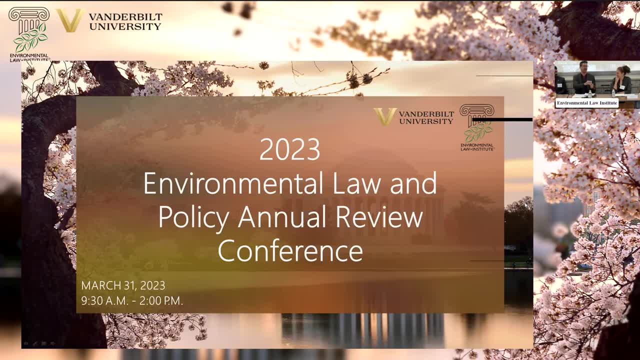 cost solution. it will avoid. it will have sensitive environmental areas, it will have heavily populated areas, So it's not just least cost. but then within all these things, it will chart out the least cost solution. So, of course, the least cost solution. 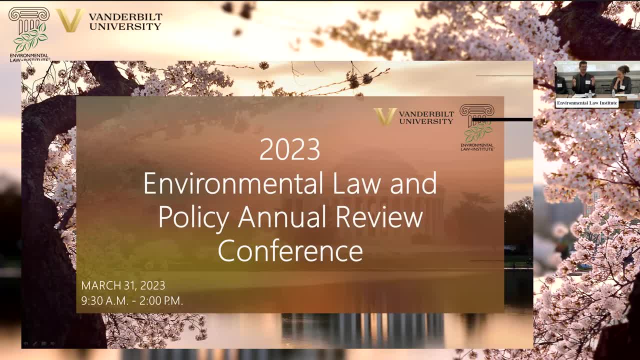 based on the property prices to acquire. these things will end up reflecting potential discriminatory practices that have gone on for decades in the past, such as redlining that was done by the federal government going back into the 30s, 40s, 50s, 60s, 70s, up until still now. 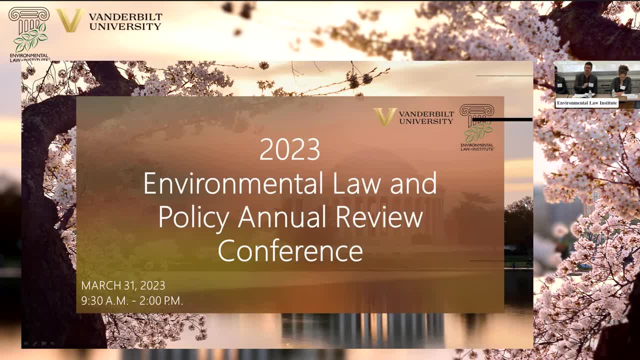 probably for private banks who are still based their loan decisions on these underlying assumptions about the communities, the people that live there, the value of those communities. you take and do that as your input into this algorithm. it's going to be the least cost. 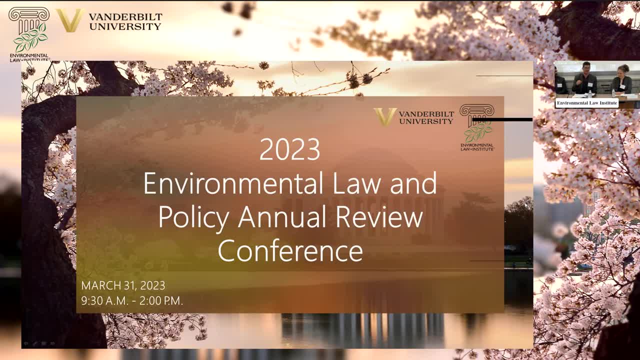 solution. it's also going to go to the most disadvantaged communities, the people less able, least able to represent themselves, the people with the least resources, most impacted already And then, just to give a slight, I guess, the uplift, the good things that we can do with. 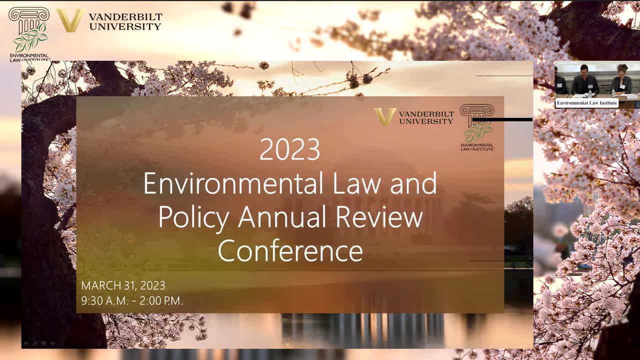 algorithmic decision making is that a project I worked on right before going back to the Department of Energy was working with a data science NGO trying to identify where they could make a difference in the sort of environmental justice or energy justice issue, And one of the things that we 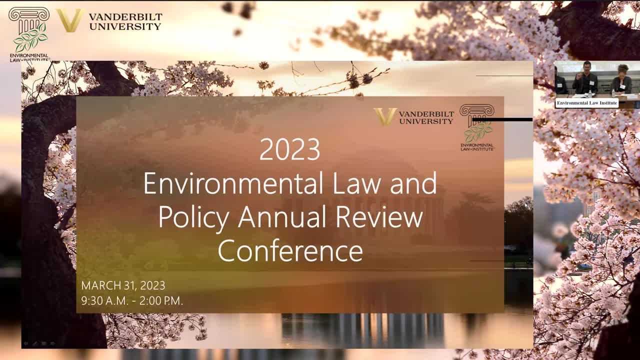 started to uncover as we dug into it is that there are a variety of federal and state programs that will help people with electricity bills for heating and cooling. federal programs that will help fund people weatherizing their homes, which used to just be thought of in terms of you know. 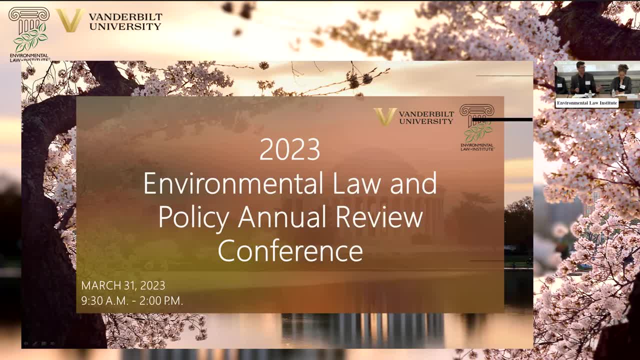 surviving cold winters is increasingly important now And we're seeing, you know, a shift in where these funds are needed to a climate adaptation thing, that in the warmer climates people are needing better insulated homes because they're starting to feel that impact more. 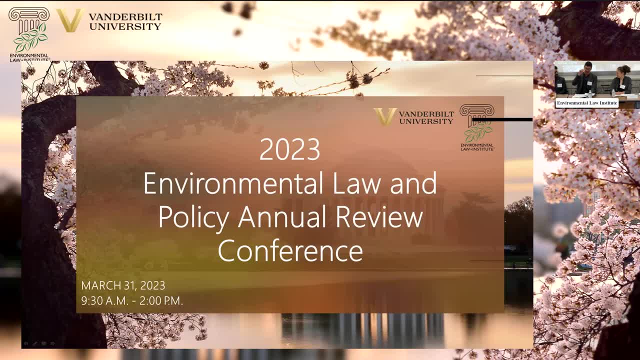 in their energy bills. And one of the things that we're finding with the- some of the study was done already and where we were directing this data science group to go- is that usually these things were done on sort of the census block level right, And census block is that might be 600 to. 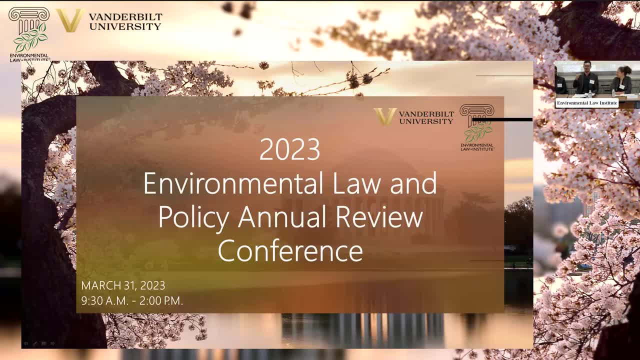 3000 people, 5000 people in a census block, And that's sort of how fine scale the data could be With using some machine learning and some advanced algorithmic decision making. people were doing additional studies, doing finer grained information on both geographic specificity and specificity. 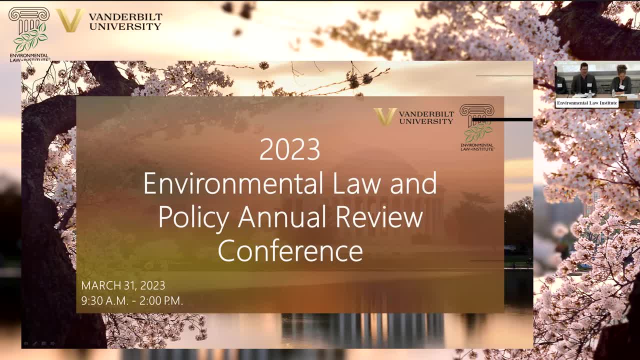 from you know energy uses down to a household level. we're finding that the the energy burden was the gap in the energy burden, the sort of the energy efficiency for the poorest households versus the wealthiest households. Past studies doing this on a census block level thought there. 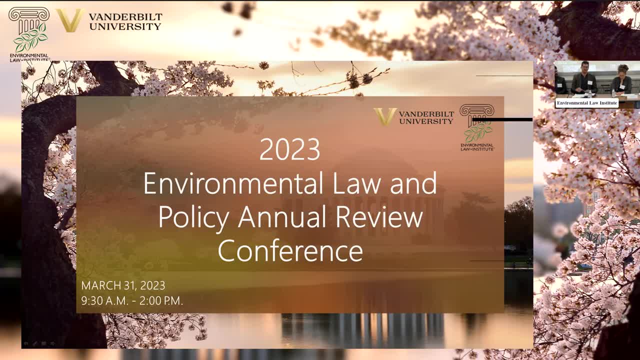 was about a 25% difference. poorest households are about 25% less efficient. when they started doing this at the more fine scale detail, they were finding things more like 27 to 167% less efficient in energy use, And so it's both uncovering a deeper problem than we realized, also giving the tools to better target. 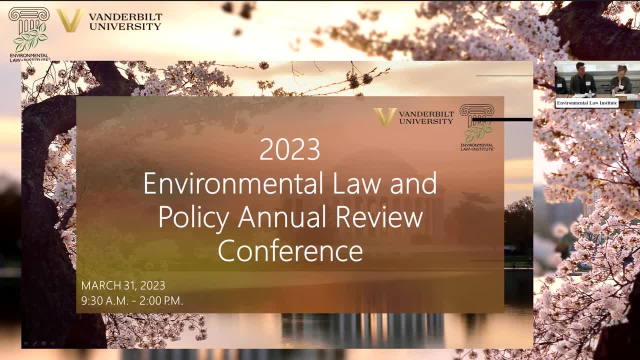 the relief to those who need it most. But coming to the participatory question, then, though, is- and what I would think, the next big thing that would be helpful for policymakers coming from the academic of building on the areas that you identified there, particularly on that last piece of helping figure out the most effective. 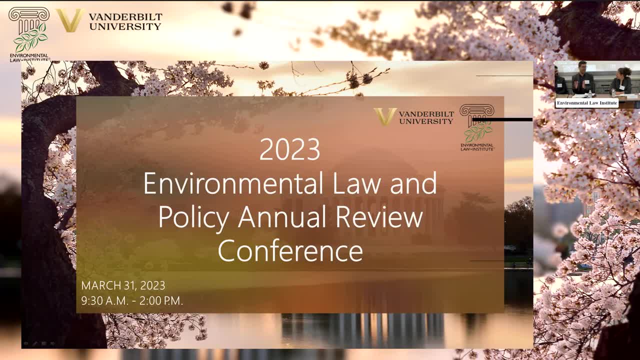 ways to engage and get input into the process from those most impacted, those most vulnerable, those with the least of the least, the least resources. to be able to participate in the process will be a key part of helping use the algorithmic assisted decision making. 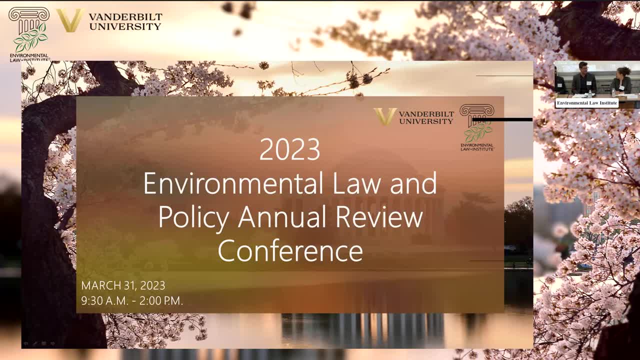 to both uncover the biases and correct them going forward. So, thank you, I'm sorry if I went a few minutes over. You don't have a Nobel Prize, but we still gave you an extra minute or two. Thank you. Yeah, but we will get one. 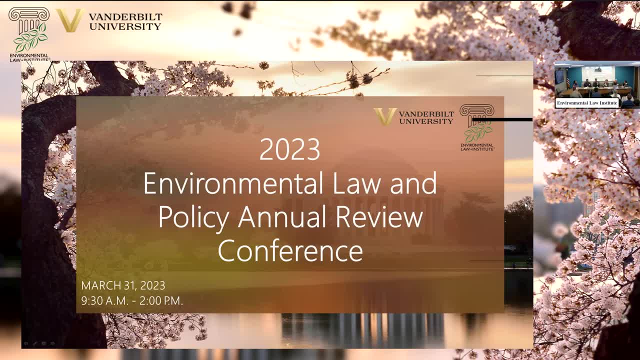 Yeah, someday- That's an anticipatory kind of move- It's going to be in medicine. Okay, Thank you very much for those really helpful comments. Mohit, do you want to go next? Sure, So I spend a fair amount of time working with lawyers. 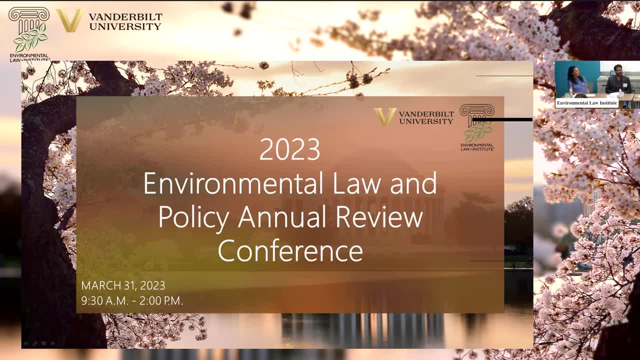 Participating in decision making proceedings and trying to help them make sense of the problem that Professor Janiya described. So what I'm going to say now- and this is in my written comments too- Rulise jumps uses her paper as a starting point, and the sentence she 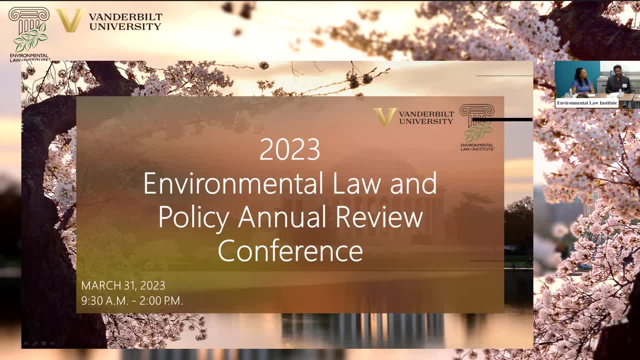 said that just getting information and understanding the process isn't enough. That's just a starting point. So what I grappled with was how do you empower advocates, stakeholders, technical and non-technical, to actually participate, to be able to make a difference? 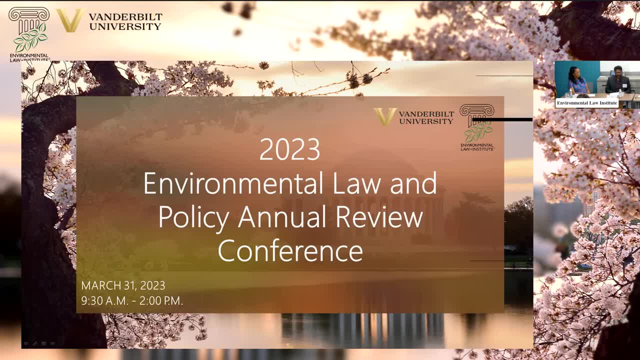 How do you go about thinking through that? I came up with a concept- could be better name, but I'm calling it building algorithmic intuition. I came up with a few questions that will help you start to get there. Before that, I think it's lost on no one that we are here because of what algorithms tell us and 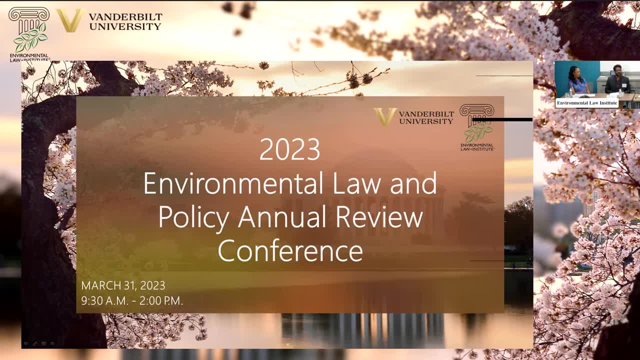 models tell us. Models tell us that global warming is happening. four degrees centigrade comes with a certain amount of devastation, and that's why we're here. So it really is. you can't get away from algorithmic tools in decision-making and policy-making in this field. 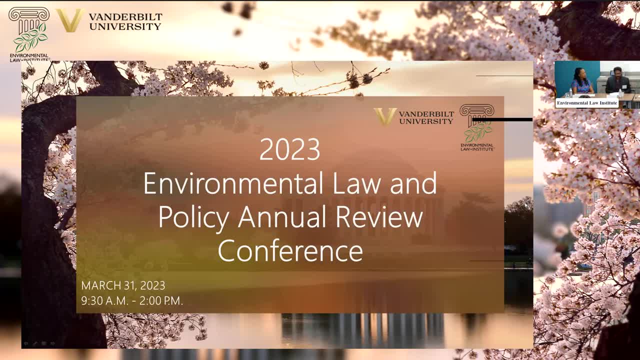 right. That's the basis of why we're here. An example is California. a few years ago passed Senate Bill 100,, which is the first of its kind, required zero carbon electricity by 2045. And I didn't see any proof of an algorithm deciding the date or how you get there. 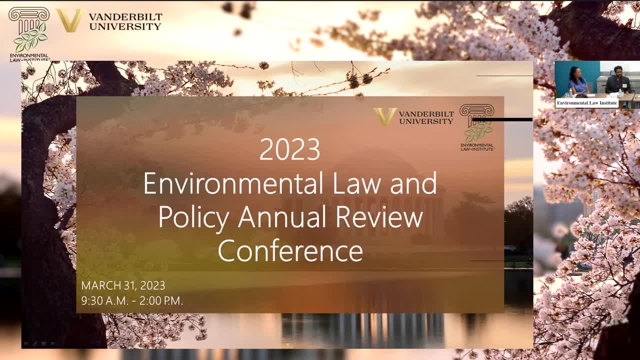 But once they decided that the California Energy Commission, Public Utilities Commission were tasked of figuring out how to do that in the least cost manner, keeping all our environmental constraints- And of course they used a bunch of complicated models to do that, Reason being that electricity travels at a reasonable fraction of the speed of light, 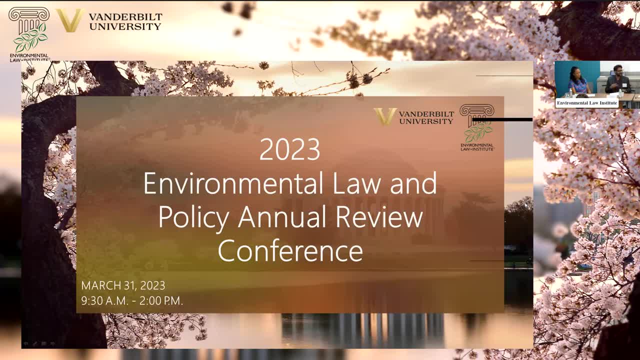 what you do on one end of the grid impacts all other ends. It's really hard to make these decisions without a tool. So well, what is this algorithmic intuition thing? So I broke it down into three questions. The first is understanding the scope of the problem at hand. and the scope 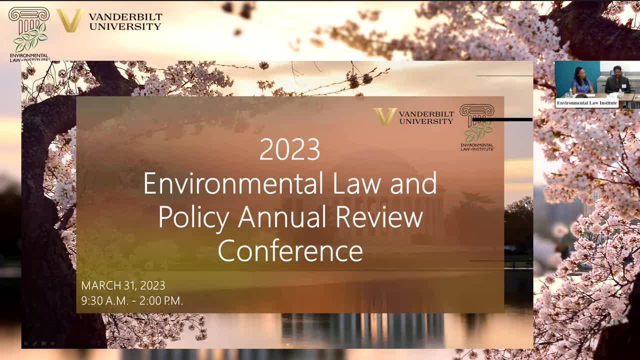 of the model- key parameters. The second is understanding the scope of the problem at hand and the scope of the model. And the third is understanding the scope of the problem at hand and the scope of the model. So I'll take an example of what I consider one of the darker black boxes that I've come across. 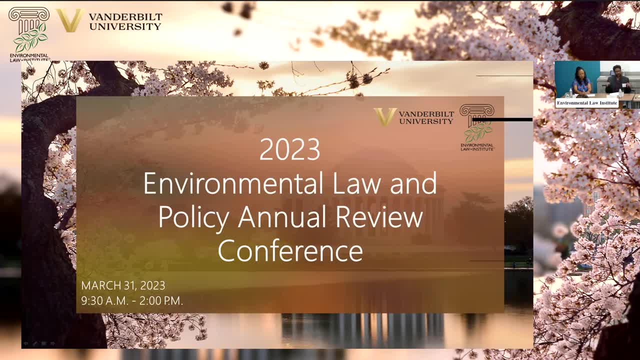 recently tell you what it is and then apply this concept to it and show how you know you could possibly participate in it. So the issue is the social cost of carbon or the greenhouse gases. The EPA recently tried to update that number. Some of you may have heard of it. 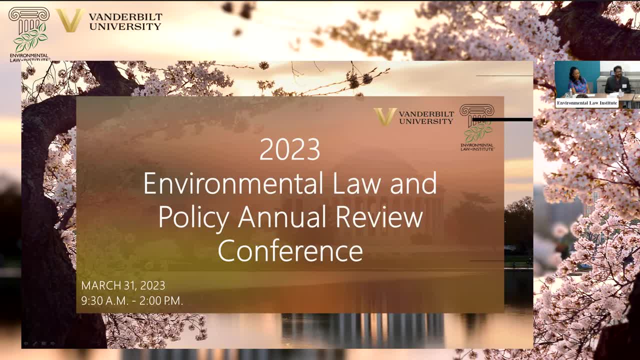 Basically it's an economic estimate of future gas prices And it's an economic estimate of future damages that carbon emissions cause. And it's important because when looking at regulation it's one way to figure out how much money should be put on mitigating carbon. You know we put in that much money commensurate to the benefits, right in simple terms. So how is it calculated? You start with surveying a lot of economists and policymakers to figure out future global gross domestic Product for the next 300 years. you know, broken down by regions and associated carbon emissions. 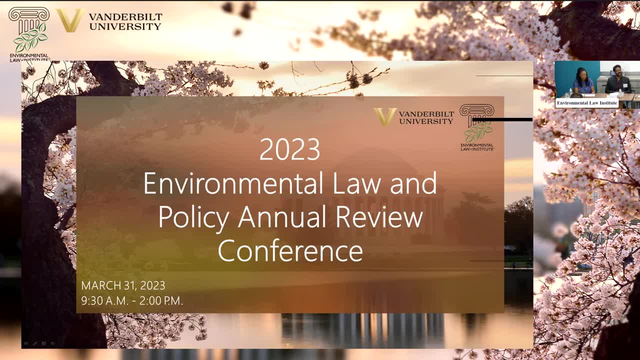 Then you take that as your baseline and you use climate models to understand the impact of an additional gigaton of carbon emissions on this. you know forecasted GDP and that many uncertainties and scenarios within that. Then you look at recent research. you figure out: well, what does that change in carbon emissions do in terms of temperature? 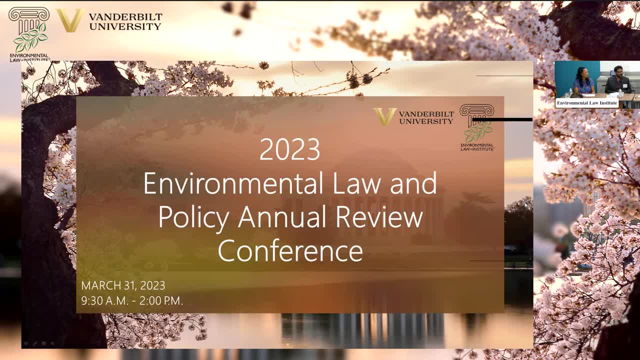 sea level rise and such, And then you try to figure out what's the economic damage in productivity adaptation And then you present value it to today, accounting for the economic conditions and your discount rate, how it would change based on how wealthy you are and how big of a disaster you. 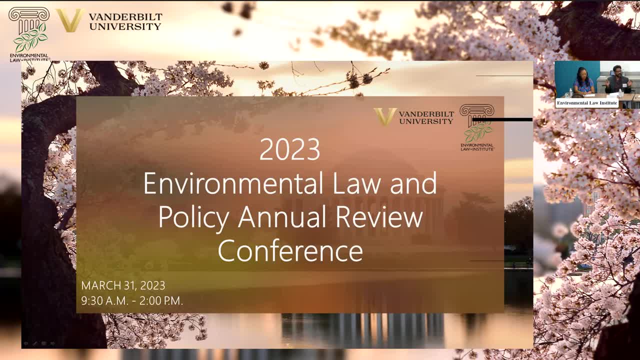 think is coming up. This is with a lot of simplification, And they, of course, do this differently for different zones of the world, They value mortality differently in different countries, and so on. So it's complex And I was, I had. 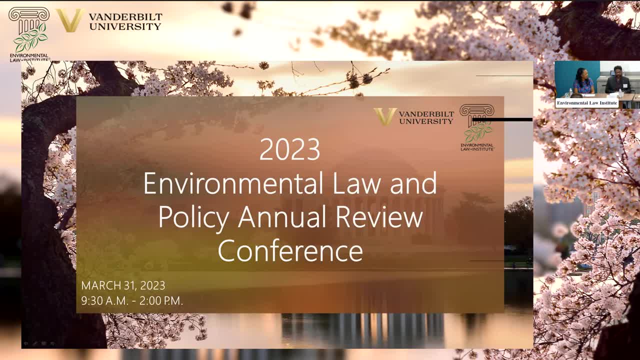 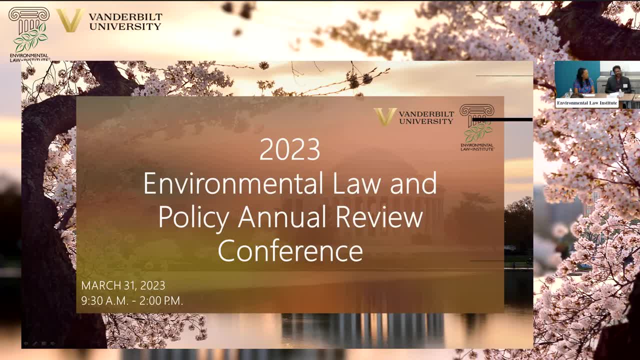 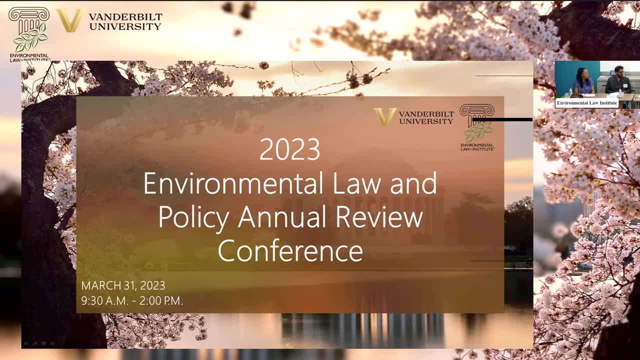 this EPA value is $185 a time. So that speaks to what Professor said about value-laden assumptions and how they impact outcomes. That's a very clear example. So let's apply this concept, starting with the scope. The first question is: should we account for damages only within? 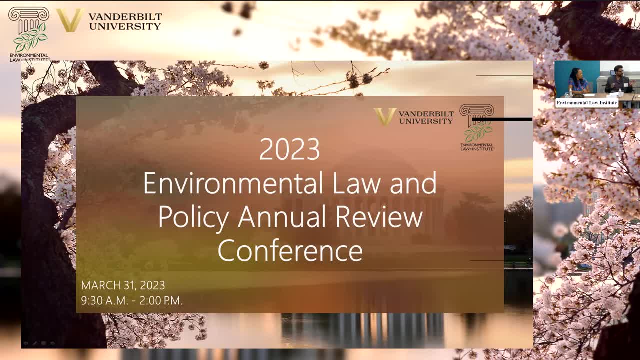 our geographic borders? Okay, Okay, Okay, Okay. orders in the US for US policy, or should this be global? Now, that's a legal question and a policy question, but that very factor was one of the main determinants why the Trump. 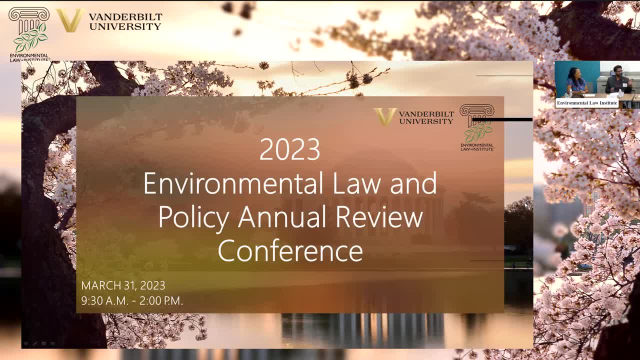 administration came up with an under $5 value. So just that scope question impacts your outcome significantly and that's something all of you could reason through and participate in. The second is what inputs matter most and why. There was a really good study done in. 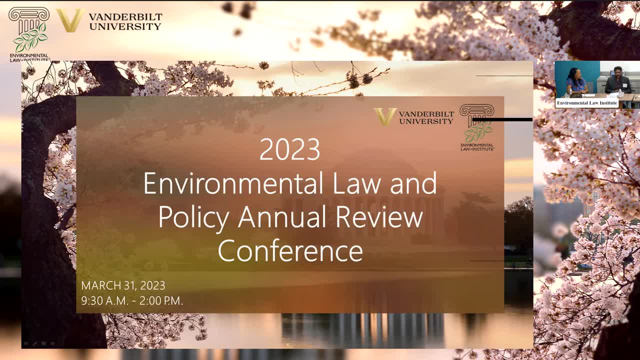 published in Nature that showed that what really matters most is the discount rate, how much you discount future damages, and also how much you value health, mortality impacts and agricultural impacts Therein. it's also apparent that this study doesn't value ecological. 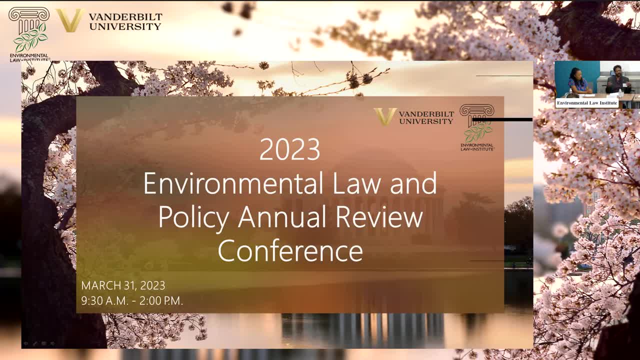 damage. So that's another place where you could weigh in on that wait. one of the biggest reasons why we're doing this is to evade ecological harm, but you aren't accounting for it And- Now you know exactly what parameters, even if you can't solve or dig into studies that 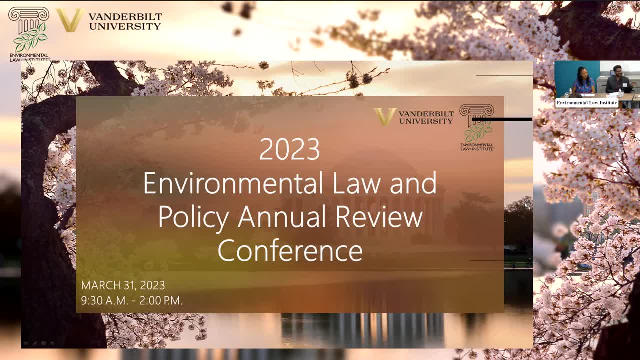 try to come up with a causal relationship between mortality and temperature, you know who to go to start advocating, And so I think, in explaining that I illustrated how the scope, key parameters and understanding causal relationships starts to form a certain algorithmic intuition, And not all of these. 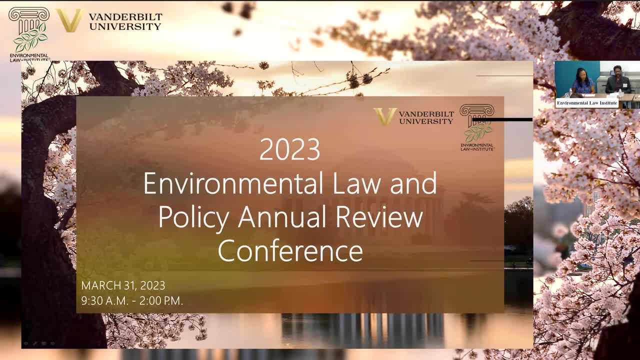 would be apparent to a stakeholder. So I think it is the responsibility of model developers and people facilitating the process to be forthright about these three things And one. I think you can all demand and ask for some of this information too, A technical way of 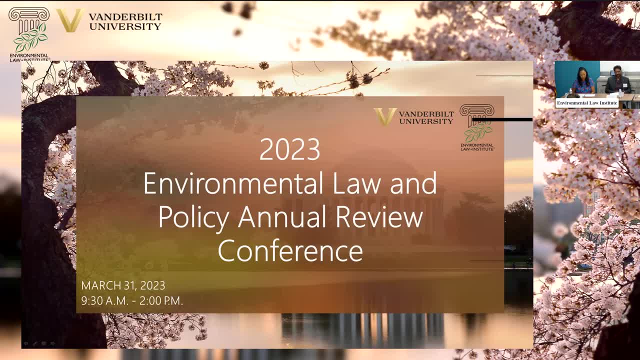 determining causal relationships. once you have a- Okay, a list, hopefully, from the developer on what parameters matter the most is, you take a model, hold all parameters constant, take the first key input, you double it and then you half it and then you go down the line and that gives you a really good understanding. 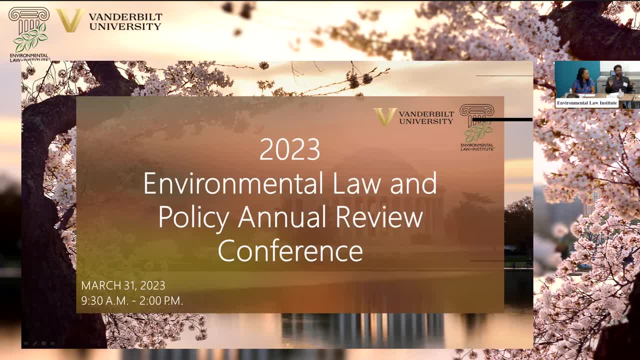 of what pressures on what part of the model produce what outputs. so you can conceptually reason out. how much of a difference would it make to my cost? should I even participate on this? and if I do, what should I pay attention to? but in closing, and to prove that I'm at least 10% less, 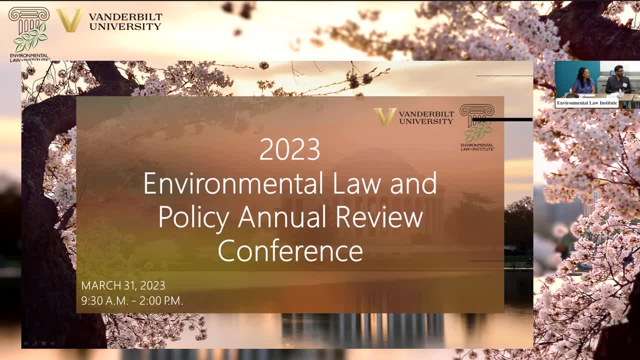 dry than chat GPT. I'll give off an example that my colleague just talked about, about the chess master, Gary Kasparov and the computer model. and Gary, our old friend, thought that he had an algorithmic intuition down. he knows chess really well, so he knew all the causal issues what moves. 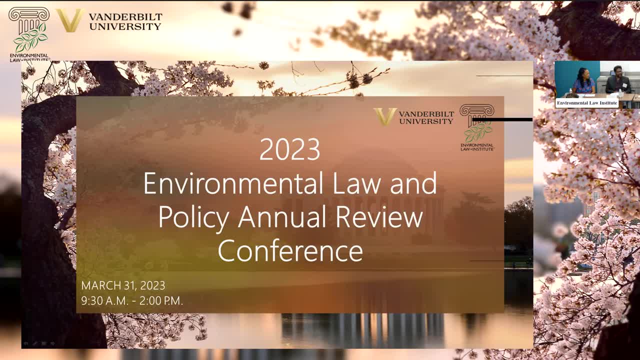 do what he knew the scope, which is that this computer is only looking at past data, right, and he knows all the key inputs and outputs. and I think, from what I've read, and if that book is true, this match was headed for a draw, but then the a certain move was played that really confused Gary, and it was a. 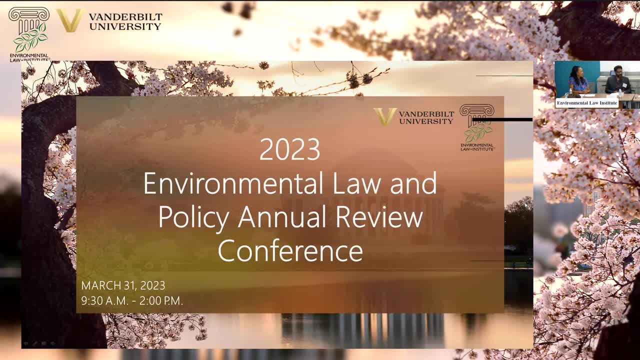 non-computer move and it made no sense from my algorithmic point of view, really confused him he ended up losing. turns out later that there was a bug and our friend's algorithmic intuition was thrown off. but if he'd stuck by this concept that I just 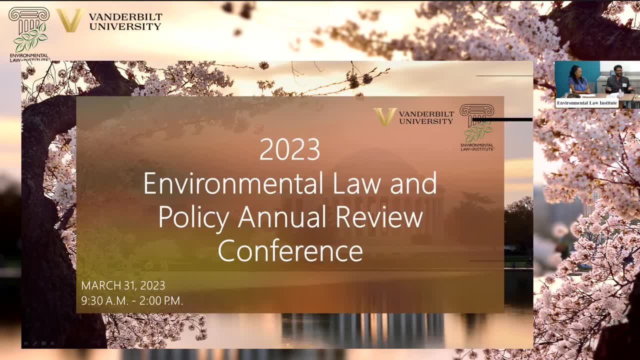 thought of in the last two days. thank you, thank you. this is all becoming clearer and clearer to me with each commenter. let me just mention a few people have referenced their written comments. in case you weren't here in the beginning, what's going to happen is that all the articles you've 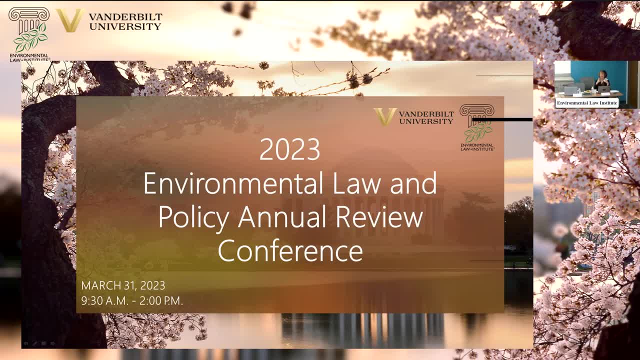 heard about today that are very long articles with a lot of footnotes have been condensed by Vanderbilt law students. they will be far shorter and then our commenters are writing even shorter comments, all the ideas to get this to practitioners and policymakers who are very busy and only have time to read shorter documents. it will be published in. 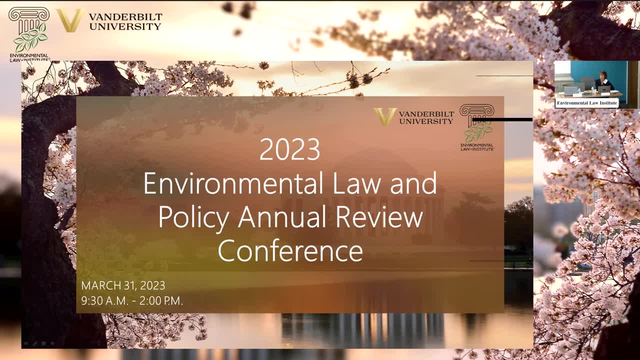 the August issue of Environmental Law Institute's Environmental Law Reporter as a joint Vanderbilt- ELI publication. but we will also be posting the articles and comments on the website in the next couple of months. so that's the reference to written comments, but the articles, the original articles, are available on SSRN social. 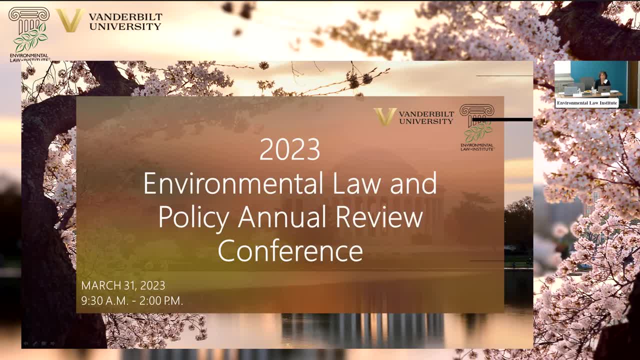 science research network and on the journal's web page that originally published the article. so if you want to slog through the 800 footnotes, or whatever it is, you can do that. so, Deborah, you're going to wrap up the comments for us, right, thank you? thank you so much for inviting me. I'd be. 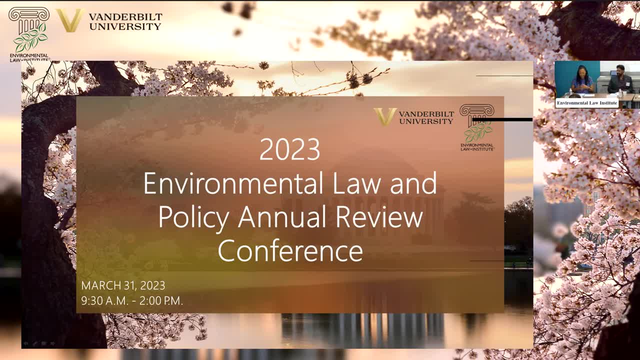 remiss if we did not acknowledge season shot this day today and labor rights. so let's just say that it's happening today. so I'm with the Greenlining Institute. we're located in Oakland, California. a little bit of bashing happening in California, but I'll share with you that California is the country. 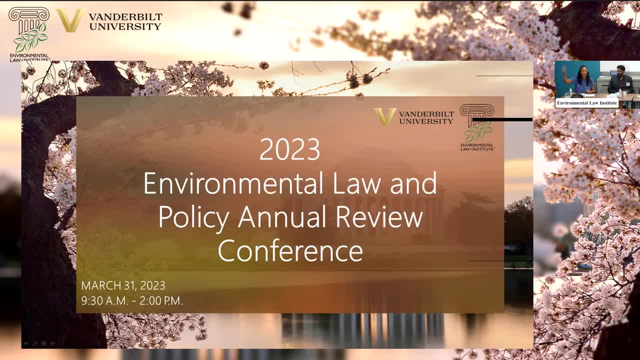 on fast forward. we are. we are doing things. some of the maps that we saw, we we were doing some of those initiatives about 10 years ago so it makes, I think, the country a little uncomfortable to look at what we're doing because we're so like leading edge, leading edge, failing fast. we are also you. 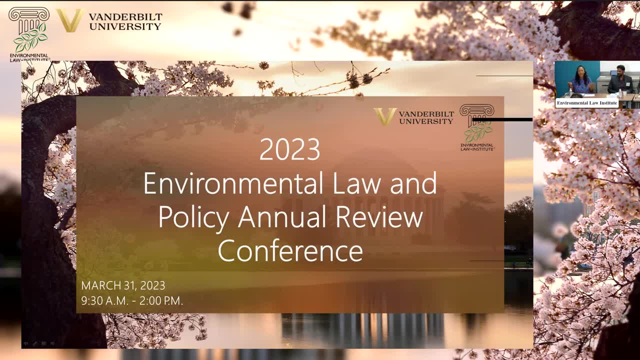 know the fourth largest economy- thank you, Germany, for dropping down. so I think that gives us a little bit of gravitas and being able to talk about, you know, sort of climate change economic equity. so Greenlighting Institute's been doing both economic equity and climate equity and we sit at that intersection for about 30 years now, and so when we were asked, 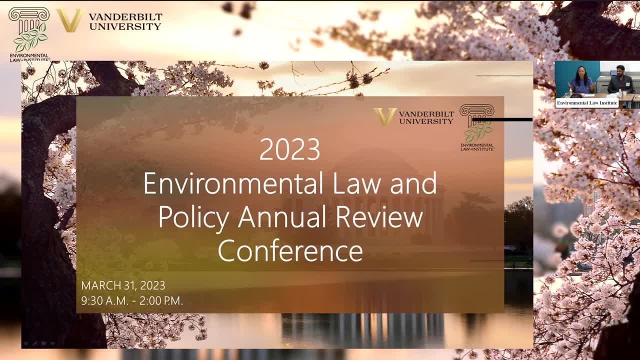 to comment on Sonia's paper. we were happy to do so. we had a particular perspective and I'm going to get you up about 30 or 40 000 feet and then you'll see how that will apply to everything that was provided. also, I I love being on the end because I have both the NRDC and EPA. 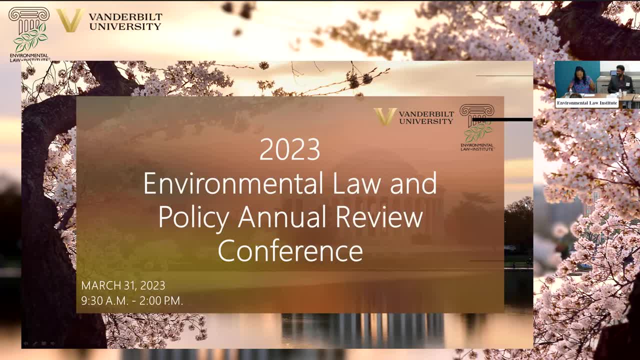 these are not these are. these guys fight a lot so but it's good they're, it's great they bring a perspective to them, to the market, and so what we, what we have seen at Greenlining to to really help set the brain here, is just straight up algorithmic bias. so the context of which you've heard here is: 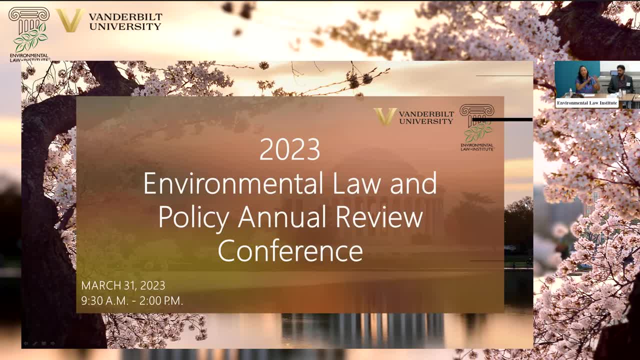 being played out in both the economic landscape and what's happening in the economy and then in the environment. and for us, if I can just Center equity right, it's not equality. I like that we're positioned between the four degrees and what's coming up, I think the ESG, it's coming up equity. 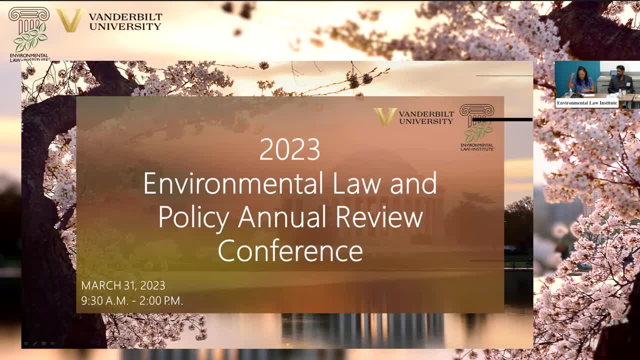 is not ESG and it's not DEI. equity is recognizing that we start at different places and that there are disparate treatment and disparate impacts, and that would create solution, solutions, systems, institutions and behaviors that account for that. okay, so if you're looking at, uh, some of 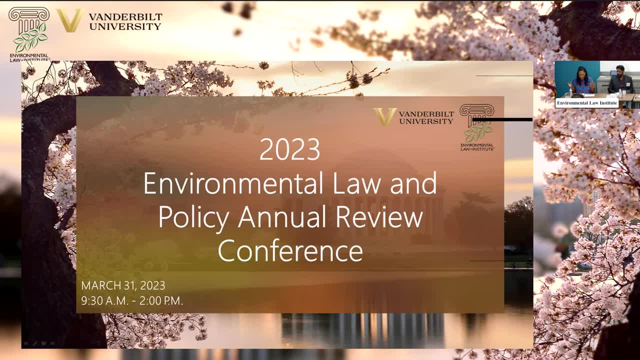 the um, climate change and some of the initiatives that are happening. um, we start to see that the algorithms are based on profits that are privatized and losses that are public, and so if you have this value and you're starting to get to it with the cost benefit analysis and 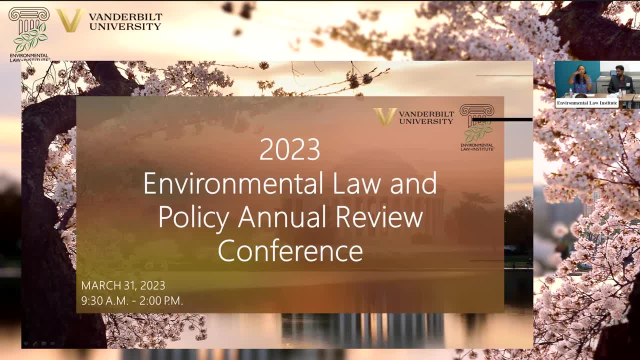 profits and some of that you will start to see the algorithms are building that in. um, we would argue you don't have to actually be understand, code and write if you can understand the training data, which is all the information that's historically available, goes into the algorithm and you look at the outputs. you can tell what the impact in the 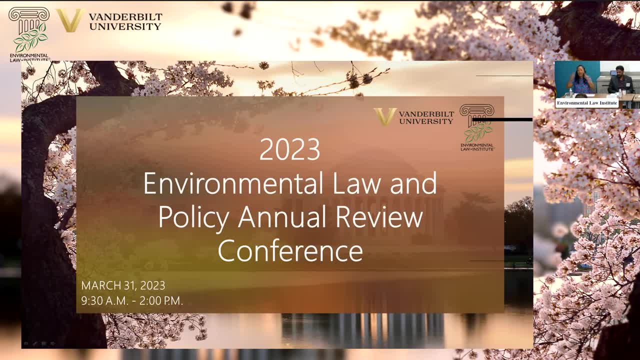 black boxes and we can say: look, this is what's going in, here's what's coming out, modify what's happening in the box, right, so? so then you can keep the IP, all the laws around, uh, the? um, intellectual property and all of that um. so what? we're also seeing that the? um the tools and 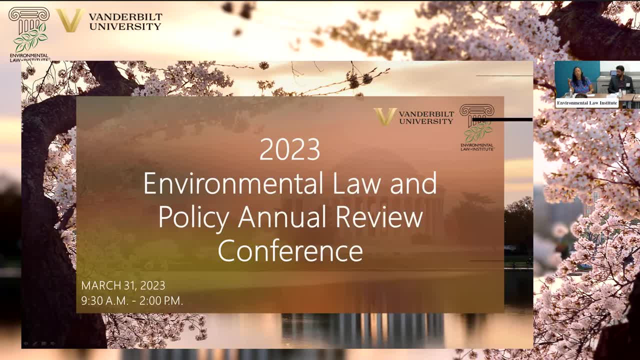 the models are becoming more evident because the problems are so complex. so if you have all the environmental information from all the satellites and, uh, the noaa, which we've been working with Noah on the data that they capture in the oceans, that's a huge database, right. but it allows me to see what 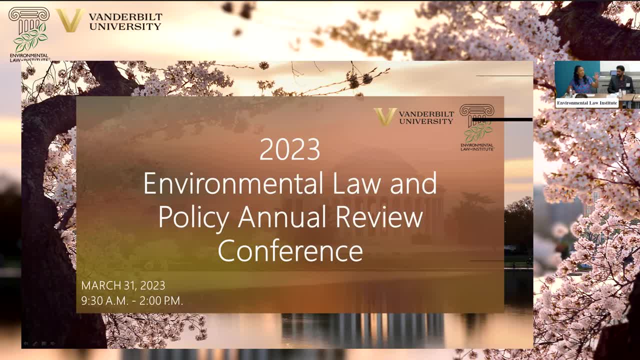 the weather is going to be in six days. and then you take all the economic data from the census facts, from um, both the you know income, um, even resume. if you take all that economic data. and then you take the social determinants of health, so now you take all the health outcomes that come. 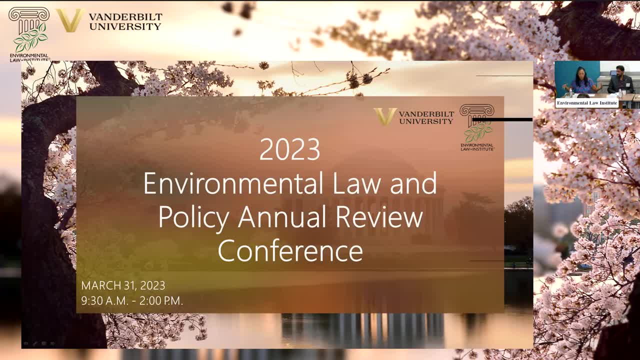 from. that's a lot of data and there and there we are now using all that data to help us make decisions right, and so the the further we get from um what the decision makers are- so that needs to have diversity inclusion- then the the less likely we are to understand those um decision-making tools and 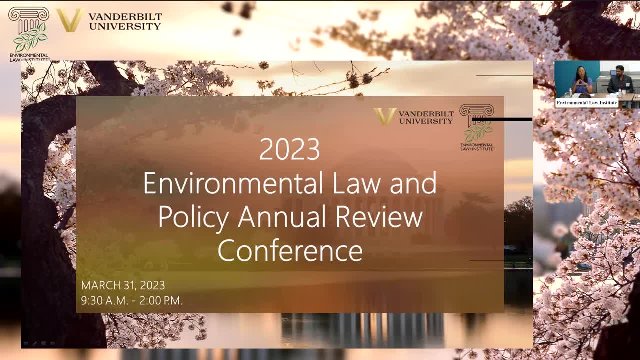 so, again, when we look at it, we do see now that the tools, the algorithms are actually producing a new frontier of redlining. so we have started to see the patterns. we look at, we take the uh, the outcomes of the decision. if it's water, this energy transportation, uh, we, you know I'm in DC um to work. 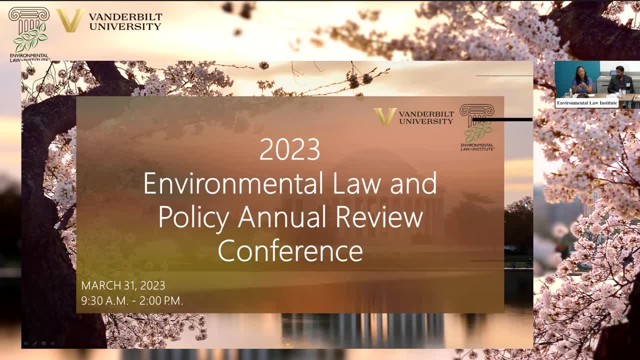 we've worked with deal ddot, Noah, Treasury, EPA, on talking about what does it look like, what's the impact on communities of color, in low income communities? and we're seeing this pattern because the data, the training data, takes all that historical decision making and just puts it into and moves it forward. so we 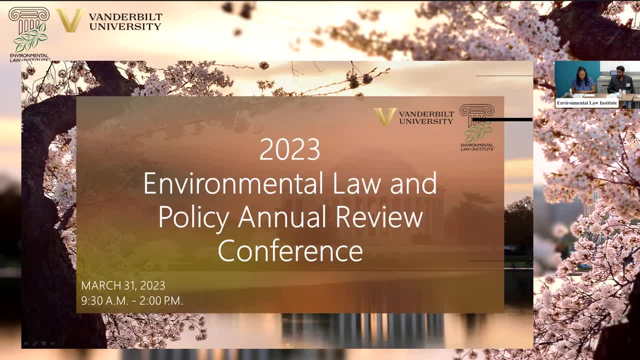 have to change the way that the, the input comes in. and the other part that's emerging as well is for us is um, you know the fintech. so the fight, the way that we are doing the capital markets are working and the way that we are using resources- i mean, i haven't been to a bank and i don't know. 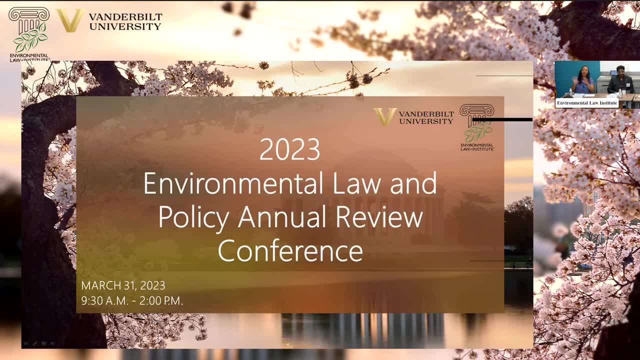 how long? right, and you just do it all digitally. but that's also creating disparate impacts for those who don't now have broadband or don't have access or don't have the devices. they're being left behind, which means the data of their usage is also not included. right, so it all starts to if 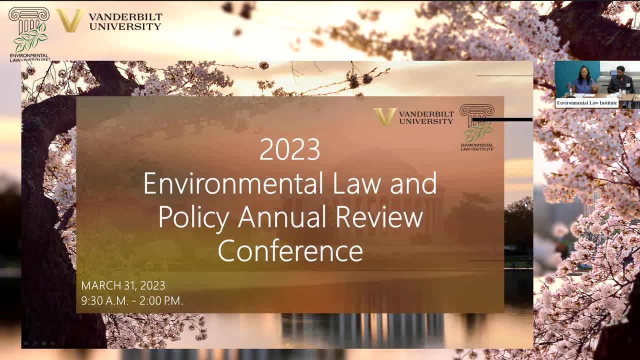 if you start to think about, like algorithms, and the modeling that it encompasses your whole of life. it's not just that we're talking. you know, yes, the environment that you live in, but it's also the economics and it's also the place that you live um. so we're seeing the technology being 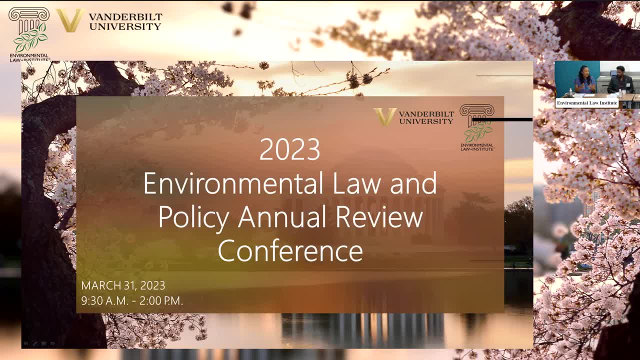 captured in all kinds of of ways. now the to the to the plus side, um, we see all of these gis. so these geographical information systems, these gs map, gis, mapping maps all over the destination areas, are cent swe. Subscribe to our channel so that you can. 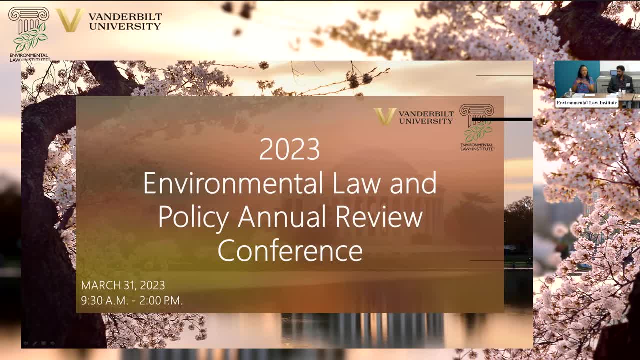 learn more about all of these great organizations. so have a great rest of the day. thanks for watching starred electricity. lllo can see a community that is bright orange because it has disparate impact and disparate treatment under the law. that has now has an opportunity to be centered and changed um the tools that i would 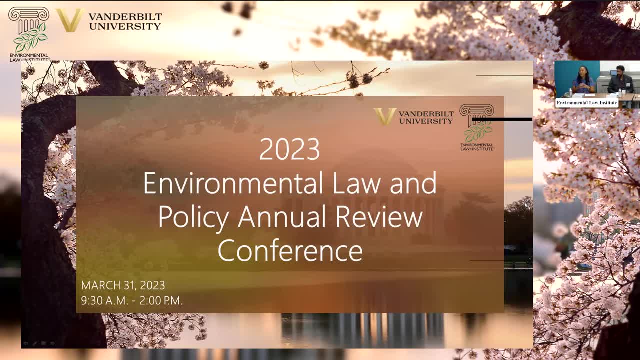 point to. so in california years ago we did a thing called uh. we have a tool- you can, those of you who have access um- called cal enviro- screen right 22 indicators where you have the social determinants of health of a community. so that's asthma, heart disease, and they take those indicators and they 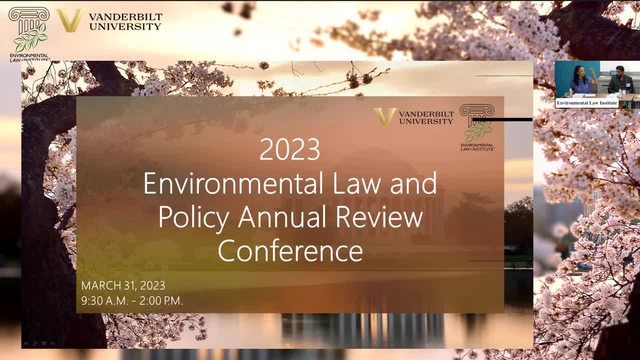 and then we do the climate side. so that's, you know our blood zones are, we have extreme heat, wildfire, uh, and then we put that on a map. so in california we use that tool to help us with policy making and resource distribution and we have been working with on the federal level on a 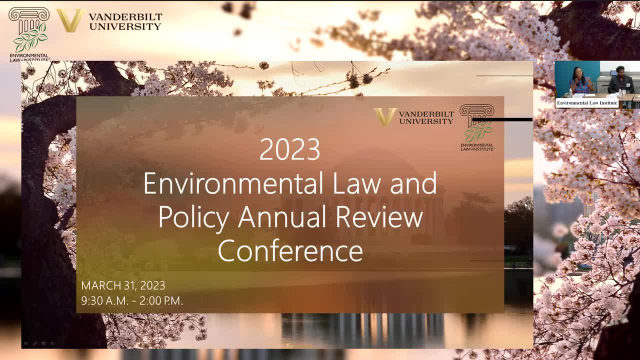 for the epa called c, just so um, c just has that same tool. and again, because we were like what's the bias in the data? what's the training data? run it through the, the box and what comes out on the other end, it was so highly correlated with 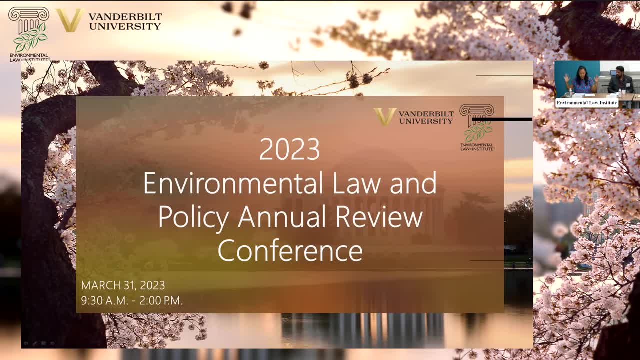 grace. it was just crazy, because you're like we didn't. you know, the decision makers weren't like let's do something that's, you know, race neutral. oh, they were like this is the fair thing to do, this is the right thing to do, and yet it all came out race biased. and so then we say okay, so how do? 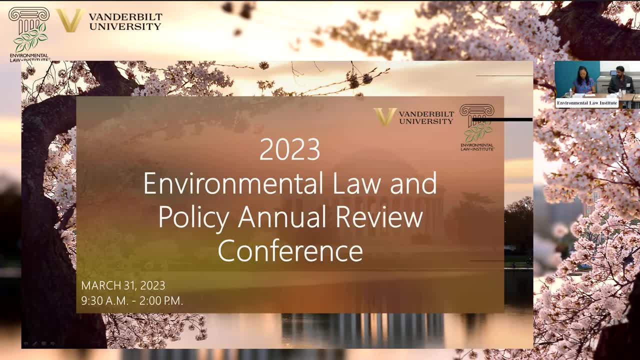 you correct that, or how do we at least create something that is more neutral until we get them to some solutions, um, and- and i wanted i got about a minute here, okay, so, uh, solutions then as we see them. procedural equity is also was brought up, so that, uh, we would lift that up. meaningful participation. 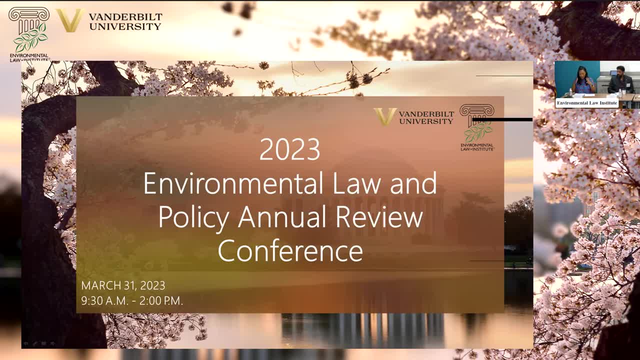 um, at the front end, um, and in the middle and at the back end, transparency. there's a complete lack of transparency, uh, a lack of future engagement. so even let's just you'll see, just, dk, okay, thanks, thanks, um that um, even when we made comments and recommendations and and in the 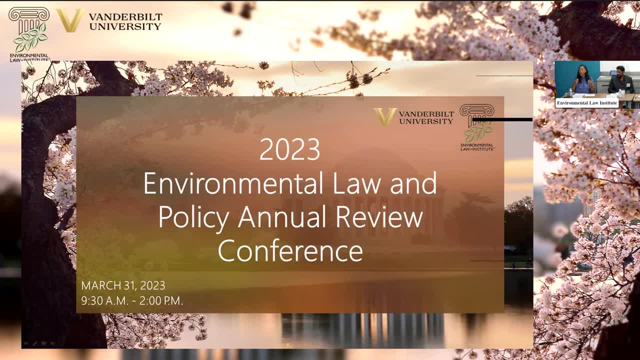 djust model. there were over 2600 comments. we don't know which ones they took, like okay, which ones did you take? and then then it'll go through. and then it's like, well, we have another chance to comment. so there's the um, the lack of future participation, and then the diversity in the decision makers as a 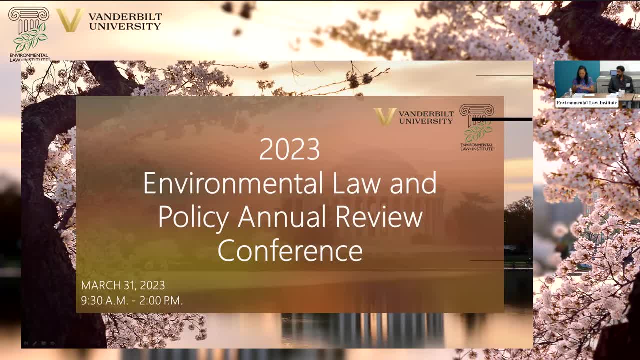 as I mentioned, And then you have to publish. The transparency comes from publishing, So publish the impacts you heard before, publish the risks and then what are the critical decision-making points that need to happen. So I'll pause there. I know I brought a lot of different perspectives. 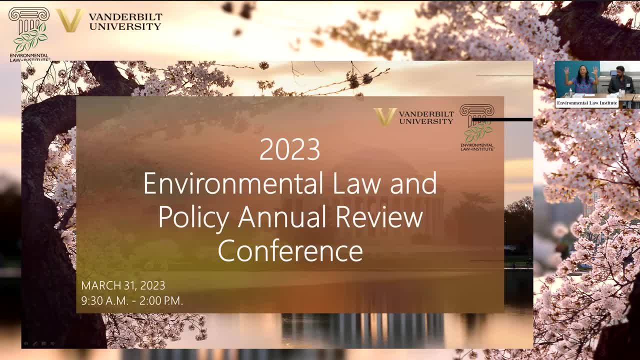 but I think if you can think of the landscape of algorithms and how pervasive and pernicious it is, it'll help you then analyze. you know, even the four-degree conversation that was had earlier and then there's going to be an ESG conversation. That sort of perspective will help you. 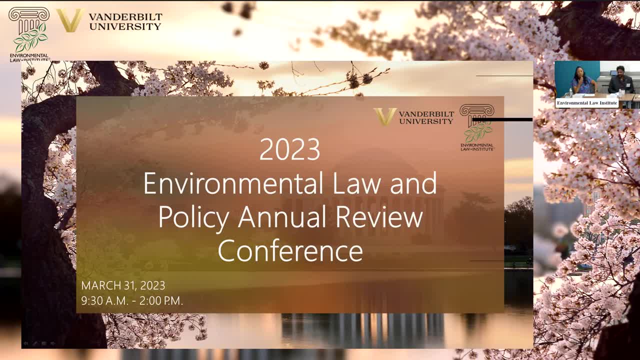 I think you know, create the laws and policies that we think will be most effective. Thank you, Deborah, and thank you for sort of trying to tie it all together. I want to give you a chance to respond to comments you heard, and then we're going to go to Tasia for the first. 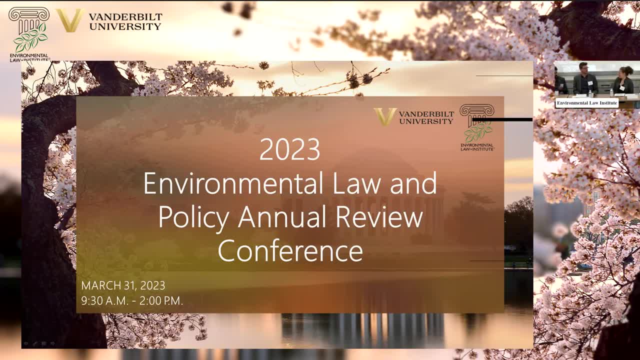 question: Great. So first of all, thank you everyone for the time that you put into this. I'm learning so much from all three of you. so thank you for being here, Deborah. thank you, too, for starting out with Cesar Chavez. I think that's really important. There's actually a good 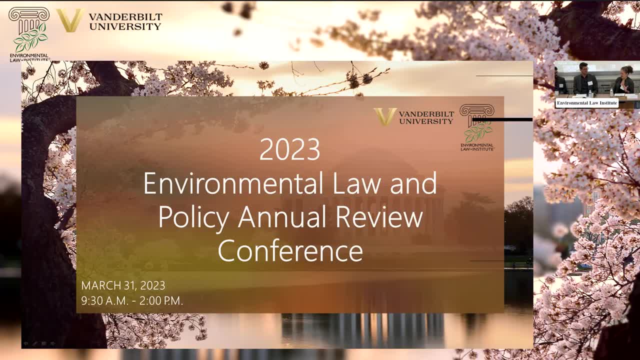 tie-in here, because what I've heard from all three of you in different forums is kind of questions about who's carrying the burden and what kinds of investments are we willing to make in terms of time and money. One of the you know kind of pernicious. 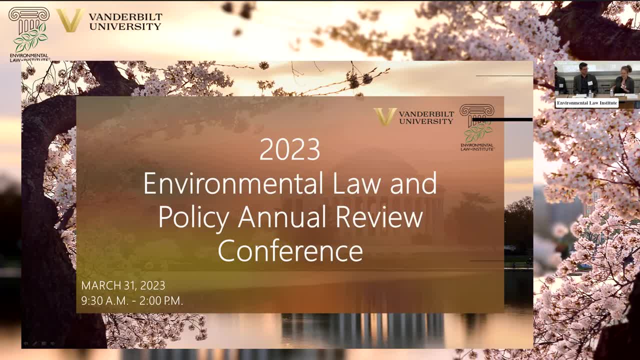 and kind of academic, it's like, not too interested in this, but from a practitioner standpoint it's really important. PUCs across the country, which you know like regulate energy utilities and are responsible in part for their transformation, don't have enough staff. 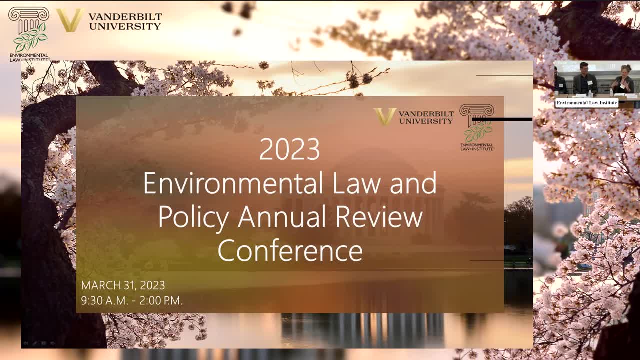 Like they lose their staff all the time. Governments lose staff all the time, so the people who we need to be working on these things aren't there And in in place of that. you know, like you were saying in Nebraska, right, like people end up relying on. 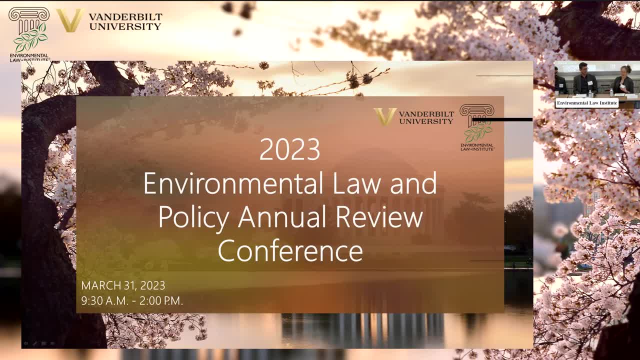 computer programs rather than staffing, And so there is kind of a labor tie-in to like how what are we willing to spend money on in order to create the kind of system in order to solve these problems? Okay, that's a little bit of an aside, but I was so glad that you brought that up. 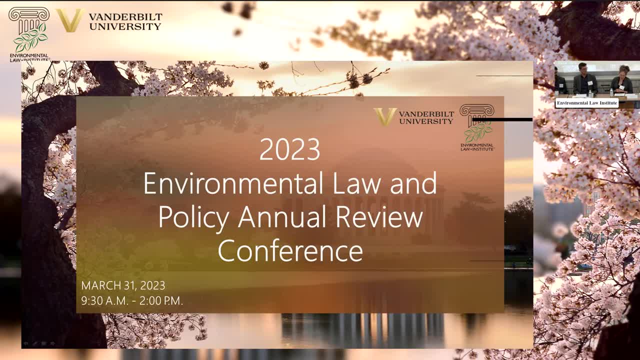 so, thank you. Investment in time, I think, and burdens are also important. when you're thinking about sharing, should we place the burden on marginalized communities, who, by definition, are already marginalized and already, you know like, have other things to do, to put an additional effort. 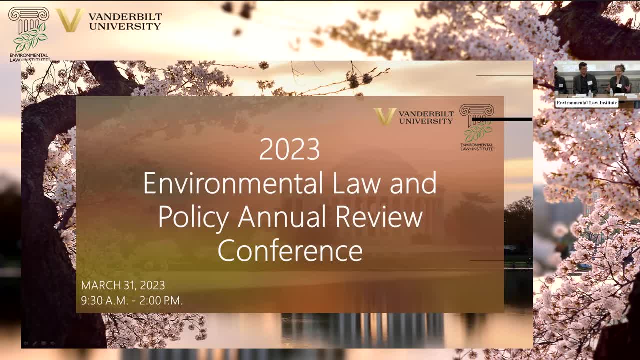 to understanding, you know, like, how hydropower modeling works. Is that really fair? What do we need to do to engage those communities and at what point do we do that? I think is a really important question that I have not answered. 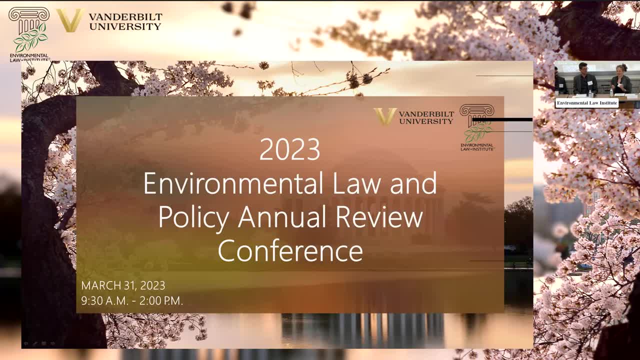 And then there's another flip side to that, which is we don't have a lot of time to adapt to climate change or to mitigate climate change like. all of this needs to happen really quickly. Public participation takes a lot of time, So doing this in an efficacious way is something, I think, that 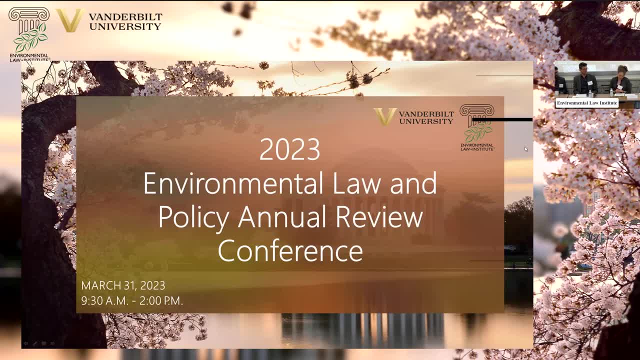 also needs to be worked out too. Mohit, I really am enjoying your application of a new framework to Garry Kasparov, But I think actually your suggestions are practical and it fits a lot with what both Keith and Deborah said. 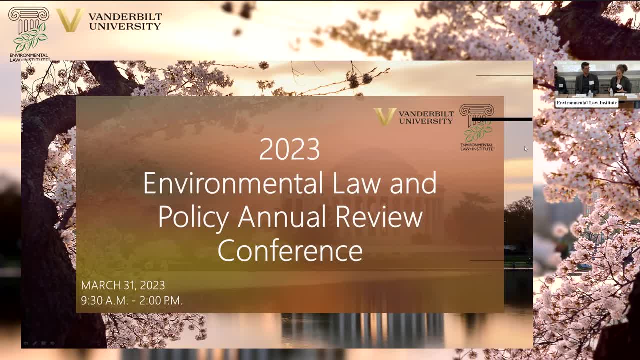 So, Deborah, you know you pointed out the importance of understanding and training data. That is a huge focus. I think that fits nicely into Mohit's. you know key parameters, But I think the geographic scope that you brought up as well is also pretty key and may also fit into what Greenlining does. also, in terms of where are you kind of? 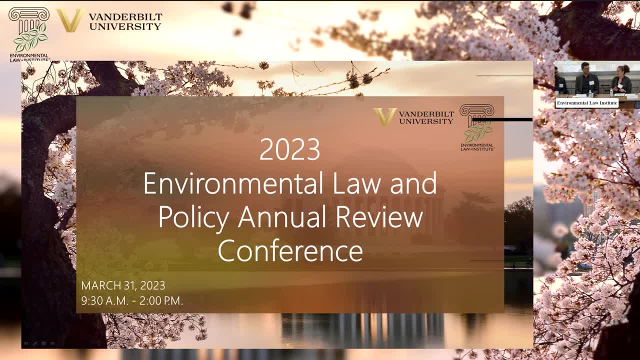 trying to make those boundary decisions, And that's where I think my initial framework might come in a little bit too. Yeah, you all brought up way more than I could address in five minutes, So I think I'll keep my comments there, but I'm looking forward to continuing discussions. 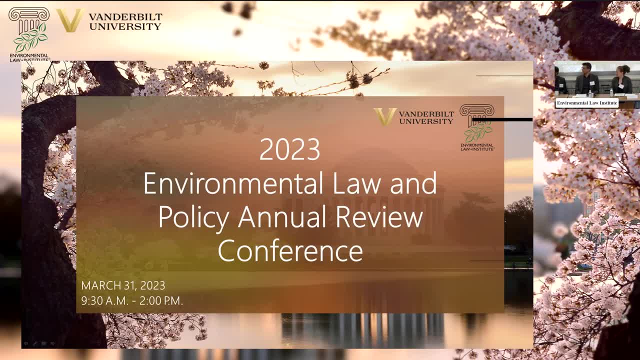 Thank you, Tassia. do you want to pose the first question? Sure, And I think the discussion has started a little bit already, but my first question was about that question of burden, Because it seems like your article does a really great job. 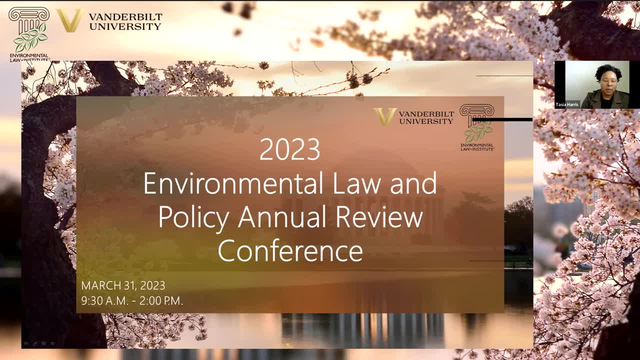 Yeah, Yeah, I think it's been a really great job presenting the framework as helpful for both developers of these tools and then advocacy groups or impacted groups that might want to evaluate them afterwards. But the ideal situation would be, it seems like, for the developers to kind of engage in this inquiry as they're creating these tools. 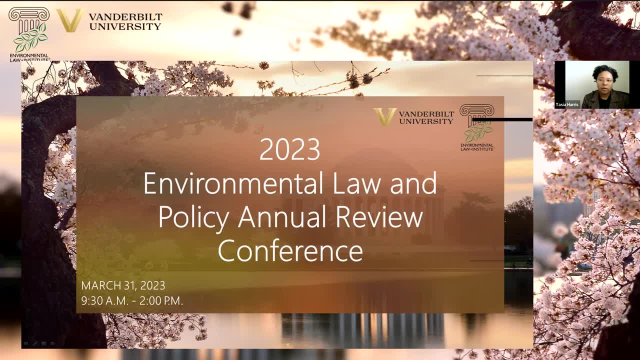 So I was wondering if you know you all could talk more about what you see as the incentives or paths towards getting developers to do this work proactively, Knowing that there may be some kinds of evaluations that are always helpful to have on the back end, but just how do we get to having this happen on the front end? 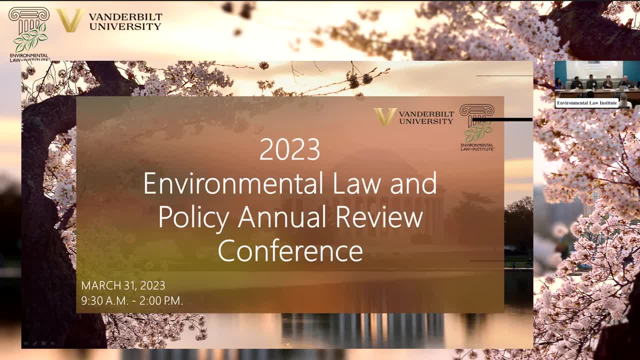 So I'll take that question first, if you all don't mind. If you look at the engineering and engineering and social science literature, there's quite a lot of work being done on this. Like this has been a known problem for decades. 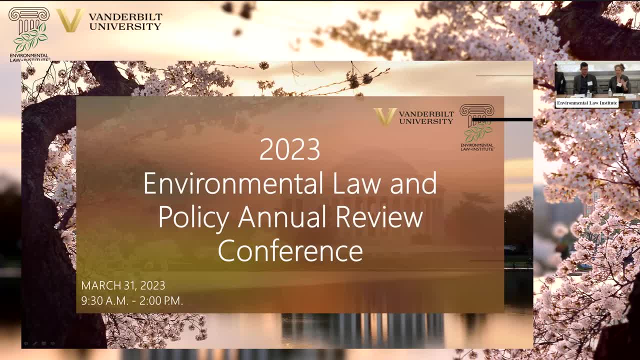 And there's a lot of research particularly about getting end users To be more helpful earlier on. That said, I think that there's some important things about keeping developers siloed at times, And I don't want to lose sight of that. 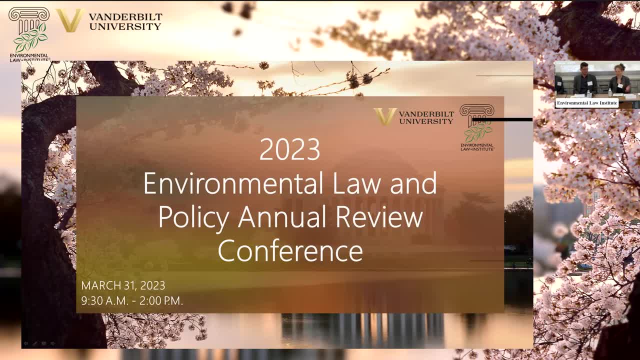 Because it takes some creativity and it takes a lot of technical expertise And it's during those initial kind of stages where they can kind of get traction. So it's easy to get muddied down If you don't already kind of have an initial idea. 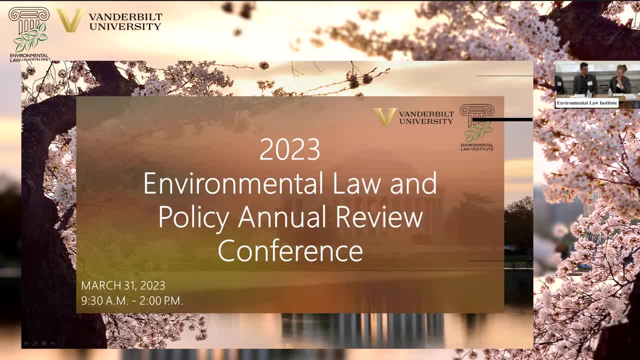 So there's kind of a timing problem there. But in terms of incentives, you know government has a lot of incentives. It's great for developers. if a government decides to adopt their model, That's a really good contract. Then they can take it elsewhere and say: look, this amazing jurisdiction is using this. 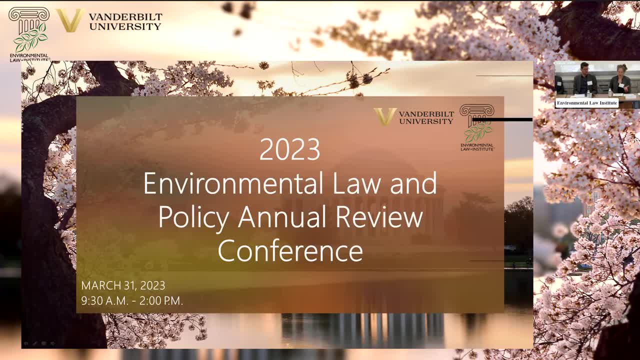 So this happened with Resolve, which is one of the models that I talked about in my paper. You know a model that they developed, I think, for California- The first moment might know this better- Also used in Hawaii and other states as well. 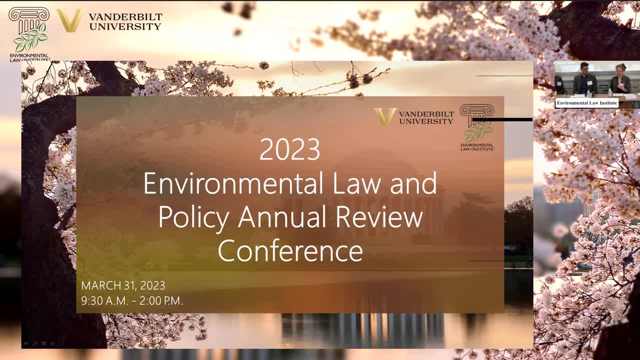 And so, by having that initial contract, there are incentives that you can put in place, Or even just rules about: look, we're going to have workshops to figure out how to do this And, you know, include people in this earlier. 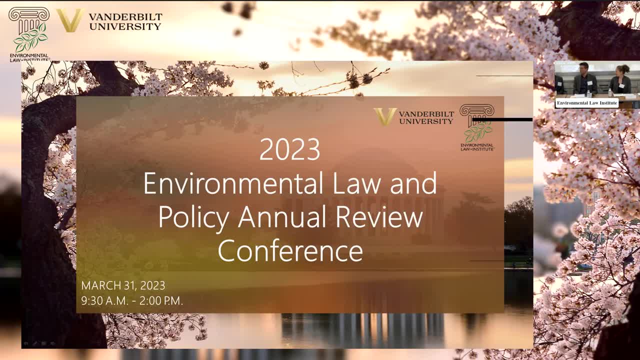 So those are my initial thoughts, Yeah, okay, So I definitely have some thoughts. So the academy is really jumping in. So we, you know, we sit right between UC Berkeley and Stanford, So we have two real big sort of think tanks. 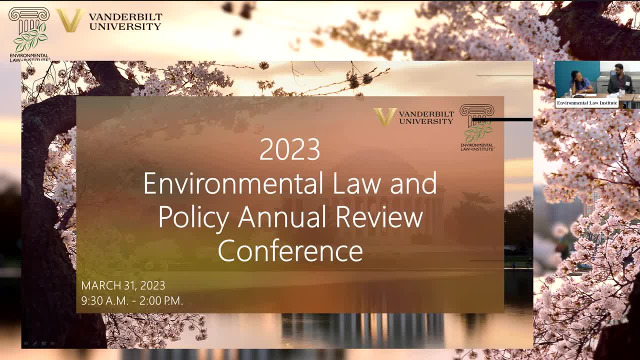 So Berkeley, we participated. They're submitting for I think it's the EPA grant of the hydrogen hub. So they're going to do $6 to $7 billion hydrogen hubs. So some innovation and creativity on the development side is going to be coming through. 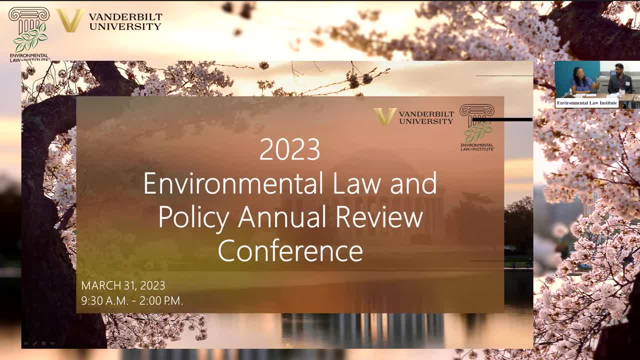 To help facilitate that. Then you know, down at Stanford they just stood up a sustainability school. The question is, how much does it cost to stand up a sustainability school? It's like $1.7 billion, But they just stood it up. 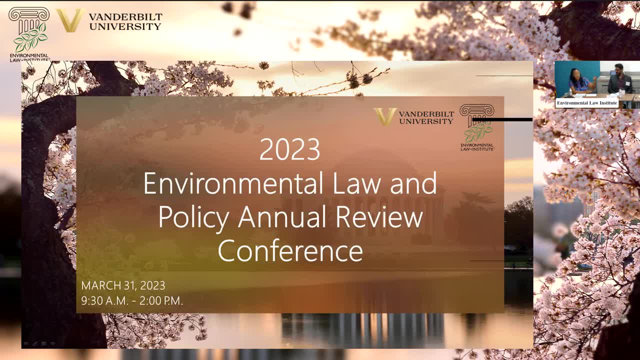 And the venture capital is being incentivized by the IJA and the IRA- You guys know these acronyms by now- Because the public funds and the production tax credit right back to profits and losses privatized, and public Production tax credit, investment tax credits are significant enough to make those projects pencil now. 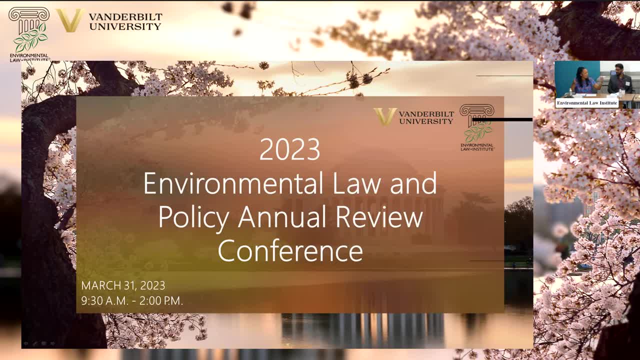 So you've got the public dollars coming in with the private dollars to incentivize the market in big ways that are very innovative, And you know you have it both at a public institution and a private institution. So I'm sort of really hopeful that we will be able to activate some innovation around the energy that we need. 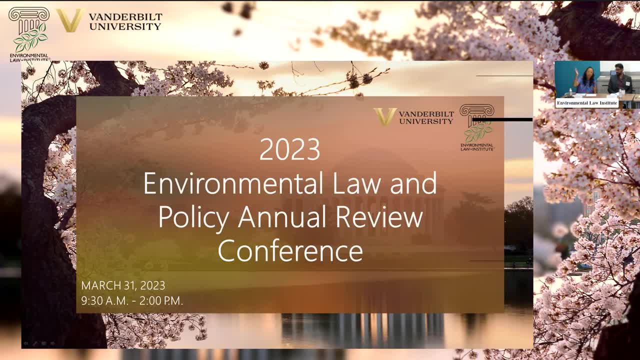 I think from you know the hydrogen, all rainbow colors of that to wind farms. We have big wind farms off the northern coast of California, So I think there is incentive there now And then it's just some creativity that needs to take place. 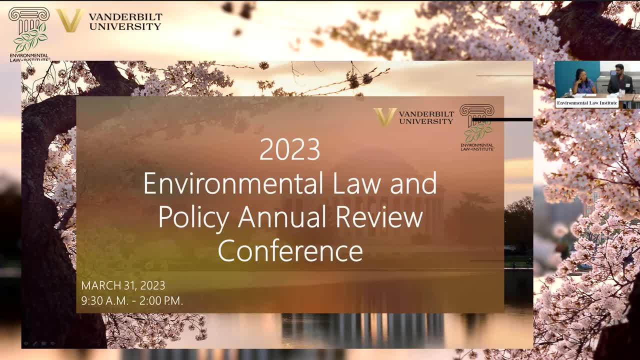 And then risk. It's a risk-reward kind of profile, But I'm encouraged about innovation. I'll add something to this. So I think a fair amount about what Sonia said. What's the right balance between engaging versus burdening? Folks have a lot going on in their lives and participating in deep technical conversations may or may not be the best use of their time. 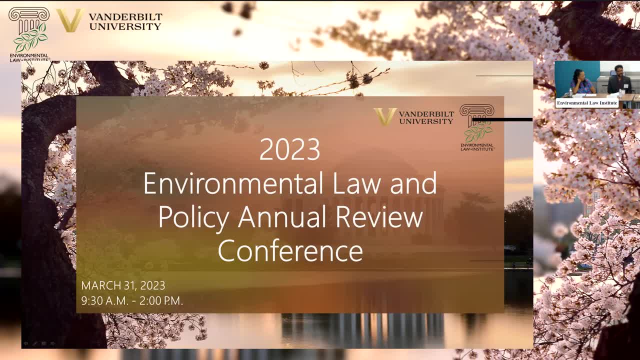 So I think, at a minimum, what developers, regulators can do is understand needs of communities in relation to what they're working on, And if they do that right Over time, people will see the outcomes of processes, Because there's no real substitute for trust. 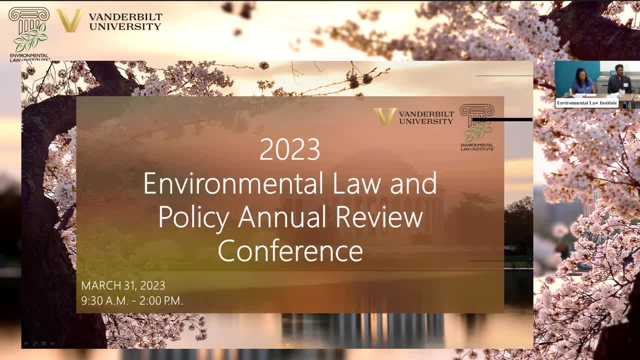 In today's political environment there is a lot of broken trust, So folks want to participate everywhere to make sure things are going right. But that's not sustainable over the long term And one way I've been thinking of getting out of that is really understanding needs in relation to what you're working with. 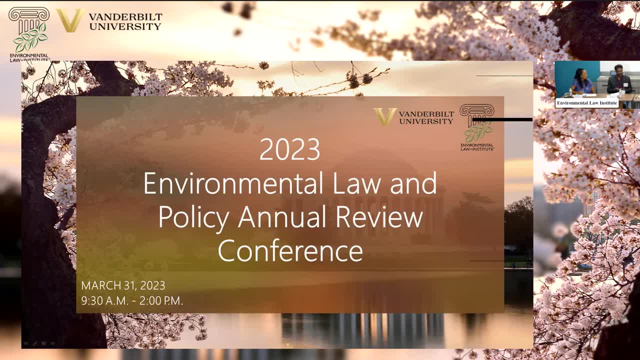 And how they would impact communities, integrating that and, over time, building that trust. But I don't see a better way to do that. But if you do tell me about it, I'll just give a quick thought on that, which is less an answer than a question that I have and one of the things that I'm working on. 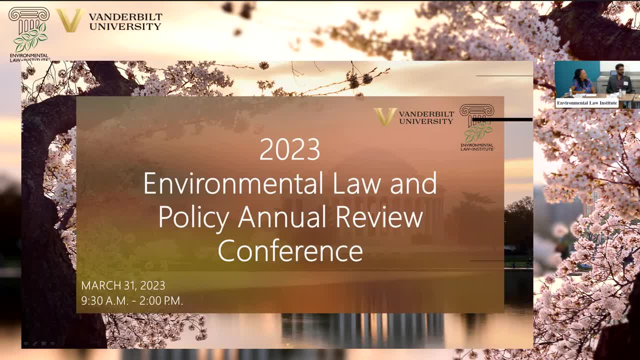 So in the government processes, in the public processes, regulations go out for comment or a new tool goes out And it's sort of this public comment period. That's one way where the public engages and to try to It's entities like Greenlining Institute or NRDC, that kind of the public writ large relies on to represent the sort of non-directly commercial interests. 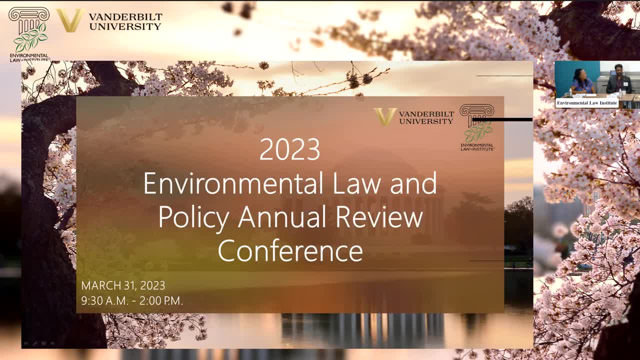 Right, Whether it's environmental values generally or representing disadvantaged communities, to sort of get their input into the process. One of the things that we'll be doing at the Department of Energy over the next 10 years, as you mentioned one, is like sort of hydrogen hubs. 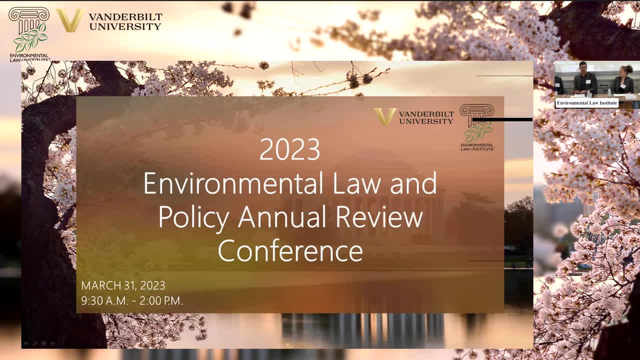 There's like $100 billion of grant programs and then another $200 or $300 billion of loans that are authorized to try to build out the infrastructure to help accelerate the energy transition. And one of the things that I've been thinking a lot about and trying to talk to colleagues about is figuring out for those reviews of individual projects. 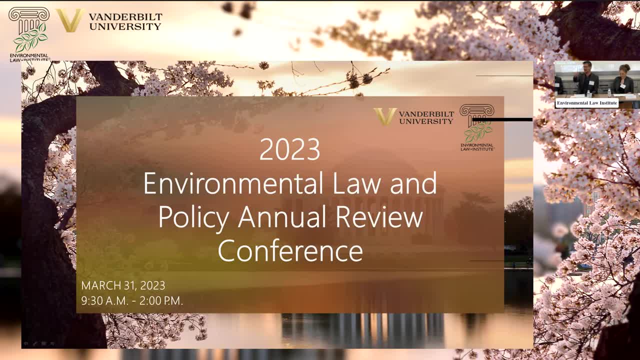 You know the hydrogen hubs that's going to go somewhere on the outskirts of Palo Alto or in Oakland, where we used to have refineries, or you know wherever they're going to go. How do we improve the participation of the people directly affected, of the disadvantaged communities, without it being burdening? 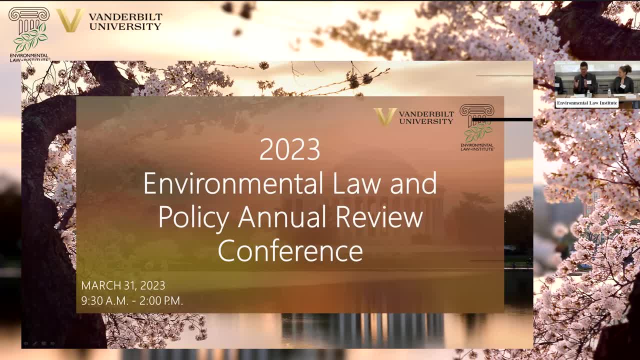 And how do we make sure that those people in that area that will get those some benefits and a lot of burdens Are, in fact, able to get there Right Again, that is something that we're working on, And so we're working on looking at how to make sure that every person who you know is working on a project in the environment from a further perspective doesn't get hurt or affected. 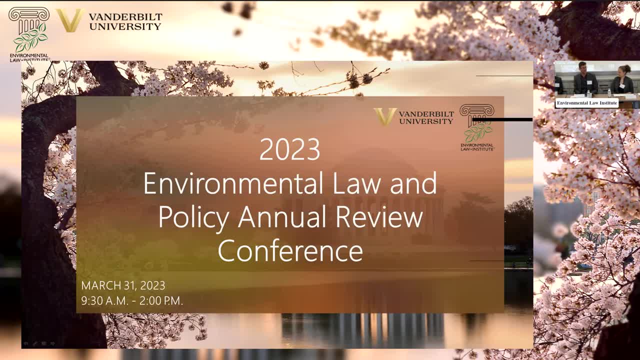 Or that their voice is heard, whether it's via better engagement with existing NGOs or directly into the process, But sort of closing that I don't know that. that particular part of it on the specific ones is. and, again, if people have good ideas of how to do that, I would love to hear them because we're in the process of focusing on that and building that out now. 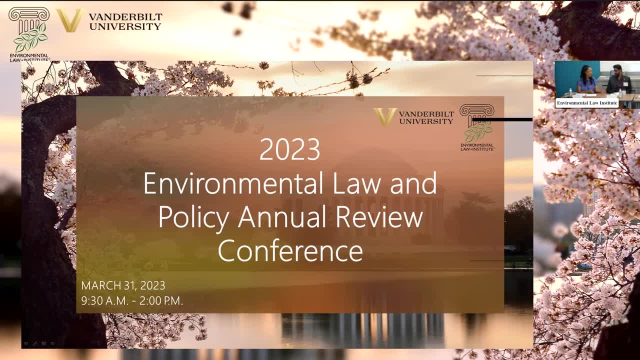 And I know you're over time, but I think that's what the Justice40 is trying to do: benefits, not the investment. 40% of the benefits go to disadvantaged communities And so that's to say, if you respond to an RFP. 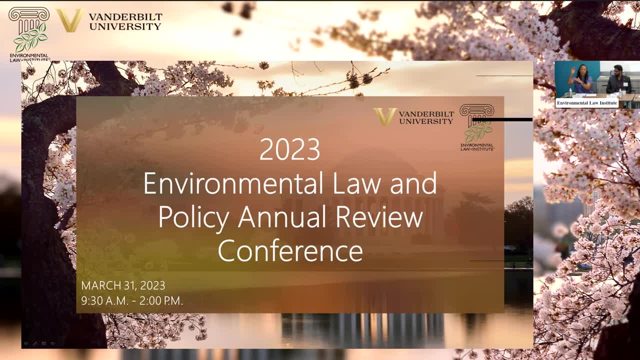 you will get points of credit for how well you address Justice 40. So that can sort of No, no, no. that also gets us into the question of the algorithms and also making facts transparent, And I'm talking about that additional piece. 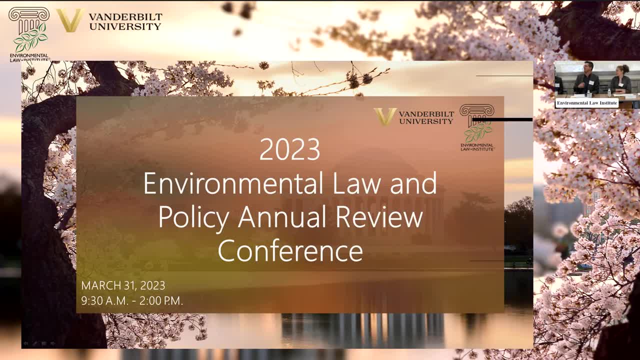 of that, of making sure that we're valuing the things that would be valued by those people in that particular area and that it's not just the product of an algorithm. But anyway, sorry, No, no, we're running a little bit over again. 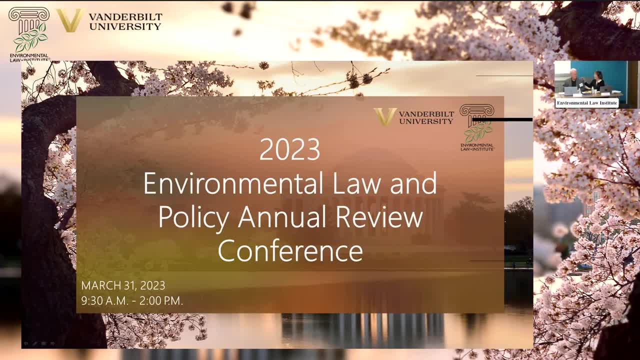 like note to self. we need more time for these panels. Does anyone? I know Mike has a burning question. I have a question, but does anyone in the audience want to respond to anything they've heard? Question that I come to And I'm going to repeat. so the webinar hears: 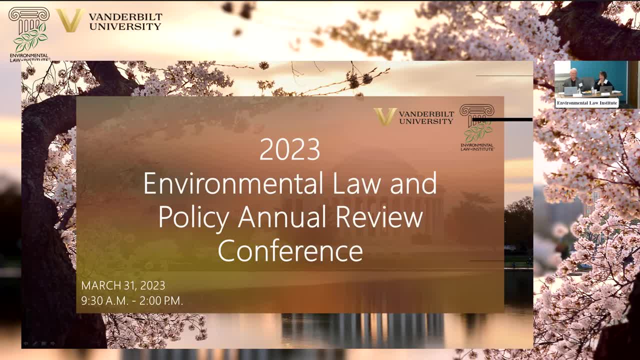 I'm going to have to repeat what you say so the webinar hears. That could be a problem. So a question that I come to With this panel is: Sonia, I really appreciate your point about transparency of the algorithm, And that really impacts what I'm thinking today. 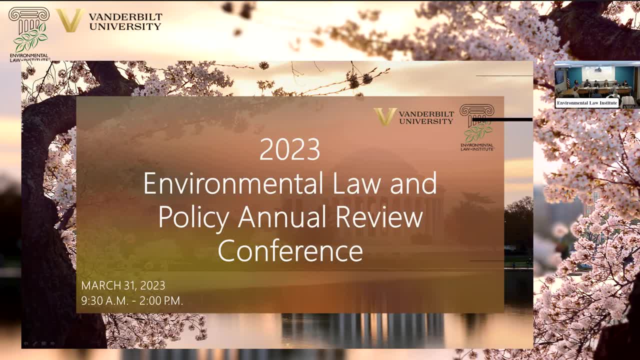 But, Keith, you sort of touched on a question in my mind is: is the real problem the data? Are the algorithms, pretty much faultless, in the process of bad outcomes? Is the input data the real problem, the source of the problem? And if that's true, how do you regulate that? 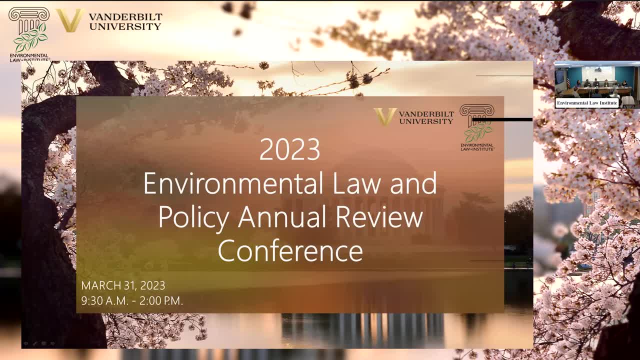 Is there something like an for the health of input data to algorithms? I have a very I'll try to be a quick answer. I mean, I think the answer is that it is both actually So we need to be aware of the possible biases in the algorithm. 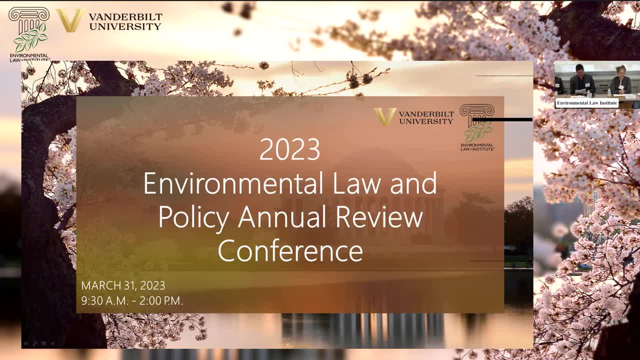 And I think that's a really good question, Thank you. Thank you, And I think that's a really good question. I don't think the answer is based on the algorithm at all- Chat GPT. so when I asked that, how do I know your answers are not biased? 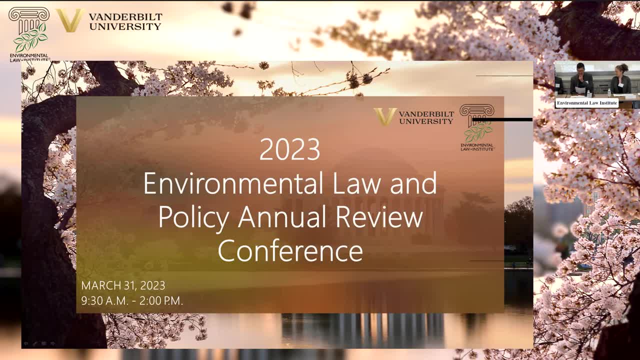 said, as an AI language model, I do not have personal beliefs or biases. My responses are generated based on patterns and associations learned from a large corpus of text data. However, the accuracy and relevance may depend on quality data used to train me, as well as the phrasing and specificity. 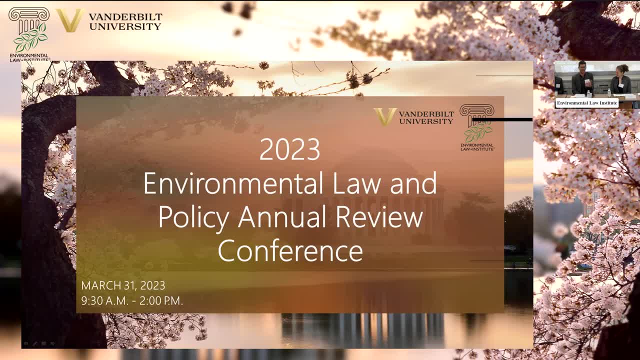 I would actually say that would take issue with chat GPT there of even saying that the response does not have biases. language that it is trained on has underlying biases in it. it's still going to be reflected in there And so. but I think the quick answer is that it's we need to be aware and mindful of both. 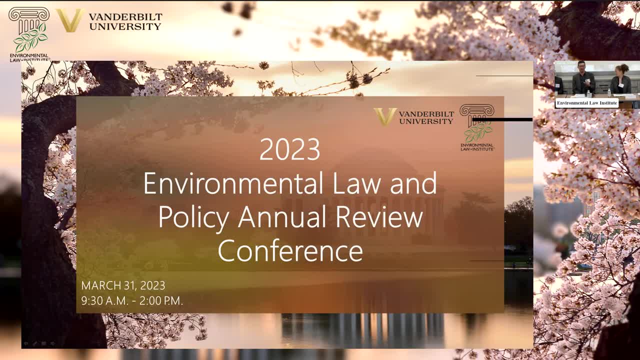 and we need to engage a wider variety of people into the development of these to help spot and uncover where those biases might be that might not be spotted, if it's just So, in the model development that's done. you know, for a lot of like the federal energy models, the Energy 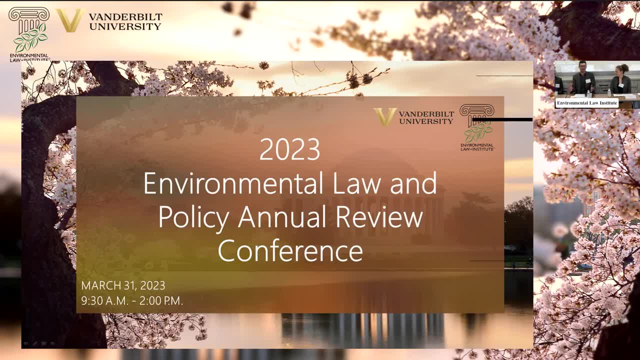 Information Administration that does the energy outlooks every other year has a big national energy modeling system model. You referenced it in the in your article that this is. you know Congress and the Inflation Reduction Act said: hey, build more integrated damages assessments. 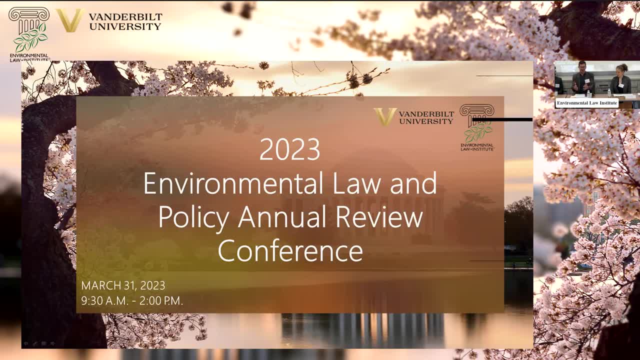 into this as well. So that model by rule is required to be is required to be public and publicly available. like any of us- any of us. I've looked at the systems requirements. anybody with a Windows 8 computer can go and download the National Energy System. 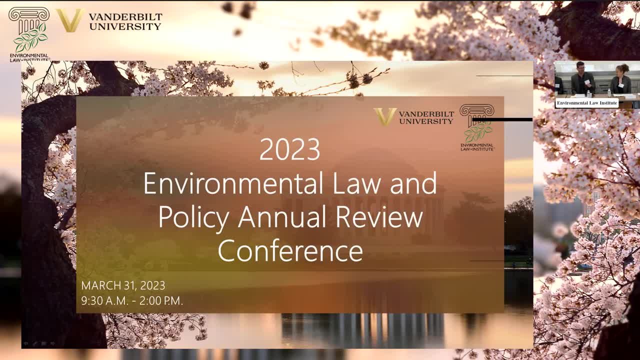 energy modeling system and download a little bit of proprietary software and run the basic case And there are companies who've downloaded it and modified it. So in that sense it's transparent. but when we develop it it's still developed and the review goes with a bunch of energy modelers. 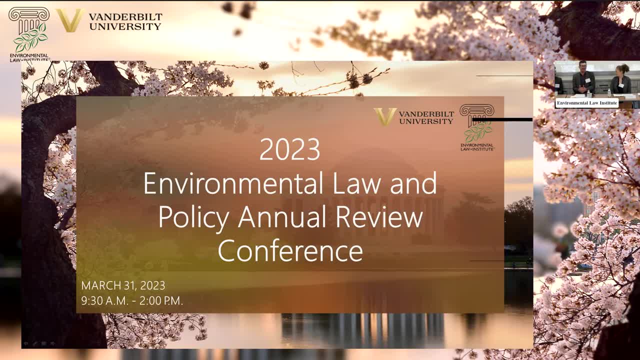 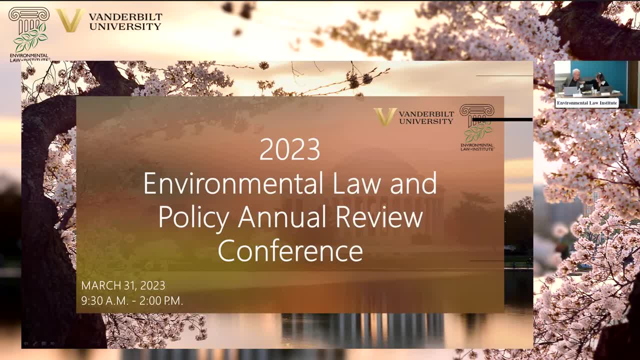 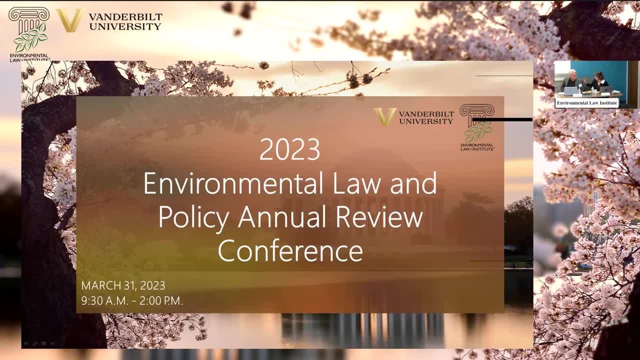 right with you guys, And I know you want to say one thing in closing, but before you do, I'm just going to say lunch is going to be available The other room. grab a box. We're only taking a 10 minute break again, So take more time if you need it, but come back with your box. lunch webinar. 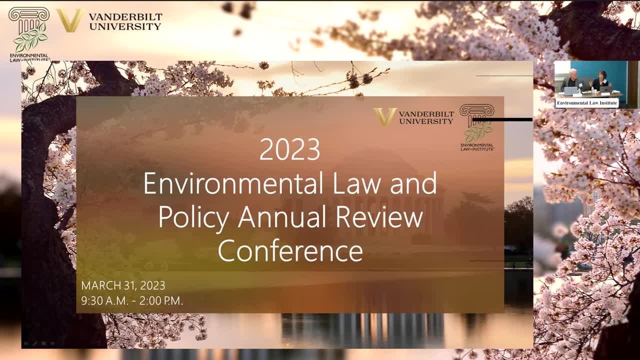 folks. Sorry, It turns out when you start a webinar, you cannot stop a webinar, So you're going to hear what's going on unless you mute the audio. We're going to take some pictures of the sandwiches for our virtual audience, So I'm going to just to raise a question Again- we are in a partially academic setting- and see if 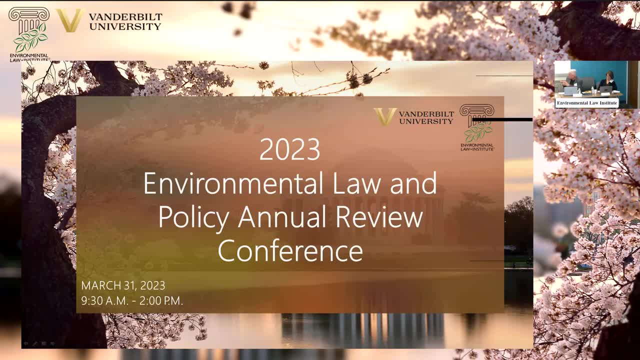 we can take it to one more level And my question draws on your overall thesis, I think, and part of what Keith talked about in terms of transmission And I think part also what Malik talked about in terms of discount rates, and then ultimately Debra your overall thesis And that is for the 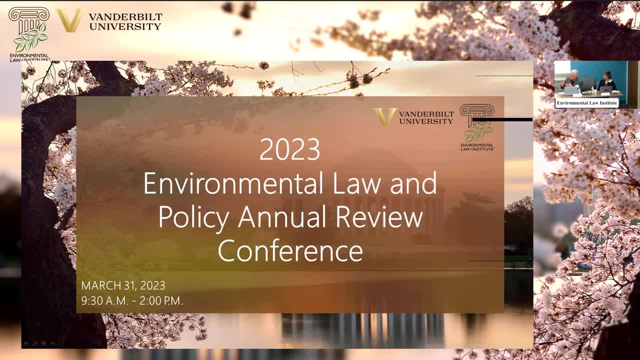 job, And I think part also is for the co-pilot to be informed as well. right, We all have to make the same decision. When you think about what is already possible for any of us, I think that we're going to be making decisions that are going to be. 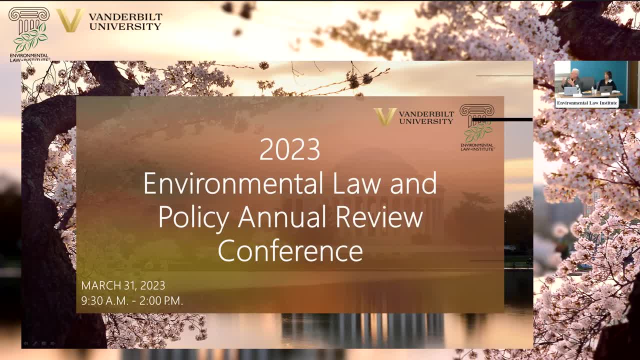 more actionable, that are very realistic where we want to be. The other thing that is also going to be the understanding of how we operate ourselves. A substantial amount of the carbon we released today will still be warming the planet 500 generations from now, And that means that the disadvantaged communities that will be farmed today also will be the descendants of those disadvantaged communities, will be farmed for 500 generations, And yet we tend to talk about justice and equity as if it's all in this generation. So I'm curious about how the algorithms or the underlying data can be dealt with to account for the idea that we have a 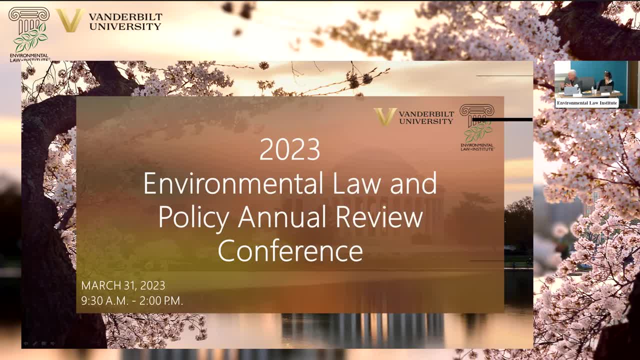 multi-generational problem at work here- And that may be one of the biggest injustices we face- is that the most disadvantaged communities- offspring- are going to be the most disadvantaged by climate. I'll give you a quick example that relates to Mohit's point: An environmental 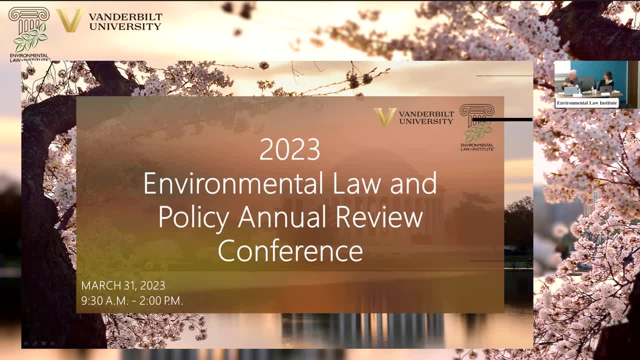 economist a little over a decade ago said that the entire economic value of the planet in 200 years, using the then recommended OMB discount rate, would be valued at about $10 billion today. So a pure cost-benefit analysis: you wouldn't spend $10 billion plus $1 to save all the economic. 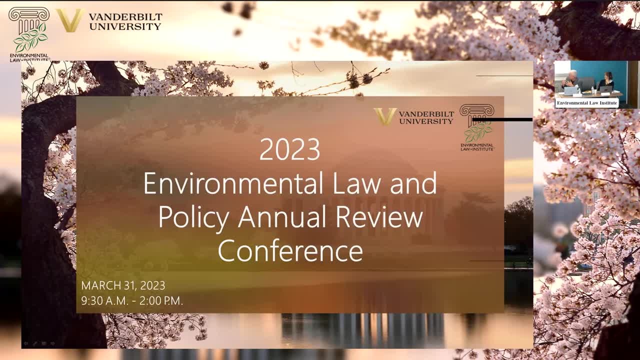 value of the planet in 200 years. It just tells us how much are kind of. what seems like a neutral value can also have an intergenerational justice question. Are people already thinking and writing about that? Are those issues implicated in what you do, Or how should we all think about the? 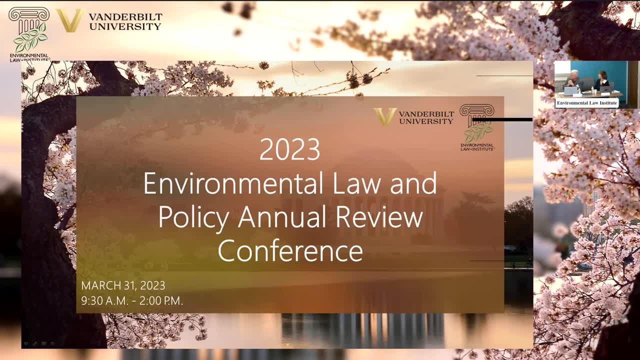 intergenerational as well as the intra-generational question. I'll take a first swing at it. So your question really is about a choice. I think of it as the intersectional choice of values. How much do you value future impacts versus today's impacts And an economic question? 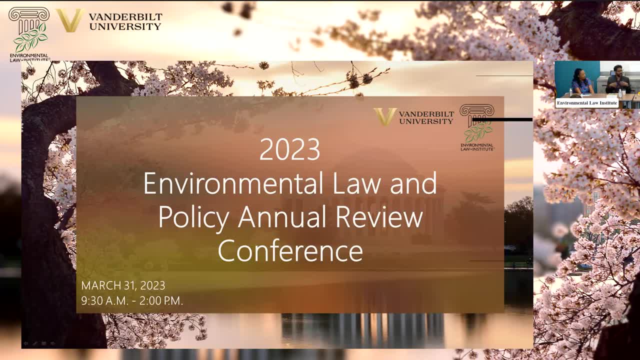 given our limited resources and funds today, how much should we work to say- I used to live in Oakland- how much money should go to hunger and housing versus climate change? that would impact people- a few hundred, So- Okay. I think all I'm reflecting is that you're really asking a political question And 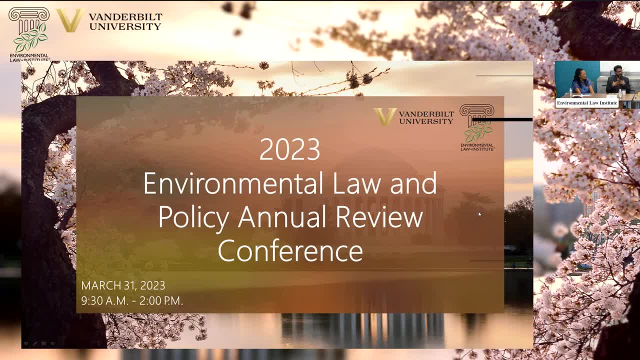 that algorithms can take that answer and use that as an input and give you a recommended solution. But that really is a central political question And I don't know what else to say about that, So I'll take a little bit. There's one on the question of thinking about it and writing about. 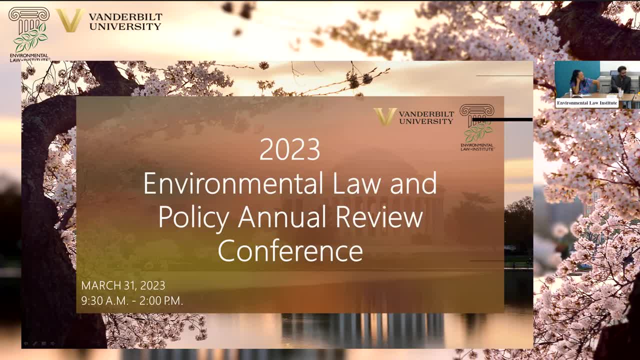 it. I think that's a fantastic wealth of writing in the economic space and the climate space of trying to tease that out. That's addressing it two ways. The one is the political, policy, moral question of how much do we put the value on the damages later in time. The other one is a factual, 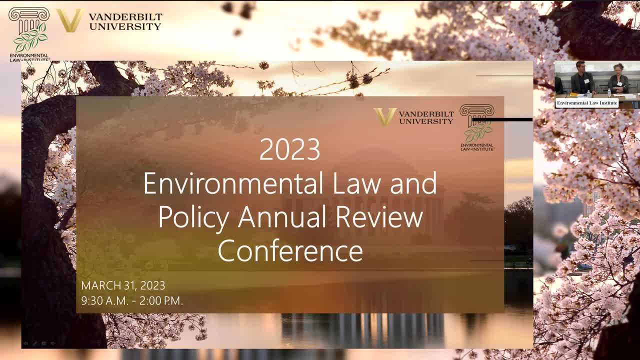 question of what information do we have about how people actually do value things? We don't have many markets for- Yeah, Actions that happen 100 years in the future, much less 200 years in the future, but we do have some things. 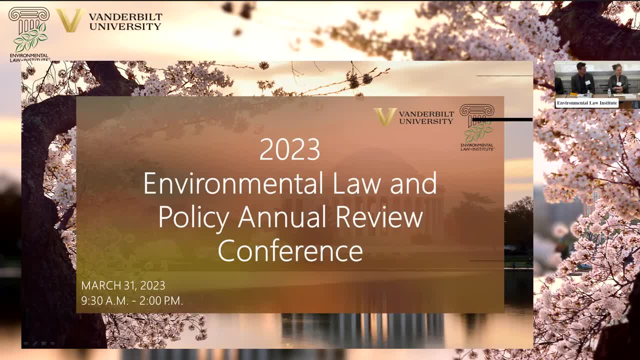 So we published a paper where we asked people: if you had $100 to buy a better reputation, how much of it would you put toward your reputation today versus your reputation after you die? If you ask most economists, they'd say zero after you die- because I'm dead right- But people answered $40,. 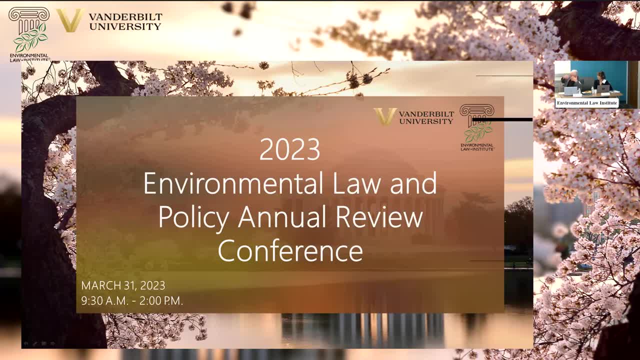 basically that they would put 40 bucks toward their reputation, after which gives you some indication that they do value- That they do value it. Yeah. And so there are people who've done, you know, based on UK housing data and the value of freehold estates versus 99-year leases, which most things are saying. 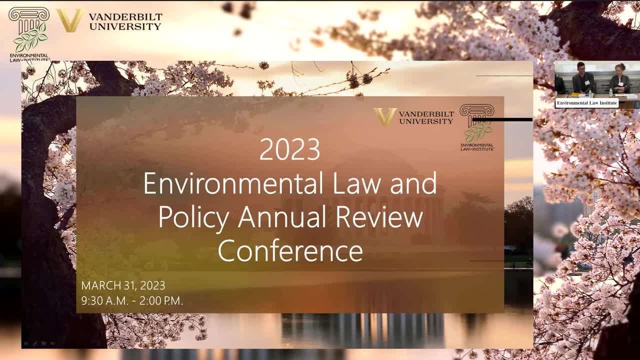 have come up with. you know what the market actually reveals about discount rates. To the extent that there's an empirical basis for it, they tend to be pretty low discount rates that would value those future damages higher than would be done by the usual market measures. 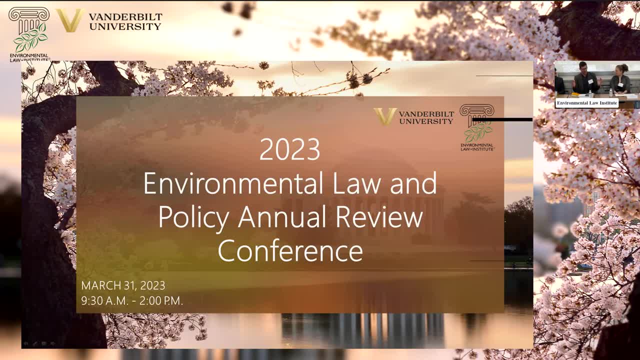 And that's also, as Naheed mentioned, the biggest difference in the different values on the social cost of carbon and the- EPA calculations and the inter-agency working group are whether or not you include international damages or not. But the other one is: what discount rate do you use, And if it's, at one you know. 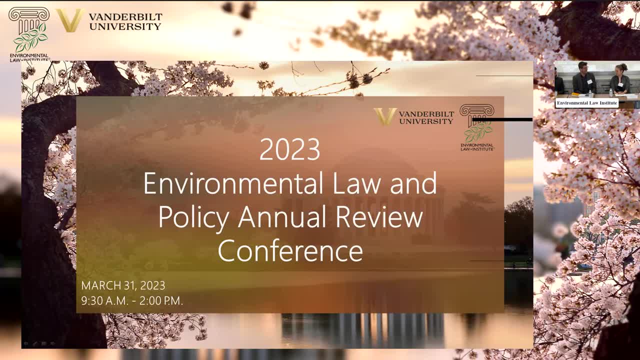 from one to 7% and yeah, there isn't necessarily a right answer in there. Right, right, I'm getting the hook here. I don't know if you want to close up. Yes, Can I just tip that a little bit. If you're valuing, the question is, what are you valuing? 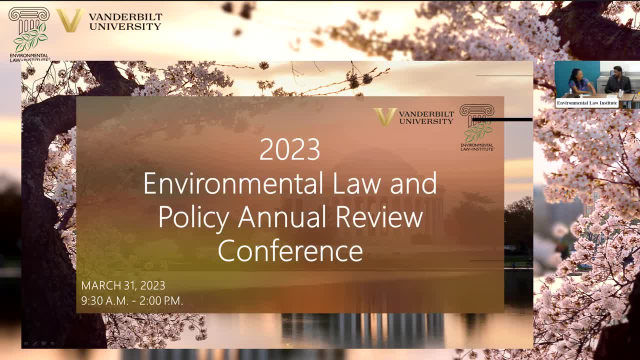 And then if you center, what are you centering? So, if you center those who have been most impacted, you're going to get a different valuation than if you center those who have had resources. So you can use whatever discount rate, you can do whatever cost benefit, but what is it that you're? 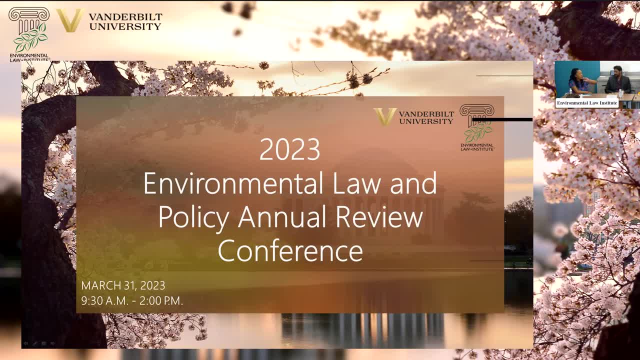 valuing, And that would materially- and it does when we're talking with some of these algorithms- that it changes the way they actually write the algorithm if they're centering something different. I can't resist to say one thing: Sorry, Sonia. 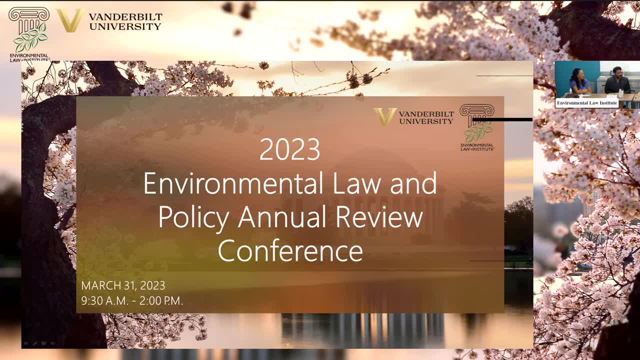 Is that one of the issues with the social cost of carbon that made the news was mortality and life? Yes, And how did that change your your view of the social cost of carbon? Yeah, well, I think it's. it's really important to think about. 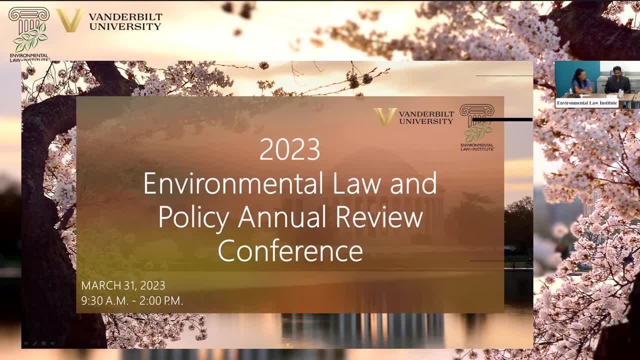 and I'm not saying that it's all the same, but I do think that it's. you know, there's this idea that you know, lives are valued differently in different countries based on a person's willingness to pay and economic ability to pay. So, if you follow what Debra just said, 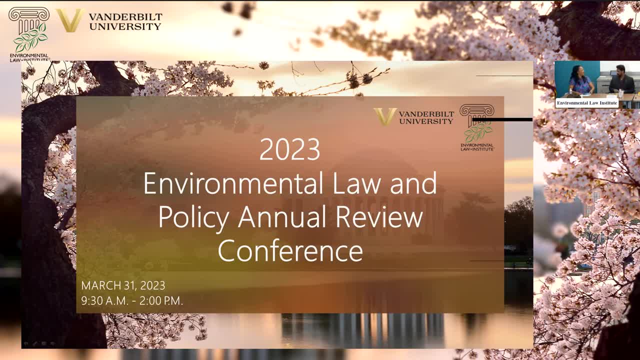 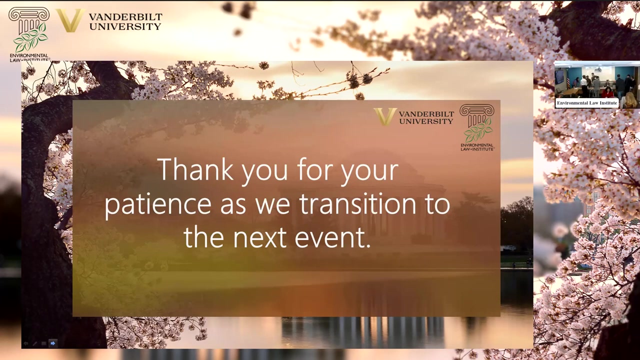 it's countries that are not wealthy and are hot, where most of the deaths would occur, where lives are valued the lowest. We're coming back at 12.55.. We'll be right back. We'll be right back. We'll be right back. 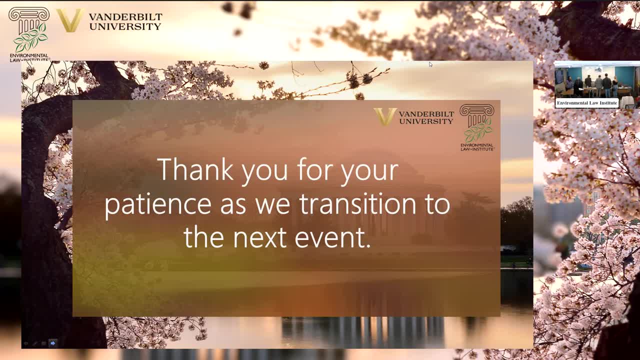 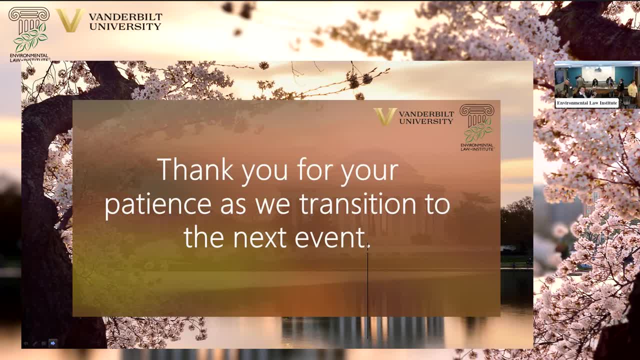 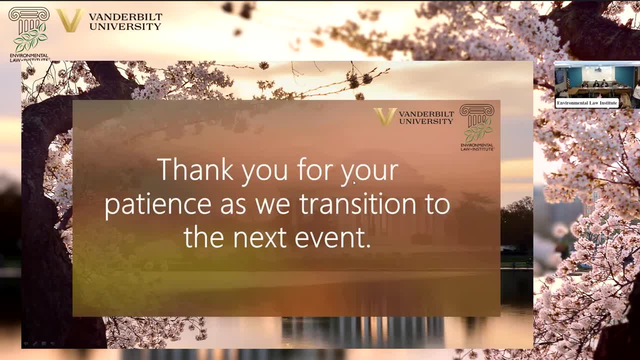 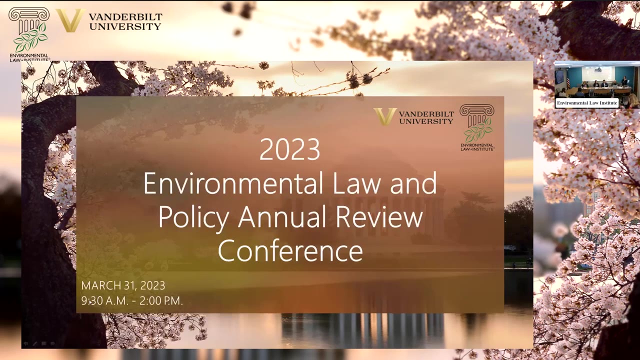 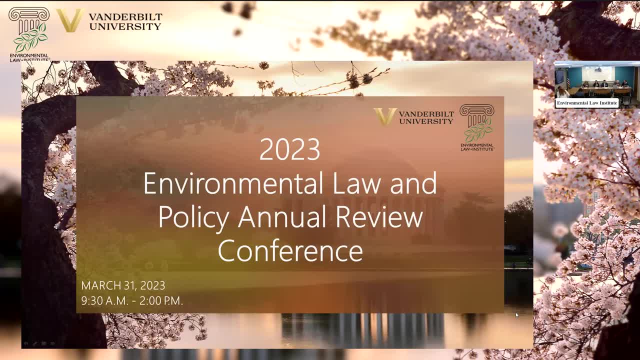 Yes, Sorry for the delay for the Okay back if you're just joining us. i'm linda bregan. i'm a senior attorney with environmental law institute. this is mike vandenberg with vanderbilt law school. um, those of you who are eating um, or? 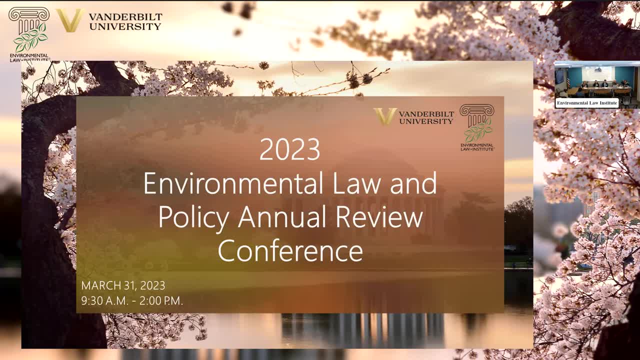 need to still come and go. that's totally fine, but we want to try to stay on schedule. so i do want to remind you, we have a reception right after it too, because i know we haven't had a lot of time to talk in between. so please, um, please, stay for that and, um, i want to remind, uh, the folks that are on. 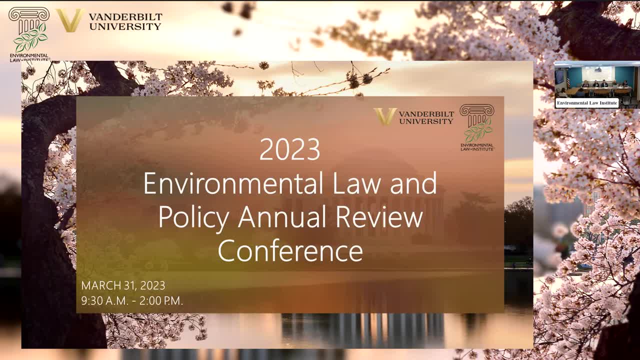 via webinar. if you have any tech issues, put them in the chat and our tech team will get back to you as soon as possible. if you have questions, put them in the question of thoughts, and there are instructions in the chat for how to make different windows bigger than others. as you're watching. 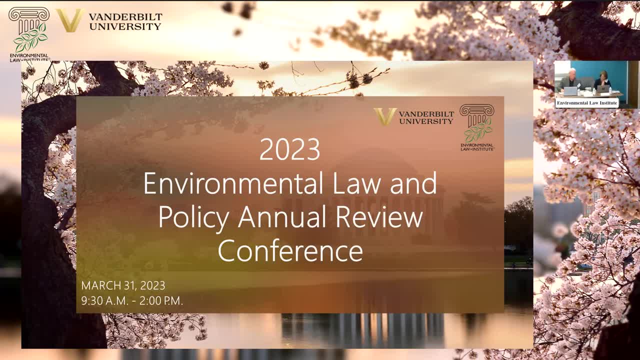 um the webinars. so with that um, i am going to hand it over to thomas boyden, who is a third year vanderbilt law student and article editor for this article, and he is going to introduce our panel. hi, everyone, as mr bragan said, my name is thomas boyden. i'm a third year law student at vanderbilt. 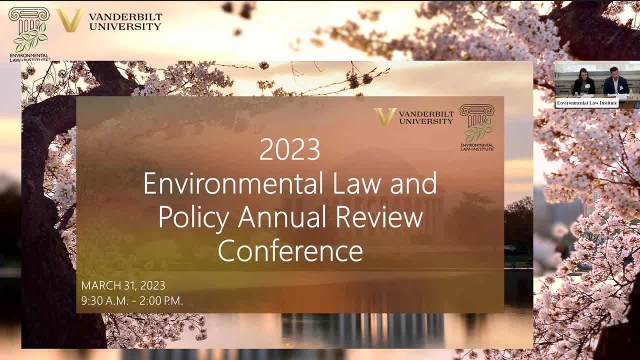 i'm an article editor for lmart um, so we're here to discuss the article. usg mutual funds deliver on their promises by quinn curtis, jill fish and adriana robertson. unfortunately quinn curtis isn't with us today, but we are lucky enough to have jill and adriana over zoom. 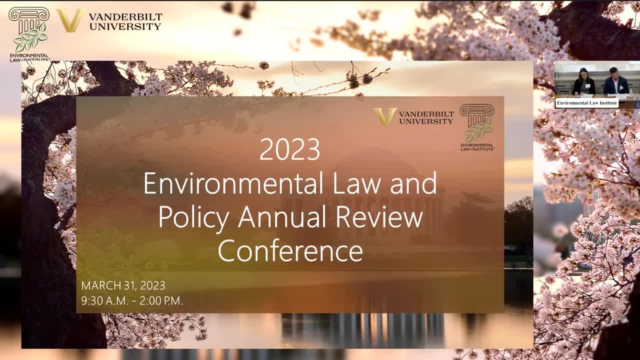 jill fish is a sol a fox, distinguished professor of business law and co-director of the institute for law and economics at the university of pennsylvania law school. she's an associate reporter, the american law institute's restatement of corporate governance. she previously worked as a trial attorney of the doj and worked at the law firm clearly got lived. 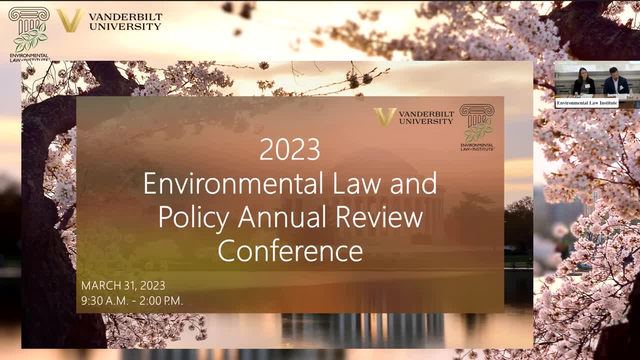 steve in hamilton and taught law at harvard law school, québec Columbia law school and georgetown university law firm. she received her ba from cornell university and her jd from yale law school. adriana robertson is a donald and frisco professor of business law at the university of. 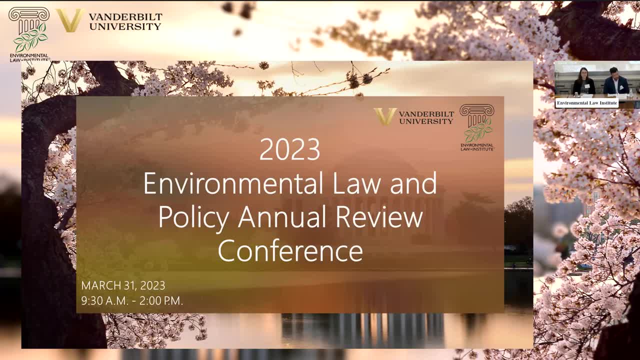 chicago law school. her research interests lie at the intersection of law and finance, including securities law, capital investment and risk management, and financial and financial issues, Capital Markets Regulation, Corporate Finance and Business Law. Adriana held the Honorable Justice Frank Iacobucci Chair in Capital Markets Regulation at the University of Toronto Faculty of Law. 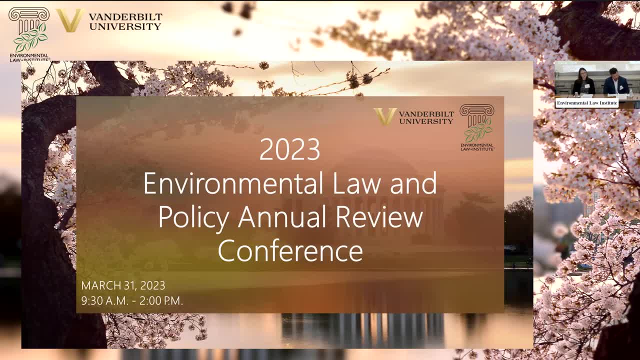 with a joint appointment at the Rotman School of Management. She is held visiting professorships at NYU Law School and Yale Law School. She holds a BA from the University of Toronto, a PhD in finance from the Yale School of Management and a JD from Yale Law School. 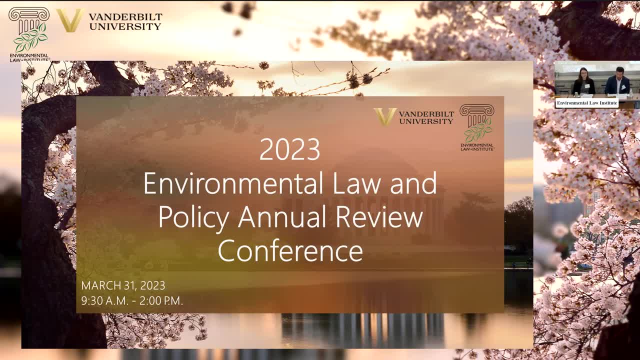 For our panel, we are accompanied by Katherine Jeffroy, Stephen Hall and Ann Kelly. Katherine Jeffroy is an employee benefits executive compensation associate at Arnold Porter in Chicago. Her practice covers employment, compensation and benefit issues, including the design, implementation and administration of employee benefit plans and benefit plan fiduciary considerations. 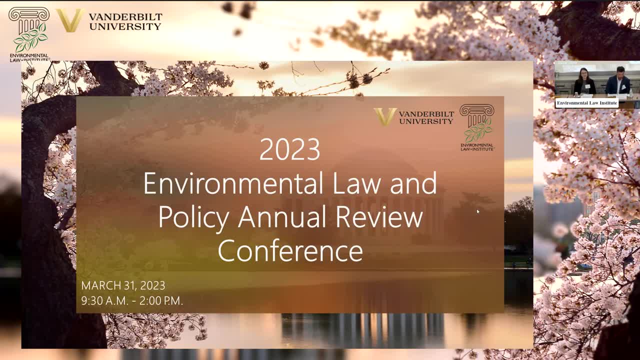 Ms Jeffroy graduated with a Bachelor of Arts in Economics and Political Science from Wesley College and received her JD from the University of Illinois College of Law Stephen Hall. we have also over Zoom. He is a legal director and security specialist at Better Markets. 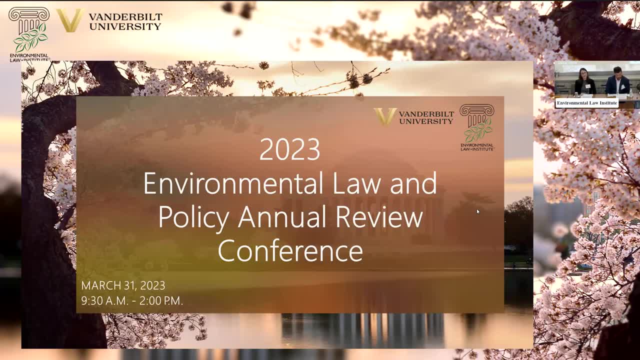 He currently serves on the Commission on Sanctions and Fitness on the Certified Financial Planner Board of Standards. He previously served as senior counsel to the Committee of Financial Services on the US House of Representatives and its Council of North American Securities Administrators Association. 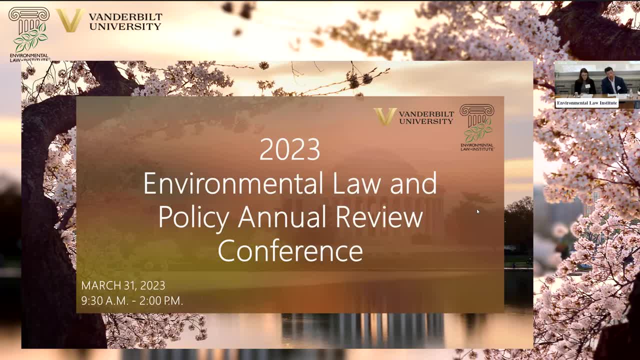 Stephen completed his undergraduate degree at the University of Michigan and received his law degree from Georgetown University. Lastly, we have Ann Kelly. She is the Vice President of Government Relations at Ceres and leads Ceres Policy Network's business for innovative climate and energy policy. 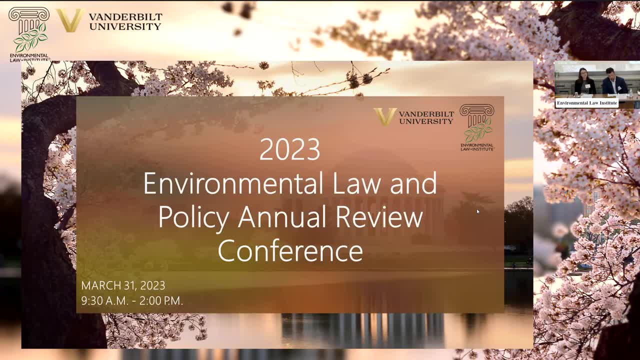 Ann is also an adjunct professor at Boston College Law School, serves on the boards of the Environmental League of Massachusetts and Massachusetts Interfaith Power and Light, and is a fellow in the American College of Environmental Lawyers. Previously, Ann served as a special assistant for EPA Region 1 Administrator, John DeVillis, and has taught at Tufts University, Suffolk University and New England School of Law. 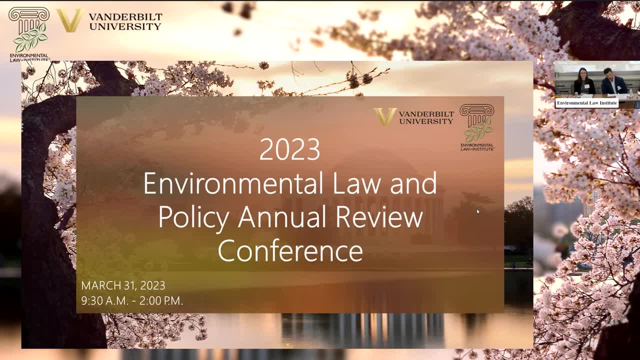 She holds a BA from Michigan State University. She has a master's from Harvard and a JD from Western Michigan University, Columbia Law School. Thank you, Thomas, Thank you, professors, for being here remotely. I know you're really busy. 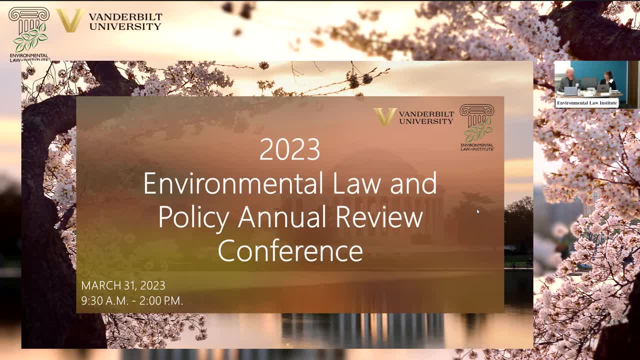 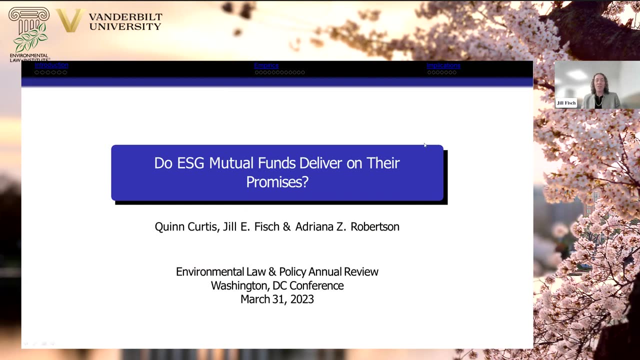 You're at another conference, So thank you for joining us And we're going to hand it over to you, professors, to tell us about your article. So I can't see. Can you see our slides? There are slides, All right. 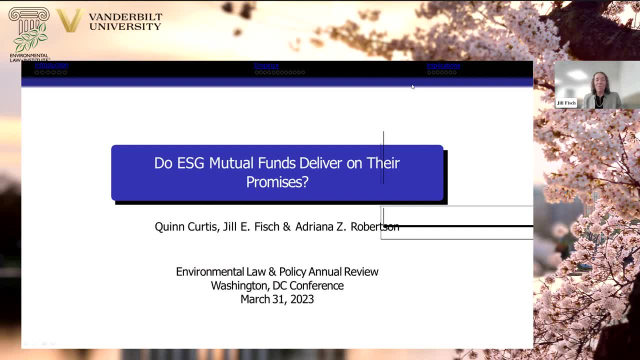 This is a very odd setup So I can't really follow what's going on here. But I'm going to give it a shot and quickly turn it over to Adriana so that I don't embarrass myself. But very briefly, next slide, please. 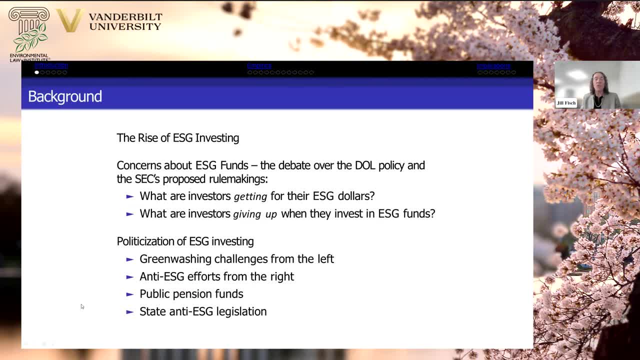 So this is based on a paper that we did from a couple of years ago. Is there any way to make this bigger? Yeah, Okay, Got it. And obviously ESG investing continues even since the time that we did our empirical research. 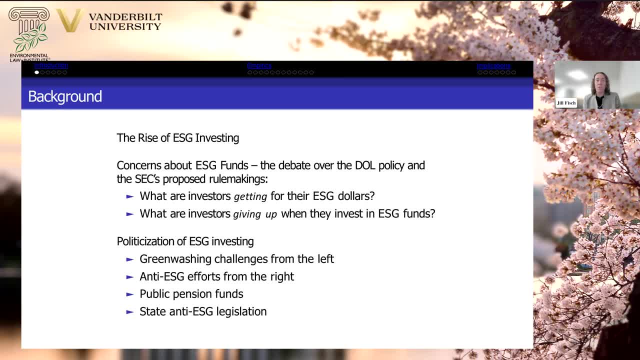 We did our empirical analysis to get more, both significant in terms of the number of dollars and more controversial. It's also stirred a pretty active debate. So we see this with respect to the SEC, various proposed rulemakings, the debate about the Department of Labor and its policy. 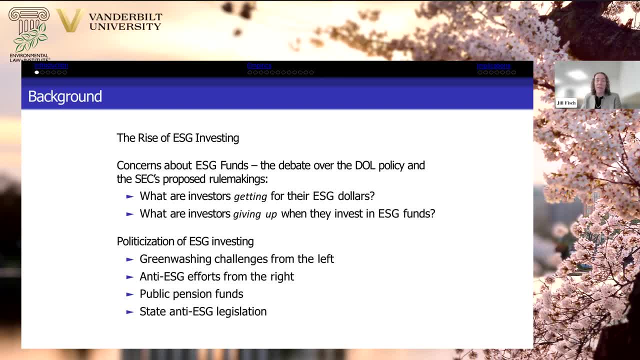 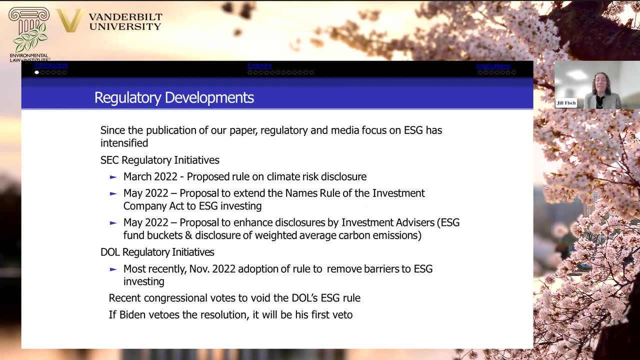 And so we seek to address two questions that we think animate that debate. One: what are investors getting when they invest in ESG? Two, what are investors giving up Next slide, please? All right, Since the publication of our paper, and even since we sent in our slides, there have been continued developments. 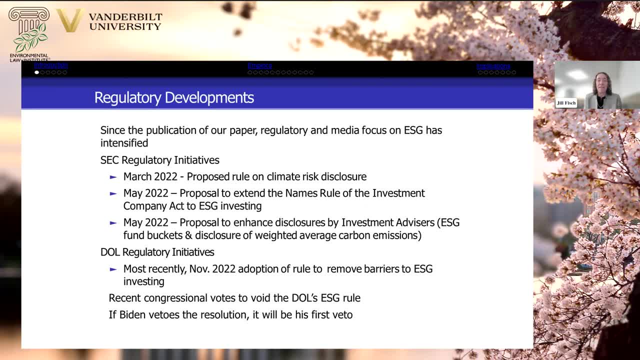 So, as I said, a number of pending rulemakings by the SEC And we don't know exactly if and when those rules are going to be finalized. The Department of Labor adopted a rule to remove barriers to ESG investing. Congress voted to void the Department of Labor's rule. 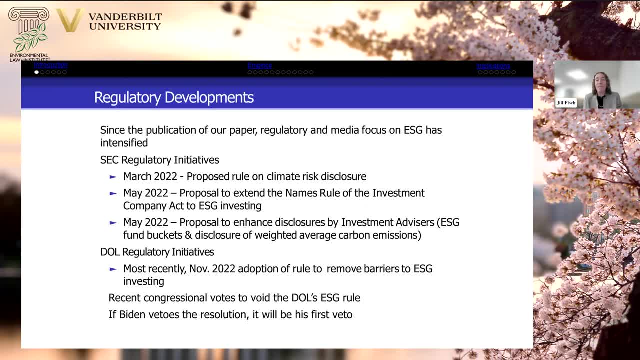 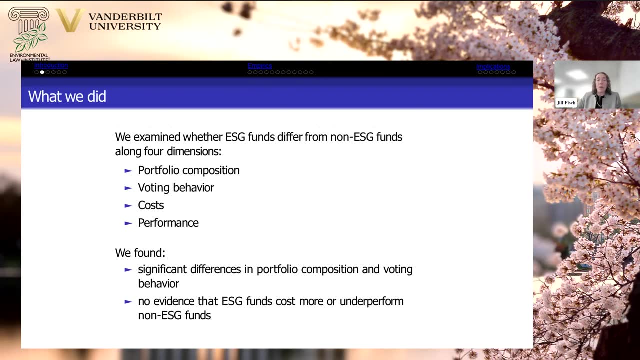 And, as I said, after we prepared these slides, President Biden got to exercise his first ever veto authority to veto the congressional resolution. Next slide: We looked at whether ESG funds differed from non-ESG funds And we're focusing on primarily on funds that use the name ESG. 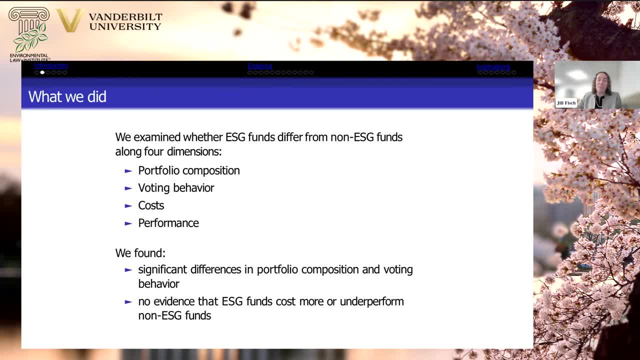 So this work also intersects with the paper that we're presenting at our conference Later today. that focuses on the SEC's names rule. But we look at the differences across four dimensions: composition, voting behavior, costs and performance. And, to summarize very briefly, we found that ESG funds do differ from non-ESG funds. 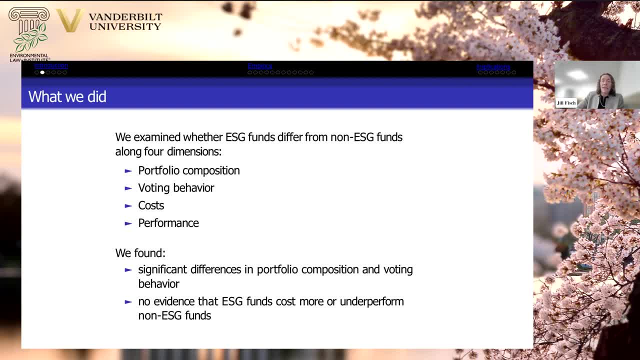 They differ both with respect to the securities they hold and how they vote the securities. And we also found that ESG funds don't cost more or underperform. Next slide, A couple of caveats, actually a lot of caveats, because, as I said, this paper and the empirical work is now a few years old. 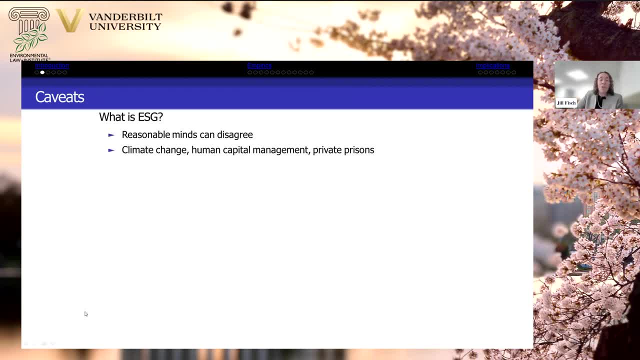 So please just keep advancing slowly. So number one, with respect to what is ESG right? that's a tough question And even over the course of the last several years people have kind of shifted their views about, for example, fossil fuels in light of the war in Ukraine. 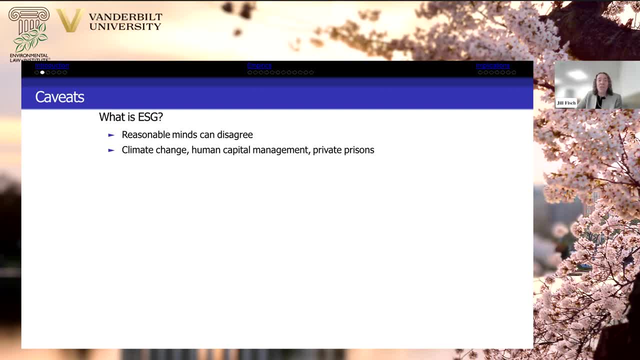 So it's a big tent. A lot of issues can constitute ESG And a lot of people have said you should be more precise in answering the question whether these ESG funds are ESG enough. But when people disagree on what exactly ESG is, that's a hard question to answer. 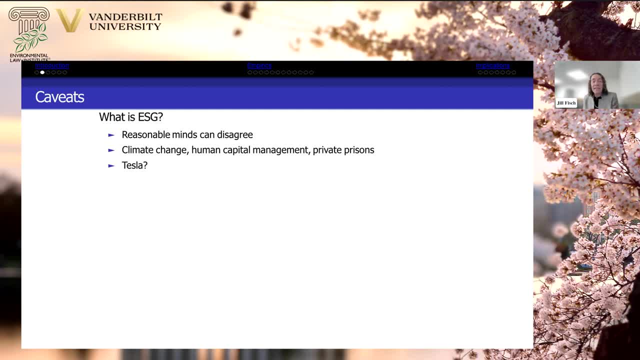 Keep advancing, please. So you know, is Tesla ESG. It's great on electric cars, perhaps not so great on employee policies. We don't adopt our own definition of ESG in this paper- Advance please- But instead we rely on the work of four different ESG ratings organizations. 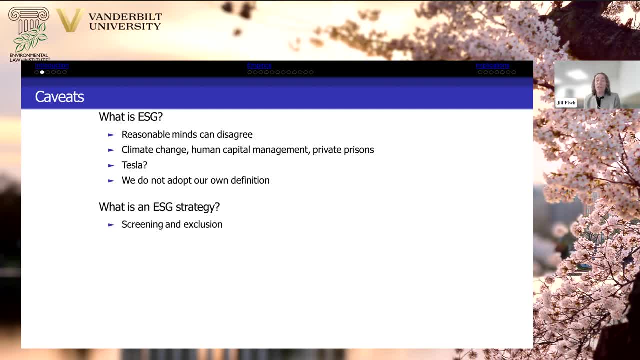 And you know, four is a lot. They use different methodologies. We think this gives us a fair amount of robustness. Second, what is an ESG strategy? There are a variety of strategies. You can choose to hold green or ESG securities. 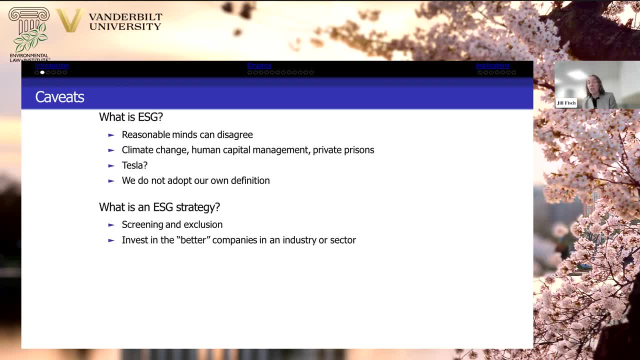 You can choose to exclude non-ESG securities. You can do it industry or sector by sector and choose the better companies within each industry. So, rather than exclude fossil fuel companies, you might hold the fossil fuel companies that are working to affect the quickest transition. 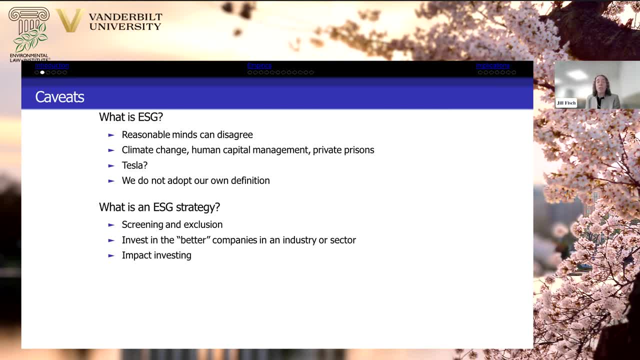 You can hold the entire market and try to change the behavior of the companies in which you invest- so-called impact investing And tilt-based strategies- And Adriana will talk a little bit more about that. Keep going, please. All right, And of course, there are the idea of ESG- can be potentially very broad. 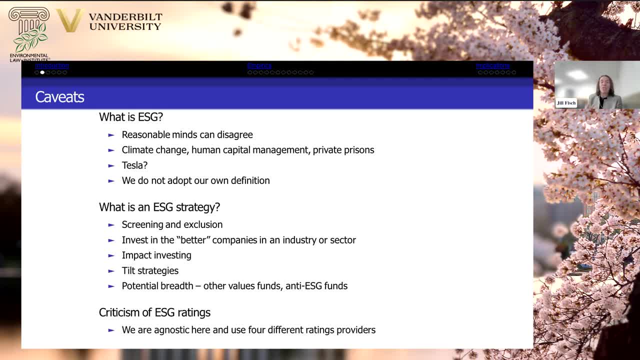 We tend to sort of fall back on climate. That's the one that everybody sort of defaults to. But there are a lot of different kinds of values-based funds. We like in particular the Catholic values-based fund, which you know you could debate. 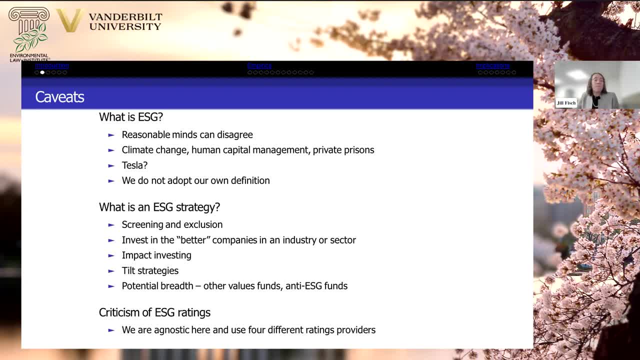 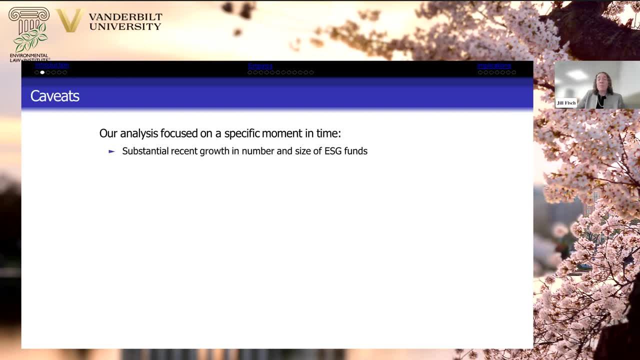 Is that an ESG fund or not? Next slide, please. So second big caveat: we focus at a specific moment in time. ESG funds continue to grow in size and in number And they continue to evolve. So our work has caused us to look pretty carefully at the market, at the funds that are out there and at the information they disclose. 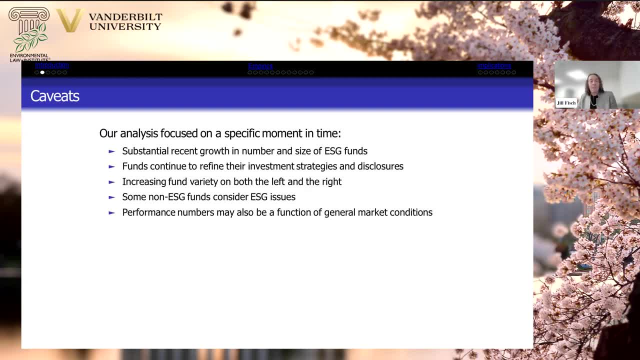 And it's a moving target. Keep advancing, please. All right, As I said, Go back. There's increasing variety on both the left and the right in terms of ESG funds, So you know MAGA fund and the drill fund. there are sort of anti-ESG funds as well. 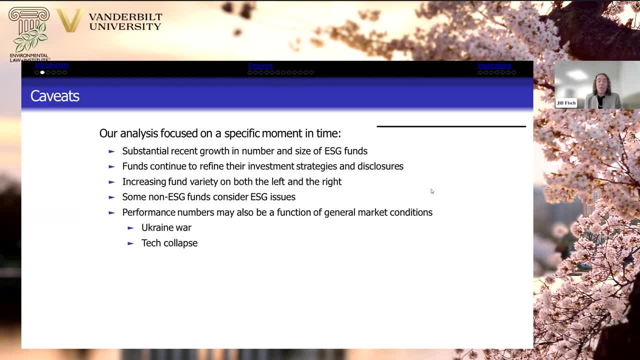 And in addition, there are some non-ESG funds that purport to consider ESG issues. So how do you factor that into an empirical analysis? And finally, I just want to flag the fact that performance analysis is very time specific Right. 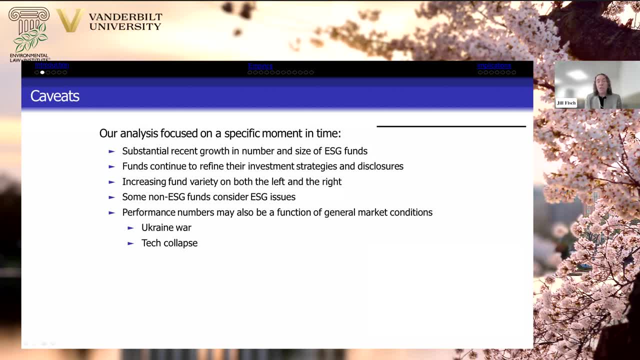 So if you go back a few years during the tech bubble, You could hold a low carbon portfolio That could consist primarily of tech stocks. When tech stocks were doing well, it looked like ESG funds were outperforming the market. More recently, as I said, with various factors like the Ukraine war, fossil fuels have been outperforming tech companies. 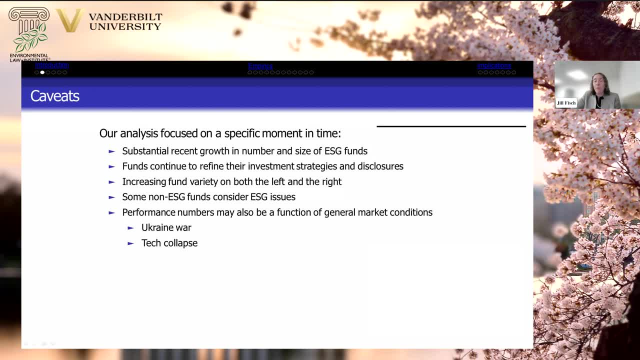 And so ESG funds, arguably, are underperforming the market, certainly over the last year. So when we talk about performance, we looked at a specific moment. We looked at a specific moment in time. We're not purporting to make general statements about ESG funds over the long term. 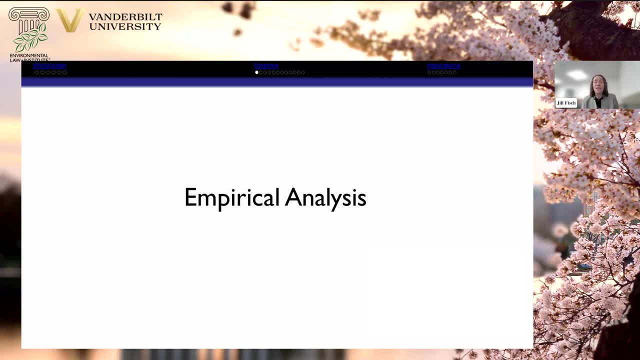 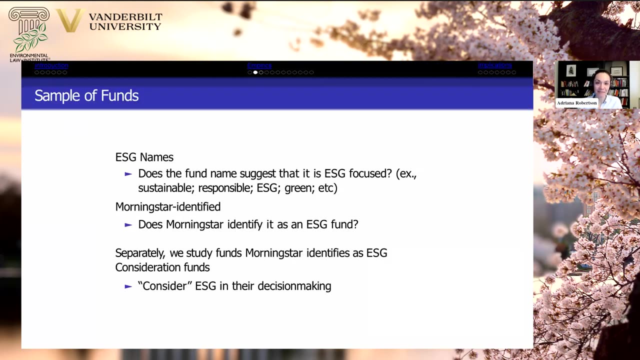 All right, Next slide: Adriana you Hello. So what we wanted to do? can you all hear me? Yes, Okay, Excellent. So if you could advance to the next slide please. It's an empirical paper. We wanted to just see, you know, are the funds doing what they say they're doing? 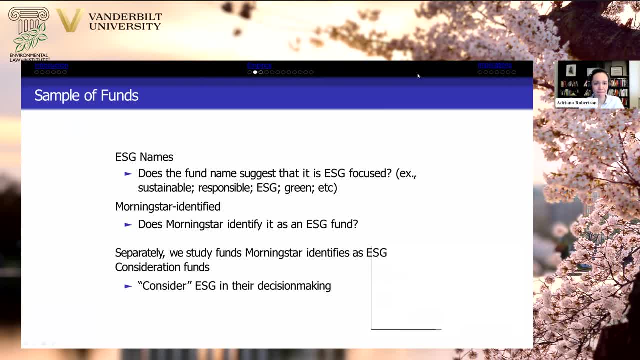 What are investors getting? What are investors giving up, Just like Jill said. So the first thing, of course, we had to do was figure out, well, what funds are going to count as ESG for our purposes. So we ended up with three different categories of funds that we pulled in. 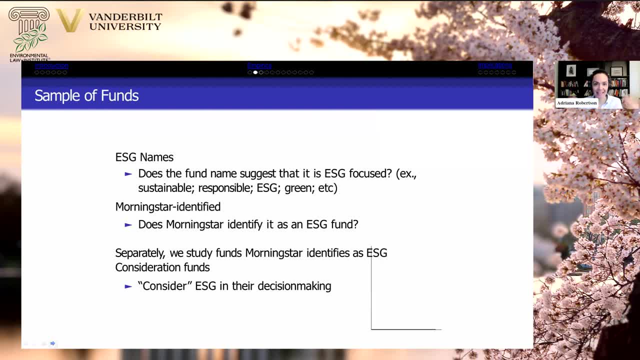 The first are funds that had a name that indicated that it was sort of an ESG fund, So it could have said something like sustainable, responsible greed, et cetera, in the name itself. The second thing we did was Morningstar, which is a mutual fund information provider that lots of investors use. 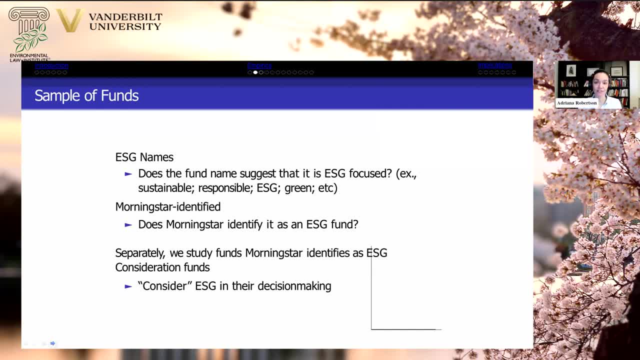 And then, finally, Morningstar identified, or that lots of investors rely upon. they identified certain funds as being ESG funds. So we just took that list. Now. there was some overlap, of course, between that second list and the first one, but not complete. 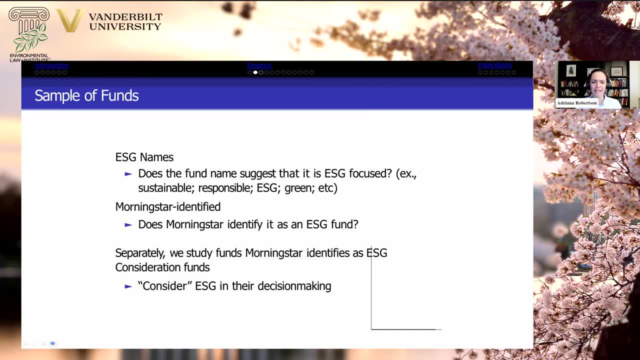 So we had both. And then, finally, Morningstar also identifies a series of funds that it calls ESG consideration. This is what Jill was referring to when she said. well, some funds they say they consider ESG without you know purporting to actually be an ESG fund. 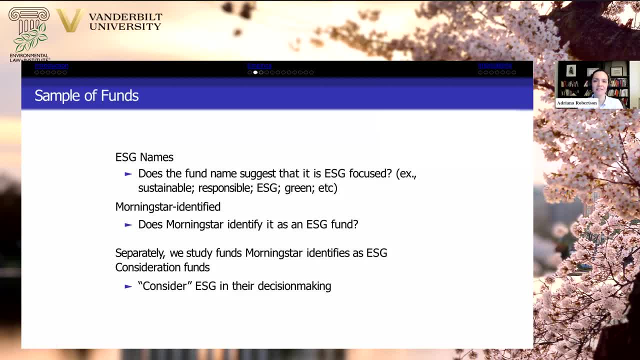 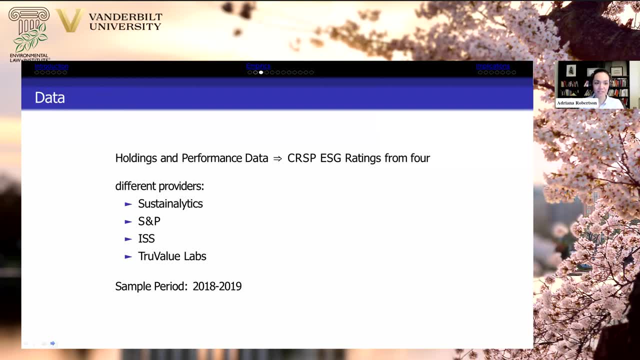 Right, It's considered in their decision making. So we considered that to be a third group. Next slide, please. You know we took very standard data sources for the holdings and the performance. That was just the Center for Research and Securities Prices, Chris. 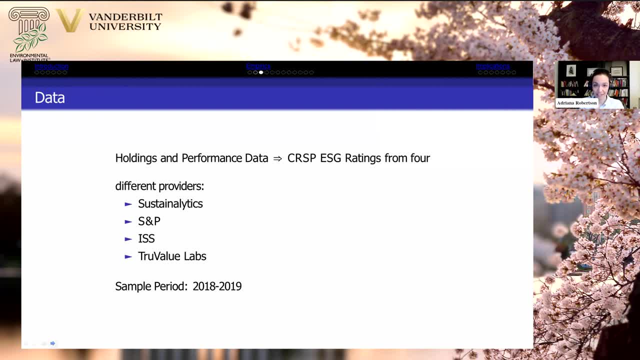 As Jill said, we used ESG ratings from four different providers. We consider this to be an important strength of the paper, because ESG ratings have often been criticized from a number of different quarters for being very poorly correlated with each other. So you know, that's a good thing. 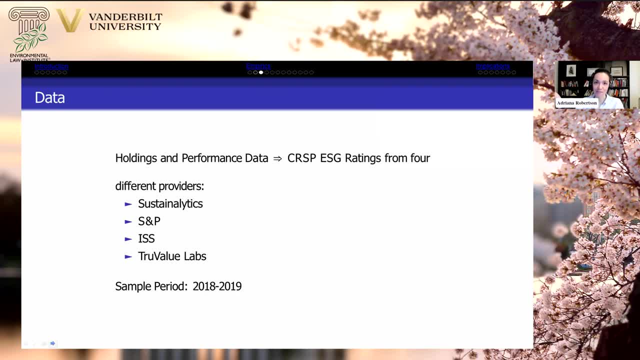 But then we also have a lot of other ratings that are very poorly correlated with each other. So you know, one ratings provider could say that ExxonMobil is pretty good, Another one might say it's pretty terrible. We're kind of agnostic. 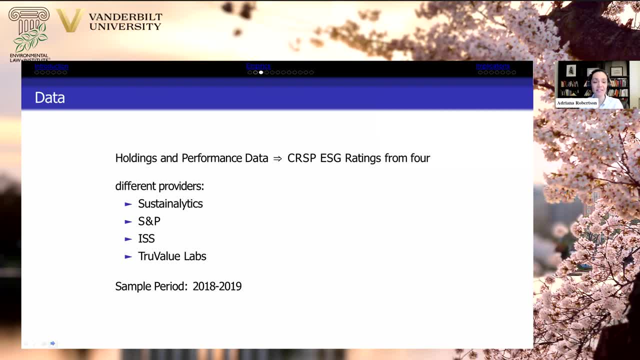 So we figure: well, look, let's just take a bunch of different ratings providers and see what we find. As Jill said, it's a very specific sample period. It's what we had at the time We wrote the paper in 2020.. 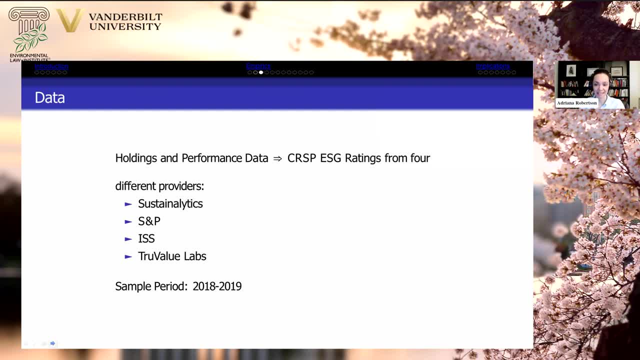 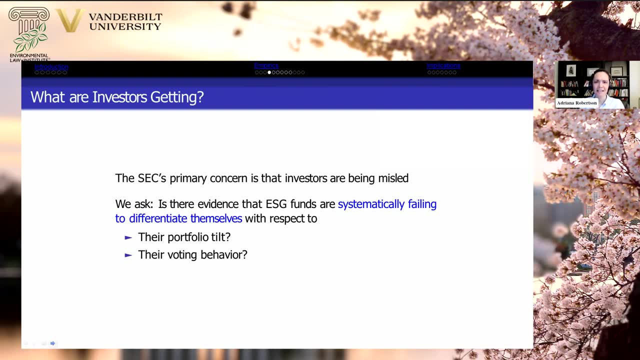 The market was changing rapidly so we didn't want to go too far back in time, So we did 2018 and 2019.. Next slide. So, as we said, the first concern is: are investors getting what they think they're getting? 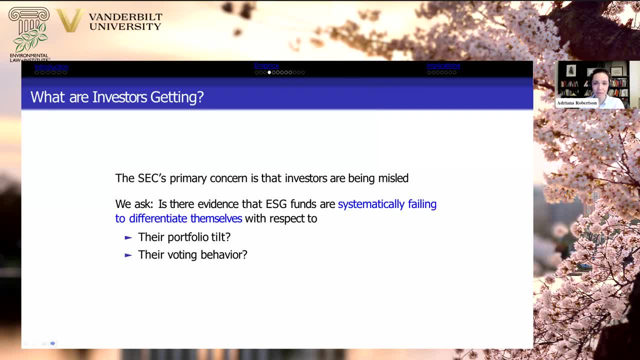 The SEC is an investor protection entity primarily, And so we asked the question: well, is there any evidence that these ESG funds are systematically failing to differentiate themselves? Are investors getting something different from a conventional fund? And we looked in two dimensions: the portfolio tilt, what they're actually holding, and their voting behavior, because those are kind of the two main things that a mutual fund provides to investors. 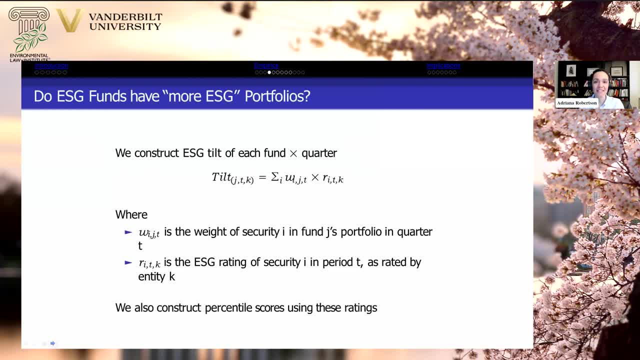 Next slide, please Thank you. So, to figure out whether these ESG funds were more ESG than conventional funds, what we did was we just constructed for each fund in each quarter, because the data we have are quarterly. how ESG? what is the average rating? 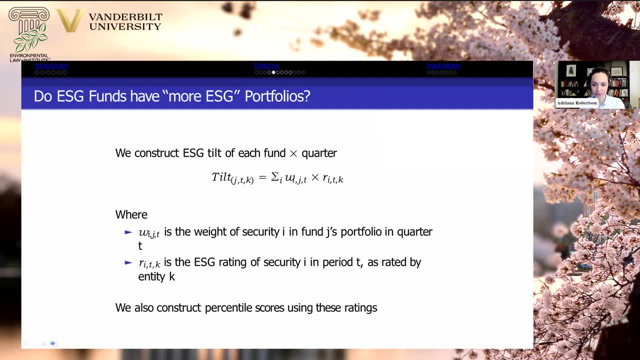 The weighted average ESG rating of the portfolio that it holds right. So that's all we're doing. when we calculate the tilt, It's just the weighted average rating And again, we're going to use four different ratings providers. We're going to use four different ratings providers. 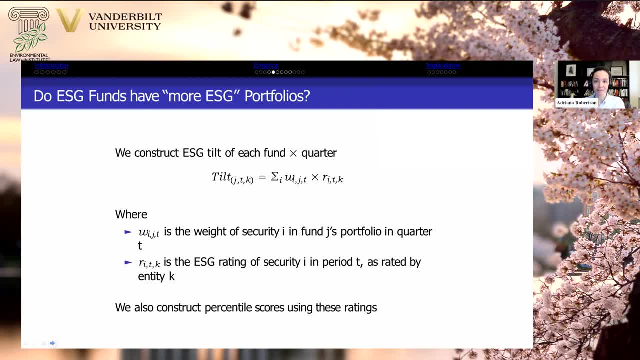 We're going to take every constituent of the fund's portfolio, multiply it by its rating as provided by the relevant rating provider, multiply by the weight and add them all up. So, if we go to the next slide, what you can see here is what this ends up looking like. 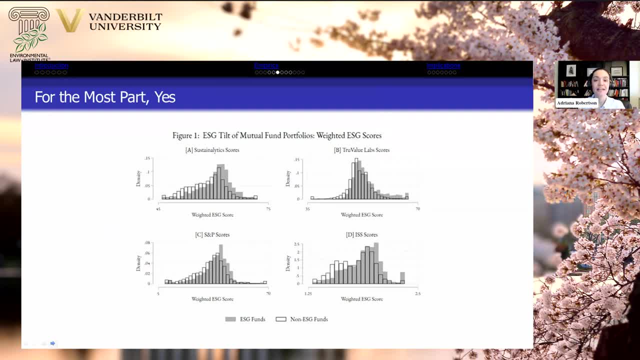 So the empty bars, the hollow ones, those are the conventional funds, the non-ESG funds in our sample, The gray bars. that's the weighted average for the ESG funds in our portfolio, And what you can see here is that with each of the four different ratings providers the gray bars are kind of shifted right. 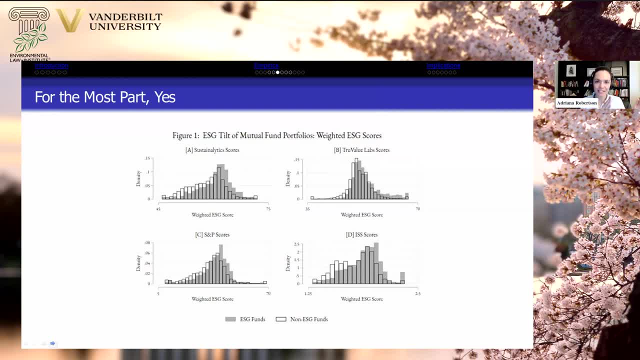 We still get a distribution in both, but the ESG ones are systematically more ESG, higher rated on average than the non-ESG funds. Now we can talk about whether, and, as Jill said, is this enough? Is it enough more ESG than the conventional funds? 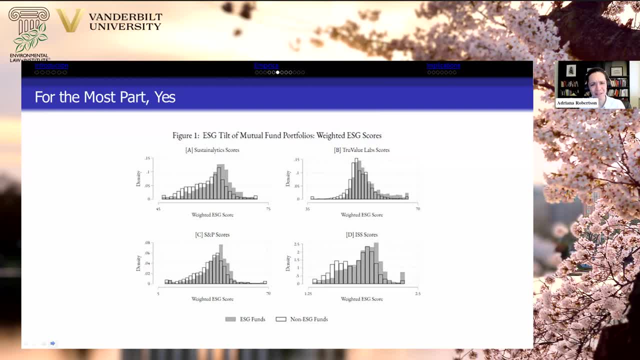 We can talk about that. We don't really have a position on that. We don't really have a benchmark on that. We don't really have a benchmark on what it means to be ESG enough, But it's certainly the case that they are doing something different, right. 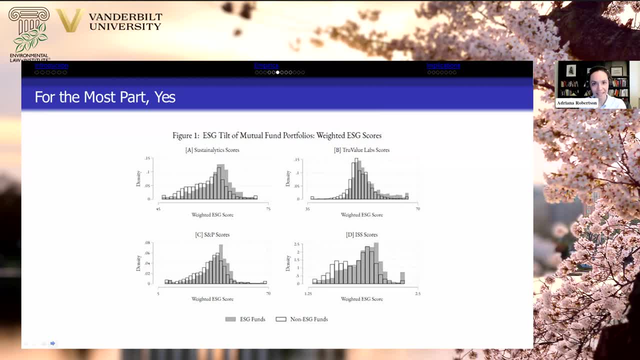 They do tend to be more green, more ESG, than conventional funds. And the other thing that's important about this I just want to flag is that this came out with all four of the ratings providers, notwithstanding the fact that they all have very different methodologies. 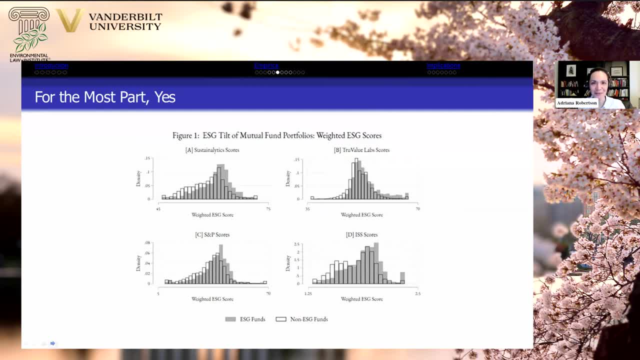 And there's no way for you to know this other than I'm just going to tell you, and you'll have to take our word for it. We actually wrote the paper using the first three of these ratings providers, because we hadn't gotten data from the fourth one yet. 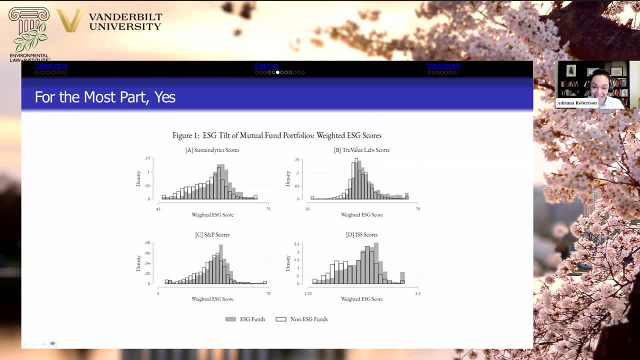 And then we got the fourth set of data. we calculated it and it turned out. so it's kind of like an external validity test. It turns out that actually everything went through with the fourth data provider. So that was kind of an encouraging thing to have happen. 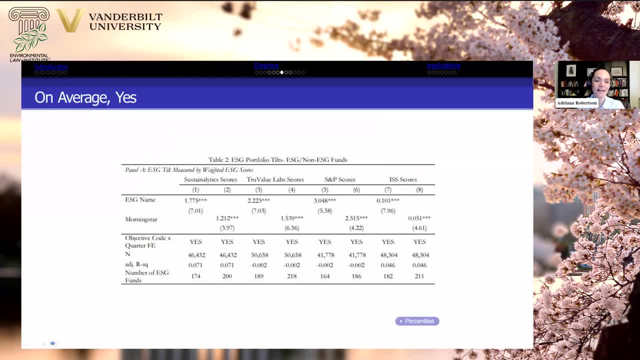 We didn't reverse engineer it. Next slide, please. Here we just run a regression where we, this way, we can include a bunch of controls, Sure, So all you see is that this is true, It's not just true in the picture. 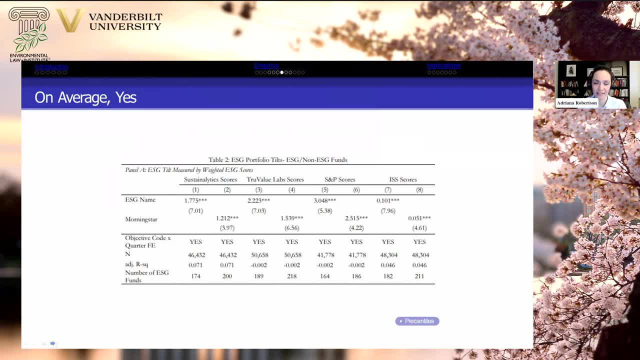 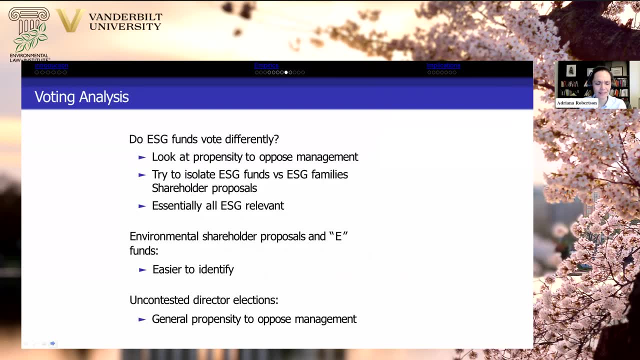 If we control for things, you still get a more positive right. The coefficient is positive. That's all I really want you to take away from this slide. On average, yes, they are higher rated. The next thing we ask, because the other thing that you get from a fund is the voting. 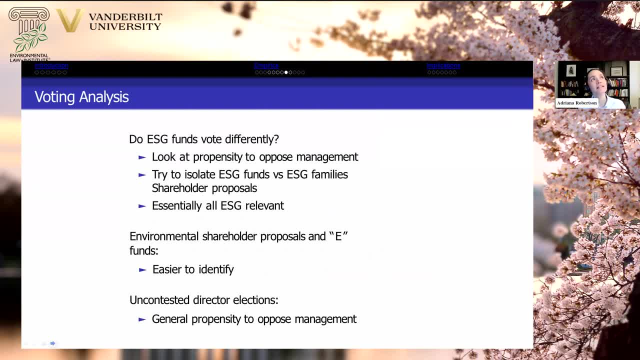 So we just ask whether they vote differently. And here what we did was we wanted to know if these funds tend to be more independent of management. That was the proxy that we sort of went with. So we looked at the propensity to vote, We looked at the propensity to oppose management. 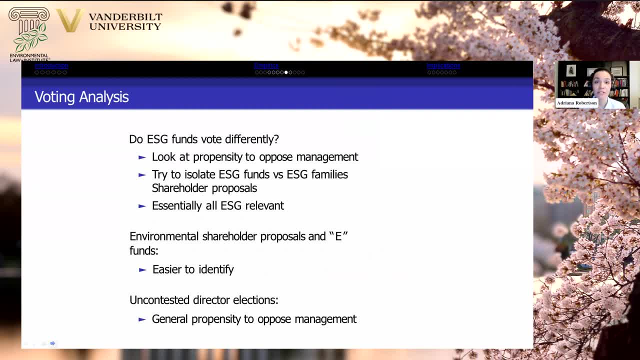 We tried to isolate ESG funds versus their families. We looked at shareholder proposals And we also looked, in particular, at environmental funds, because we actually read the descriptions to see what the funds are purporting to offer. We looked at environmental funds propensity to vote against management for shareholder proposals on environmental issues. 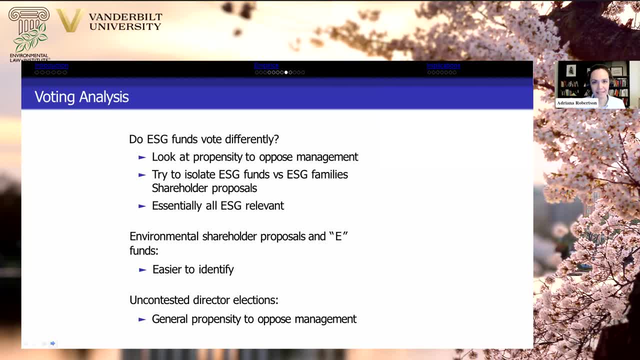 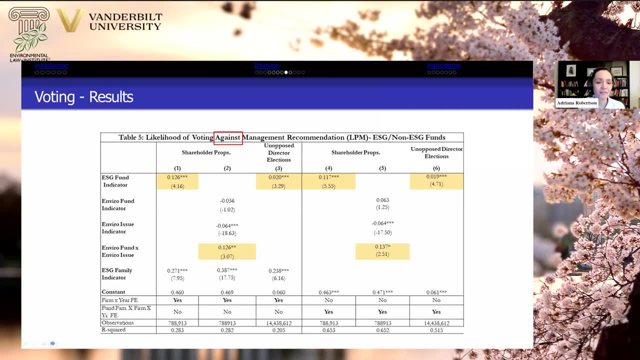 And then finally, you know, uncontested director elections. That's just again a general propensity to oppose management. That's just again a general propensity to be more suspicious of management. So if you go to the next slide Again, all we really want you to take away from this is that the coefficients are all positive. 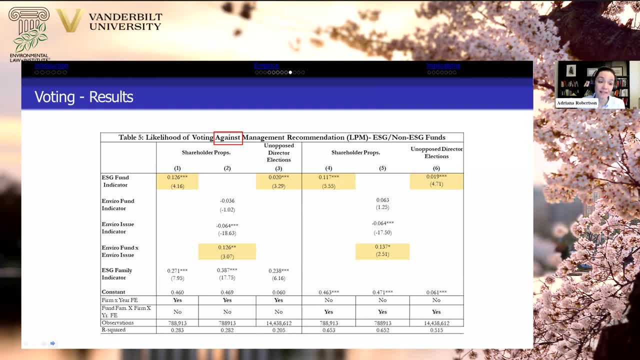 They're all coming out the way you would expect, which is telling us that ESG funds are more likely to vote for shareholder proposals against management for the proposal, Environmental ones, in particular, that second column are more likely to vote for environmental shareholder proposals. 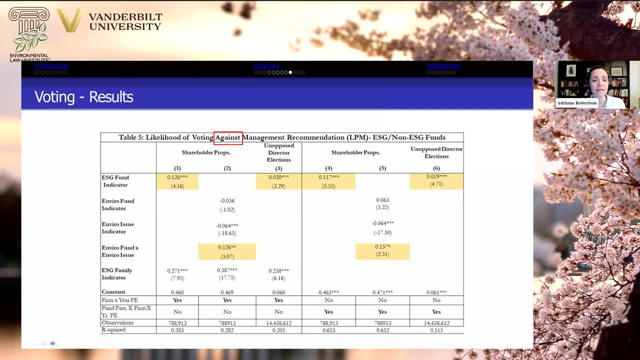 So they are doing something a little bit different. The third column: that's just telling you that ESG funds are also more likely to oppose management. The only difference between columns one and three and four through six is we just have different sets of controls right to try to make sure that this analysis is robust. 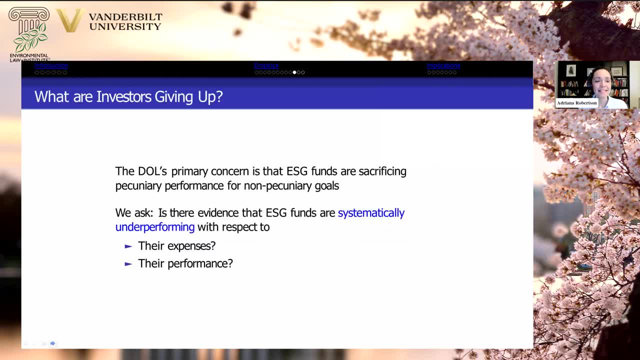 So that's all we want you to take away from that. The next thing we ask is: okay, well, that's what the investors are getting. They are getting something a bit different. Well, what are they giving up? And this is the DOL's primary concern: right, that the ESG funds are sacrificing pecuniary performance for these non-pecuniary funds. 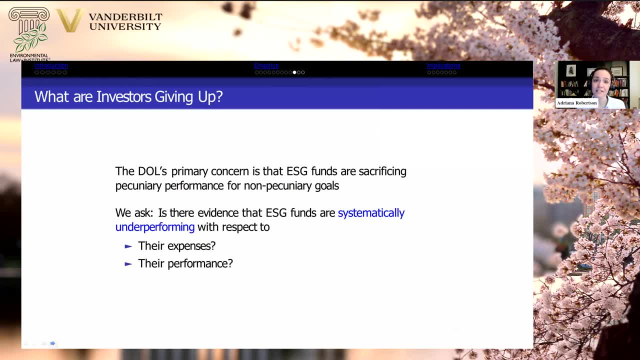 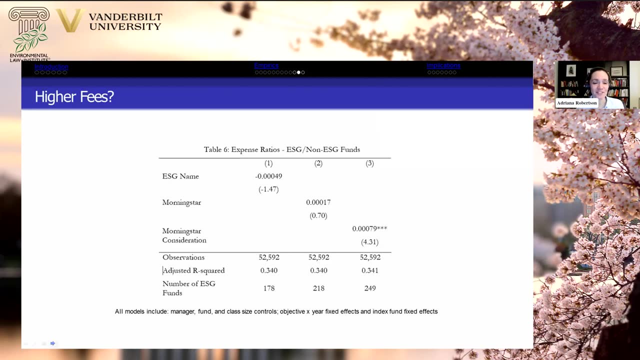 So here we just ask: is there systematic evidence that they're underperforming relative to conventional funds? Either are they more expensive or is their performance worse. Next slide, please. So here all I want you to take away: there's no stars. 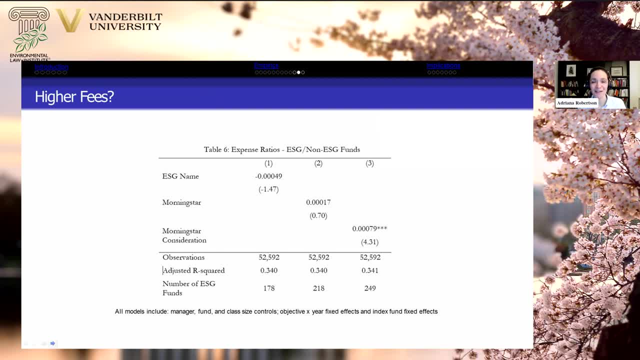 There's no statistical significance. The coefficients are all zero. The funds are not more expensive. If you press next, please, a little red box should pop up. There we go. Just want to be very clear. We're not claiming that these mutual funds are cheaper than like a broad-based, you know two basis point S&P 500 fund offered by BlackRock. 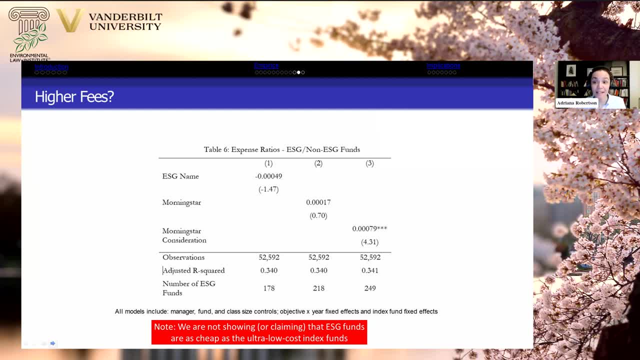 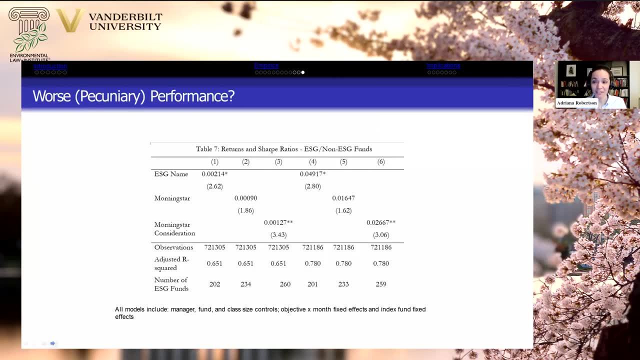 They're not. They are more expensive than a two basis point fund. But guess what? There are lots of funds that are actively managed that charge more than two basis points, that you know people buy right. So if you don't like actively managed mutual funds, you're not going to like these ones. 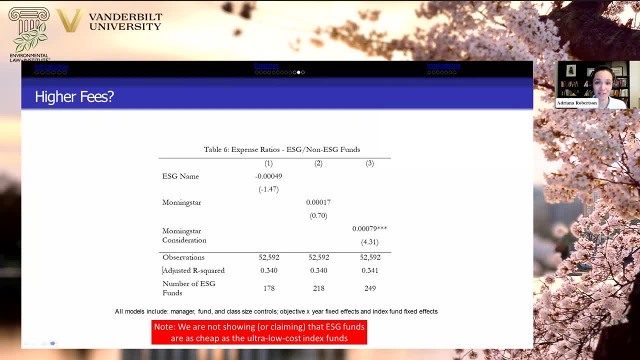 But as long as you're okay with buying something other than an ultra-low-cost fund, there's no particular reason to worry about these ones. Next slide, please. The same goes when we look at performance. If anything, the performance is maybe slightly better in this time period. 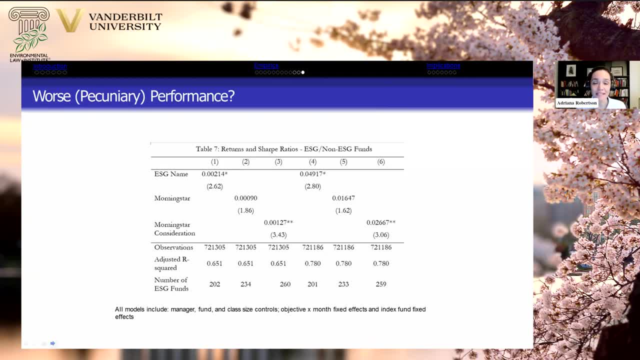 We don't want to put a ton of emphasis on that because, as Jill said, it's sensitive to the time period, But certainly there's no reason to worry that the performance is worse than comparable funds. Next slide, please. So I'll maybe pass it back to Jill to just very quickly wrap up the discussion. 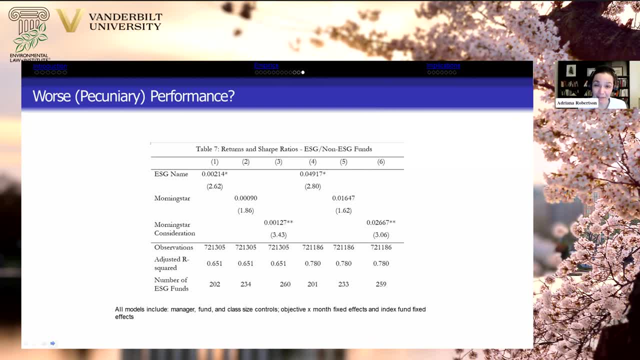 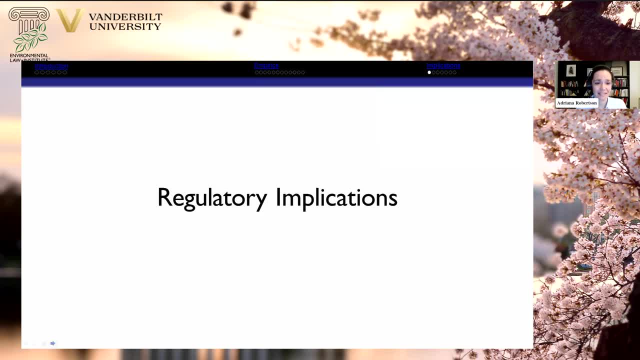 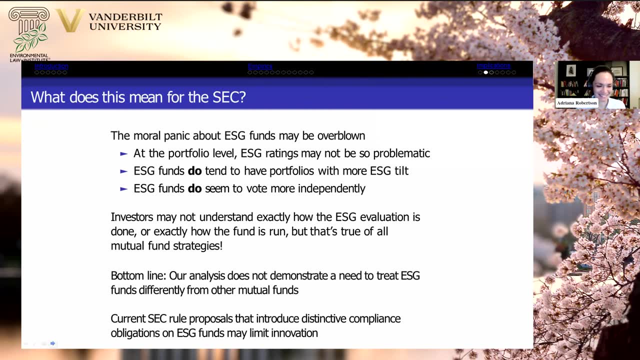 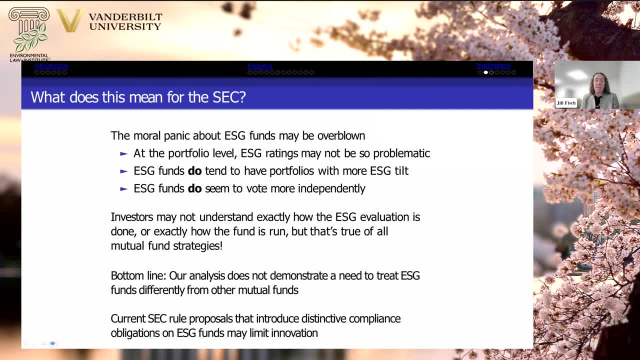 We don't think that ESG funds are distinctively or particularly problematic. They do seem to hold securities with more ESG tilt. They do seem to vote more independently than non-ESG funds And while it might be true that you can't necessarily predict from the name, 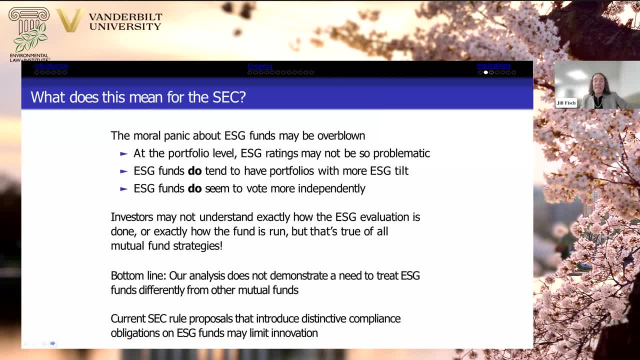 or from the fact that something is an ESG fund, exactly which securities it holds. we think that's true of all mutual fund strategies, And we don't think that's something that's disqualifying or warrants distinctive regulatory treatment. So, in particular, even though this is now a paper that's 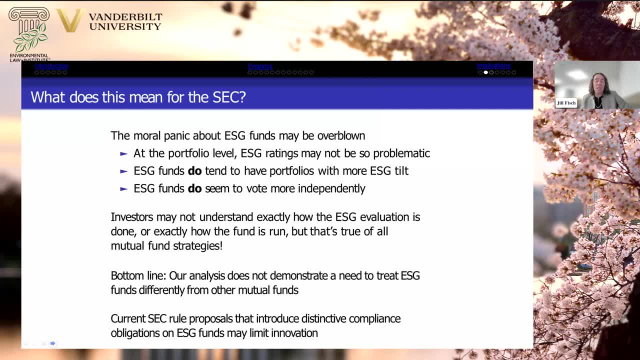 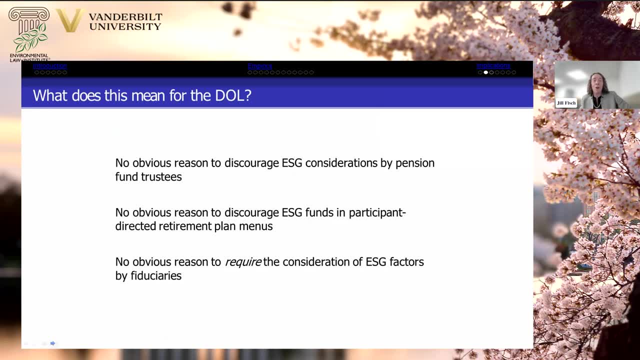 a couple of years old. we think our paper has particular implications for some of the SEC's pending rulemaking proposals. Next slide: I think that's it Right. So no obvious reason On the DOL side as well. no obvious reason to discourage pension fund trustees from considering ESG. 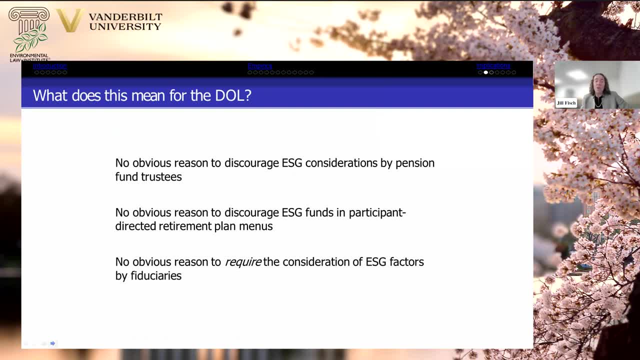 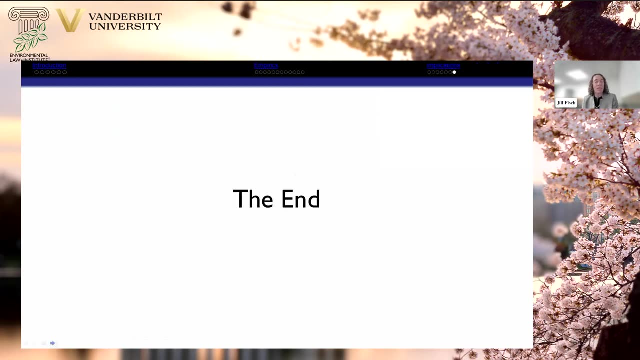 factors, But, by the same token, no obvious reason to require that fiduciaries consider ESG. ESG factors should be like anything else that you know warrants consideration consistent with a trustee's fiduciary duties, And I think that. I think that's it. 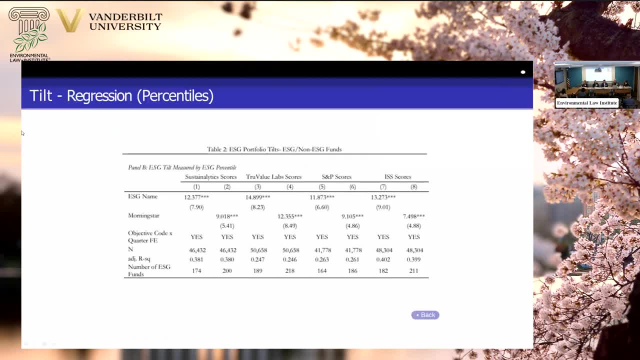 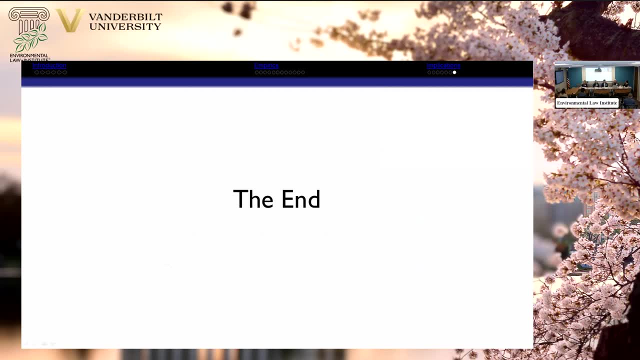 Yeah, The end That was. that was wonderful, Jill and Adria- And I can tell you've done just a few of these remote presentations before. It was like you were in the room with us. It was great, And we're going to go now to actually being in the room with some comments from Catherine. 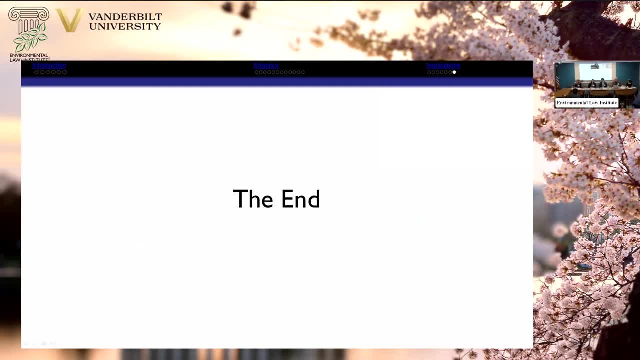 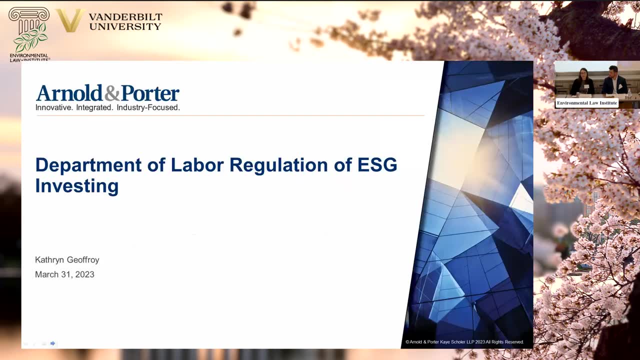 Hi. So I'm in employee benefits and executive compensation, And so when I read this paper, the first thing that I zoomed in on is, you know, the Department of Labor's regulation of allowing ESG focused investments in plan retirement plans and the broader considerations that are informing the 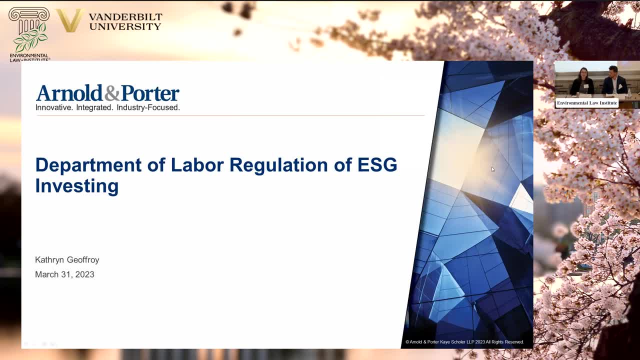 decisions that fiduciaries are making about what investments to include in a plan, So we're going to talk a little bit about that today, And then also, as both the authors noted, this is an area where there's been a significant amount of development, And so I think that's a good place to start, And I 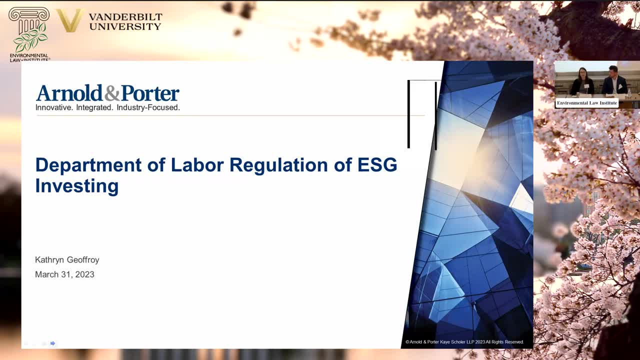 think that's a good place to start. And then also, as both the authors noted, this is an area where there's been a significant amount of development, And so I think that's a good place to start. And so I think that's a good place to start, And so I'm just going to provide some updates to kind of 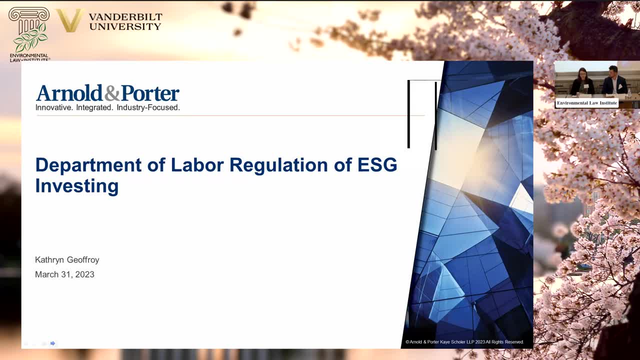 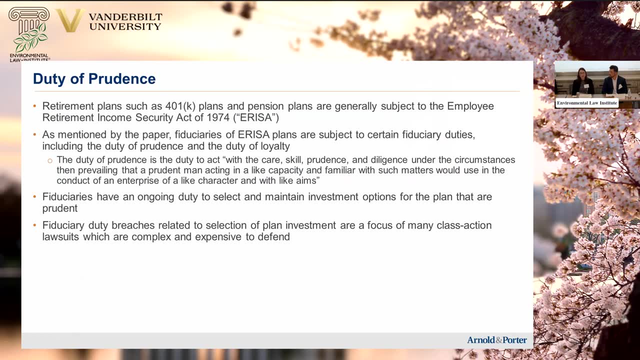 level set. so everyone understands the current legal landscape. Next slide. So underpinning much of this area is the Employee Retirement Income Security Act, which is also known as ERISA. Retirement plans, such as 401 plans and pension plans, are generally subject to ERISA, And ERISA contains certain fiduciary duties which apply. 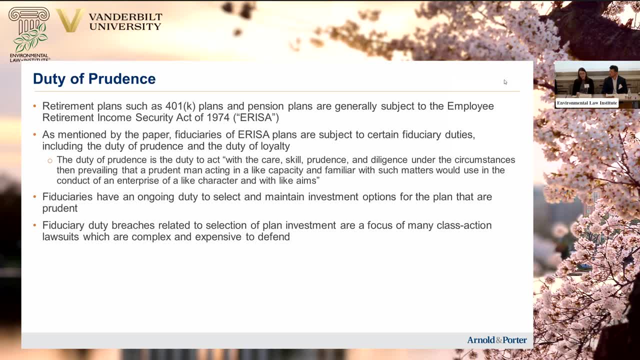 ERISA And ERISA contains certain fiduciary duties which apply to retirement plan fiduciaries. So, for the purposes of this presentation, I'm going to focus on the duty of prudence, because the duty of prudence, you'll see a definition on the slide, But in this 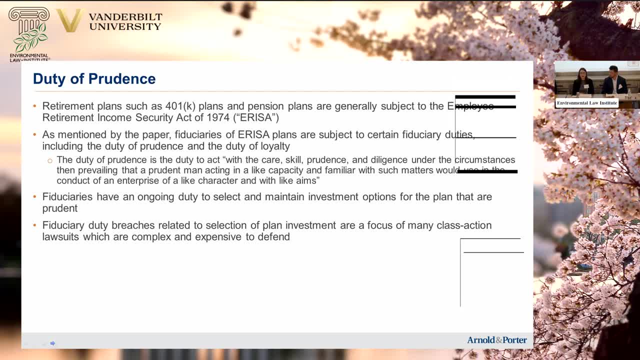 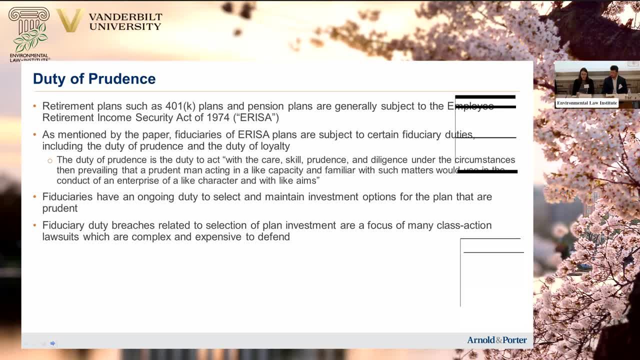 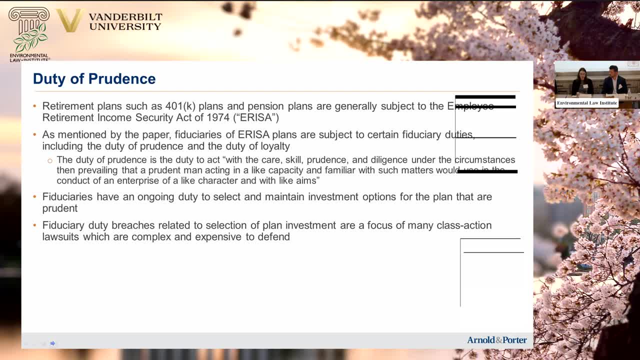 So fiduciary duty breaches relating to selection of plan investments is something that there have been a significant number of class action lawsuits relating to and increasingly, especially after case that was decided in 2022 by the Supreme Court, these cases are increasingly getting. 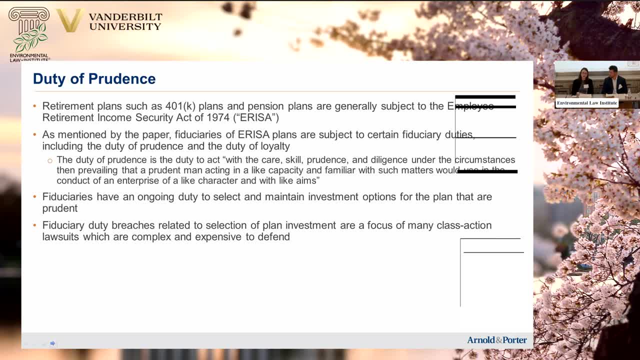 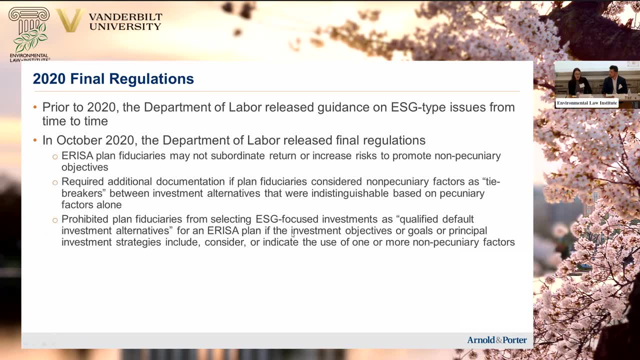 more difficult, more complex and potentially more expensive to defend Next slide. So, with all of that context, prior to 2020, the Department of Labor did have sub-regulatory guidance, which was issued from time to time, that addressed these sorts of ESG-type funds. 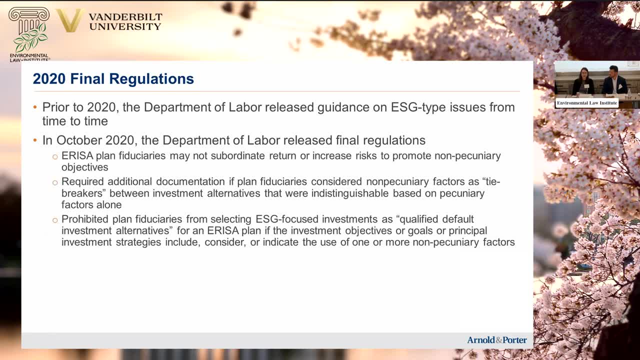 But in 2020, the Department of Labor actually released final regulations. There are a few key takeaways which I wanted to highlight in relation to the 2020 regulations. First, ERISA plan fiduciaries were not able to subordinate return or increase risk to promote. 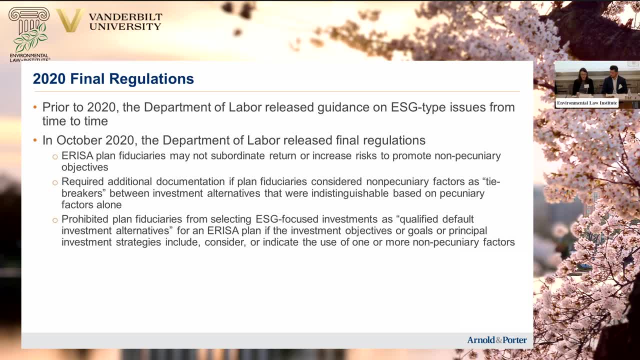 non-pecuniary or non-financial considerations. Second, if there was a tiebreaker, so if a fiduciary was able to subordinate return or increase risk to promote non-pecuniary or non-financial considerations. Third, if the fiduciary was looking at two potential investment options, that 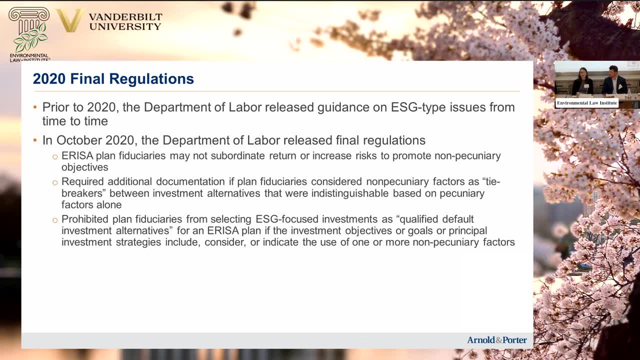 they were considering including in the plan and they thought that these two options were indistinguishable, based on pecuniary factors alone. then if they wanted to use non-pecuniary factors to kind of break that tie to decide which investments to include, they had additional. 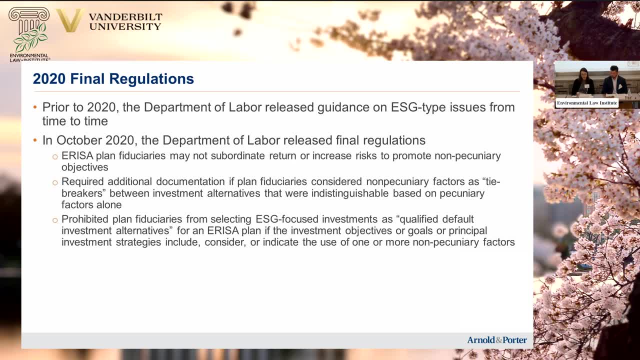 documentation requirements and disclosure requirements. And then the third takeaway here relates to qualified defense. So if the fiduciary was looking at two potential investment options, then ERISA plans had�. ERISA funds is not不 stu. So the 2020 regulation said that ESG-focused investments couldn't be used as qualified. 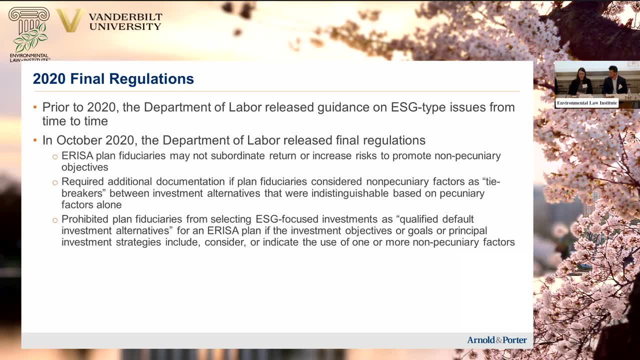 default investment alternatives for an ERISA plan if the investment objectives or goals or the principal investment strategies include, consider or indicate the use of one or more non-pecuniary factors. So it really limited the ability of fiduciaries to select ESG-focused investments as the default. 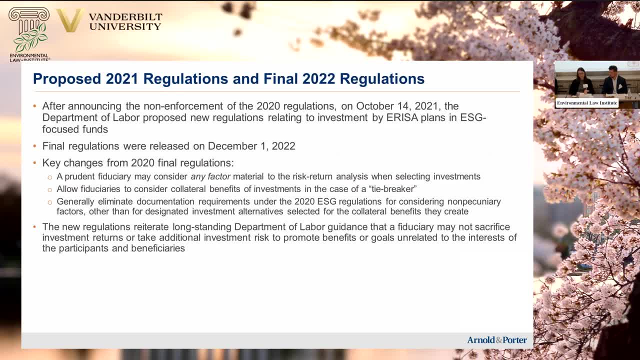 option for the plan Next slide. There was a change in administration and then, in early 2021,, the Department of Labor announced they would not be enforcing the 2020 regulation And then subsequently, later that year in October, they announced new proposed regulations. 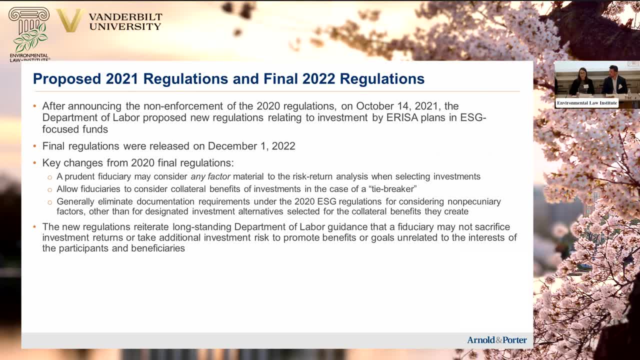 and then the final regulations were officially released In December of last year. So a few key changes from the 2020 regulations to the 2022 regulations. In the 2022 final regulations, a prudent fiduciary may now consider any factor that's material. 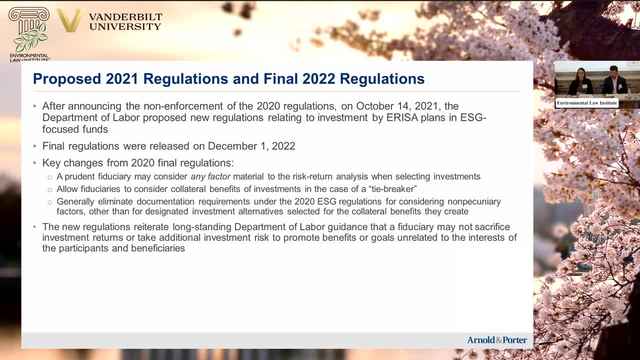 to the risk-return analysis, and this does include potentially ESG factors. Second, it allows fiduciaries to consider the collateral benefits of investments, and this is a very important factor. And third, it generally eliminates- with some exceptions it eliminates- some of the documentation. 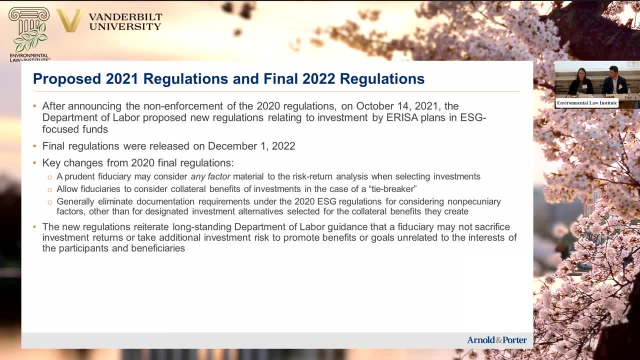 requirements that were included in the 2020 ESG regulations. So the 2020 ESG regulations were generally seen as limiting the ability for plan fiduciaries to select ESG investments as plan investment options. The 2022 regulations were generally seen as fraudulent. 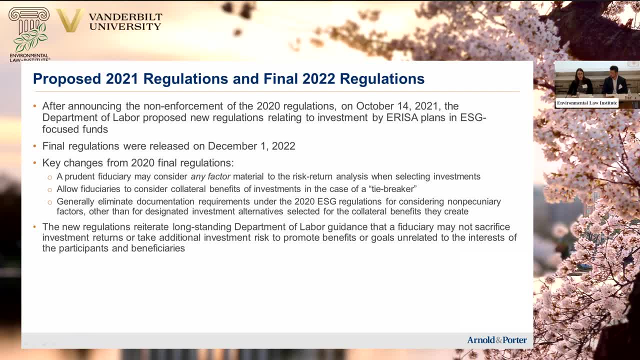 So the 2020 ESG regulations were generally seen as fraudulent. So the 2020 ESG regulations were generally seen as fraudulent. However, I do want to reiterate, kind of underpinning all of this: as I said, a lot of the fiduciary responsibilities derived from trust law. 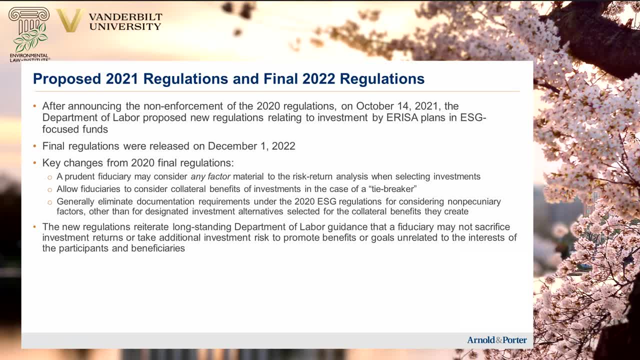 And so there's been long-standing Department of Labor guidance that a fiduciary has to focus on the interests of the participants and the beneficiaries. So even the 2022 regulations they reiterate this sort of long-standing guidance. A fiduciary can't sacrifice. 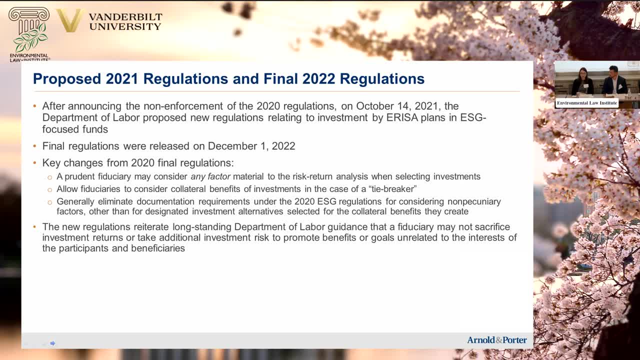 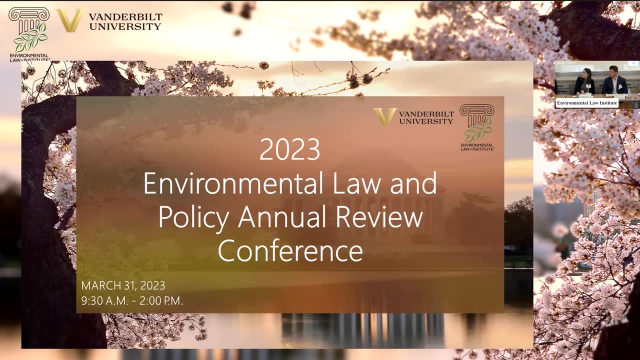 A fiduciary can't sacrifice investment returns or take additional investment risk in order to promote benefits other than the interests of the participants and the beneficiaries. Next slide: There should be one slide left. We've taken that out, Just to make it. 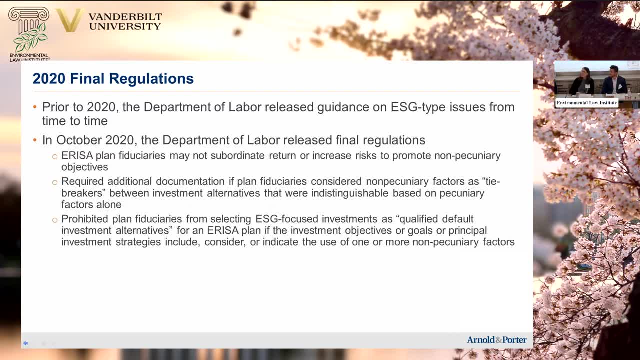 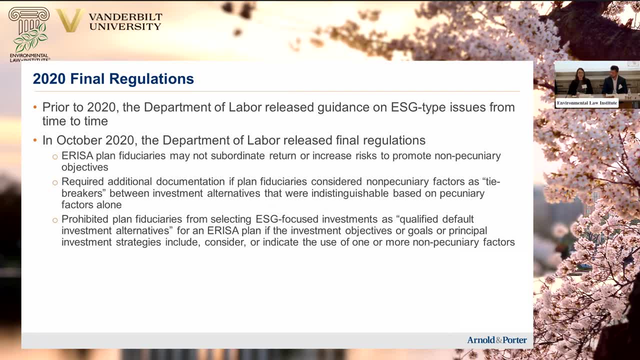 I'm sorry. I'm sorry. Next slide: It's fine. So the last slide. it just addresses some of the recent developments on ESG backlash. So, as the authors mentioned, this is an area that's become increasingly politicized. 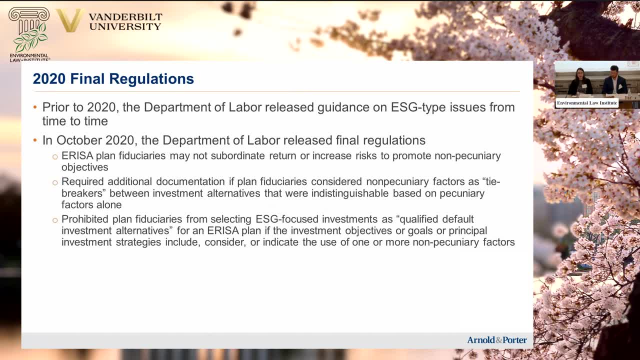 There's been a lot of political controversy, And so it's an area that's still currently under development on like a week to week basis right now. So, on the state level, several states have passed anti-ESG laws. Several states have had governors announce that no state pension funds will be invested in any investment vehicles that invest based on ESG principles. 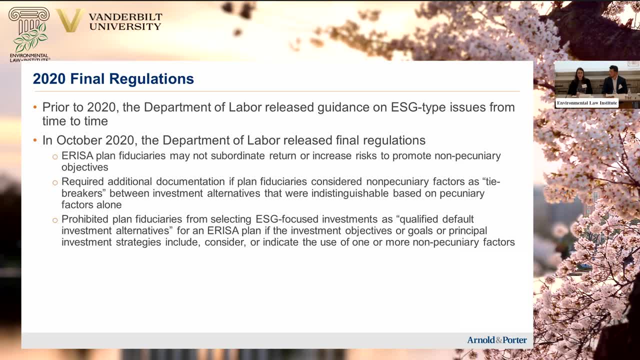 And then a coalition of 25 states sued the Department of Labor to try to prevent the 2022 final regulations from going into effect. On the federal level, there was legislation that was passed that sought to overturn the Department of Labor's 2022 final rule. 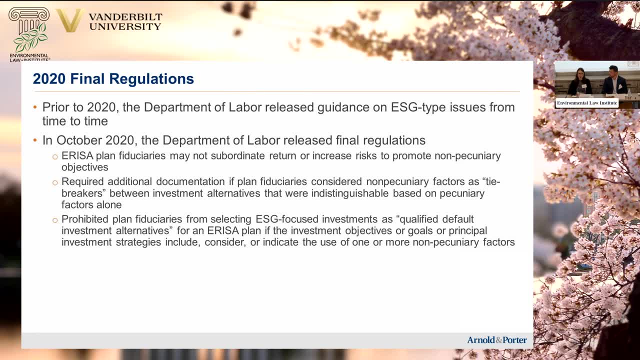 President Biden did use his first veto of this term on this, but the veto was not overruled, So it's not current law. But even since then there have been articles that have said that in the House there are already- there's already- some discussion of trying to create new bills. 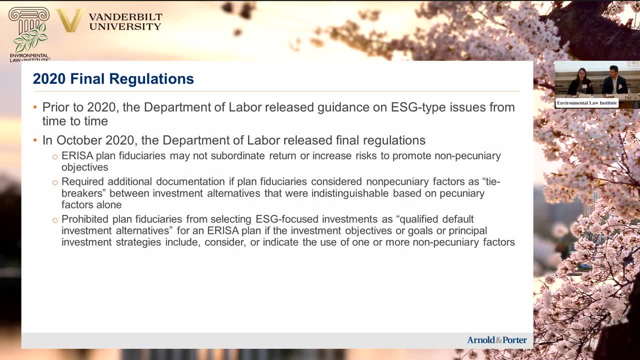 which would potentially revert essentially back to the 2022. Rule, where you're not allowed to include non pecuniary factors as a consideration when you're selecting plan investment. So that's sort of the current state of play. Obviously, things have changed even since the paper was published. 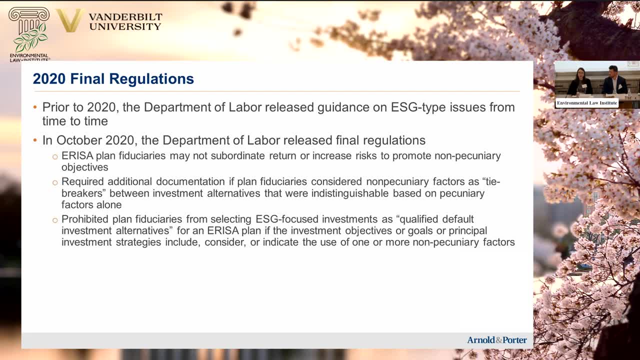 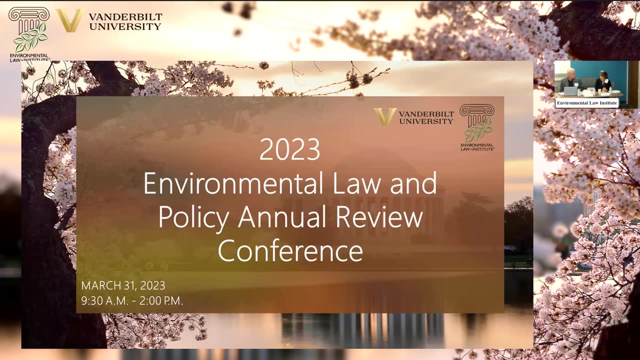 But that's just to provide some of the broader context of the decisions that plan fiduciaries are actually making when they're trying to decide what to include as investment options. Katherine, thank you. Yeah, that's just a really important angle On the issue. I do want to note it's one thirty. 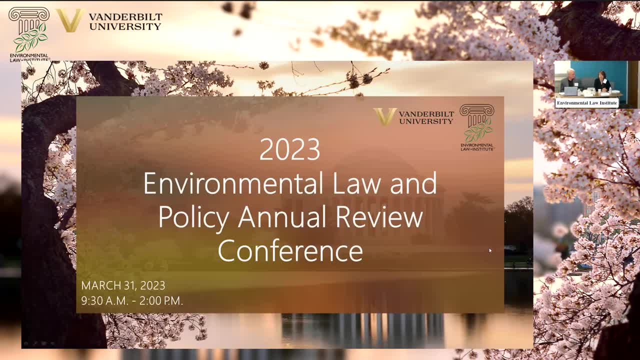 We made it from nine thirty to one thirty with no technology problems, And we now have to. we will post the full slide deck with your last slide And our next speaker. Steve, can you hear us? Indeed, I can, And I'm sorry that I am one of the two techno problems. 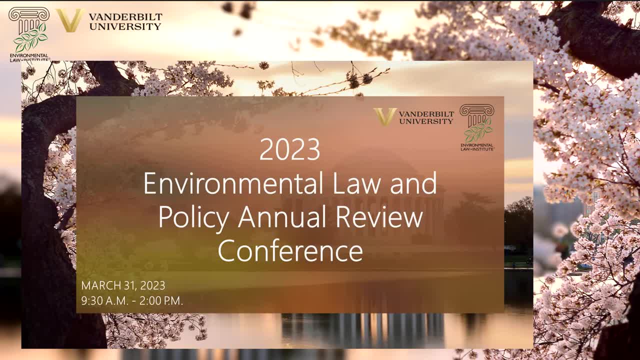 I just lost the feed, I don't know why. I'm very sorry. I'm still looking forward To the discussion And I'd love to read my my pitch, if I may Please go ahead. We'd love to hear from you And we're sorry we can't see you. 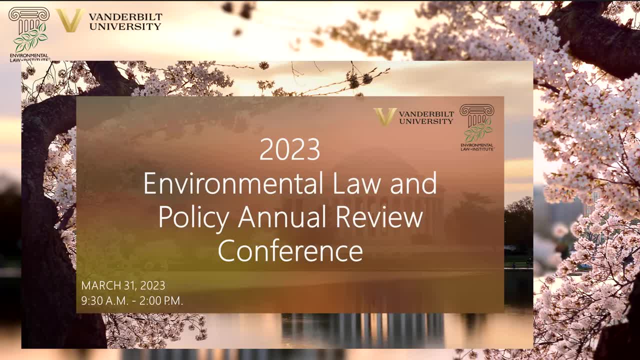 I do have an image of the room, fortunately because I was. I was connected a little while anyway, Greetings to everybody. As Thomas said, I'm Steve Hall. I'm the legal director and security specialist for Better Markets. I'm really happy to be here and grateful for this invitation. 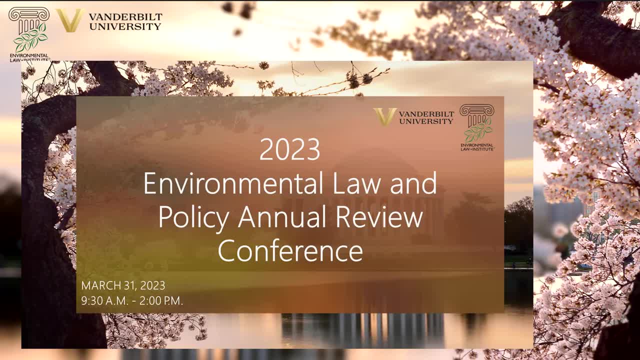 To participate in obviously timely and important topic. Better Markets is a nonprofit public interest organization. We were founded twelve years ago to fight for a more stable, fair and transparent financial system. A substantial amount of our advocacy is focused on improving the securities markets and fighting for important investor protections, including any fraud provisions, as well as clear and comprehensive disclosures. 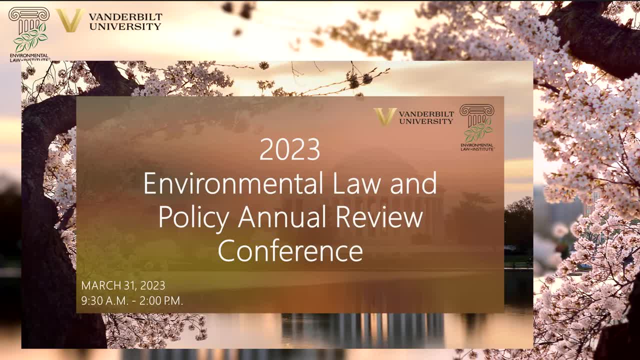 That investors need and want to make more informed decisions. ESG investing is the strategy for allocating investment funds on the basis of the extent to which the operations of a company or a portfolio of companies affect the environment, advance social justice or follow good corporate governance practices. 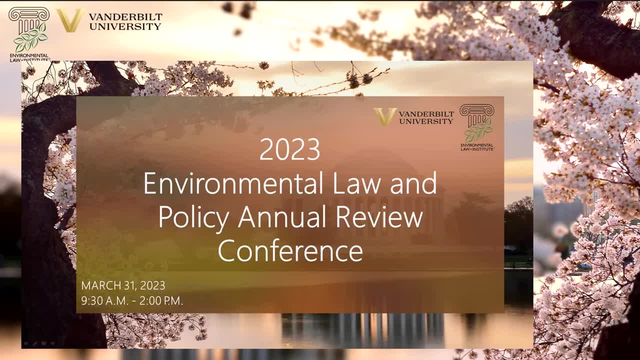 It's of intense and increasing interest to literally millions of investors who seek to minimize financial risk And maximize financial return. It also appeals to investors who seek to align their investments with their core personal values. Now the question before us today is how the sec and, to a lesser degree, the Dol 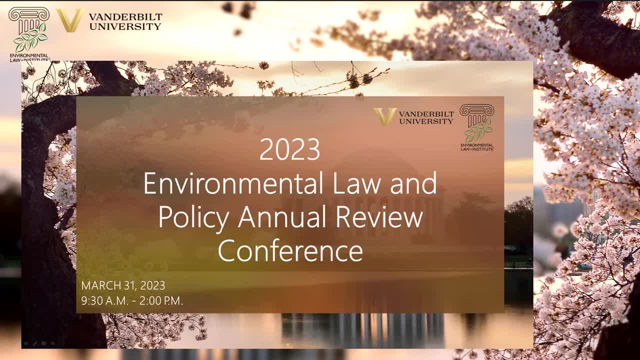 It regulates the Esg mutual fund market. The three distinguished scholars on this panel conducted some empirical analysis to gauge the need for additional regulatory oversight in this area. Now, taken at face value, Without delving into the methodology, We think the findings themselves are encouraging, at least as far as they go. 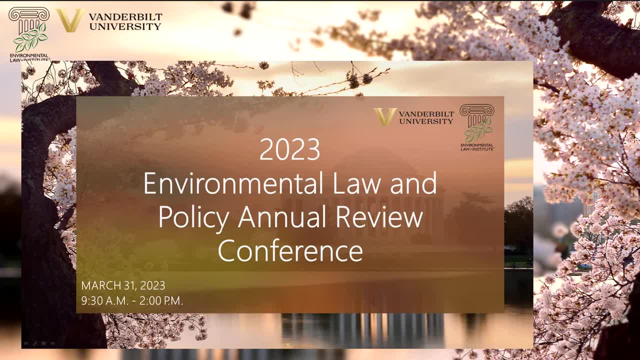 Their analysis indicates, indeed, that Esg funds really do offer their investors increased Esg exposure. They vote shares in ways that support the Esg principles, and they do so without increasing costs or reducing returns for investors. To the extent This is true. 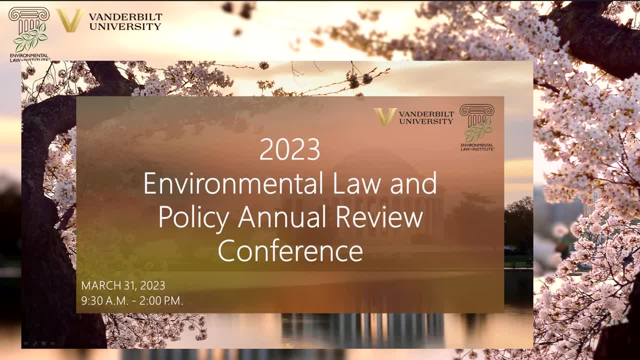 These findings actually bode well for the Esg investment movement, But a key question is what conclusion should follow from these findings. The authors contend that, in light of their study, there is no real reason to single out Esg funds for special regulation, or what they refer to as regulatory intervention. 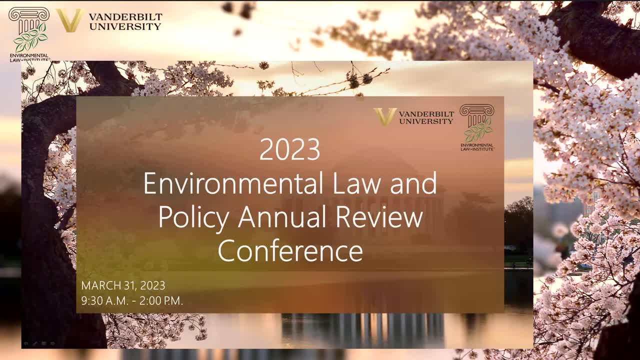 Now, here we part company, at least to a degree. First I'll note a little bit of common ground. to the extent the authors oppose regulatory attempts to limit investor access to Esg products, We agree with them And for that reason we oppose the dol's ideological and misguided attempt to inhibit the use of Esg investments by a risk of fiduciary. 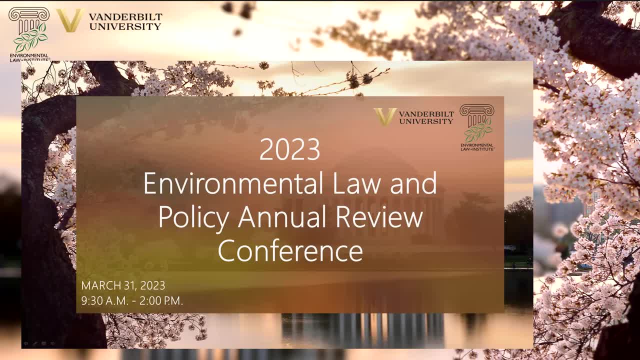 Fortunately, as my colleague on the panel has noted, the dol amended the rule and it recently survived the Congressional Review Act resolution of this approval, Thanks to President Biden's first veto. However, our core point is that there are still Very good reasons for additional regulatory requirements governing Esg funds. 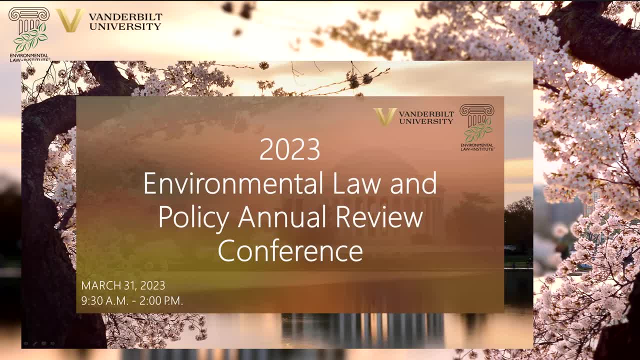 Such measures are necessary for at least 3 reasons: to protect investors from continuing abuse. to bring order to a complex and confusing market by requiring clear, standardized and comparable disclosures. and to maintain investor confidence in the integrity of this evolving market so that it ultimately can fulfill its potential. 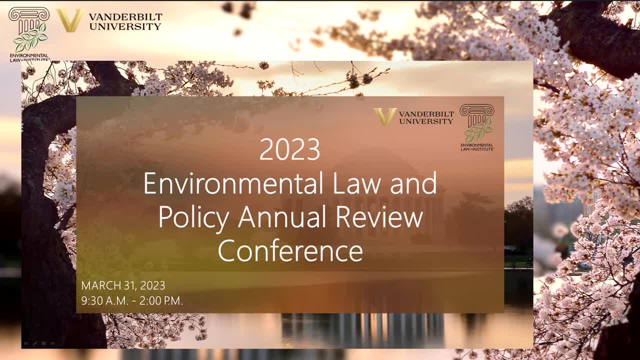 In short, regulation of the Esg market is necessary not only to protect investors, but also to foster an environment in which it can thrive. And indeed the sec is- I'll explain in a minute- is headed in this direction by proposing 2 important rules: one, to prevent the use of misleading mutual fund name. the other to provide investors in Esg funds with more detailed, consistent and comparable disclosures. before briefly fleshing out these points, 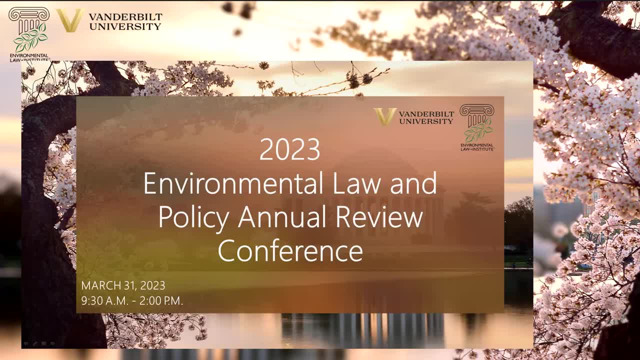 It's important To highlight the attributes of Esg investing that largely influence influence our thinking on the need for additional regulation. Esg investing is in huge demand. it's experiencing explosive growth. It's attracting trillions of dollars of investor funds. It has spawned a complex and confusing Esg investment industry. 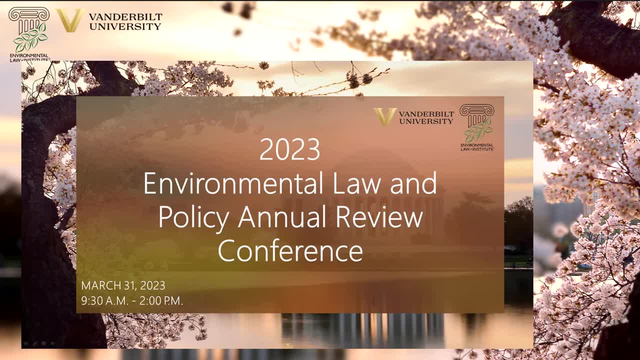 It offers attractive profits for mutual funds that can take advantage of investors. It has an appetite for Esg investing and there's every reason to believe that these trends will continue and increase, as the vast majority of millennials favor Esg investing. at the same time, 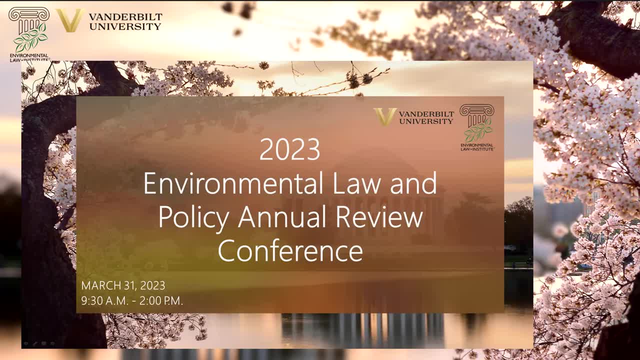 Investors are confronted by a daunting array of investment options and a lack of clear and consistent information about those options. There are hundreds of mutual funds. There are hundreds of Esg rating providers using different methodologies and countless Esg indexes that track companies using various Esg metrics. 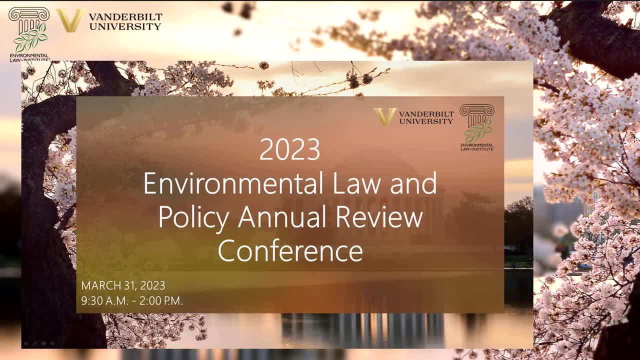 And, as the authors know, there isn't even a common, clear definition of what exactly Esg means. So, given this backdrop, the threat of investor abuse remains high. in our view, In addition, the need for greater clarity, uniformity and comparability in the disclosure of information about Esg. 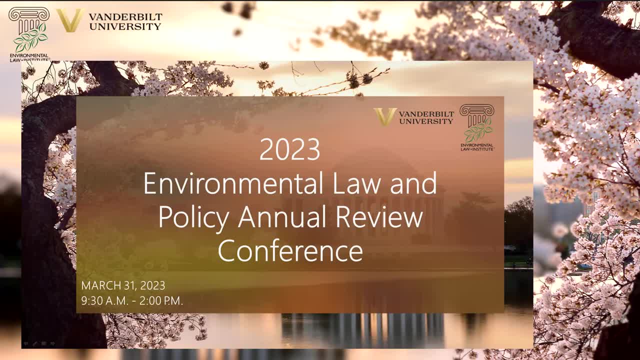 Investing should be clear. The case gets even stronger given the appropriate role for preventive regulation. Given the massive scale, popularity and importance of Esg investing, the optimal approach, in our view, is to get ahead of potential and foreseeable problems. As the Dc Circuit has said, regulatory agencies have the latitude to adopt prophylactic rules to prevent potential problems before they arrive. 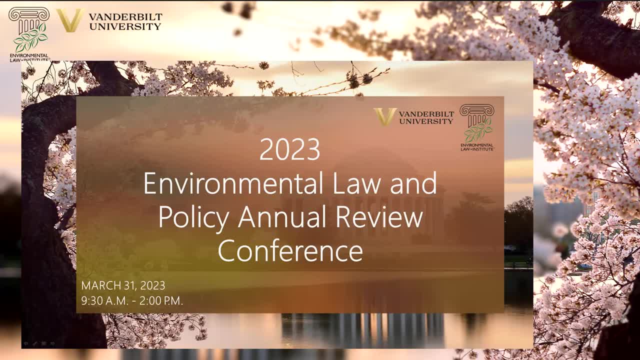 Quote: an agency need not suffer the flood before building, Before building the levy. Close quote: Even if the mutual fund marketplace were generally in good order, the Sdc Would be justified in establishing more guard rails to head off future problems. Now i'll sort of wind down by briefly touching on the 3 reasons that I flag that explain why we think additional regulation makes sense. 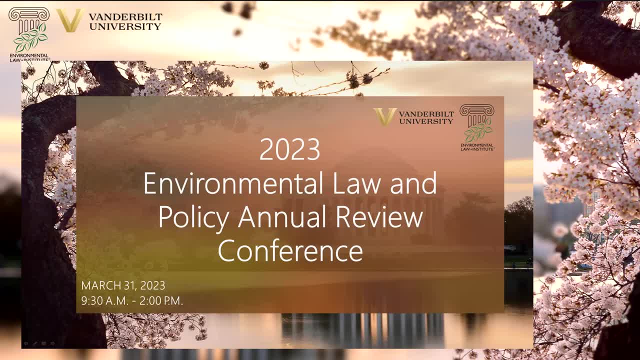 Investor protection, disclosure and market integrity. According to investor protection, of course, there have been and continue to be patterns of misconduct in the world Esg focused mutual funds and and they warrant strong enforcement as well as regulatory measures, and the Sec's actions reflect these concerns. 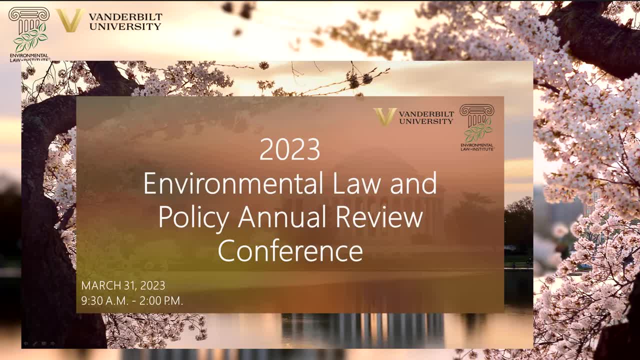 In March of 2,021, the Commission announced the creation of the climate and Esg task force within the division of enforcement to focus on inadequate and misleading Esg related disclosures. A month later, In April of 2,021., The Esd 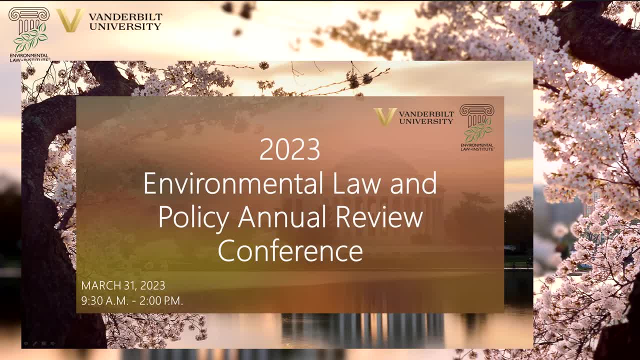 I'm sorry that the Sec's division of examinations issued a risk alert. It found that the rapid growth and demand increasing number of Esg products and services and lack of standardized and precise Esg definitions present certain risks. The alert went on to discuss several specific observations of deficiencies and internal control weaknesses identified during the examination of investment advisors and funds. 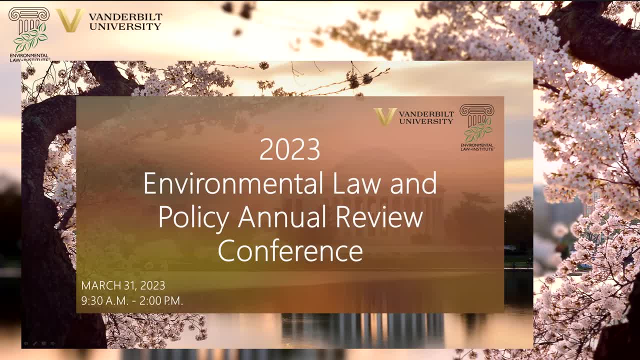 With respect to Esg invested And, of course, the Commission continues to bring enforcement actions against issuers and funds for misconduct and climate and Esg related disclosures. Now, beyond enforcement, the Sec has also taken regulatory action to address potential abuses in the Esg marketplace. 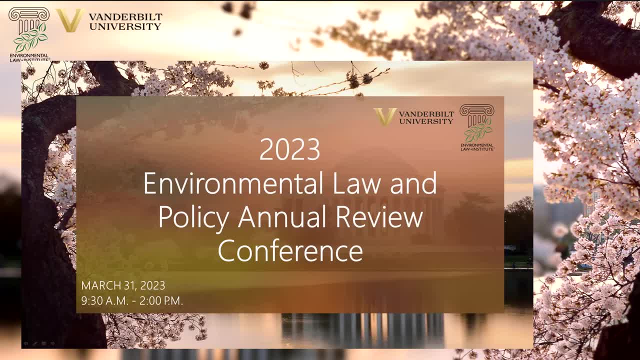 In June last year it published a proposal to fortify what's known as the names rule. That rule already requires funds to adopt the policy to invest At least 80% of their assets In accordance with the investment focus that the fund name suggests. 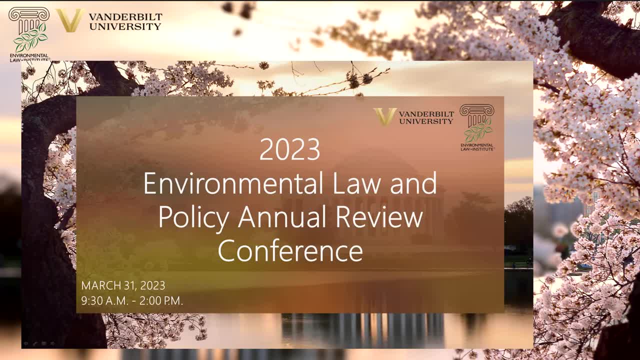 The recent proposal would expand this requirement and apply it to fund names indicating that the funds investment decisions incorporate the Esg factors. The rule would also require enhanced disclosures about how fund names track their investments, as well as perspective definitions of the terms used in a fund's name. 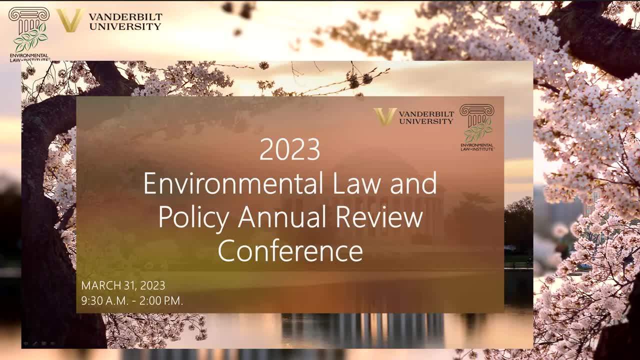 The second area where regulatory intervention is especially important is in the realm of disclosure. The fact is that investors do not have access to clear, consistent and comparable information on which to base their investment decisions when it comes to Esg investments, And the sec has moved on this front as well. 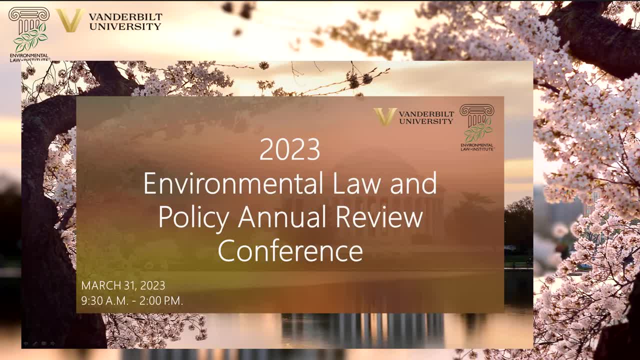 In June last year, along with the names rule, it published a proposal that would require investment companies to disclose to investors and report to the sec additional information regarding their Esg investment strategies. The sec's release actually nicely frames the core rationale for the rule. 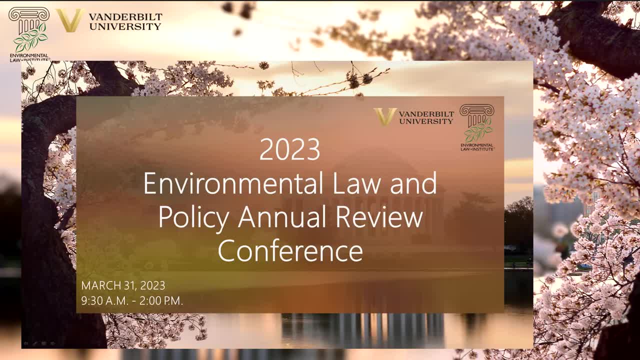 It says, quote: The proposed rules and form amendments are designed to create a consistent, comparable and decision useful regulatory framework for Esg advisory services and investment companies to inform and protect investors, while facilitating further innovation in this evolving area of the asset management industry. 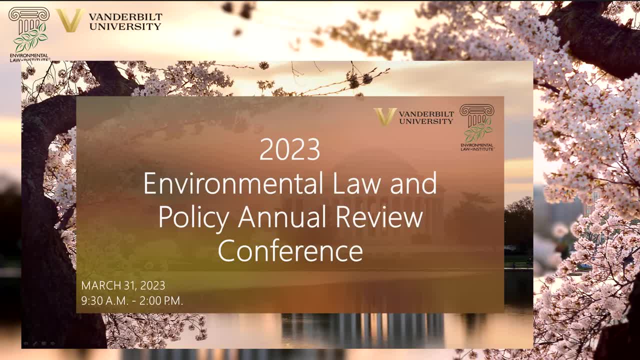 Close book. The sec's reference to innovation is a good segway to the third and final reason why we support additional reform in the Esg investment market. Additional regulation of Esg funds will actually help this important movement thrive. New protections and requirements, including those the sec has recently proposed, will satisfy investor demand for the accurate, complete and consistent information they need to make optimal investment decisions. 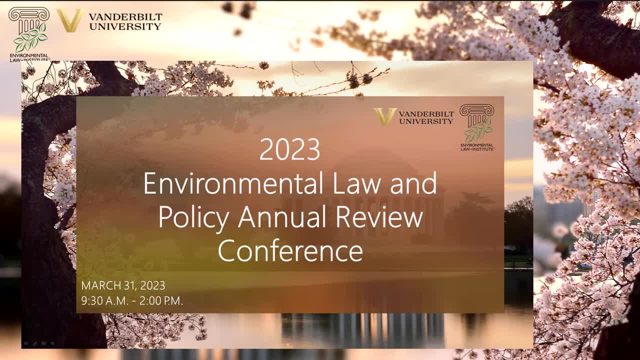 They will fortify investor confidence in the integrity of the Esg market. In short, strong regulation means investor trust, which means greater investor participation, which means more efficient capital allocation, better returns and more social good. And these benefits accrue whether investors are seeking Esg related investments to save the planet or to read better financial returns from companies that are well positioned to adapt and profit from climate change. 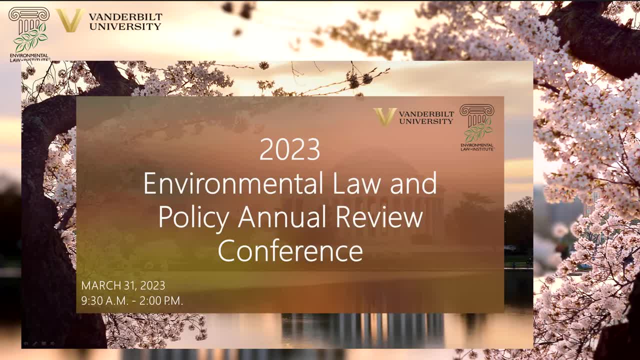 Thank you, I appreciate the touch. Thank you Great, Great, And with that I will turn to the next participant. The future of development will be determined based on sustainable development and social trends. That concludes my opening remarks. Very much look forward to the discussion. 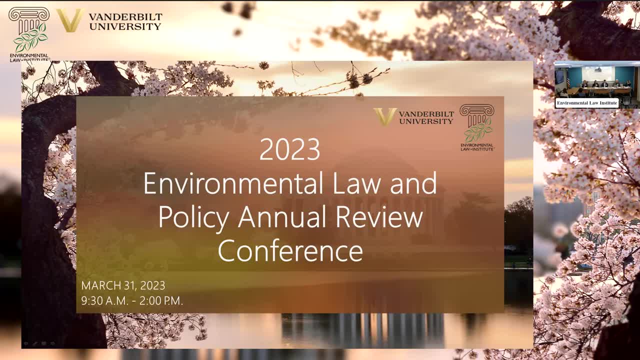 And once again sorry to be remote, by phone only, But still looking forward to participating. Great Thank you, Steven. We can hear you very well And appreciate your comments, And I suspect we will be circling back in the discussion to your recommendations. 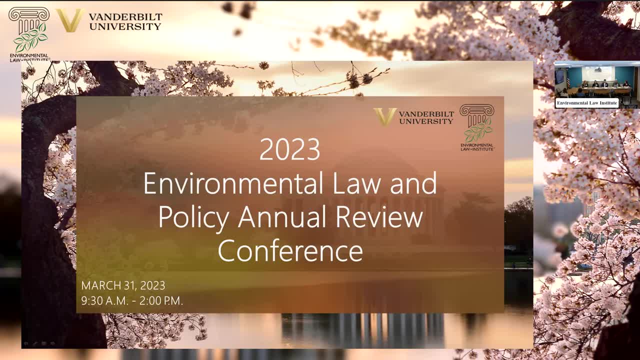 go to Anne. Thanks so much. Really appreciate the invitation. So much to say in so little time, And now I'm filled with thoughts about Steve's wonderful presentation as well. In a nutshell, I just want to remind you that Ceres is actually a coalition of investors Started in 1989. 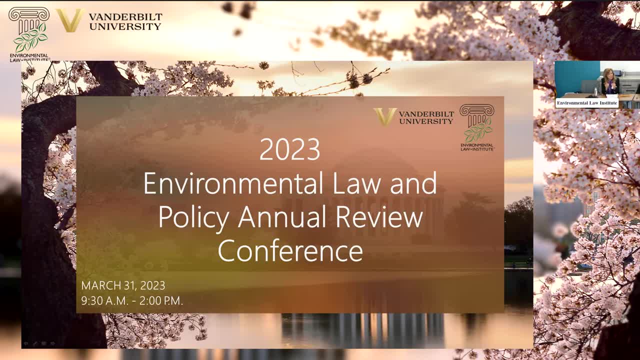 in the wake of the Exxon Valdez spill, The sense of investors really wanting to do more than the law would allow them to do when it came to the performance of the company. We started out with a few socially responsible investors before that was a tarnished word: Religious investors. 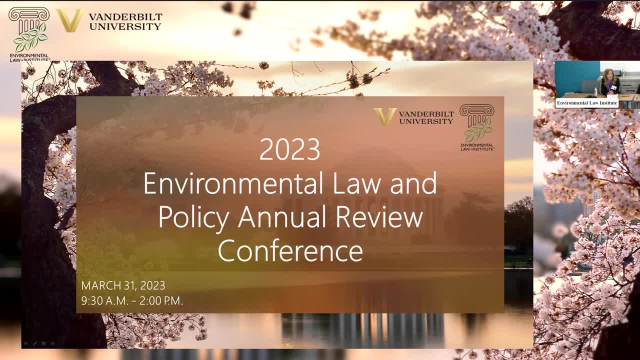 probably about half a trillion AUM assets under management. That network has grown profoundly to include all kinds of asset managers and asset owners, including BlackRock, CalPERS, CalSTRS- about $37 trillion of assets under management. Obviously, we know we own none of that. 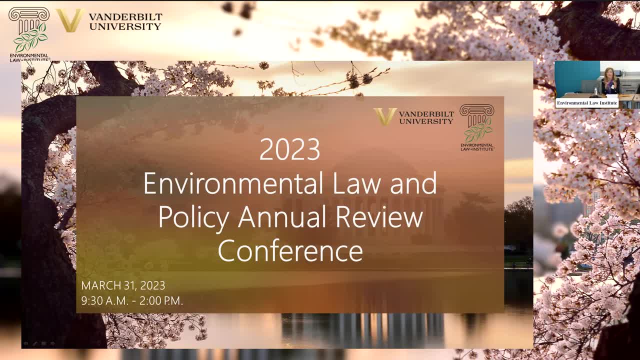 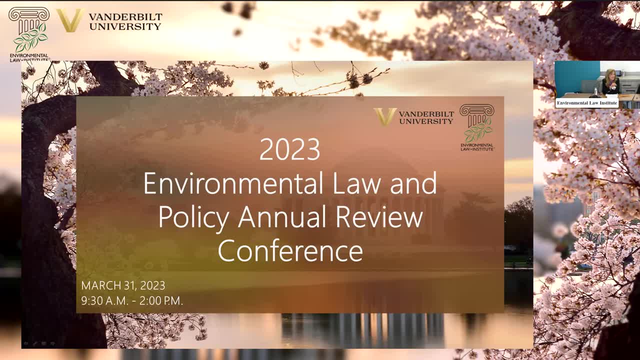 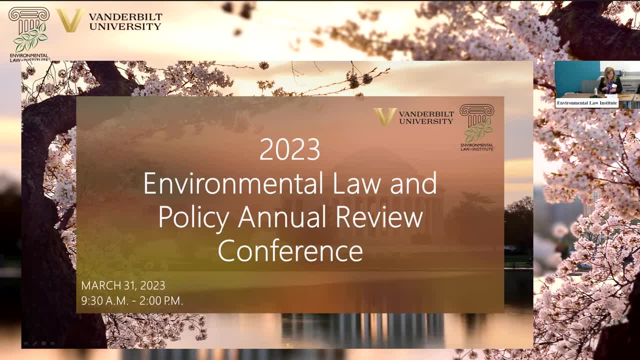 I'm completely biased. I'm an advocate. That's why I'm here. That's why I'm here. So, thank you. I was going to own that right up front and I can thank you for the invite. I haven't been. 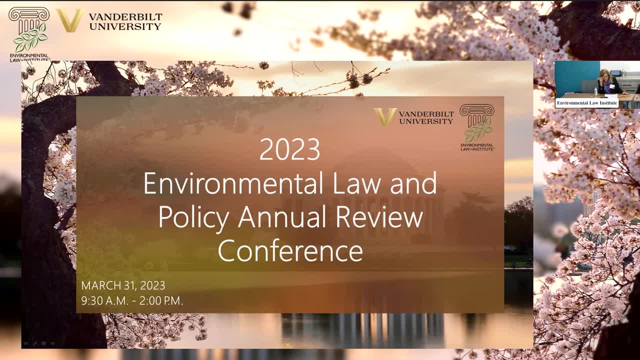 to the line for about 20 years and it's terrific to be back. I love the article. Thank you, Jill. Thank you, Adriana. A fantastic piece. Really needed to put this out. I could talk about so many of their conclusions that made perfect sense to us. 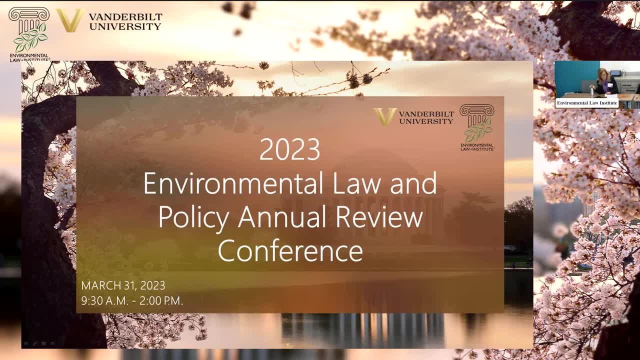 And one thing that leaps out at me, and I don't necessarily disagree, Steve, with the tweaks- and I'm going to call them tweaks- that you just suggested by the SEC. Thank you for noting that most millennials support ESG. if that isn't enough of a reason, 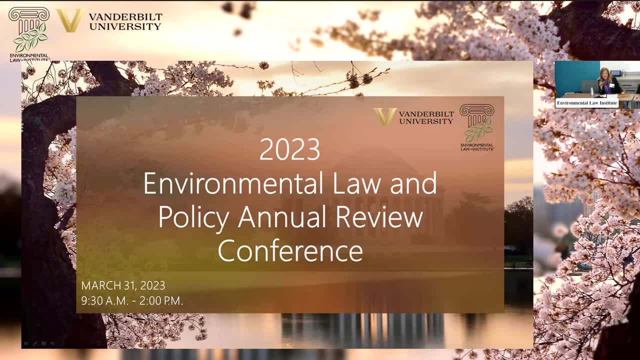 to get behind it. I'm going to guess there's millennials and Gen Zs in this room, But you, I want to make a really clear distinction between the kind of what Steve's calling for is legitimizing this area, getting more disclosure. 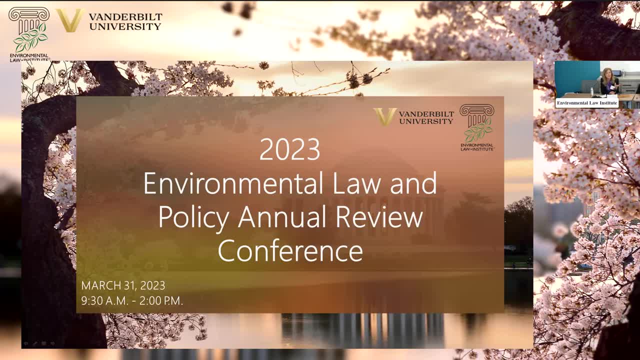 We, of course, support robust disclosure. Investors in fact need neutral, clean, decision-useful information, And that's why we so robustly support the SEC's rule around enhanced climate risk disclosure. That's what's going to lead to the fair allocation of capital. 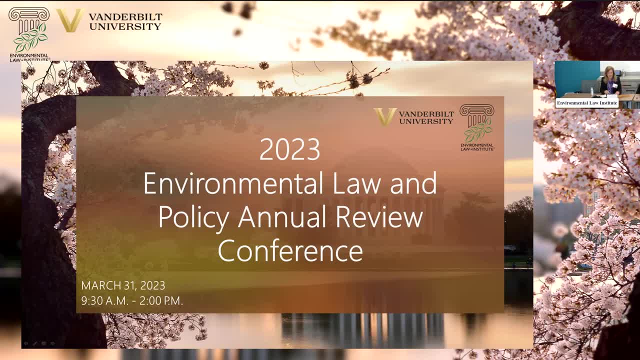 If you can understand the nature of the climate risk, then investors need to make that decision. But I want to make a distinction between the kind of tweaks Steve is talking about, for clarity, for naming, and the kind of unfortunate activity that we're seeing at the state level that I'll refer to in a moment. 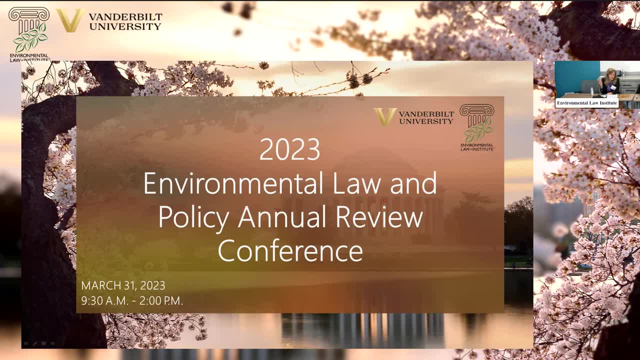 One thing about naming that Steve mentioned. I do want to point out that our authors were really astute. I thought in their discussion of other funds, Something's called a growth fund. What's growth? People get into something called a blue chip fund. 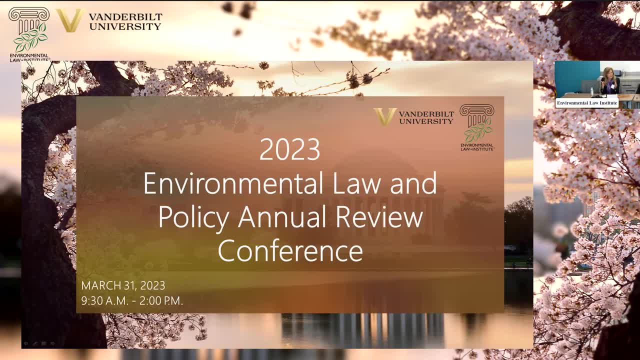 Really, what's that? So the rule is 20 years old, the naming rule? So, yes, if we're going to do that, let's look at all these funds. And I really appreciated the way the authors put this in context and concluded well. 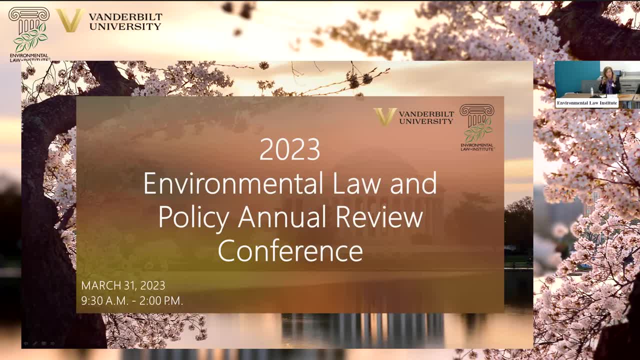 there's no extra regulatory layer needed from either the SEC or the DOL for this set of funds that you might not apply to other sets of funds. That said, what I hear Steve saying is that this area is important. It should grow. He actually used- I think he actually used- social good to become a bad word at the state. 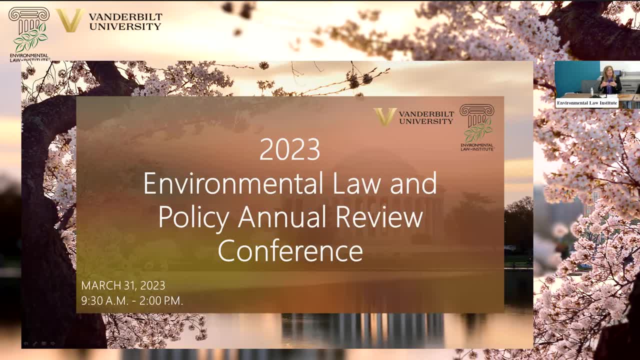 level with certain parties, And so, to make it even better what I'm hearing Steve saying- and he'll contradict me if I got that wrong- to make this even more robust, there's a reason why this is growing. Some tweaking is probably in order. 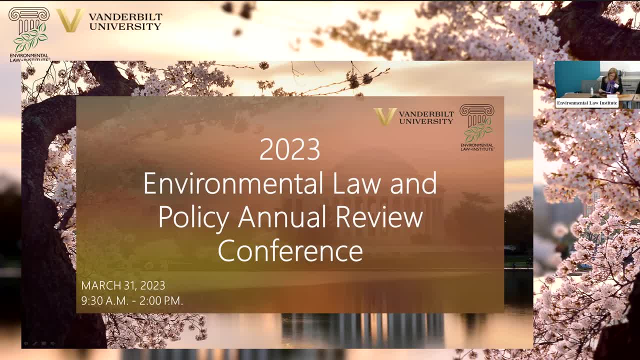 And Steve, I can't disagree with you there. What a wonderful time to be in law school. The thing you get to do in law school is to go over cases and law, some of which, with the benefit of hindsight, you say, oh dear God, what were they thinking? 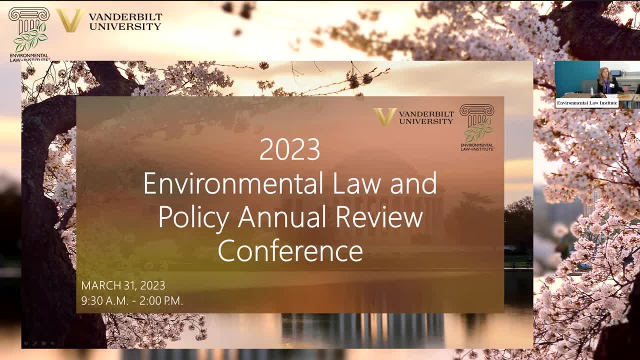 Plessy versus Ferguson, the Jim Crow laws, the fact that women couldn't vote- Where do you begin? right? And there was no internet, then We didn't get those people passing those laws didn't necessarily get to know the political. 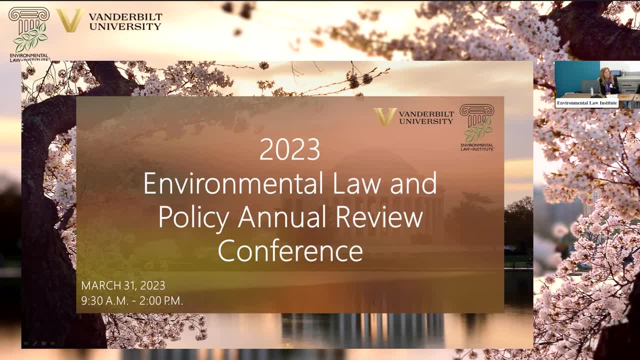 dynamics around those decisions the way you can. So you are seeing in real time just a stunning set of development at the state level in this area, And it allows you to really say: well, now, wait a second, how is this going to be looked? 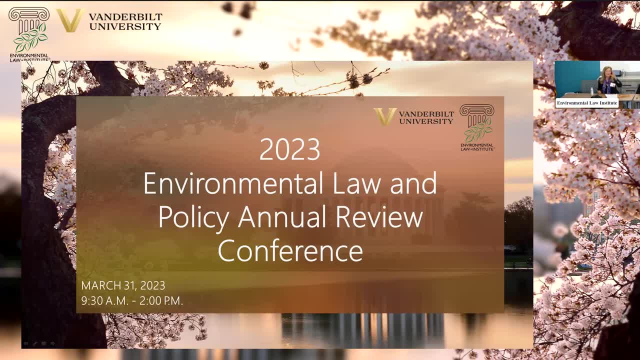 at in 25 years, in 50 years, in 100 years? What was that? in the 2020s, Let's see now. they had seven years at that time before complete and total climate destruction. OK, And so some people were trying to shift their funds to avoid climate risk and to participate. 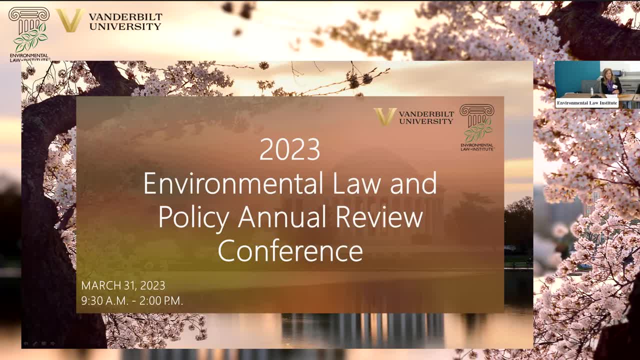 in the opportunity of renewable energy. How dare they? So you'll be able to- and I know that when you're reading the law now, you're thinking about this- such that you're able to separate clear legal matters and controversies from what is strictly political theater. 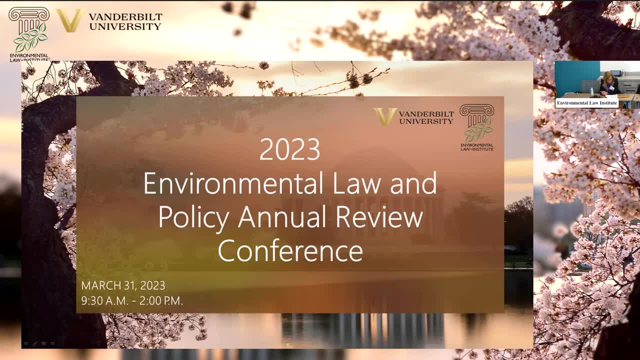 Larry Fink, for what are investors thinking and doing and why Larry Fink? chairman and CEO of BlackRock for years now we do climate risk and investment risk. That's still the case. One of those critical tasks of an asset manager is to provide clients with insights on short. 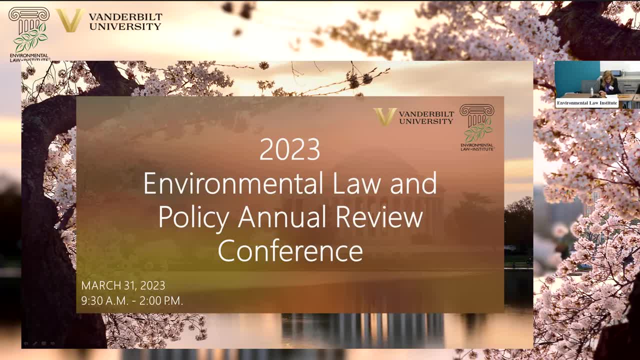 and long-term trends in the global economy. Climate risk is such A trend. We believe that companies that better manage their exposure to climate risk and capitalize on opportunities will generate better long-term financial outcomes. Climate risk is financial risk. That is the cold, hard fact to ignore. 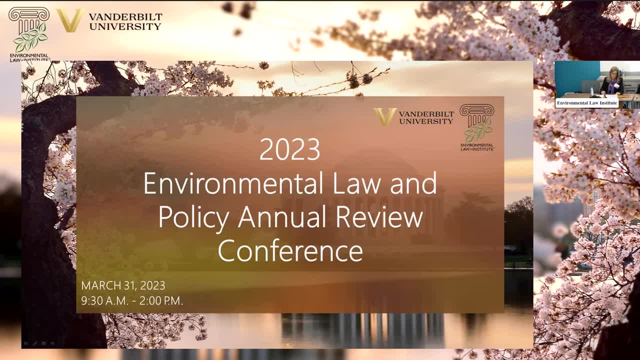 It would be a dereliction of duty, Michael Farris, Illinois state treasurer. Kirstie Jenkinson of CalSTRS, the largest, second largest, pension fund in the country, ignoring pervasive risks such as market disruption by climate change, and ignoring the investment opportunity presented by the transition to. 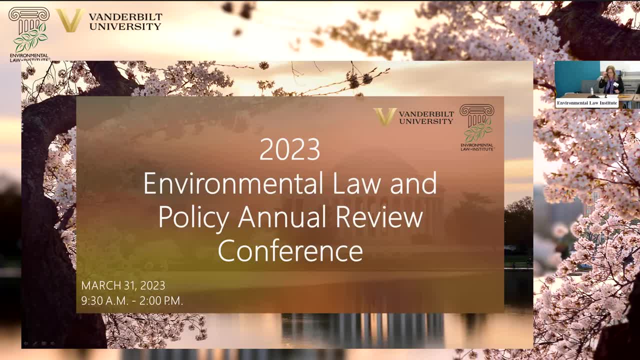 a low-carbon economy is asking us really to stop doing our jobs, So I appreciated the detailed description of fiduciary duty. Understand: investors really want to make money. That's what we want to do If the marketplace is moving in this direction, as much as I'd love to believe that, Larry. 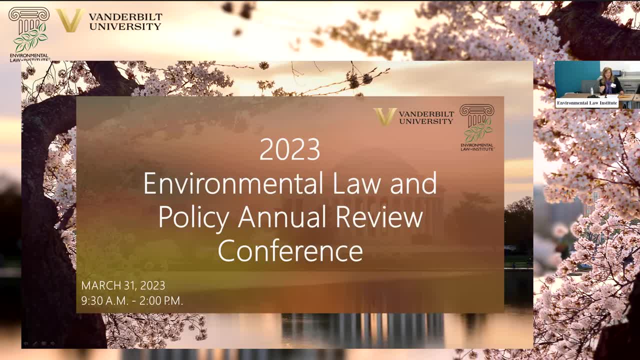 Fink has a great big heart and must do the right thing. the dude wants to make money. Let's just be honest about that. Most of these pension funds have to be thinking about long-term income. They have to be thinking about, They have to be thinking about a long-range plan for people like nurses and teachers, and 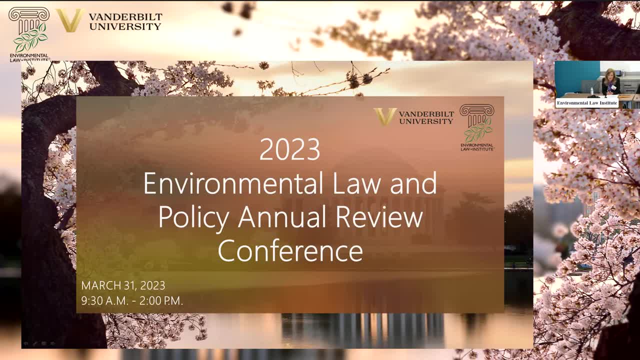 firemen who may not retire for 30 or 40 or 50 years. So that's their intention. That's what Kirstie Jenkinson, who represents a bunch of teachers, is getting at Ann Simpson, Franklin Templeton- we're not woke. 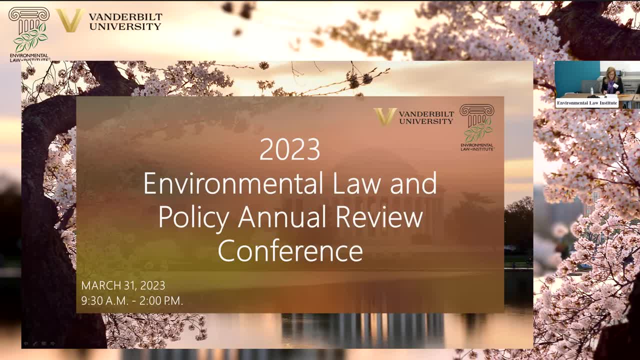 We're awake. She's the stability manager for Franklin Templeton, which of course has extremely conservative roots. She said: you know what we're about is prudence, loyalty and care. back to the definition of fiduciary duty. 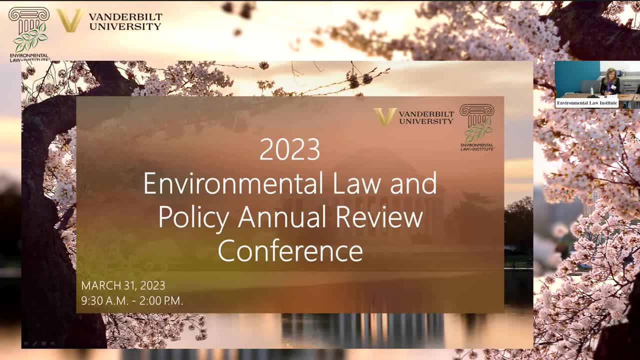 When it comes to ESG, her advice is: keep calm and carry on. This is somebody who's been at this a very, very long time, So I guess my point is: this isn't Greenpeace. okay, I love Greenpeace. 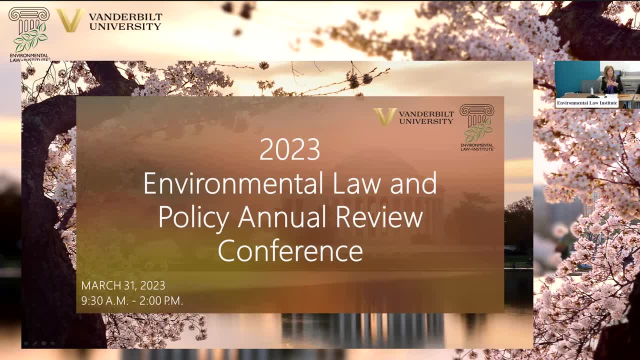 This is cold hard investment strategy where you're going to get, You're going to do prudent risk management and you're going to look for opportunities. okay, And so that's basically free market capitalism. And I have to quote here the governor of New Hampshire, Governor Sununu, Republican, who 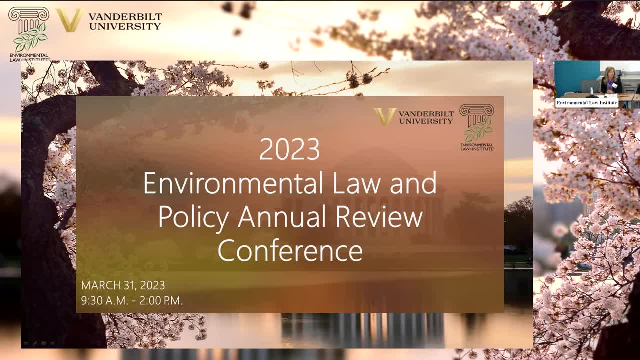 said, I probably don't love ESG, but it's not the government's rule to over-report And to start to determine where folks should make their investments. So, as a result of the overreach that I'm going to describe in a moment that Catherine referred, 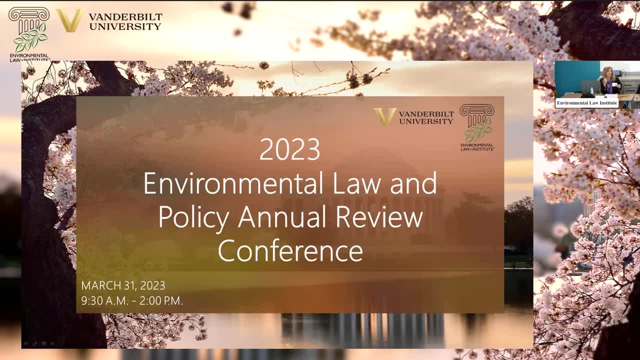 to. we launched a campaign last week called Protect the Freedom to Invest- and that's my button: Protectthefreedomtoinvestorg. It's just a whole lot of asset managers and asset owners saying: let's just protect the freedom to invest responsibly. 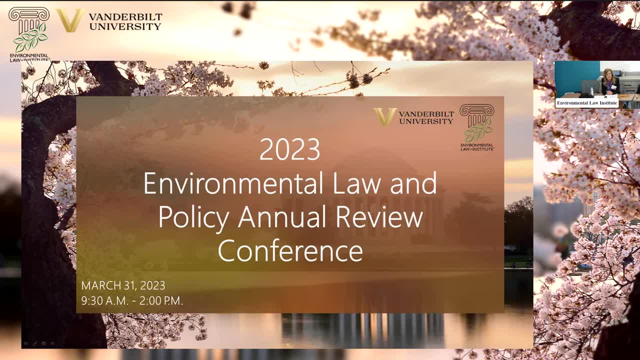 Allow the free flow of capital, which is a really conservative idea, and allow investors to make those decisions. We're in the whole realm of Again. not to say that some of Steve's criticisms were not warranted and that we could use tighter definitions, of course, more robust disclosure, more transparency, no question about it. 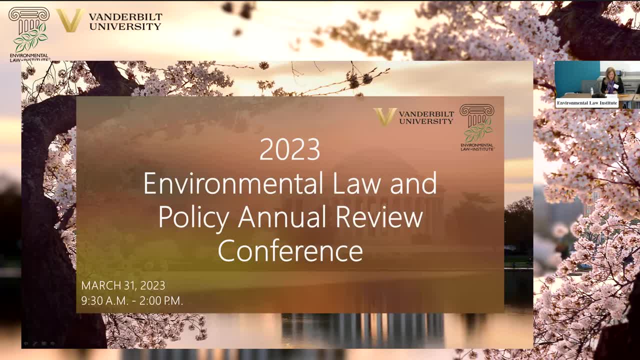 But basically it's a movement to say: do not restrict. Well, why was this necessary? More than 130 bills have been introduced so far this year that would restrict investing practices by limiting or prohibiting consideration of non-financial or non-pecuniary factors. 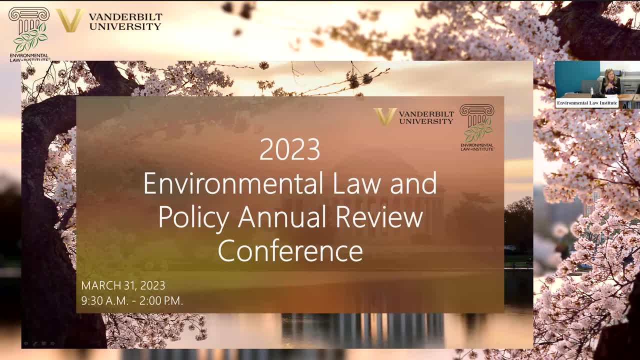 Well, here's where we have a point of controversy right away, don't we? We're calling it non-pecuniary. Well, that's funny because Larry Fink said climate risk is financial risk. I'll just tell you that Siri said that in 2003.. 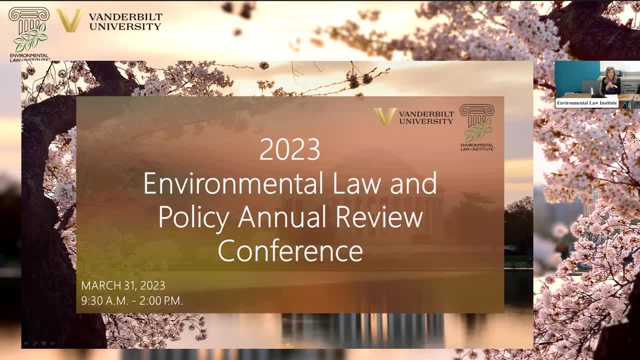 She was saying: no, it's not. What are you talking about? Now? Wall Street is saying climate risk is financial risk. I don't have to share with you the numbers about the weather disasters of the last year. Guess what. 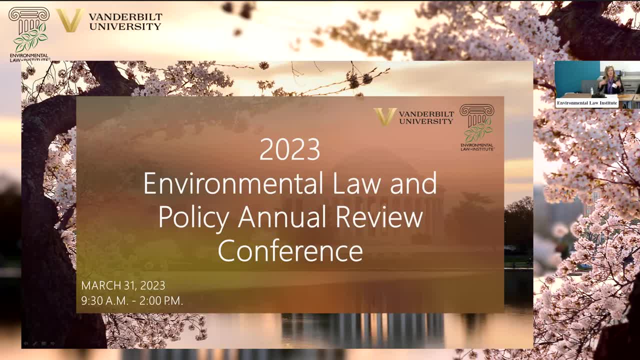 Business interruption. There's money to be lost, Damage happens. Taxpayers pay. It's financial risk. Again, it's Larry Fink saying that It's not our beloved environmental colleagues. In addition to the bills, There were bills that passed in Texas and West Virginia and Utah. 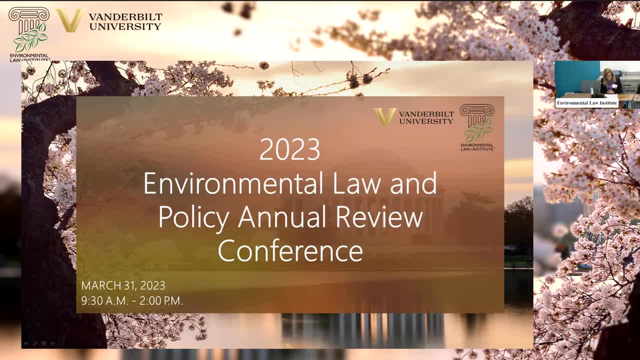 There's now- I don't want to, I can't go to time to go over them all- but in Arkansas and Idaho and Montana passing bills that would prohibit EAS considerations as an investment in pension funds. Okay, So again, this is partly a debate about long-term short-termism and I'd love our wonderful 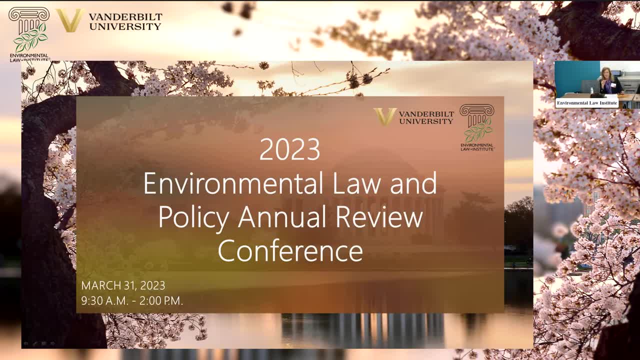 authors to take that on. Your business school colleagues are discounting the future. We have valued the short-termism. That's one of Wall Street's problems: not looking into the long-term. Simply because you look at long-term assets does not mean that you're doing anything. 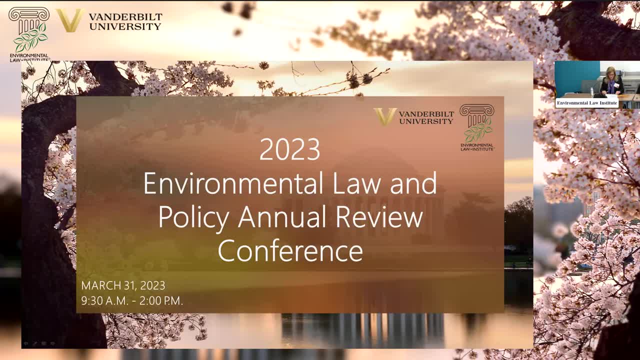 illegal. Our investors would suggest that's consistent with your fiduciary duty. I think it's important that many of these efforts, including those in North Dakota, Virginia and Wyoming, have been scuttled amid revelations about the millions of dollars in additional taxpayer costs that these policies would result in. 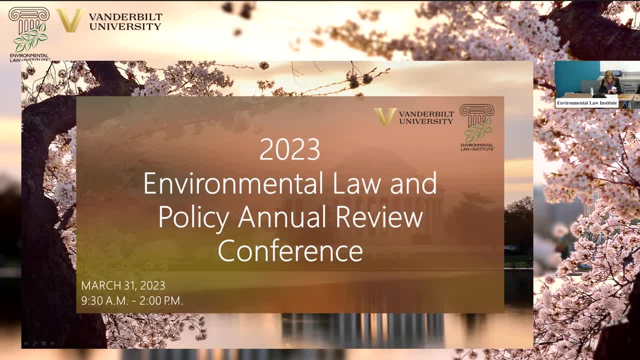 So a few examples. The Kansas State Division of Budget projected reduced returns of $3.6 billion over 10 years for the Kansas public retirement system. if the currently proposed investment restrictions were adopted, The Arkansas public employees' retirement system estimated they would lose $30 million. 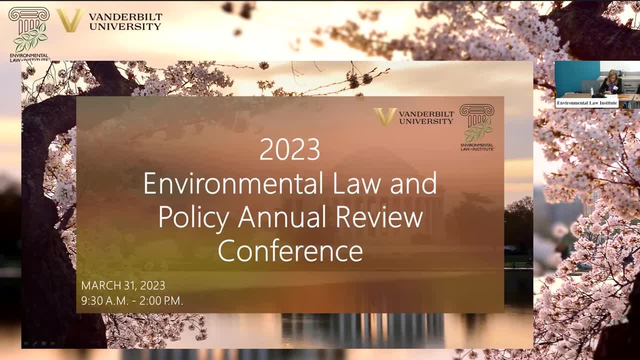 to $40 million a year due to an anti-ESG bill that would require the state treasurer and public entities to divest from certain institutions that use ESG metrics. Same thing with the Indiana public retirement system. It could result in reduced aggregate investment returns for defined benefit and defined contribution. 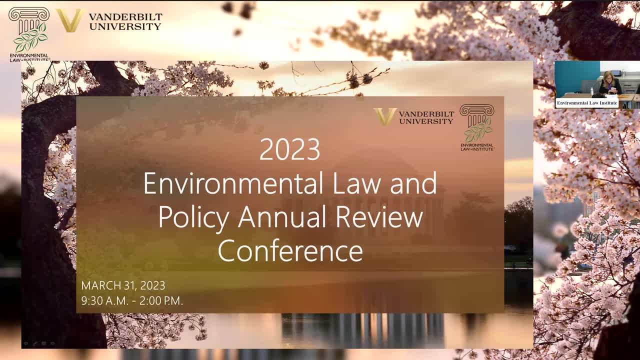 funds of $6.7 billion over 10 years. So it's set to decrease or reduce an estimated annual return of investment from $6.7 billion to $6.25% to $5.05%. You know that as fiduciaries, these folks have a statutory duty to return. 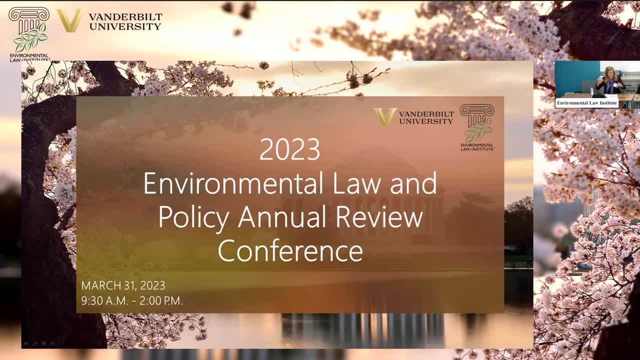 So what's going to happen then? Those employees are going to have to pay a greater contribution. So, as a result of what are called fiscal notes at the state level, fiscal note is like what the CBO does at the federal level. What's this thing going to cost? 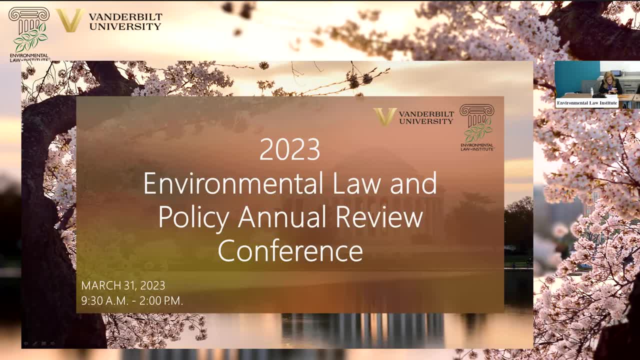 I'm happy to say that several bills have been defeated in Wyoming and Virginia, where the session is now over, in Colorado, New Hampshire, North Dakota, Mississippi and Tennessee. So when state many of these? if you look at the numbers, many of these bills are crashing. 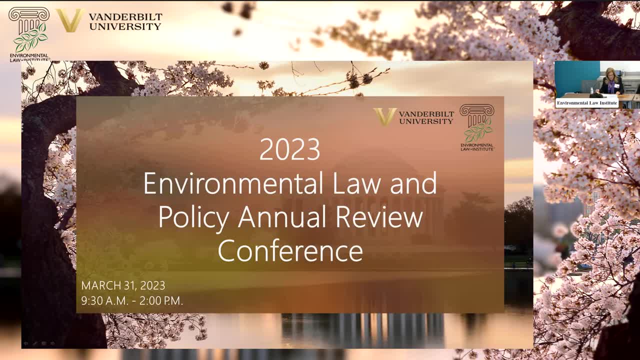 down. That's really important And again for our wonderful authors, were they to go back and do a little more analysis. it would be interesting to see you know what has happened to those states where the taxpayers were actually negatively influenced as a result of these bills. 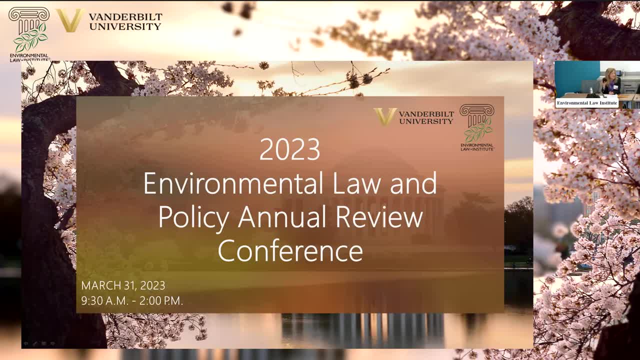 And you also have the benefit of looking at what's really behind these bills, What's really behind the effort. So using a word like wealth in such an inappropriate context, talking about someone doing something that might be good for people, how dare you? instead of having a financial return, 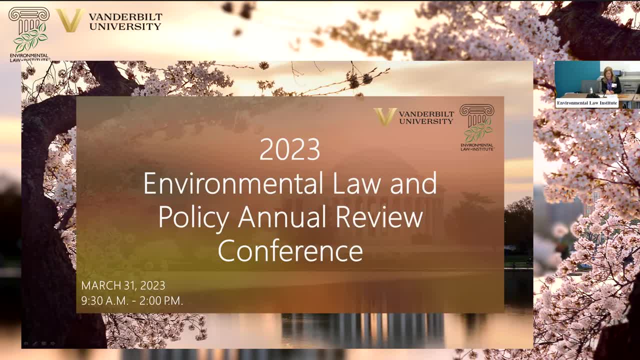 But what I'm here to tell you is that these are hard-pulled calculations. The term ESG originated in 2004 with the US Global Compact, by a whole bunch of financial firms like HSBC, Goldman Sachs, Morgan Stanley. Again, these are the folks who said: well, this will be a useful investment strategy. 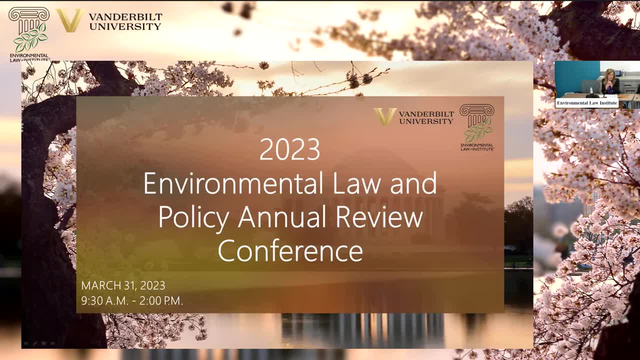 We can aggregate these things And we can create new investment funds. So I'll conclude. I'll look forward to your questions. I'd love to take this apart more fully, But just wanted to provide the larger context, I think, some of the cautions that we need. 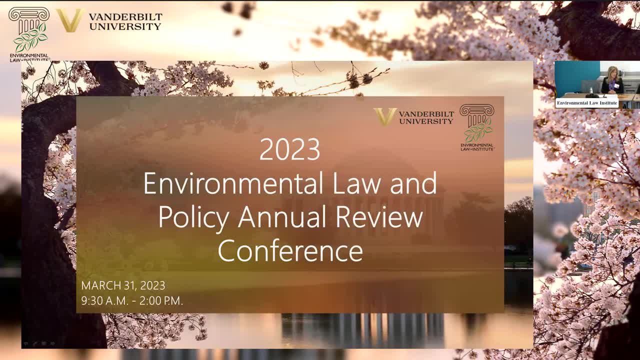 to look at, At the same time certainly agreeing with our wonderful authors of the article and some of what Steve had to say upon I look forward to your questions, And you're such a font of information. I wonder: does CERES have a white paper or something that includes a lot of the data? 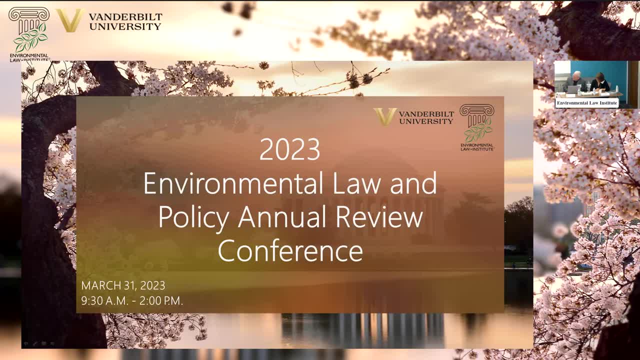 that you just mentioned. I can imagine that would be very useful for people. Yes, We do FreedomToInvestcom. I can't remember if we bought com or org. Many of the articles are there, But then I have my own private working paper that I'd be happy to share with you, Mike. 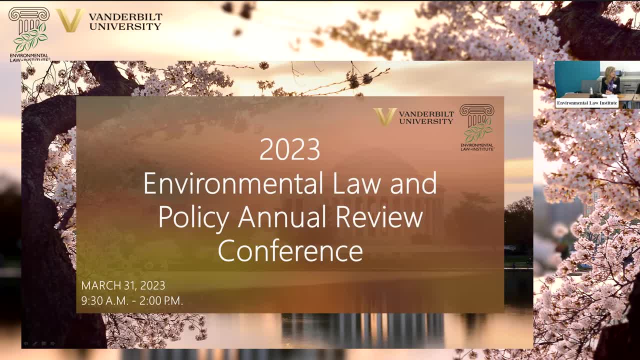 That'd be great. Thank you, Yeah, that's great to get that perspective. And it's funny that you quoted Ann Simpson on the we're not woke, we're awake, Because she was going to be on this panel but we had a scheduling problem. 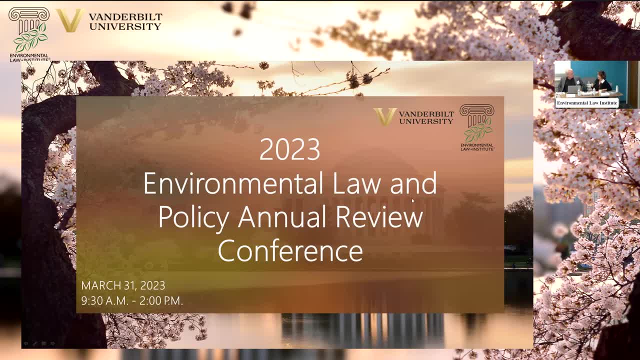 But when she was at CalPERS was here, I guess a year and a half, two years ago, So we've got a real downgrade And she knows her stuff Well. it's wonderful to get this range of perspectives. And before we circle back to other commenters again and questions, I want to ask Adriana. 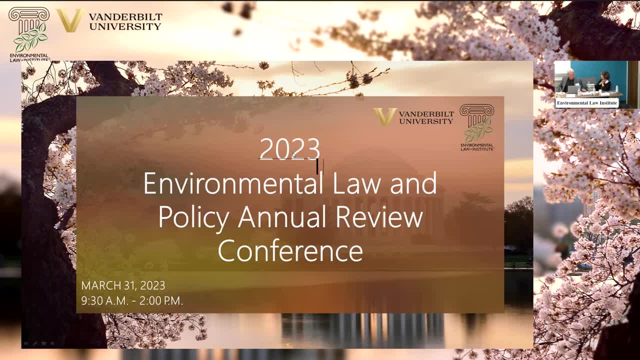 and Jill if they want to respond to anything they've heard. Adriana. Well, I was going to say what I suspect you were going to say, which is related to the names rule that Stephen mentioned. So it turns out, Jill and I actually have a paper on that. 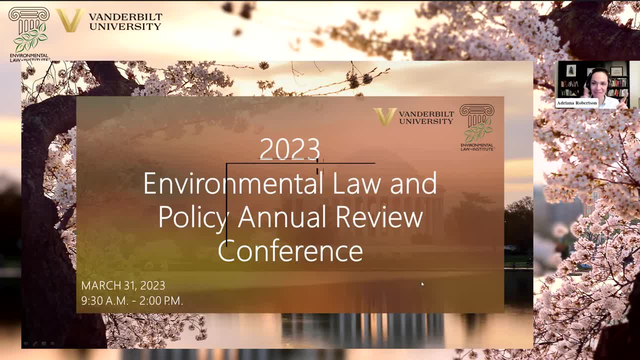 And the reason we're not at this conference is that we're presenting that paper at another conference. So we'd be glad to send you the link to the working paper. We actually, I guess we do disagree in the sense that we actually think that the proposed 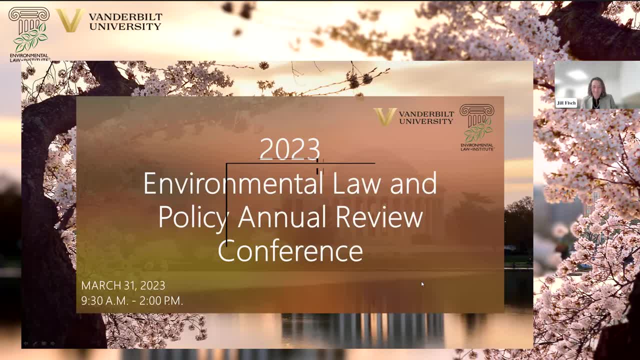 names rule is not. not only is it unlikely to be helpful, we actually think it is actively potentially harmful to ESG investing and to investor protection, And for a couple of reasons. not because we disagree, we are very pro-truth. We are very opposed to misleading investors. 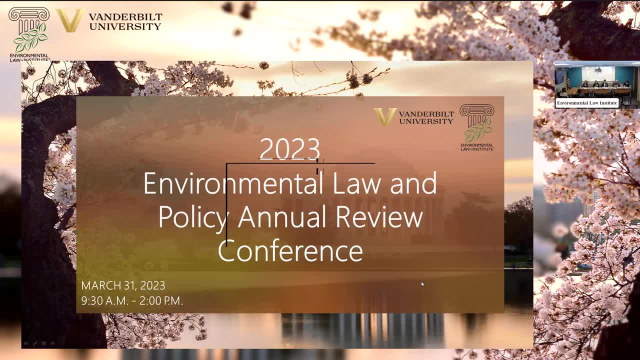 We are anti-fraud. Let's make that clear. We are all on the same page on that. As we understand it, as we read the proposed names rule, it actually seems to make it very, very difficult to engage in a wide variety of well-known, well-respected, totally acceptable. 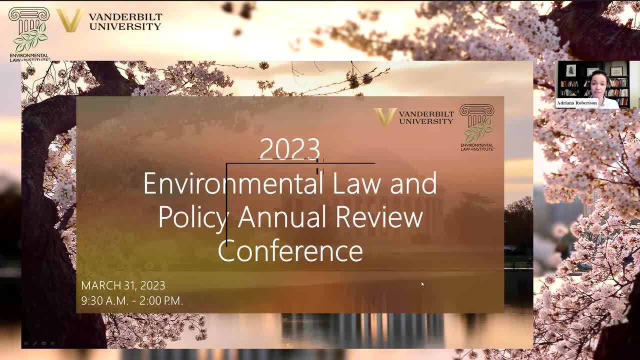 ESG strategies. They don't fit well within the proposed names rule framework. Moreover, we do sort of a fairly simple example to show that. you know, it's just really hard to give investors a clear sense of what they're buying just by putting it in the name. 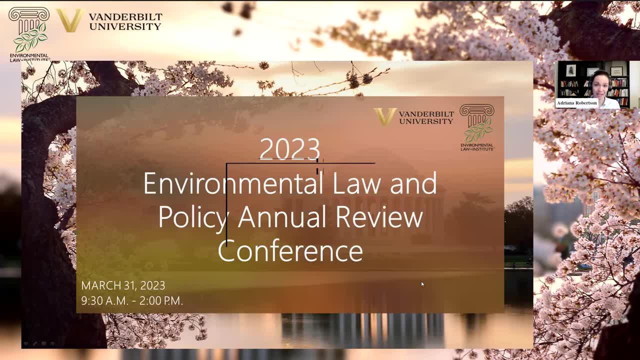 And so we do some simple examples to try to make that point and drive it home. That being said, you know it doesn't mean we don't think that more disclosure is better. We're just not sure that this particular rule is the way to get us there. 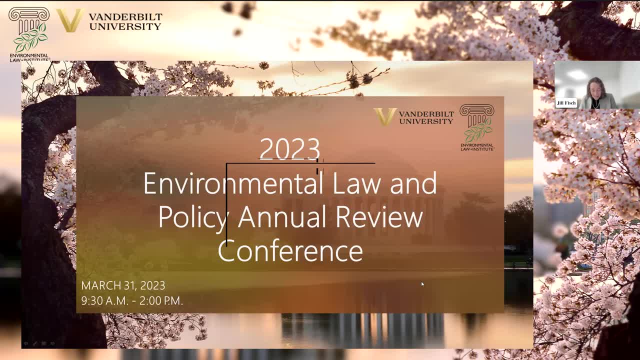 Yeah, I agree, of course, with all of that, But I guess you know we're academics. We are working really hard in both of these projects to try and figure out what's happening in this space from a market perspective and also what seems to be motivating the SEC and 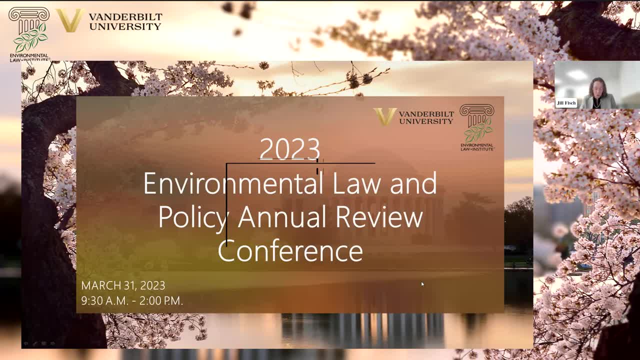 better markets and a bunch of the people who are supporting more regulation, And I guess you know, Steve. maybe offline you could help us out With a little bit more specifics. So in your remarks you talked a lot about potential problems and future problems. 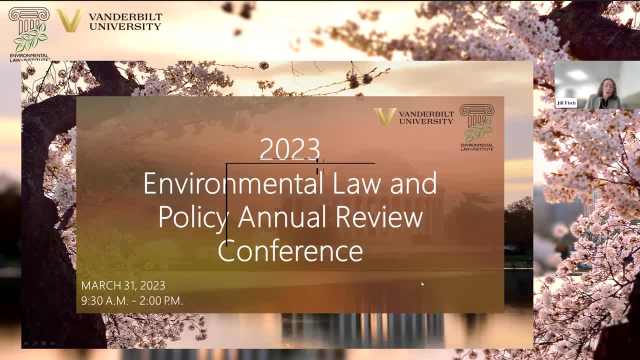 and patterns of misconduct. And when I presented our other paper earlier this week, one of the people in the audience said: well, what is the indication that there's really fraud in the ESG space? Is the SEC bringing enforcement actions? Are private litigants bringing enforcement actions? 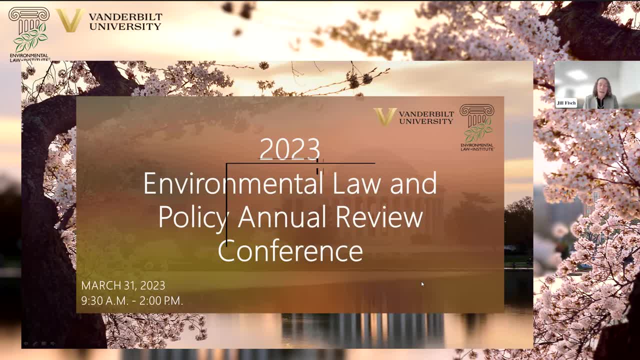 Because, as Anne is at the first commentator, as Anne said right, there's lots of litigation in the mutual funds space. There's lots of potential for class actions. When we went through the SEC's rule, the SEC said, well, there's all this money, investors. 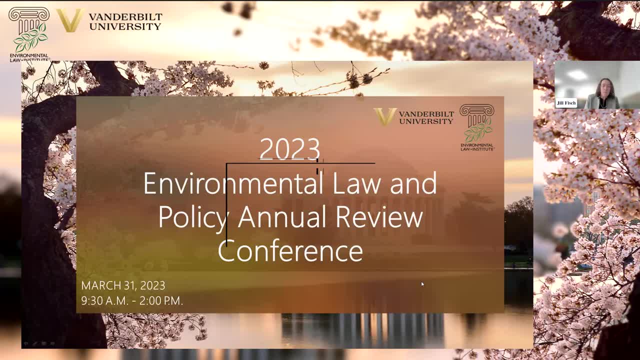 are flocking into ESG funds and that seems to be a problem, But you know, we're not really judging what goes on in the market. If investors want something that is ESG and if, as our data suggests, it is measurably different from the other alternatives in the market, 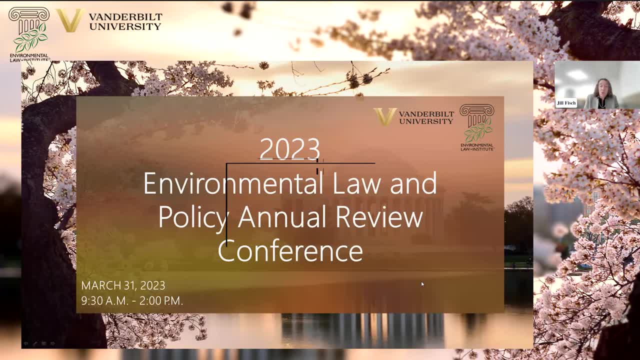 you know why exactly should regulation be concerned? Why is that a problem to be prevented? So you know, I think that you know I've opened a door that probably, Steve, is too big for you to answer here. But you know, if there is concrete evidence, we'd love to see it and examine it more carefully. 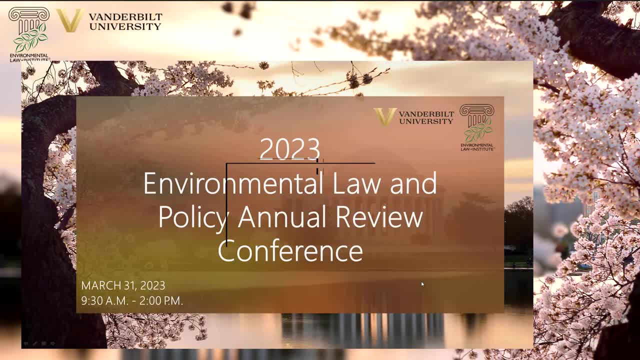 Well, if I could, the all very interesting input and comments from everybody, a couple things I just wanted to offer in response, not necessarily in disagreement, but yes, on some things. I think that the label tweaking- I think Ann used it- is, I think, a little bit off the mark. 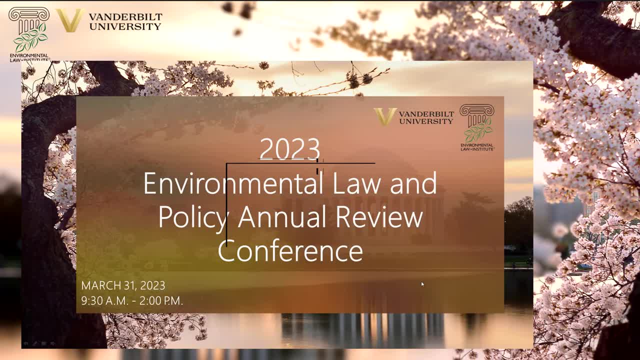 for really three reasons. One is: a lot of the discussion, except for the last very reasonable question, tends to gloss over the potential for abuse, the history of it and the potential for it going forward. Tweaks, kind of regulatory tweaks, doesn't really have an aperture to count for that. 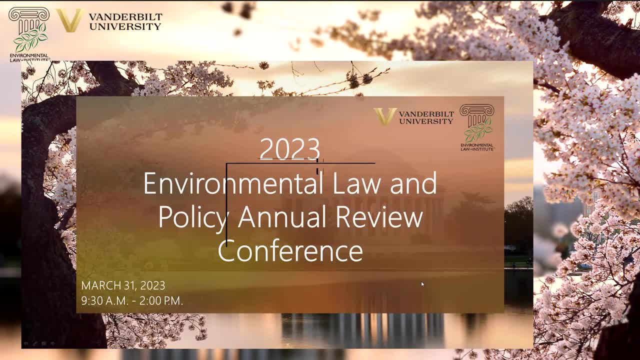 And, in our view, the scale of the ESG movement, the complexity, the enormous popularity, which is a kind of engine or driver. that in some ways is very good when you think about the larger issues, And that state is nevertheless, in our view, inherently perilous for investors. 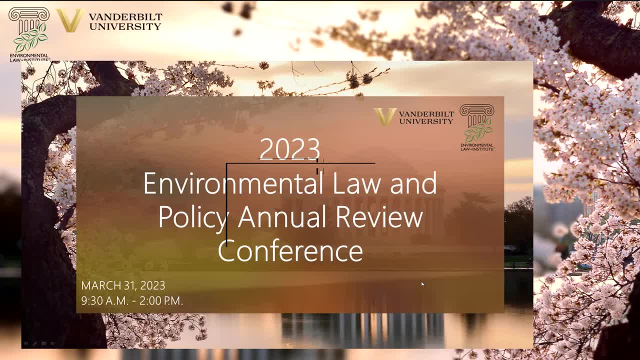 And the financial industry- I hope I don't offend anybody, but in the view of better markets- is always looking for opportunities to make loads of money and to take advantage of this kind of context. The other thing is that tweaks, I think in a sense devalues the ESG disclosure rule. 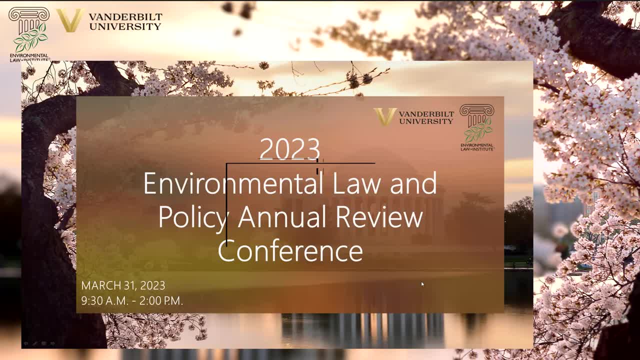 that the SEC has, The SEC put out and the names rule. I mean one thing: you know these are really important things and, as the SEC said in the release, it's both protective and it's constructive. It's helpful to the movement itself. 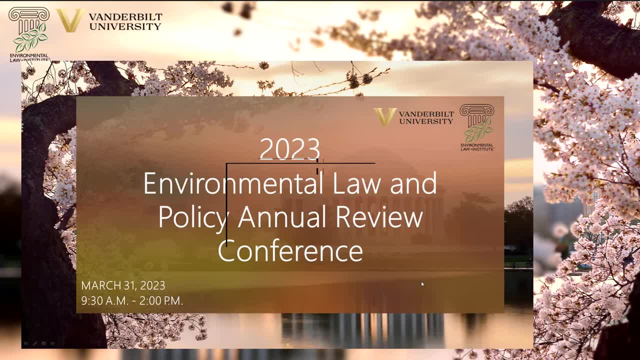 And then, finally, I would say that as we watch this fascinating and important movement go forward and evolve Yet further, I think we're going to need to be vigilant again, not be too complacent and constantly look for new trends and reasons to be concerned on both fronts. 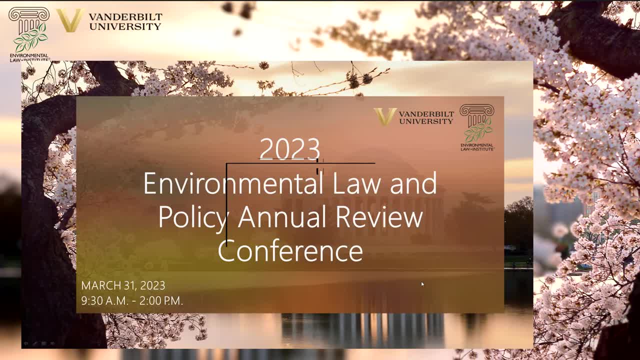 Is there fresh abuse, new varieties of it? Is there a need for even more disclosure requirements and guardrails? And then, finally, on the issue of whether there really is much abuse, it's a very fair question. I didn't say this in my remarks. 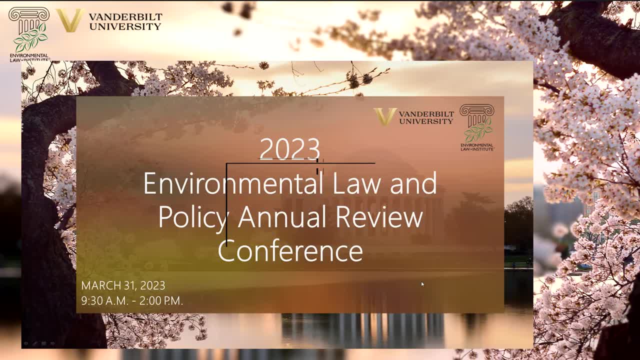 In an earlier draft I had just a reference to the two enforcement actions last year against BNY Mellon and Goldman Sachs in November of 22.. Mellon was May 22.. There's still reason for the SEC to be on alert in accordance with its own risk alert. 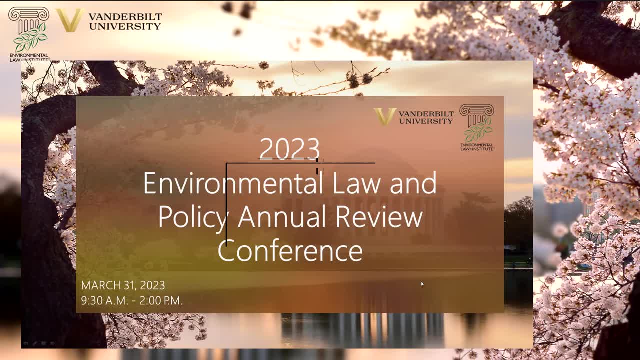 There's a reason why they're throwing lots of resources at that And if Yes, It seems that all of those steps and the layering of regulation actually prevents abuse. that's an argument for those measures and their success. It's not an argument that we should just stand down. 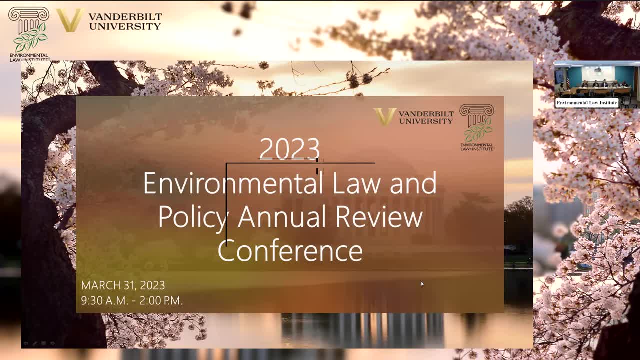 There you go, Thank you. I just wanted to see if Ann or Katherine want to jump in on this or if we should go to a question. Yeah, no fair comment on Steve's part. I didn't mean to be pejorative about using the word tweak. 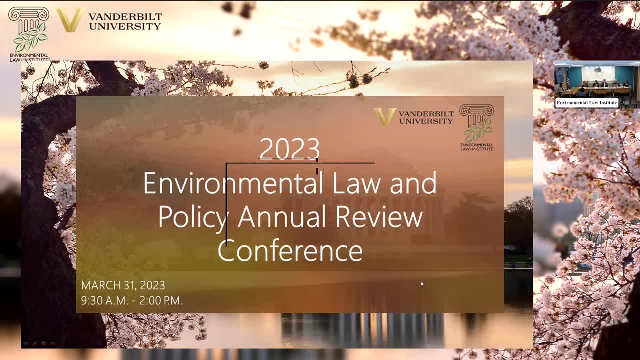 It was just relative to what Steve's calling for is avoiding abuse and legitimizing a movement and getting more clarity or disclosure, and I was only using the word tweak relative to these blanket boycott bills that are happening. I knew he wasn't going to like the word when they say that. 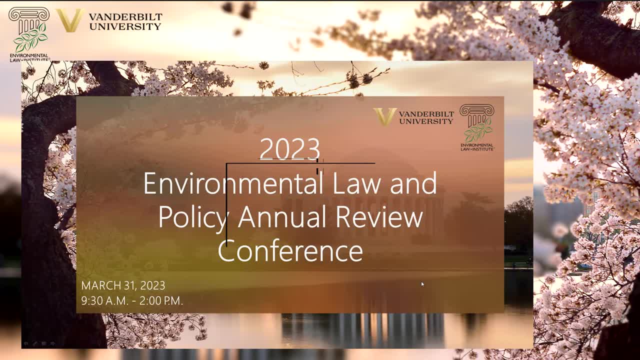 But he did. I'll thank you for that. I would say I would modify it in a subtle but important way, the phrase you've just used, which is to legitimize the movement. In our view, it's more about creating the regulatory environment that maintains the integrity of it and lets it get as much legitimacy as it may deserve, as long as it doesn't victimize people and deceive them. 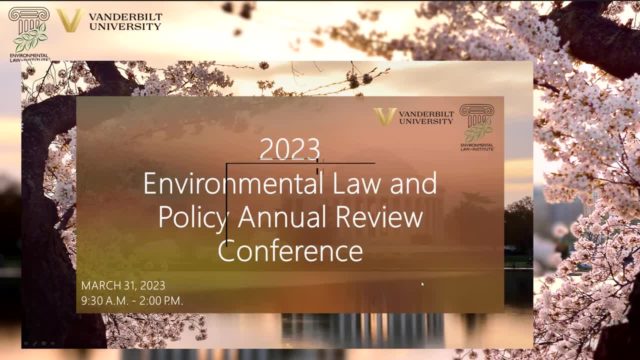 And as long as it really gives them the information they need, in accordance with the cornerstone principle of securities law, which is you got to give them all the material info. It's got to be truthful, It's got to be timely, And then let the market decide. And there I think there's a lot of common ground. 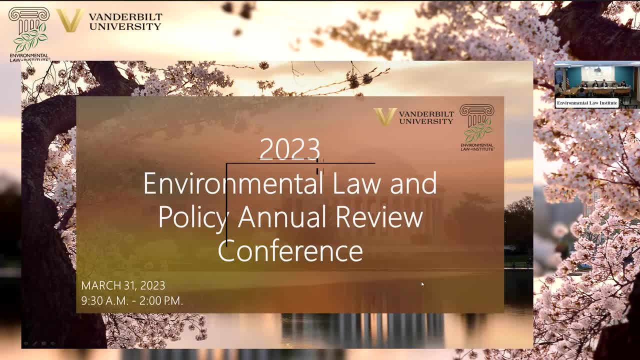 For sure, And I think I shared Jill's question about if there's abuse, you know, let's take a look at that If people truly have been abused as a result- And I'll look forward to their article on the naming. There's another aspect that's important here. I think a lot of the work that I do is with social psychologists and looking at the role of social norms in steering behavior. 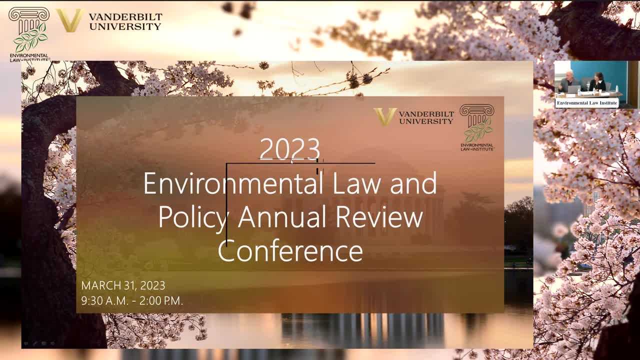 And we all say that we make our own decisions, And yet we all tend to do what others around us are doing most of the time, even though we deny that that influences our behavior. Best way you can predict most behaviors is by looking at the circle of people around you. 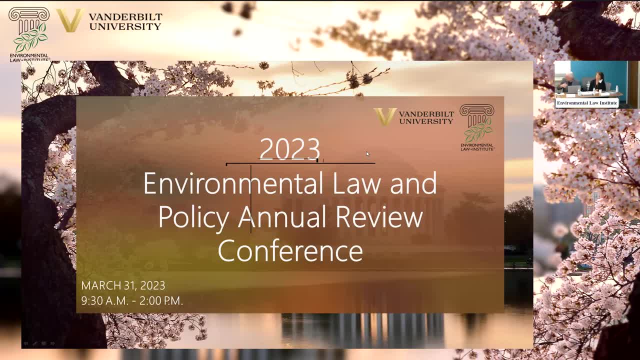 And as you increase the amount of attention on ESG funding and so forth, you create this sense of common behavior out there among corporate managers and investors And and individual investors, investment managers. So I think there's also a value to having a fairly expansive approach to ESG, just to create that sense that, hey, I'm doing what everyone else is doing. 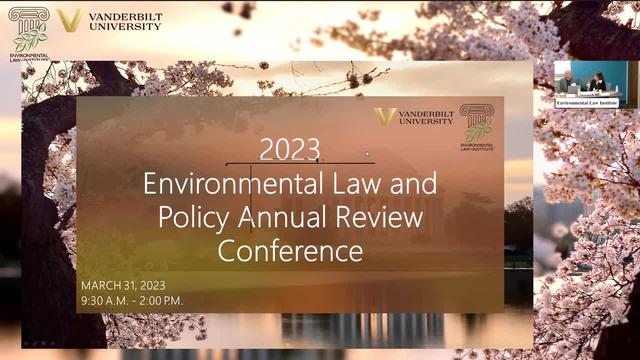 And that in of itself, could be an incredibly important driver in this area. Thomas, do you want to ask a question before we start to wrap up? Sure, So this is a question for the authors and the panelists. The paper concludes that regulations might not be necessary because ESG funds deliver on the promises. 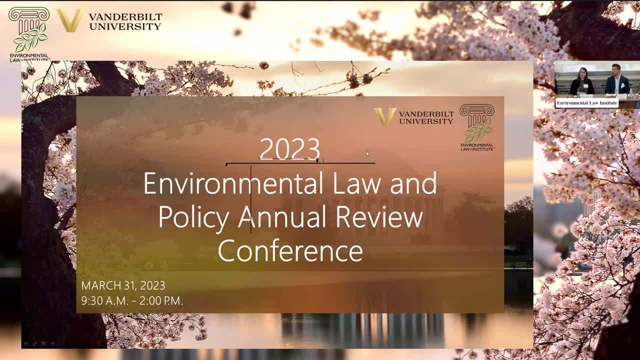 I'm wondering what are the environmental impact of ESG on other business, And I'll tell you why that was: environmental dangers, if any, of subjecting ESG funds to these heightened regulations. So great question. In the paper we worry about regulatory burden. 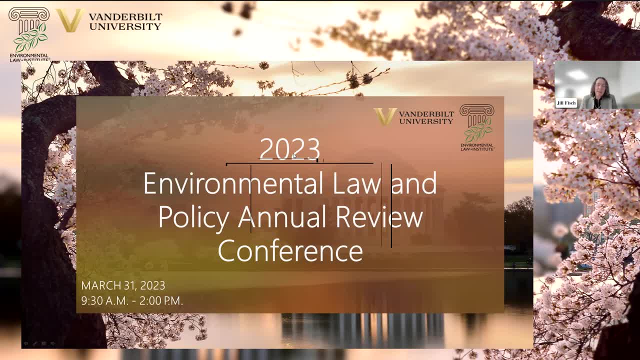 Obviously, one of the challenges in market regulation is: if you increase regulatory burdens, you're going to limit innovation. You're going to have funds that are risk averse With respect to the names rules. since Steve spent a lot of time on that, one of our worries- 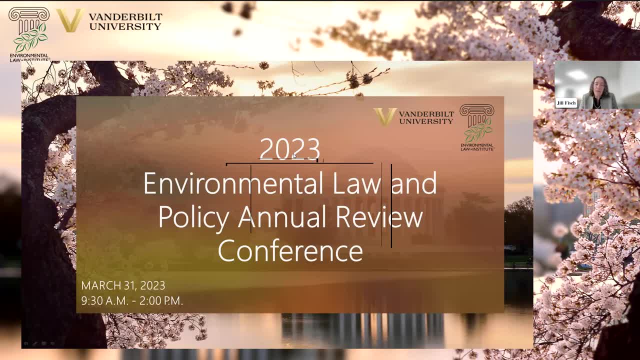 is that we won't have as much information conveyed through the name. A name is an imperfect measure, But I can always stay clear of any names rule problem by calling my mutual fund Fund A or the Magellan Fund and not calling it an ESG fund. 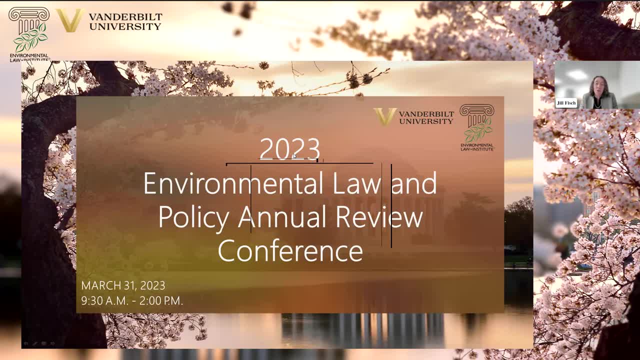 And since we know that a lot of investors use shortcuts, how are they going to find ESG funds if the name doesn't convey any information? With respect to other disclosure? other disclosure is a great thing. Investors should be able to know a fund's investment strategy. 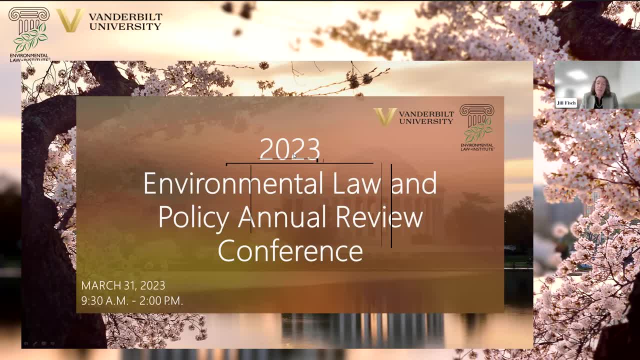 what kinds of securities a fund excludes, what kinds of factors it takes into account. As I said, we've been watching this space really carefully And we've been looking not just at the fund names but on the disclosure on fund web pages. 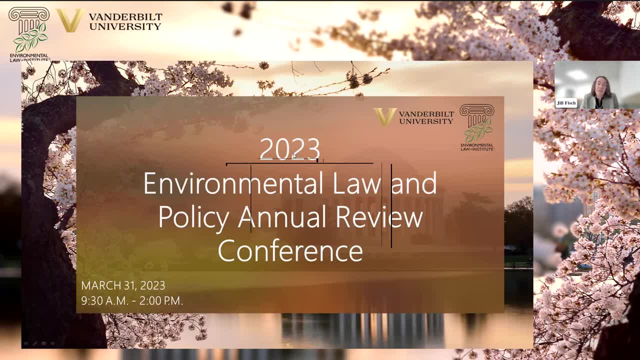 on the filings that funds already have to make with the SEC, And we see that funds provide a tremendous amount of information. So when we're talking about well, funds should be required to provide more or funds should be required to standardize. 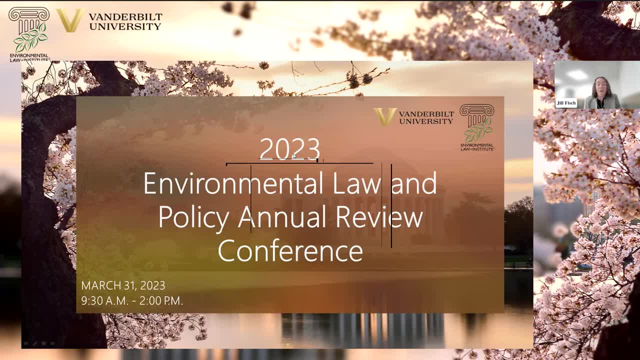 standardization is another word for well. let's not have outliers or let's not have all possible investment strategies. Let's require funds to fit with one of the SEC's three proposed buckets, And we think that's costly when investors want a variety. 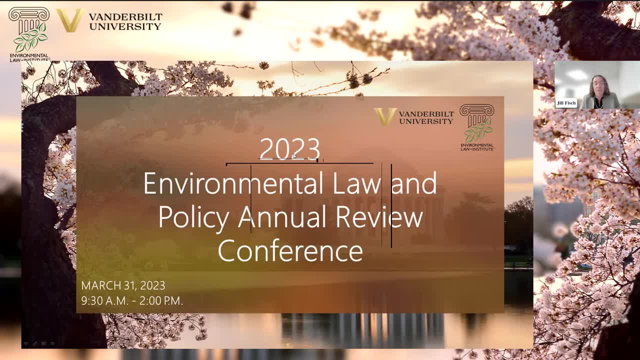 of different things and want to achieve different goals with how they invest. Go ahead To chime in, I'll wait my turn. I just wanted to say, just seconding, what Jill said, the other downside of standardization is this is, as we all know, a really young market. 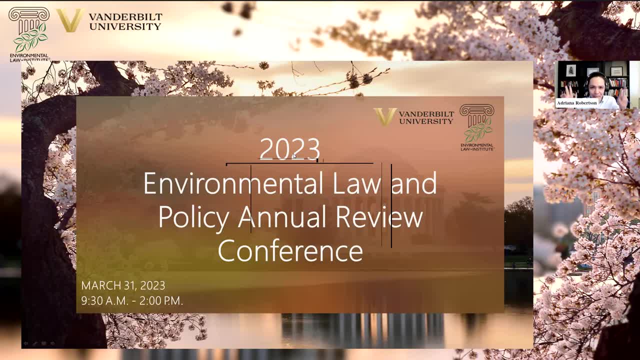 It's an evolving market. We don't know yet what the best, or right, or wrong for that matter. answer is: And the more you look at it, the more you'll see. you know you impose regulation, the more you impose cost. 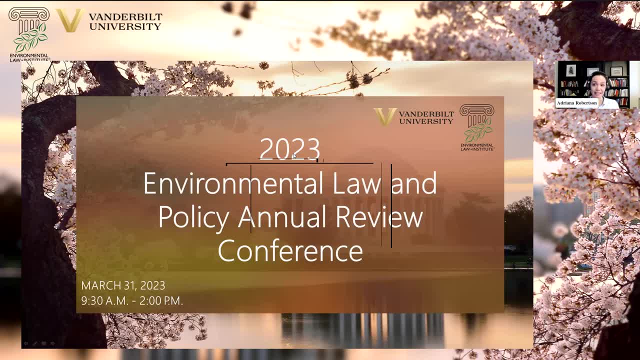 the more you try to force standardization, we worry you're not going to get the innovation, We're not going to be able to get to the kinds of products that investors are going to want, And we think that that's just like the downsides there. 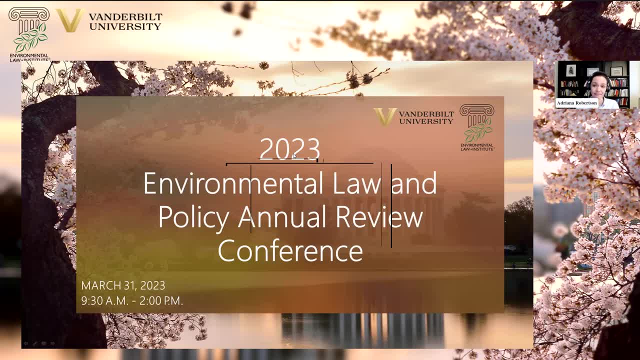 we think are also really important to weigh Dave. Yeah, real quick On the names rule. I mean, the flip side of the coin, already talked out, is, of course, that it is an extraordinarily, extraordinarily powerful influencer of investors. 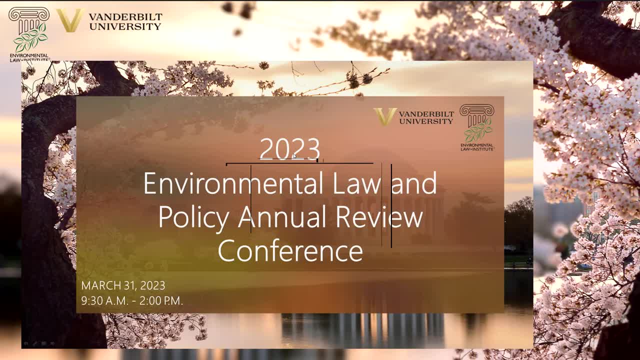 I mean, I think everybody in the room knows that that's been a longstanding concern And the fact is there's repeated cases demonstrating that adding an ESE term to a name can basically overnight increase your flows dramatically. So it's sort of playing with dynamite. 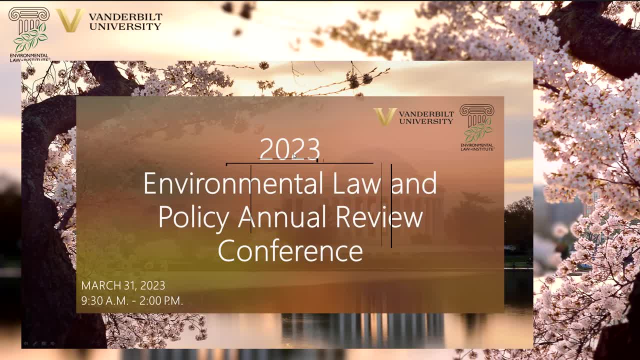 And that's why I think, that's the reason you know- that should trump the concerns about maybe struggling with how best to describe a fund. The short answer to the very good question that started off this round of discussion, to my way of thinking, is that, in the long run, 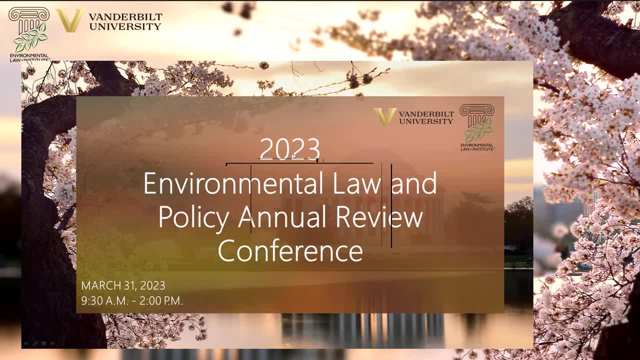 the additional regulatory requirements are, of course, going to be good for the environment as well as investors. That's our core thesis. And finally, the notion of regulatory burden. it is, you know, it's a constant refrain. It's one reason why better markets remain in business. 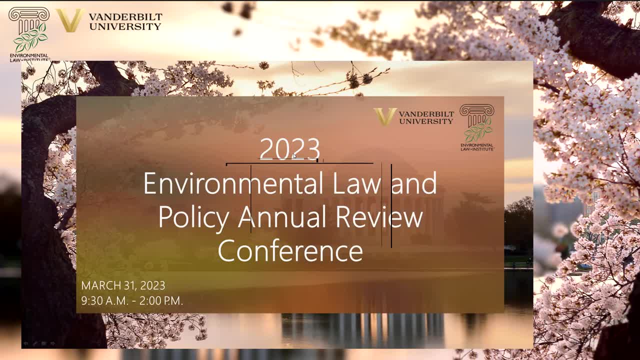 Because we feel the need to push back against the contentions that regulation is overly costly, overly burdensome, and also, especially, push back against the notion that it stifles innovation, Because we just don't see that. I mean to the point made earlier. 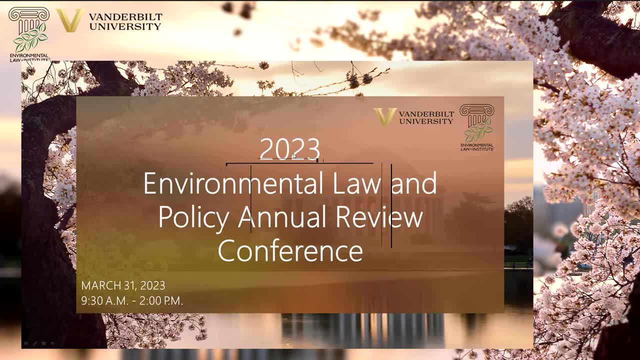 what's the evidence of abuse? Let's have that discussion. I think it's very good. Let's also have, at the same time, a discussion about, well, who is really in the financial markets, in the fund space, who's really deserves sympathy because they couldn't innovate? 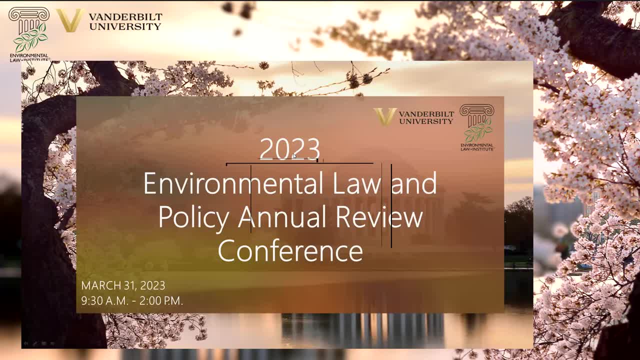 Let's find concrete examples of that. Great. So we're running out of time, But I want to put two big ideas on the plate, just because this is both a policy event and an academic event. One is just- and I think Anne raised it- the question of time. 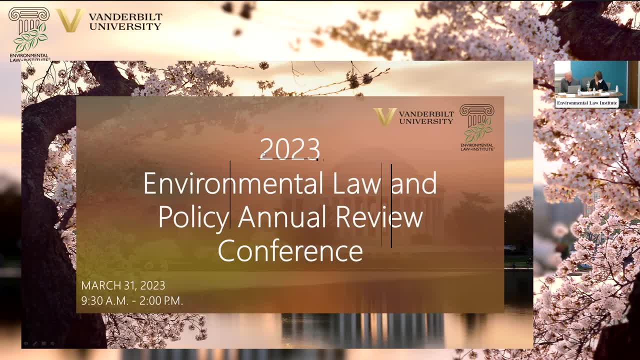 If I invest in a pension fund, I'm not that concerned about the returns next year and the year after. I really care that there's going to be a big pot of money in 10 or 20 or 30 years, And so how does that factor into all of this? 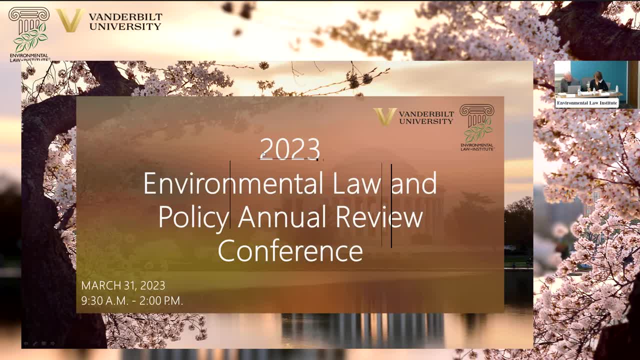 And I know it's hard for academics when you try to do this kind of research, to look forward. You all were able to look two years backwards, which is incredibly helpful and a powerful paper. I'm just curious about how we deal with this question. 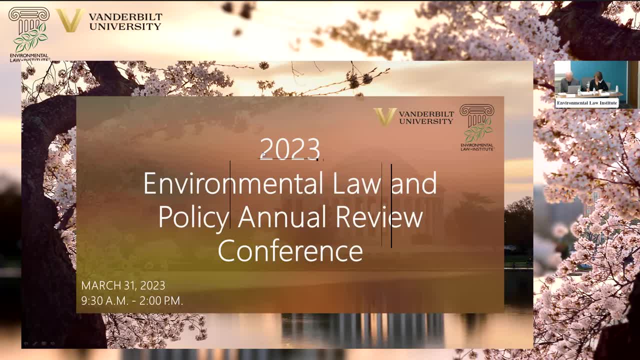 about whether these funds- you know funds- might perform better over time, because they are considering factors that are going to grow in importance over time. That would be one, And the second big picture one. and if you can answer all these in 15 seconds, that would be awesome. 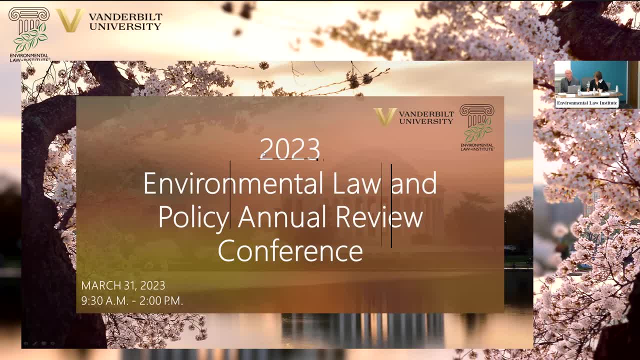 The second one is universal owner theory. So as we get more and more asset managers managing massive index funds, do they own the economy, in effect, and therefore benefit from owning a large basket of stocks and therefore benefit from reducing the negative effects? Yeah, 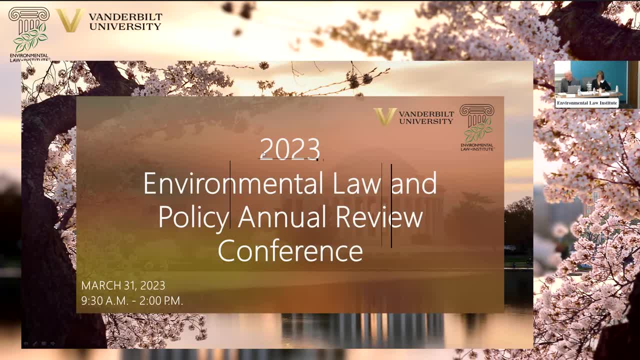 So I think the question is: is that the question of what are the negative externalities of the companies in that basket, rather than benefiting by any one company making more money? Does that have an effect on our thinking here, Or what's the status of that looking forward? 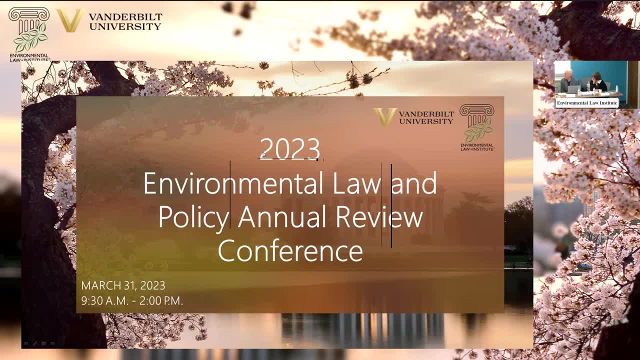 So in 15 seconds, Professors, Any thoughts on either the universal owner question or the long-term horizon question? I'll give you 10 seconds on the long-term horizon. I guess our view is there's lots of different investing theses out there. 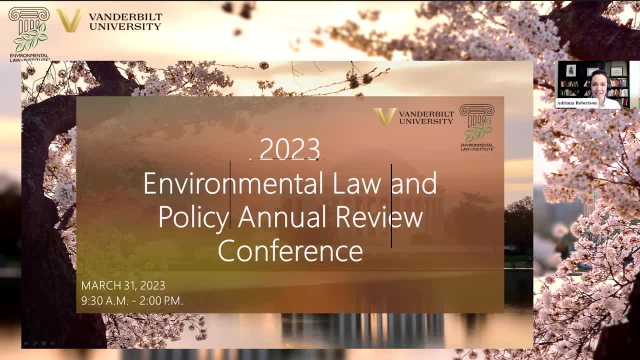 We don't typically say: you know, any particular kind of stock-picking strategy is legal or illegal. so if we have an investing strategy that says that there's going to be a transition, that is going to mean that these particular companies are more valuable. 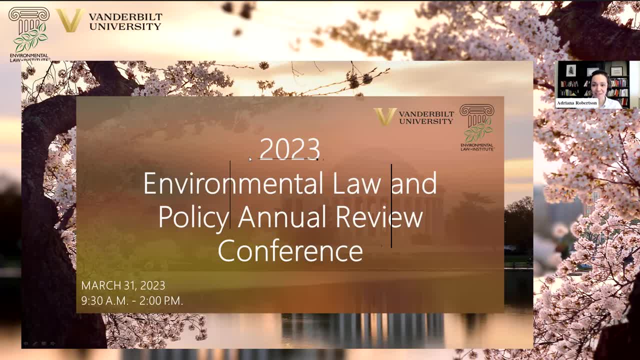 that's a pecuniary strategy that seems like a totally legitimate thing for a pension fiduciary to take into consideration. Doesn't need special regulation. That just fits within our current framework perfectly, Michelle, As does the idea that if investors want to buy,